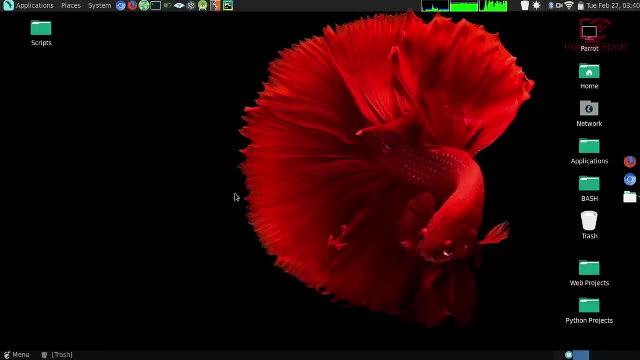 first thing you need to understand is that it will allow us to intercept the data being sent between your browser and the web application, So it's it's a great way of understanding how data is being transferred and how data can be manipulated- be manipulated between the client and, obviously. 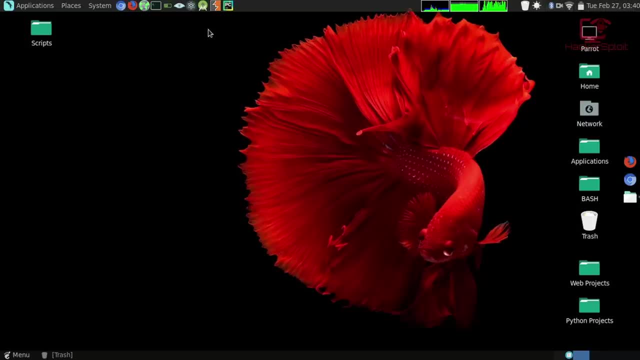 the web application. Okay, so the tool we're going to be using, as I said, is Burp Suite, and I'm currently running Pareto. So don't worry if you're running Windows or Kali Linux, it doesn't really matter, All you need to. 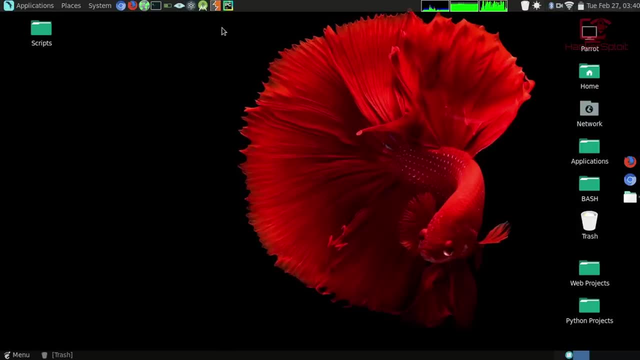 do is just download and install Burp Suite. It's pretty simple to get set up. you don't have to register, you just download the free community version. Now, obviously, down the line you might choose to to buy the professional version, which I do recommend and I have used, but I don't use it. 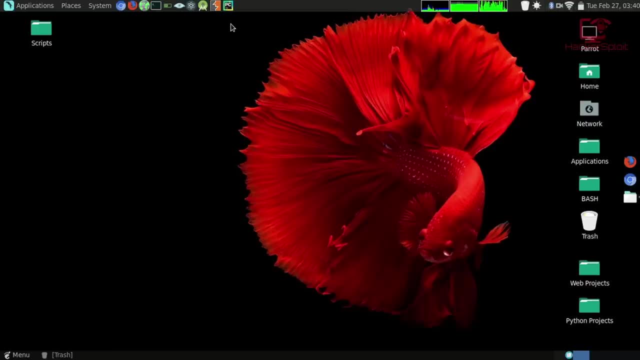 as often. I'm not, you know, specifically a web penetration tester. I'm more of a, I'm more of an offer web server penetration tester. So I really work with a different vector. So by default you can choose to bite. that's once you become experienced And you know you've chosen whether this is the 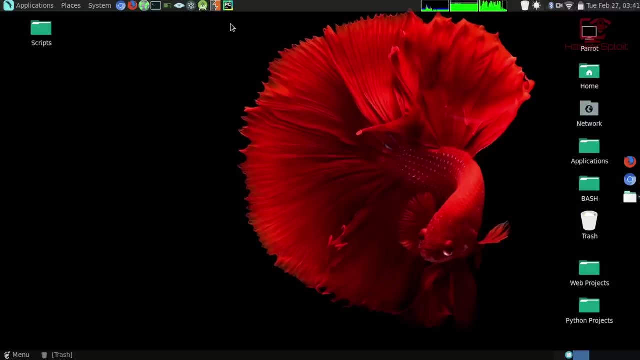 path that you want to pursue. It's a fantastic path. I know a lot of people who you know make good money with bug bounty, So you know it's something that you can look into as well. Alright, so let's get started with setting up the proxy. Alright, so this is the intercepting proxy that. 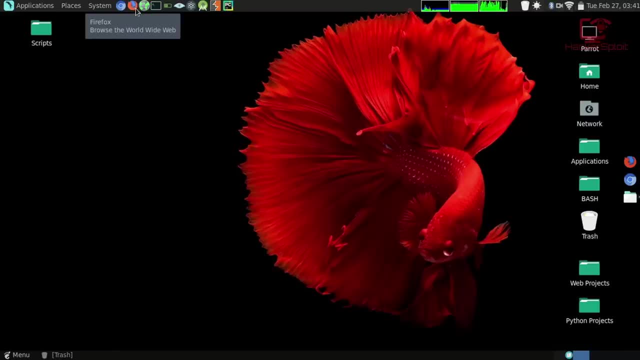 allows us to obviously to intercept the data being sent to and from the client and the, the web, the web application. So to do that we need, we can just do it through Firefox. So the browser I'll be using is Firefox. you can use whatever you want. 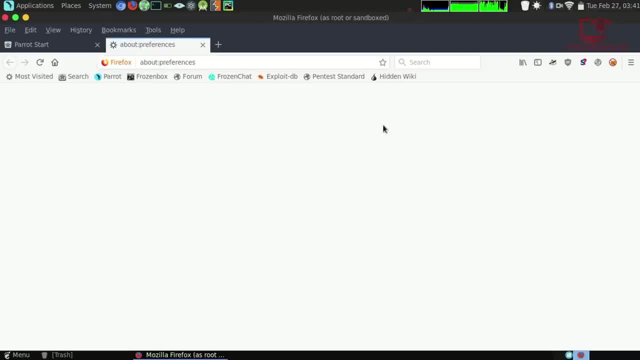 And by default. you want to go into your preferences. that can be found here. preferences, there we are. And you want to go all the way into the bottom here. that way it has the network proxy and make sure you go into settings. And you want to go into manual proxy configuration? Alright, 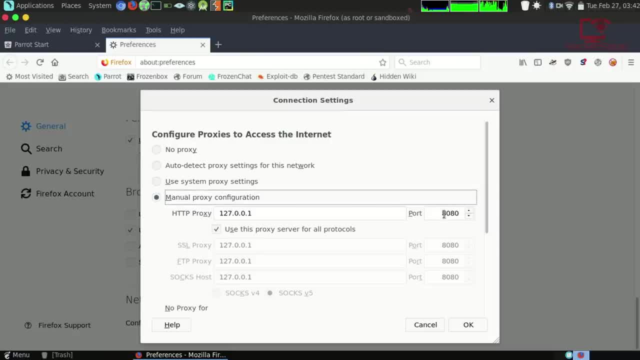 so this is where we're going to configure it To be the localhost, with the port set at 8080.. Alright, and then you want to make sure that the sir you use the server proxy for all protocols. So that is the proxy we're going to be using, and just. 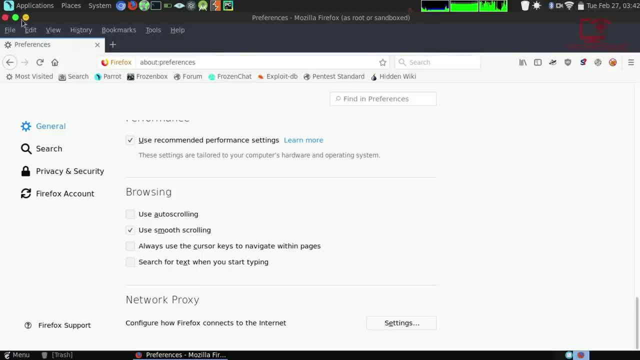 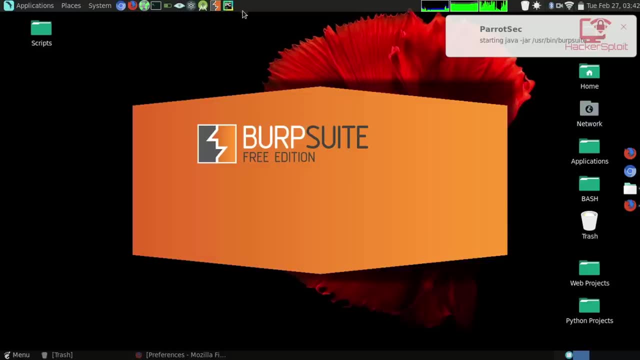 hit OK Alright, and once that's done, you should be good there. Now, you, what you want to do is just open up burp suite So you can search for it, or I have it already on my, on my little taskbar here. 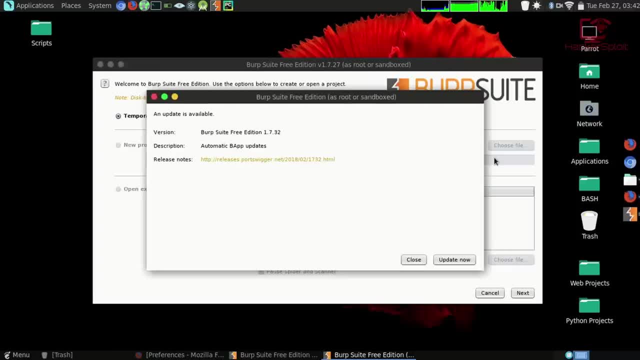 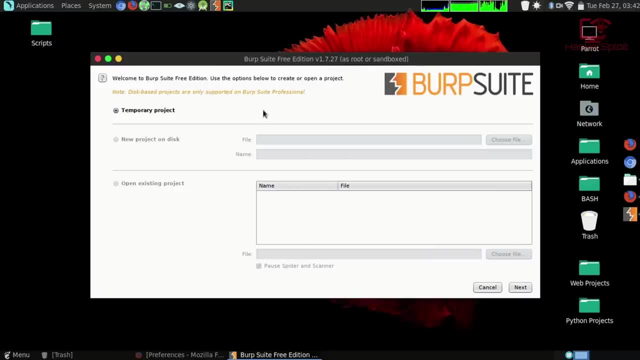 And I don't think I've updated it for a while, So probably need to do that later, But for now I'll just close that the update prompt. And it's going to prompt you: Welcome to burp suite. And it's gonna say: not depending on the 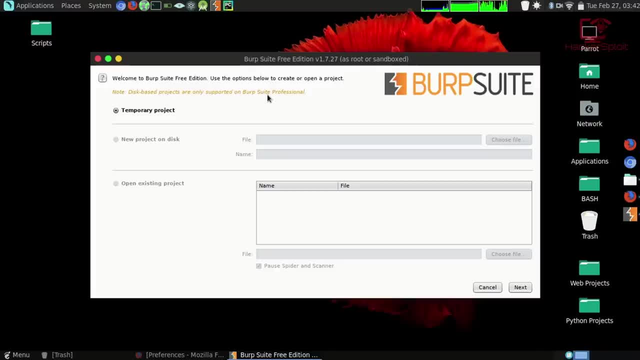 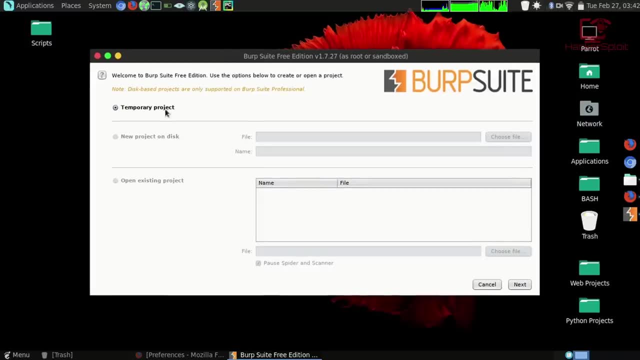 version that you've chosen to select whether you have chosen the community version, which is what I have here, or the free version, as it's called, and you then have the pro version. So, by default, the community version only allows you to use a temporary project If you have the professional. 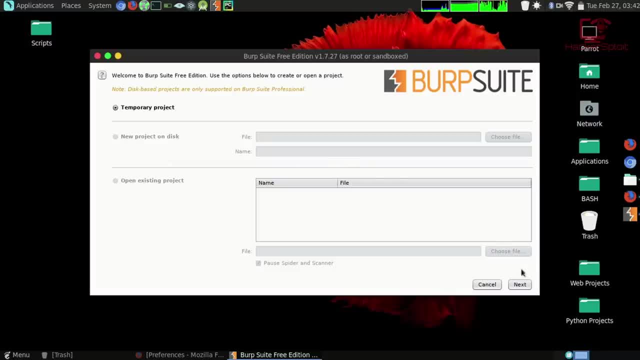 version. it allows you to save your project, which is, you know, great functionality as well. So just hit next. And you just want to hit use the burp defaults And just hit Start burp And just give that a few seconds to start it up. Alright, and 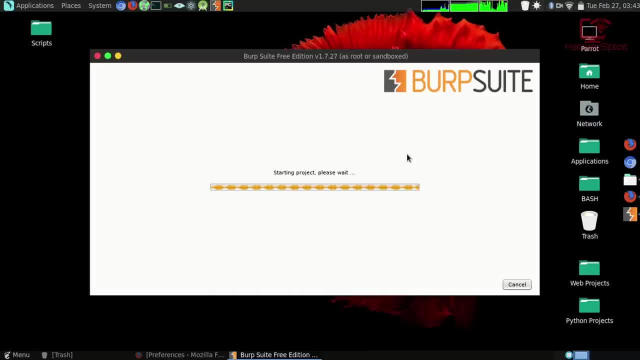 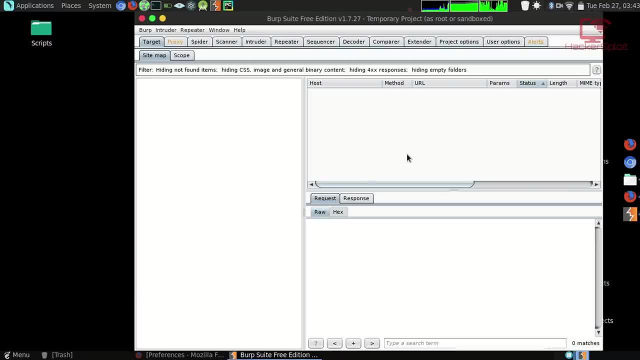 I'll explain the interface generally, but we'll be looking more into how burp works In the next video. I just want to get you set up with burp in this video And you understand what exactly is going on. Alright, so welcome to burp Now, by default again. it may seem a little bit. 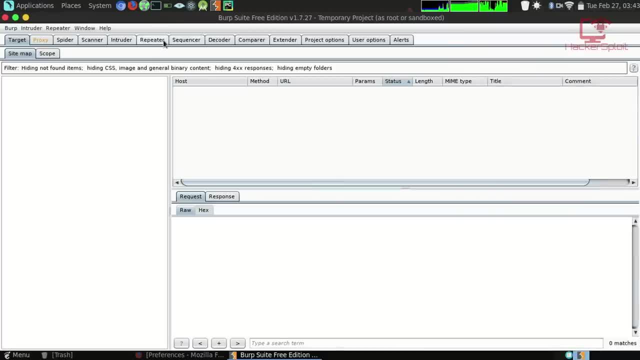 intimidating, mostly because, if you're a beginner, you have not heard of any of these of these words here and you don't really know what they're doing. Alright, so by default you have your target proxy spider, scan, intruder, repeater, sequencer, decoder, comparer, extender. your 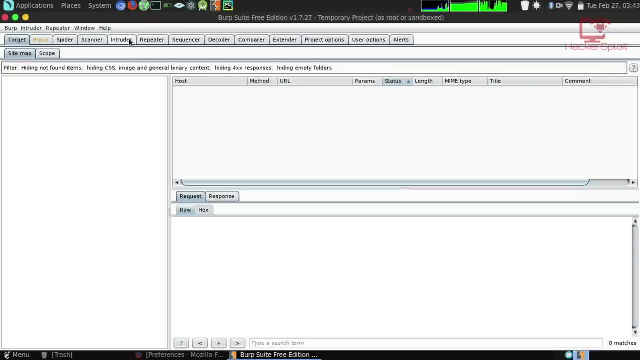 project options, your user options and alerts. we'll be going through all of this as we, as you know, perform real world testing on our, on our vulnerable, on our vulnerable target. I'll be showing you how to set up damn vulnerable web application soon, and many others, But for now, 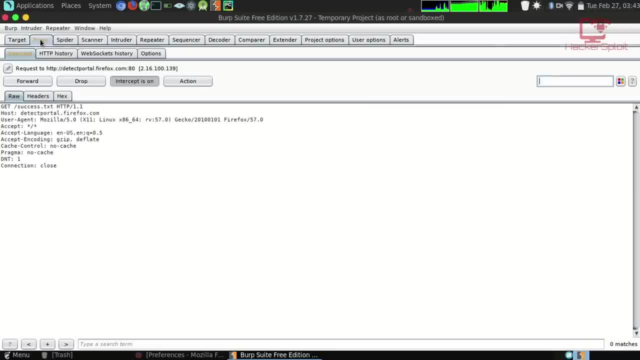 just focus on burp suite, Alright. so by default you want to just go into proxy, Alright, and for some reason I already have some data. So you know what. I'm just going to leave that as it is. I just want to turn our intercept off, So 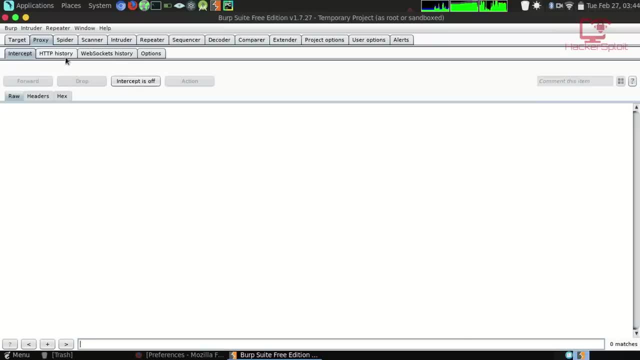 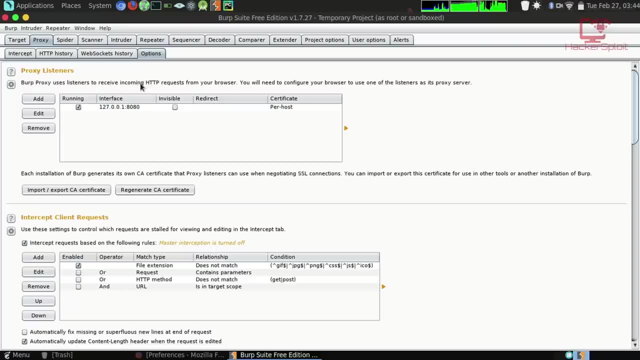 we're not intercepting any traffic as of yet And you want to go into your options And you want to make sure that your proxy listeners- as you can see, birth proxy uses listeners to receive incoming HTTP requests from your browser, So you have to make sure that your proxy is set as the as the one. 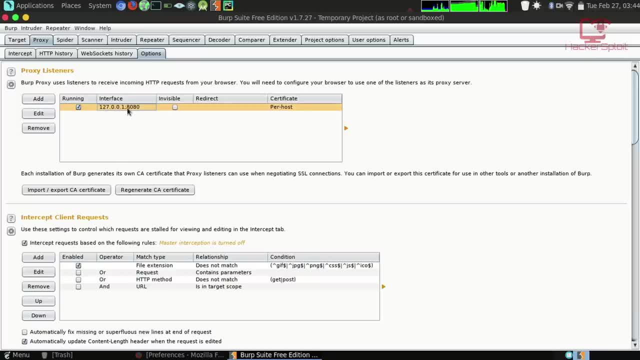 we set in Firefox, which is the localhost, 127, point 0.0, point one, and the port is 8080.. And make sure that that is running All right. you can also create your own and add it here And you. 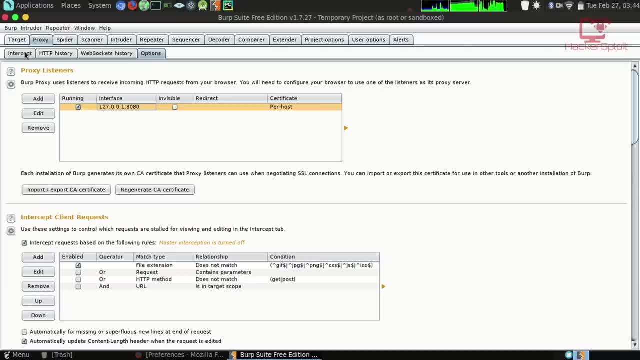 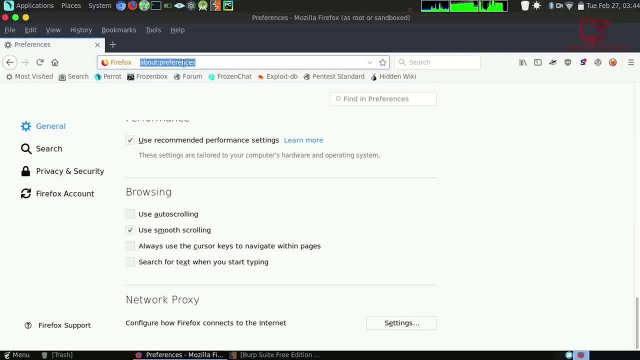 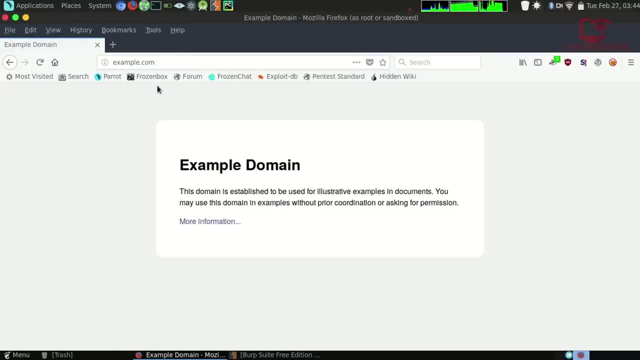 can also remove it. So you get the idea Now, by default, if I just go back to my intercept, if I just go back to my browser, and this is where the real magic happens, If I just, you know, if I just open this and I type in a simple test site, examplecom, and I just hit Enter, all right, 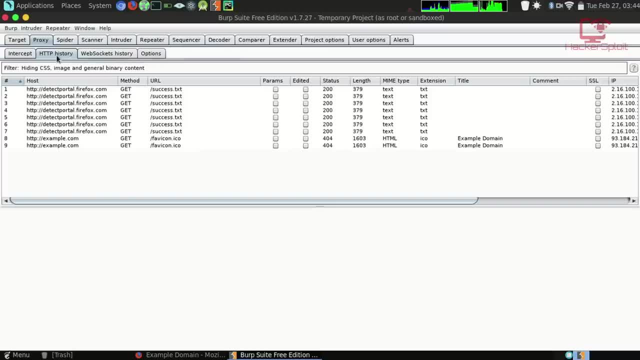 it's going to load it up here. But if we're going to burp suite- and I go into HTTP history- you can see that by default there are some off Firefox portals. you know some get methods here, but we'll be looking at all of these methods or 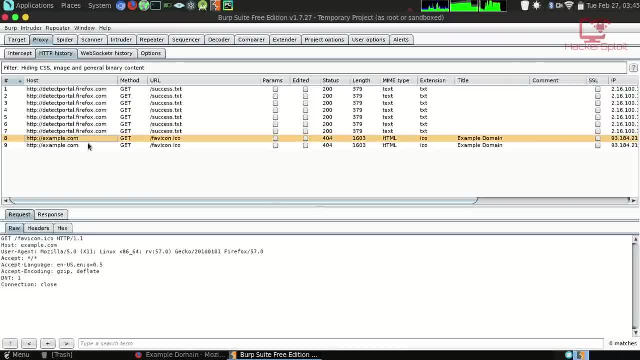 requests By default. you can see that the examplecom, the examplecom URL that we entered, you can see there is a get request And, furthermore, if you go down to the bottom here, you can see there is some more information regarding what a request was sent to the web. 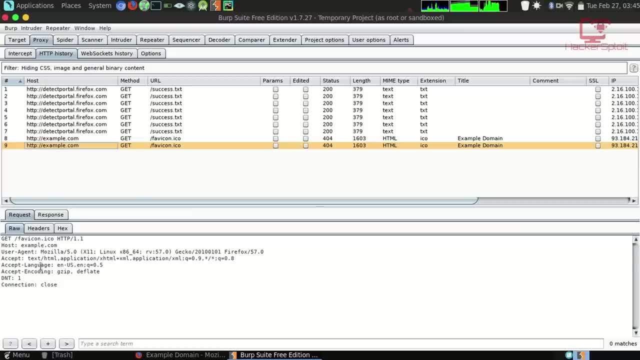 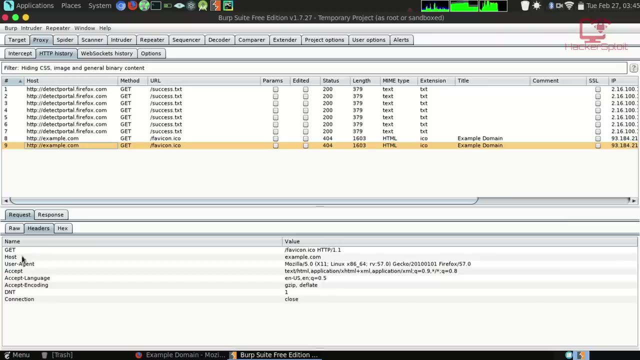 application Or so by default. you can see that the host was examplecom And it gives you more information like the accept language, the encoding, the connection, And if you look at the headers, you can see that the the header shows you know very, very clearly. 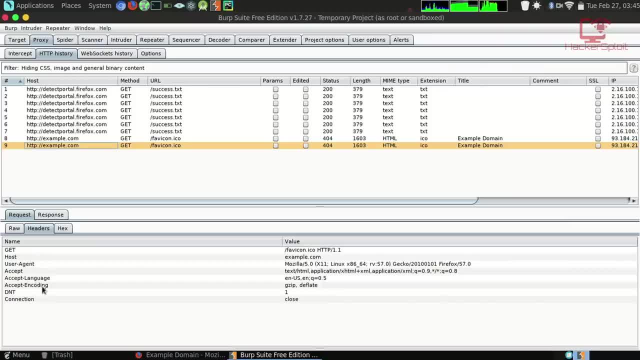 you have your get host user agent, accept language, the accept encoding connection etc. etc. So you might be a little bit confused if this is your first time hearing about. you know headers and the request and response pairs, but don't worry about that, we'll get to. 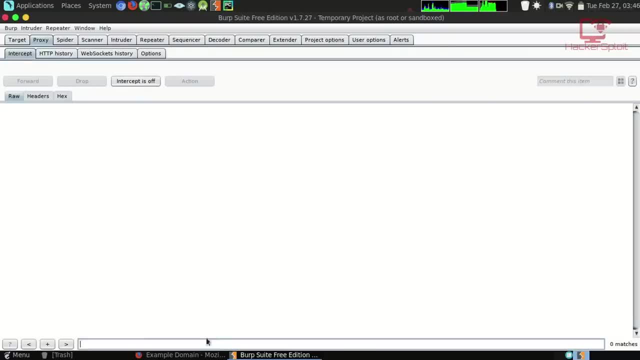 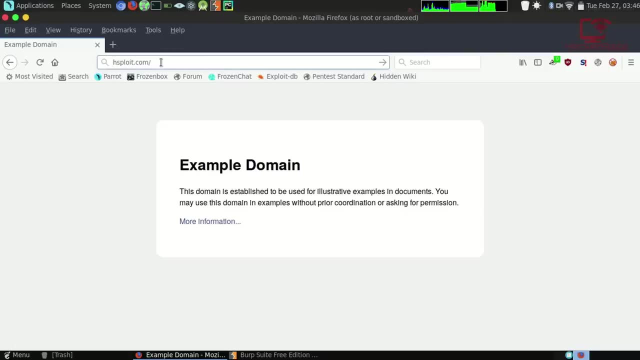 all of this For now, if I just go back into intercept and let me just open up my browser here And we open something like the- my web, my website, which is hsplaycom. So before we do that, I just want to hit intercept on. Alright. 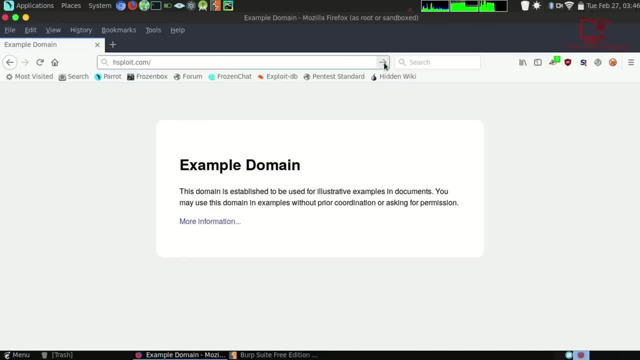 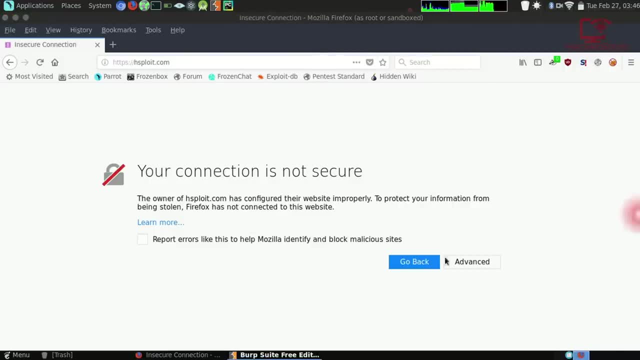 so now it's going to intercept actively And we're just going to hsplaycom And I hit go All right, now by default is going to tell me that essentially that my connection is not secure. don't worry about this, just go into your and just add this. 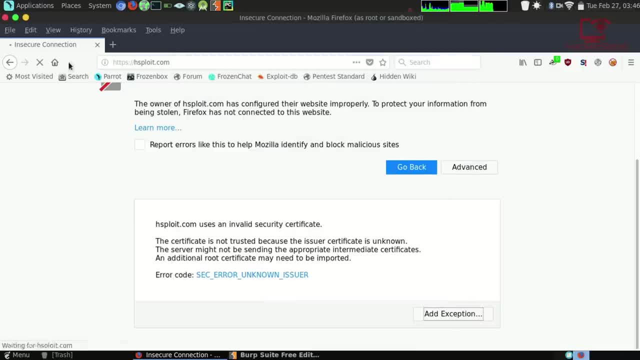 as an exception. There we are, I'm going to confirm exception, And now it's still not going to load the website And the reason being is we have not forwarded the request and they are being intercepted by burp suite. Alright, so if I go into back into burp suite, you can see that it. 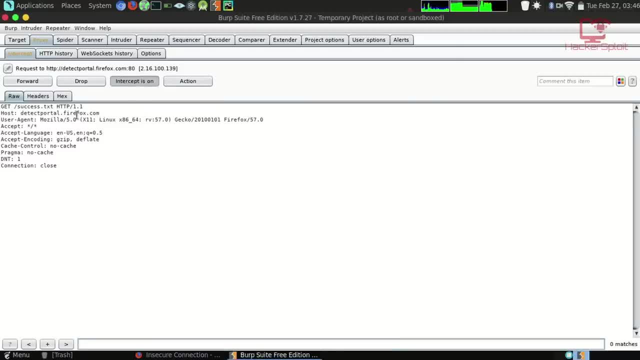 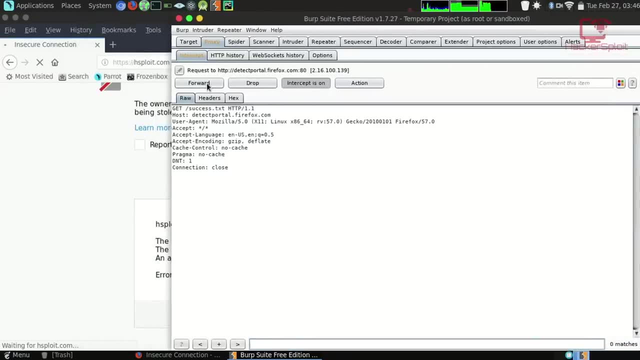 has started the intercept process And by default, you can see that we need to forward. we need to forward the request here. So if I just forward it, let me just fold that again. There we are. let me just fold them for hackersploit. There we are. 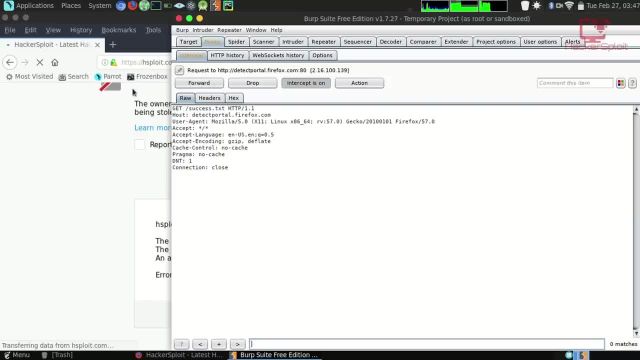 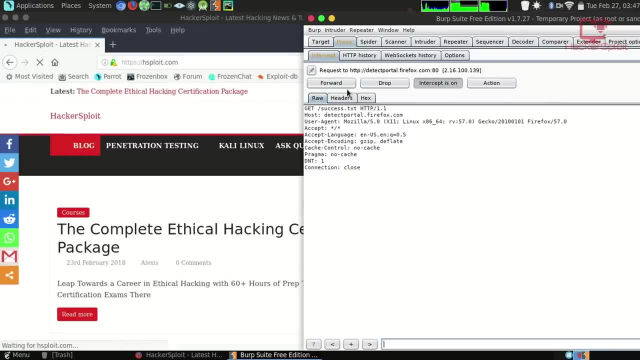 That's the correct one. So I'll fold this again. And there we are. So now hackersploit should be up and running And, as you can see, it should have loaded the site. give that a few seconds. There we are Alright. so, as you can see, that is how you intercept the data that is being sent from the. 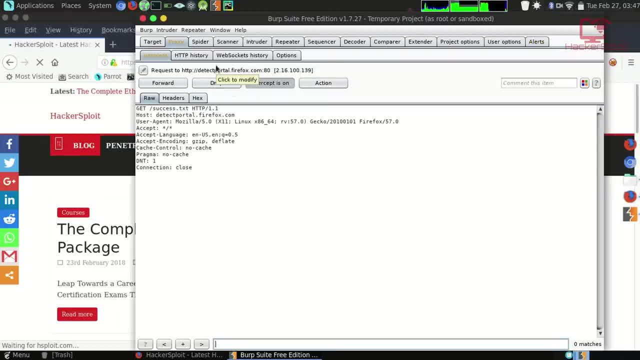 client to the web application And, furthermore, that's how you you can analyze the data being sent and, furthermore, manipulate it to obviously find vulnerabilities within the web application. Alright, so, irregardless of all of this, I know this was very, very basic and it's not really covered anything in terms of web. 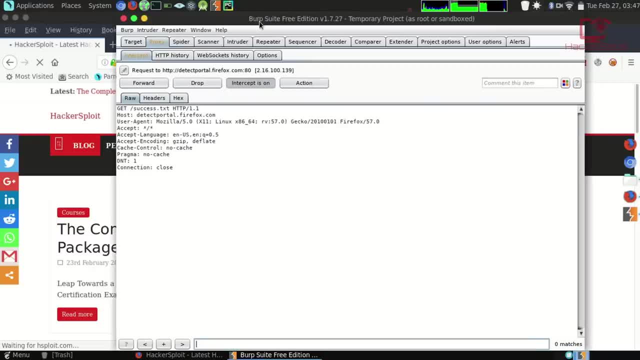 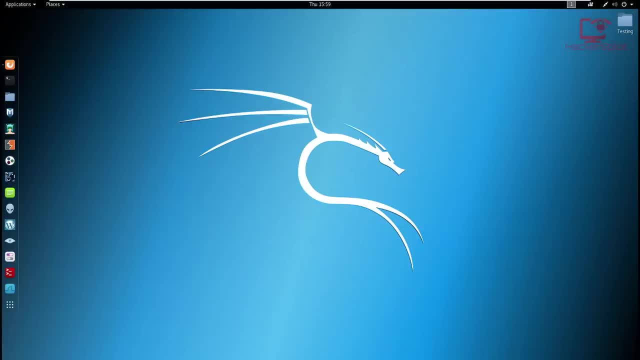 application penetration testing. But don't worry about that. you know, we start off really really simple and we build on that. We're going to get started with spidering, more specifically, spidering with burp suite, And you know the purpose of this video, or this. 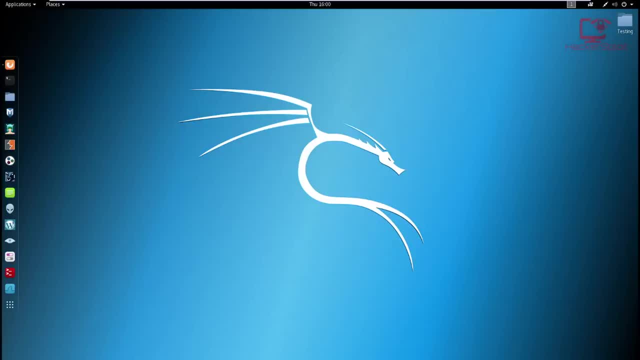 tutorial is to help you understand the spidering process and how to go about doing it with a burp suite. Alright, so there's going to be a little bit of theory here, But I'll be explaining a lot of things. So, again, this video is really focused on understanding. 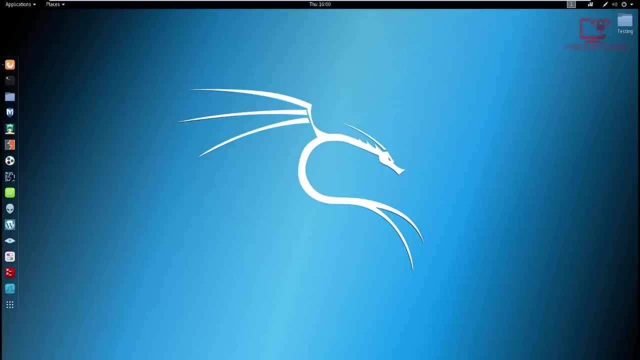 spidering. Now, before you get started with that, I just wanted to let you know that the target, or our web application that we're going to be targeting, we're going to be attacking, is the damn vulnerable web application. Now, if you don't know what the damn vulnerable web application is, 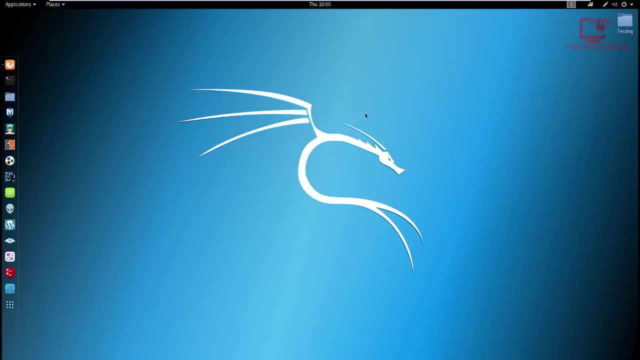 that's fine. you can just Google it And I'll probably make a video on how to get it installed on Kali Linux. But what I would recommend: if you're you know, beginner, or even if you're a professional in hacking, you're going to want to know what the damn vulnerable web application is. 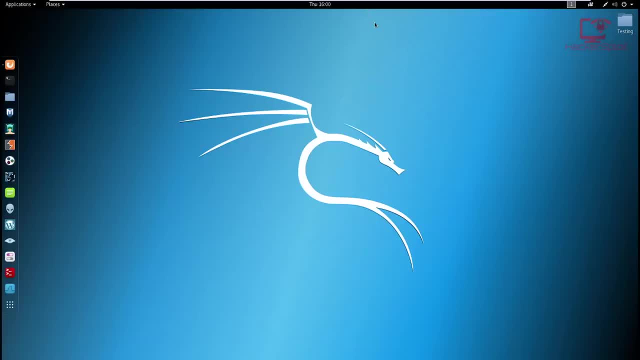 Probably one of the best things that you need to have, you know, in your kit is metasploitable. two, all right, And for the simple reason that it contains, first and foremost, a vulnerable operating system And, secondly, it contains all the vulnerable web applications that we will be. 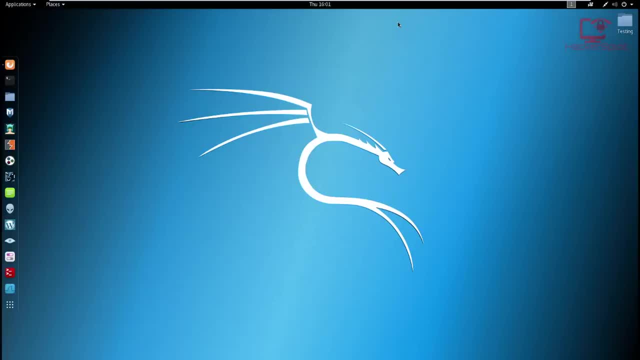 using at one stage during this series. Okay, so we're going to be starting off with the damn vulnerable web application And, as I said, it comes pre installed with metasploitable two, So all you need to do is get the local IP address on your metasploitable two virtual machines. 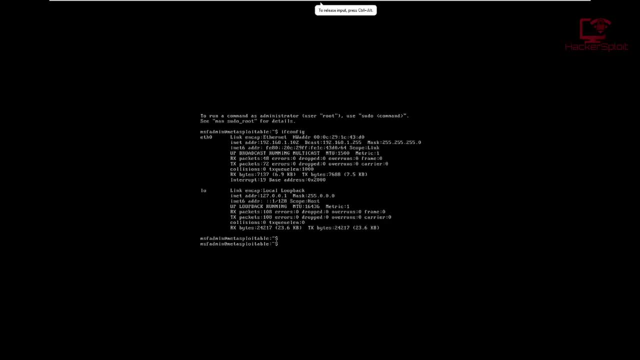 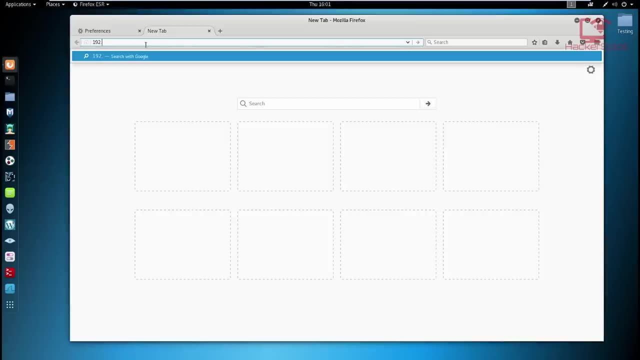 which in my case is 192.168.1.102.. So what I'm going to do is I'm going to open up my browser and I'm just going to open up that web, that IP address, point 1.102.. And just give it a few. 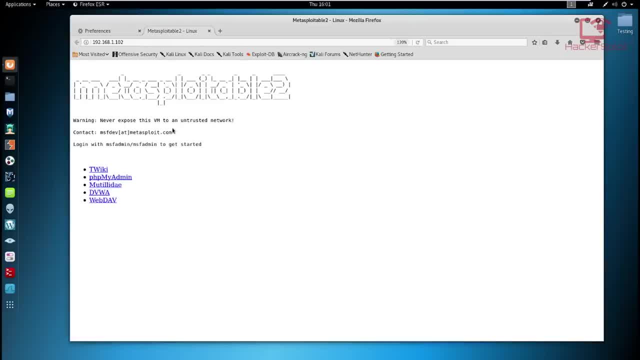 seconds to load up. As you can see, there we are. that's metasploitable two And it's going to prompt us to select what vulnerable web app we want to use. In this case, we're going to select the DVW. 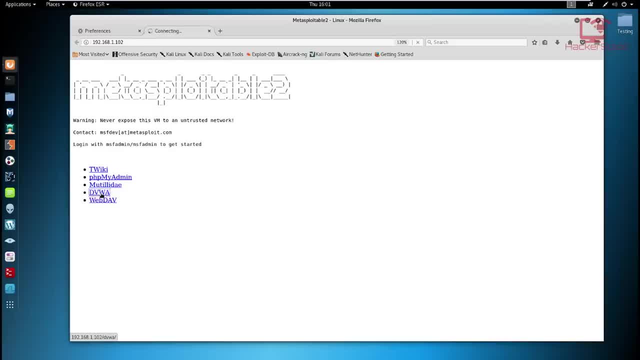 a, which is the damn vulnerable web application. So just click on that And now it's going to ask for your username and password, In this case, for your username and password. sorry about that. In this case, the username is admin and the password is password, Alright, so just hit login and it's. 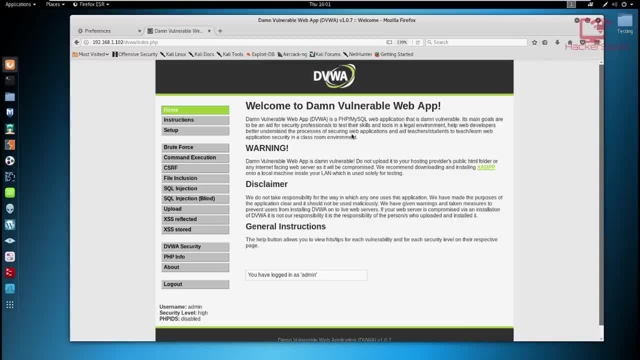 going to log you into the damn vulnerable web application. Now, we'll be looking at this at a more in at a later video, And the reason is we have to go through all of these options. But for now, if you go to the, if I can just remember where it was, if I can just go to the security, 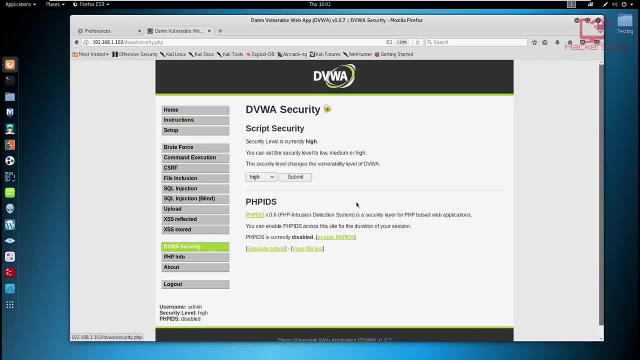 so to the damn vulnerable web application security. at the moment it was high because I was actually performing some tests on it, but just change it to medium or low. But for now you won't be using it. I was just letting you know what web application we're going to be using. 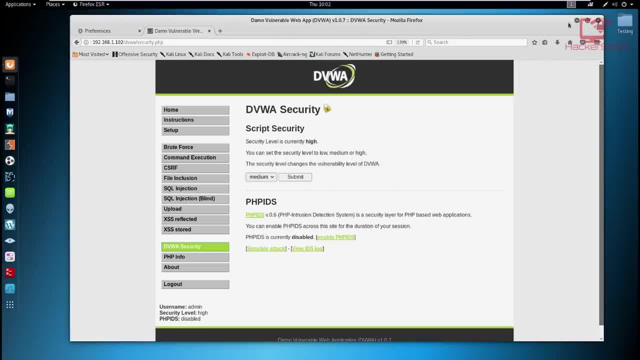 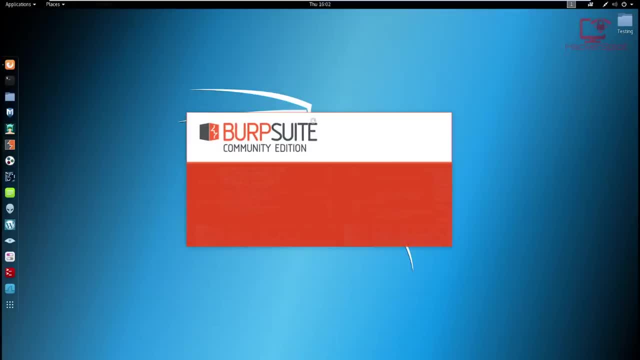 Alright. that being said, let's move on to burp suite. Alright, and we can. I can start explaining the spidering process. Alright, so let me just open up burp suite. So I've updated it to the latest version. I think I'm running calendar next Now. in the previous video I was running parrot. 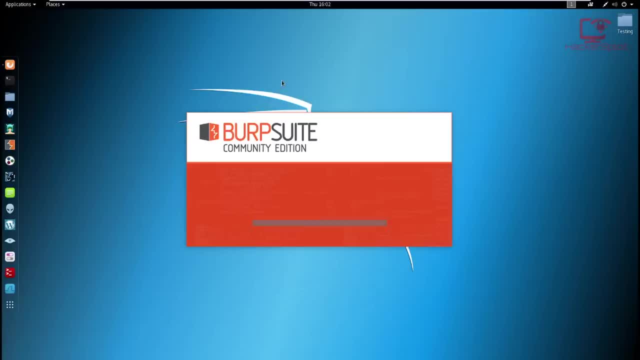 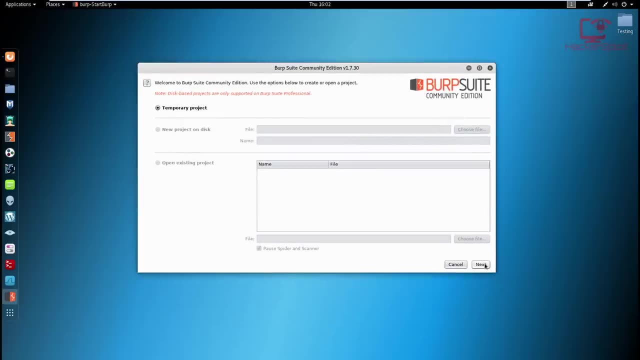 So I think there should be an update, but I could be wrong, So let's just give that a few seconds to. yeah, there is an update, So I'll do that later And we'll just click on create our temporary project and use the BEP default and start that, Okay. so once that's starting, let me explain. 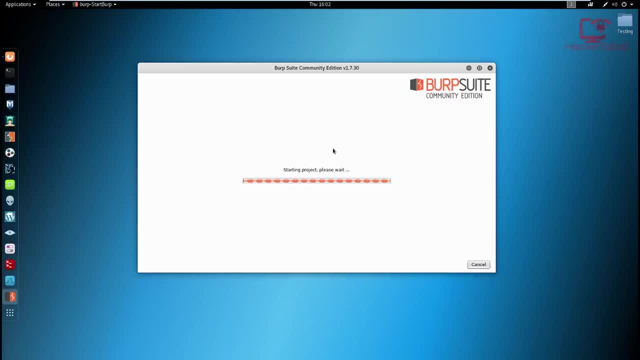 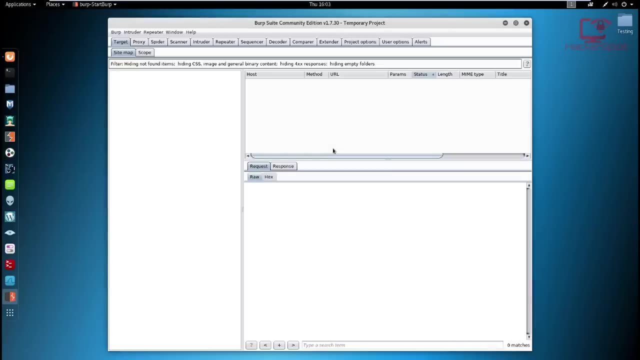 what spidering is Alright. now, the purpose of spidering is to identify our scope, all right, or what? what we want to scan Now? this is not exactly scanning and we'll be looking at scanning, But essentially, spidering is the process of mapping out our web application and is very 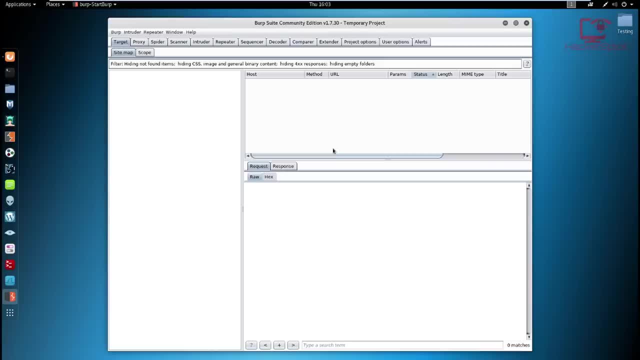 very useful for finding links and and web applications. So let's just go ahead and look at the web forms, which is also very important, because it will allow us to then, furthermore, attack the web forms, manipulate headers, etc. etc. Right now, when you talk about 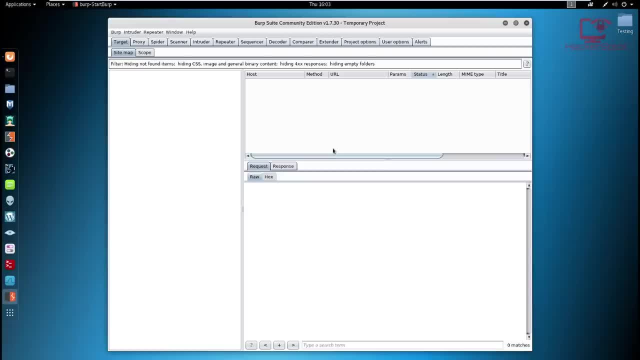 automatic spidering with burp suite. it's essentially when, when burp is spidering, it follows links and it'll it'll start following links and it will start identifying for files, folders and forms from the web application And it'll the great thing about this is it will. 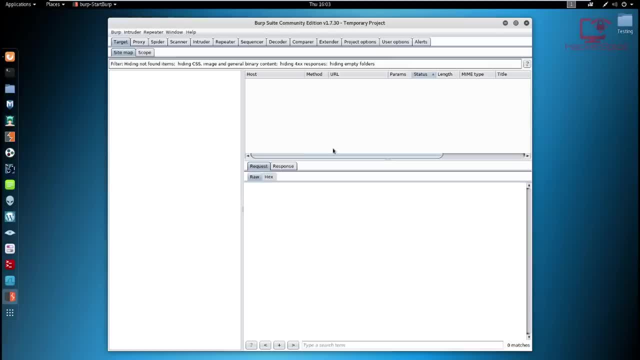 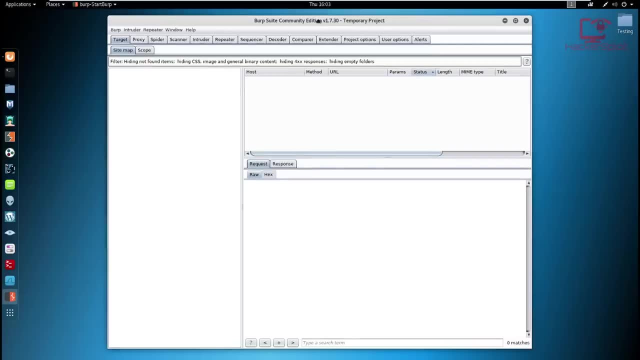 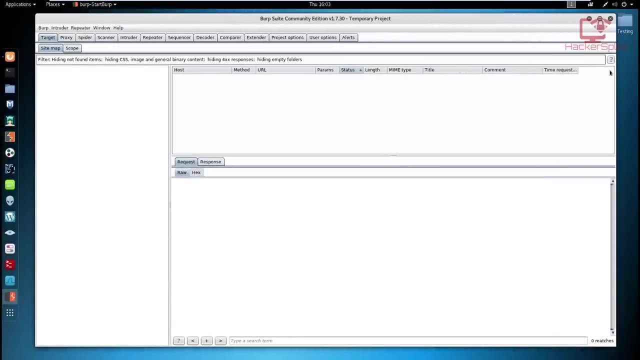 record all the requests and responses forming the whole spidering process. Okay, so once you have a burp suite opened up here, you can let me just expand it So we have a greater picture of what's going on exactly. Sorry if my virtual machine is a little bit slow. I need to configure it correctly. Anyway, 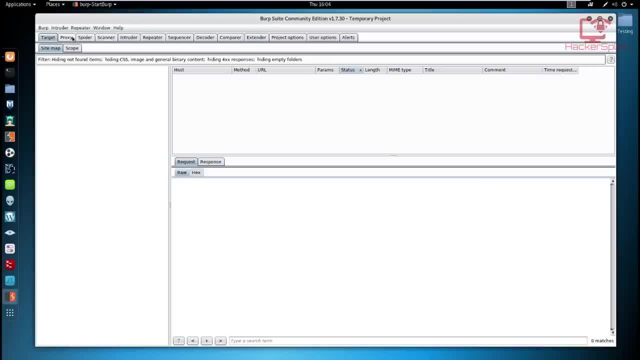 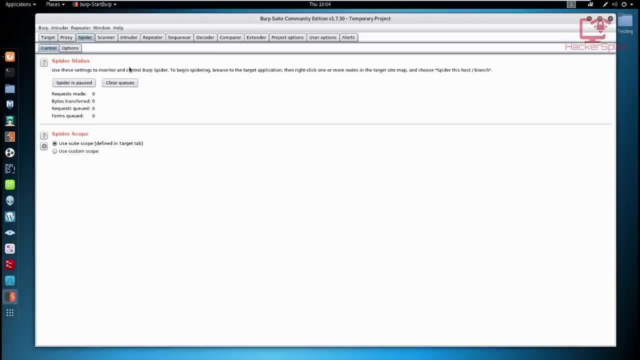 what you want to do is: we've looked at the proxy check section, let's look at the spider section And in here this is a very, very simple menu And to understand it, you can see that we have two tabs available. we have the control tab and we have the options tab. Alright, 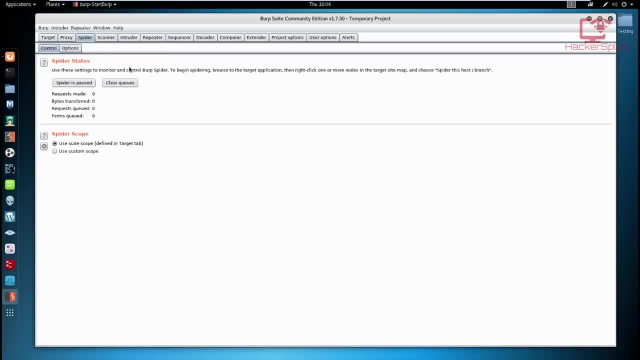 the control tab. essentially, if I just click, if I just look, if we look at it, as you can see, these settings are used to monitor and control the web spider, So it allows you to stop, to start and stop the web spidering And you can also clear the cues. Alright, when you look at the options. 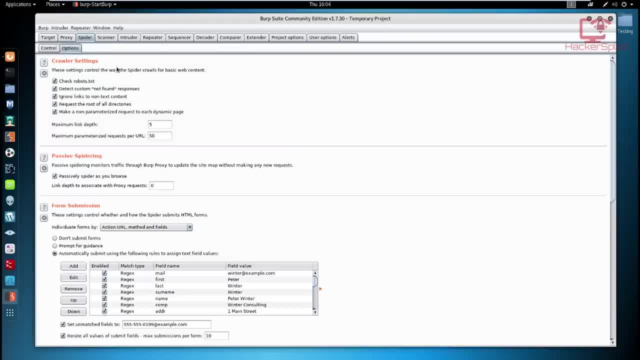 which is right here. sorry about that. When you look at the options, there are a lot of options. we'll be looking at them. We'll be looking at them in a second. Sorry about that. I actually got an email, apologies there. 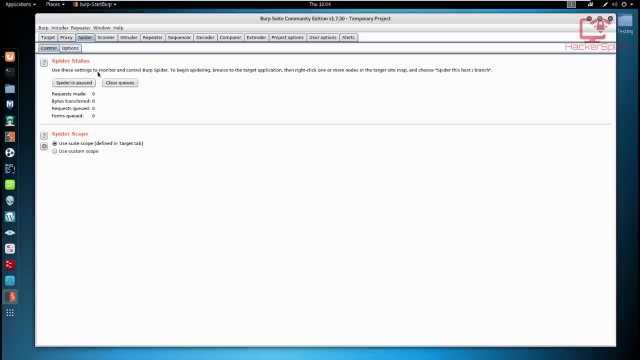 now with the control section. So the control section it allows, we are able to control the spider status, where we can stop it and start it, And you know, furthermore, we can clear the queues that already exist there. Alright, we then have the spider scope. where we can, we can define our. 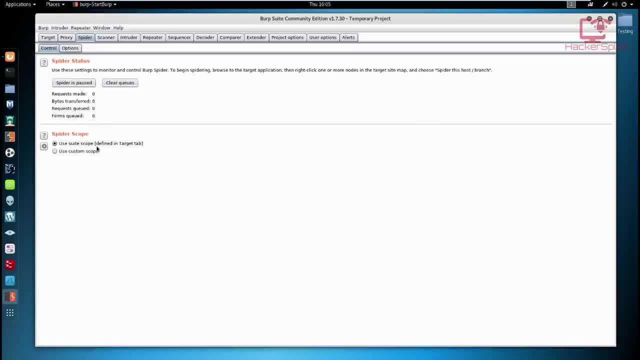 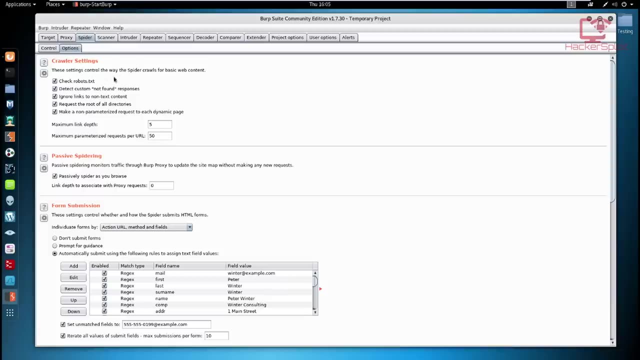 own scope And depending on what we want to spider. we look at that in a few seconds. And finally, if we look at the, well, if we look in the options section here, we have the crawler settings which allow us to specify the way the spider is going to crawl for the web content on the web. 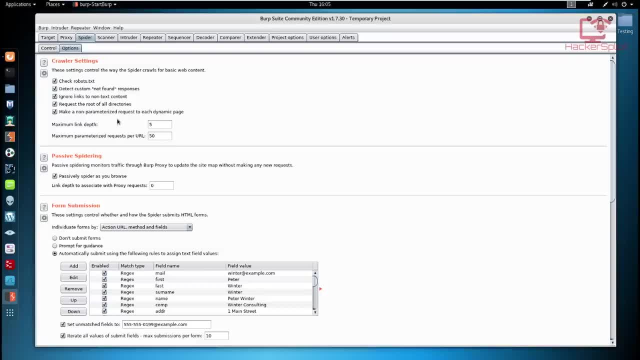 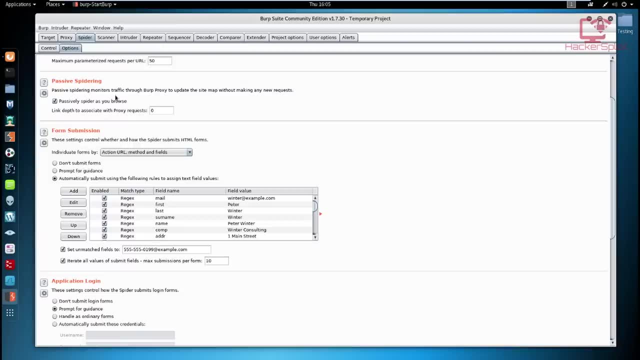 application. we'll be looking at the maximum link depth and what that means: passive spidering that allows us to essentially spider, to continue spidering. when we are looking through or we're going through the web application. we're performing requests and responses. when we're performing. 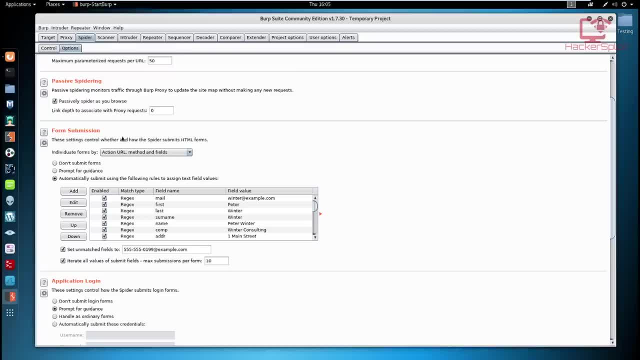 requests. As for the form submission, this is probably something that we'll be looking at in the next video, And we'll be doing this practically. we will be actually performing the will be performing the spidering process, But for now, let me see what. 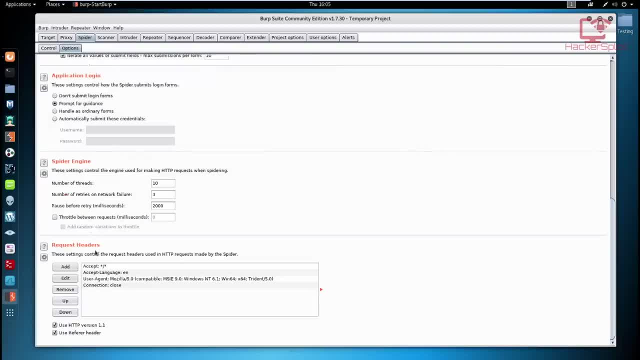 else. Yes, the request headers. the request headers are used to. you can manipulate, essentially, the headers if you've learned about HTTP headers. by the way, I really want to cover HTTP because it's very important that you understand how the headers work, But we'll be looking at this all in. 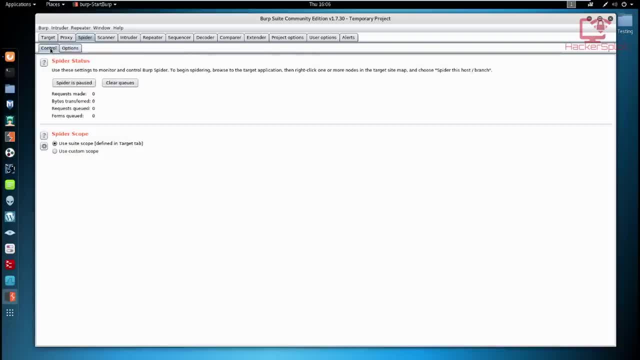 advance. But now let's start off with the spider status. Well, not really with the spider status, but looking at the control tab. if you look at the spider scope, you can see that you can. it'll use the default suite scope which is defined in the target tab If you just click on use a custom scope. 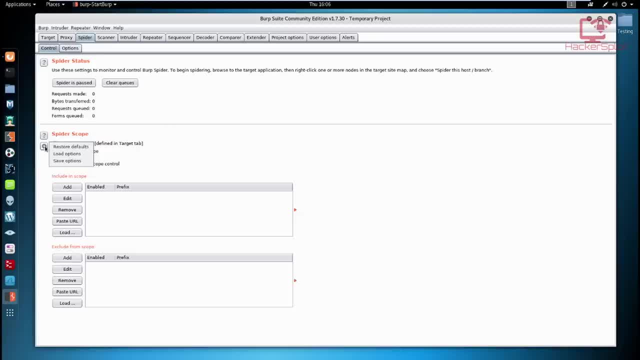 you can see that. Okay, first you, if you just click on this cog here, you can restore the defaults, you can load your own and you can save the options. So that's just to do with that. Now, when you talk about using the advanced scope, here's where you can. essentially, this is where 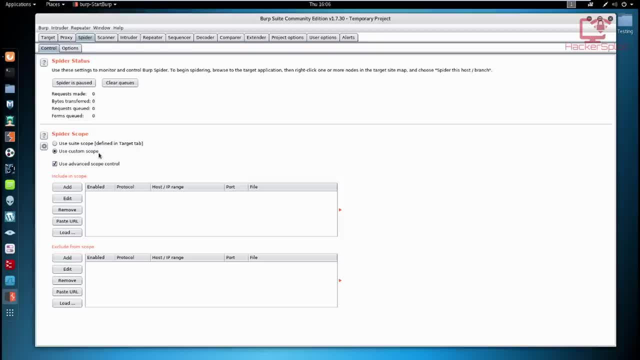 you can specify a host, the port, etc. etc. Okay, again, we'll be looking at all of this as we move along, But for now we're just going to use the default suite scope. We can just if, once you click, 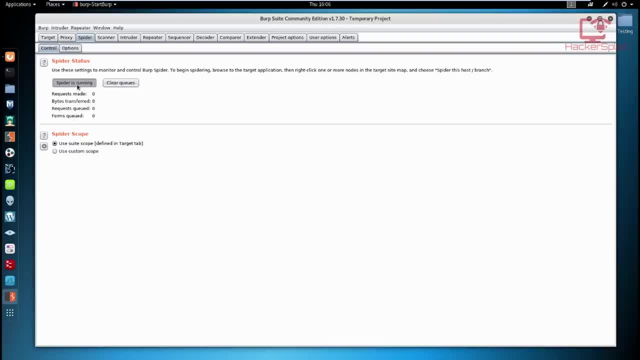 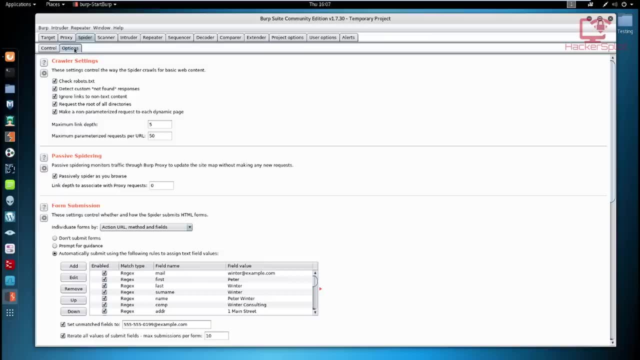 on. that is going to stop the spidering process, but we don't need it right now. So I'm just going to come, just going to pause it. And if we move on to the options now, the options tab has a lot of stuff that we need to look into. First and foremost, we have the crop, the crawler settings. 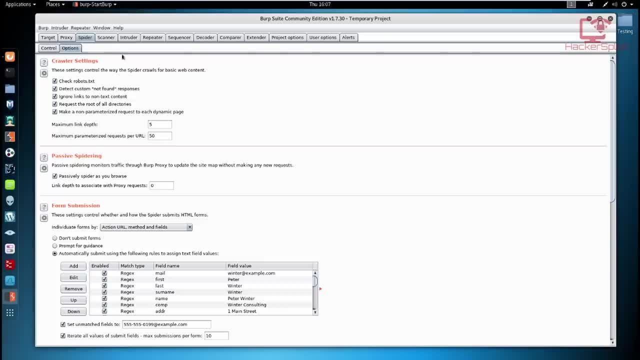 right. So when we're talking about the basic options, for example, specify what the spider will crawl for, So it you can choose to select for robots the robotstxt file, which is very important because it shows you, you know, exclusions you then can detect. 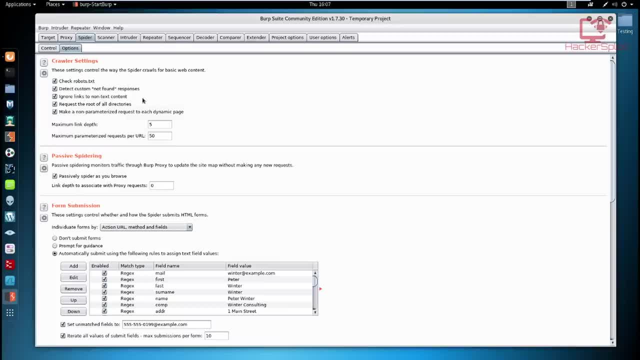 you can ignore the links to non text content. you can request the root of all directories- very important stuff- But again, you can customize this to your liking. Now, one of the things I would recommend that you do not touch with if you do not know what you're doing yet, is the maximum link. 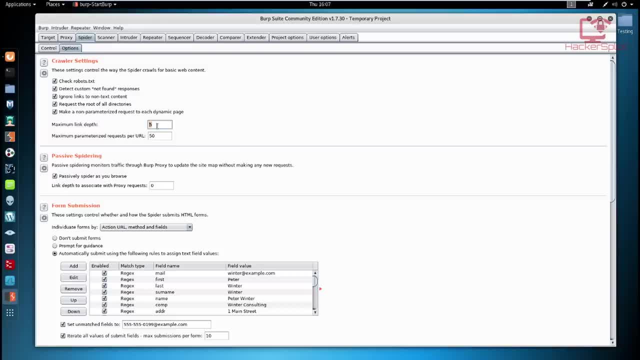 depth right. the maximum link depth is essentially the number of links you want the spider to to, essentially to crawl or to map. Now, by default, five is in my, in my, in my situation or in my case. what I like doing is alternating between 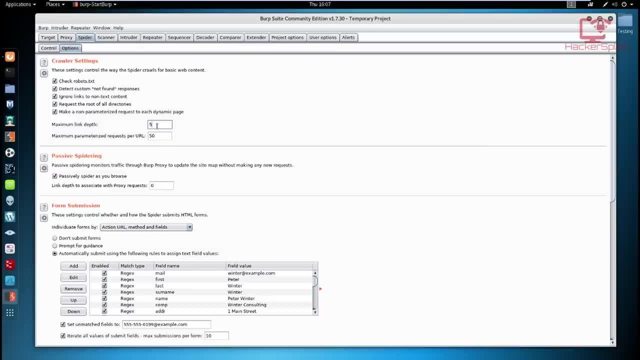 three to five. anything higher than that will usually overload the web application and it will cause it to lag or to respond very, very slowly. And you know, again, that might not mean a lot right now, But trust me, when you'll actually be performing the penetration test, you'll be able to. 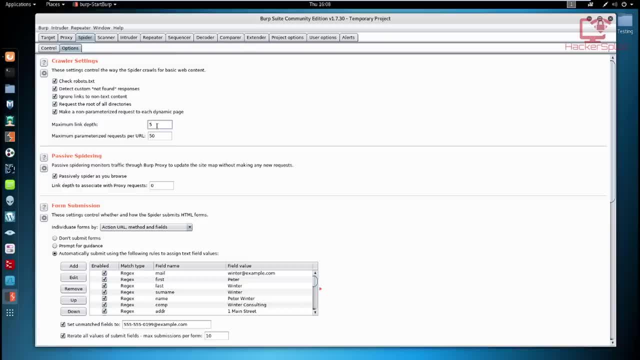 test on the web application. you really need a good response, Otherwise you have your time to live, etc. etc. Okay, so let's look at what passive spidering is. Alright, so, as passive spidering, as I said, is essentially just, it allows you to continue scanning, you know. 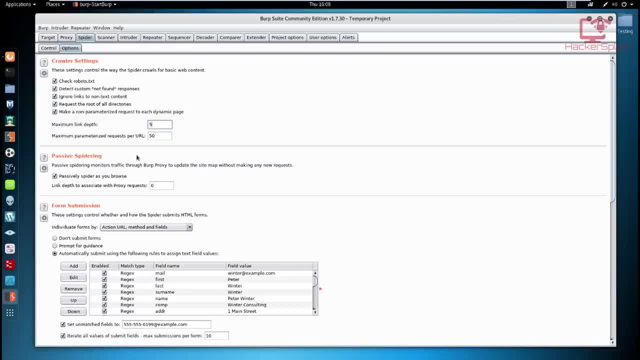 or going through or actually performing your requests. as as it, it essentially allows you to continue the spidering process as you're performing any other tasks. So, as you can see, it monitors monitors traffic through the bug proxy to update the sitemap without making any new. 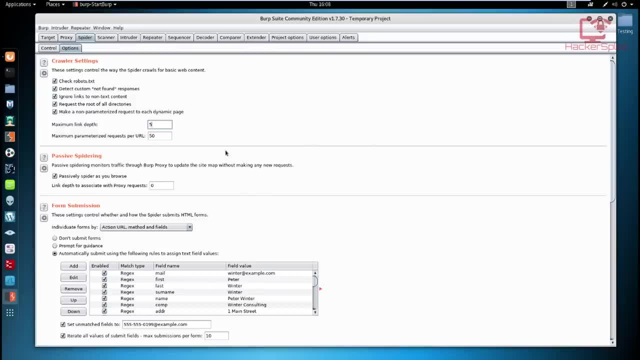 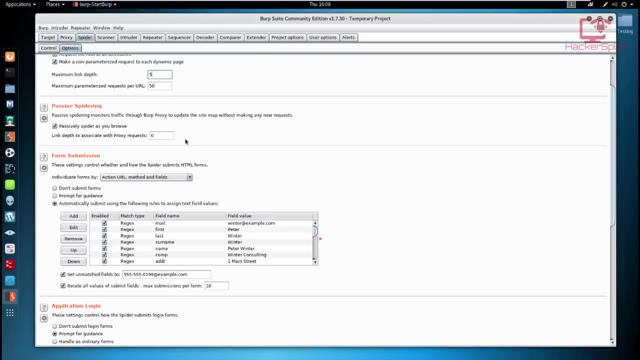 requests. Alright, so passively spider as you browse. you can also select the link depth associated with proxy requests. Now, this I would recommend keeping it at zero to two, And that's because, again, you do not want a very, very deep alert link depth, in the sense that you're also 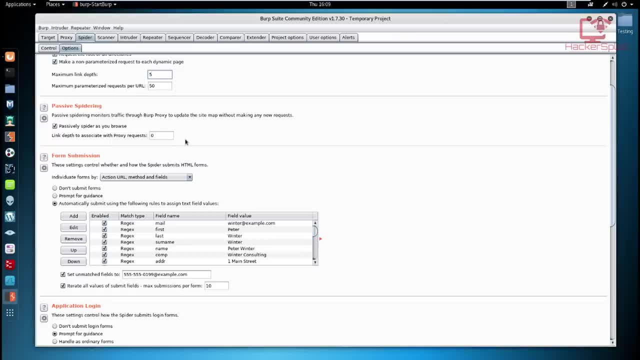 going to be performing your own requests And you'll be doing many other things. you could be looking at the decoder or you could be looking at. you could be focusing on the target And you don't want it again to slow down the web application. Alright, so form submission. again, this is something that I said. 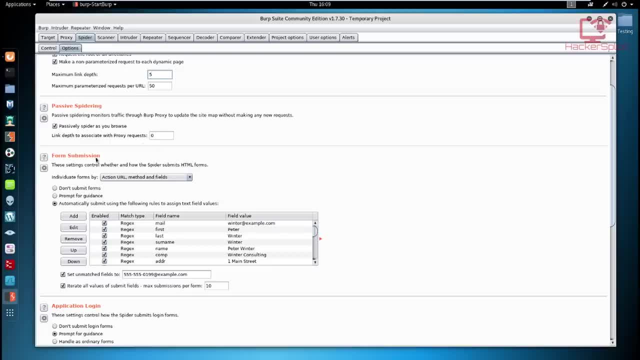 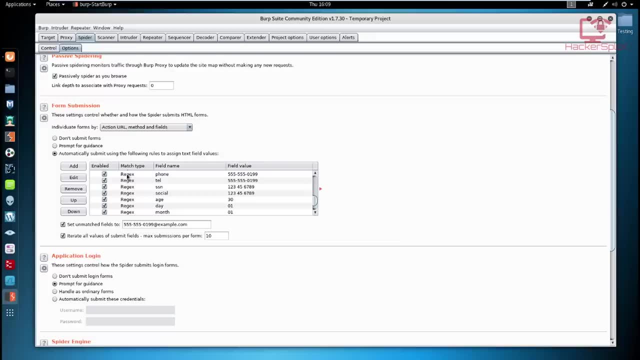 we'll be talking about in the next video, because it is quite advanced, and we'll get started with the damn vulnerable web application. They're moving on to the spider engine. we'll be looking at application login as well, But for now, just we will just skip over that when we talk about the 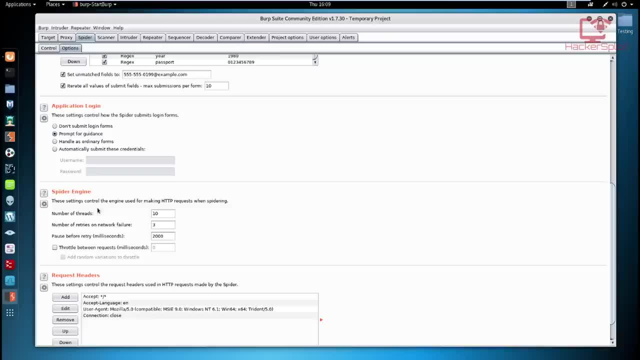 spider engine: All right, these are settings control the engine used for making HTTP requests when spidering. All right, so this allows you to change the number of threads you want to use And, as I said, using more than you can see. right now it's at 10, what I would recommend is still keeping it. 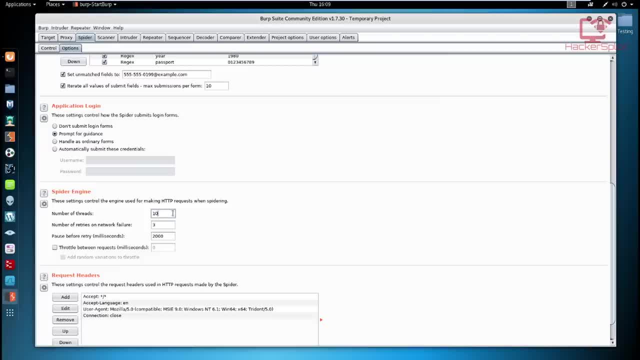 within the range of two to five, or you might- you might cause the web application to slow down, And these are more advanced settings that you can use, dependent on timing. All right, and we've talked about the request headers. they allow you to modify the way the spider will. 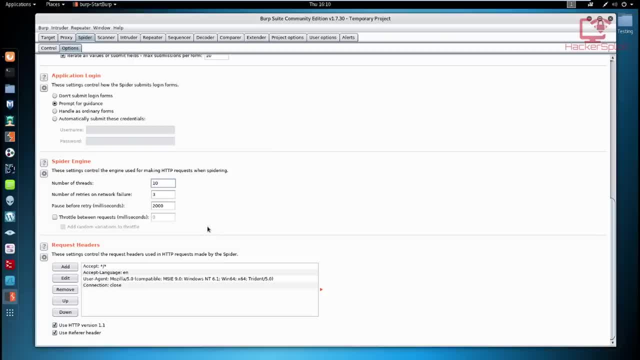 will look towards the web applications. For example, you could, you could- edit the, the device that is being used, and you could change it, for example, into a mobile device, and you get the idea. you essentially allows you to to change the request headers And from that, 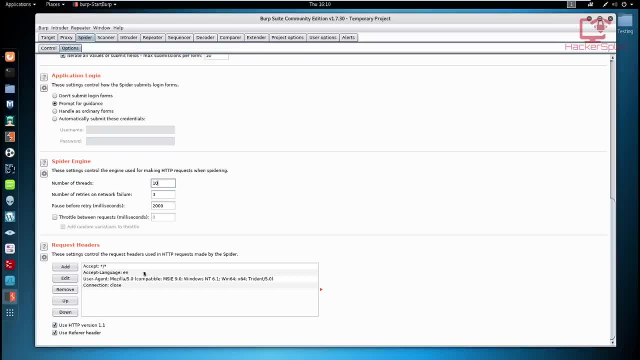 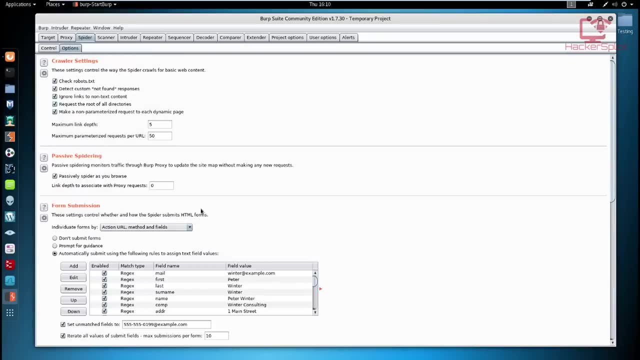 obviously you'll get a response back, dependent on what you changed. Alright, so that was the spidering, or actually the theory revolving on spidering. Now we'll be looking at how spidering really works In the next video. I know some of you may not like this- that I actually went to. 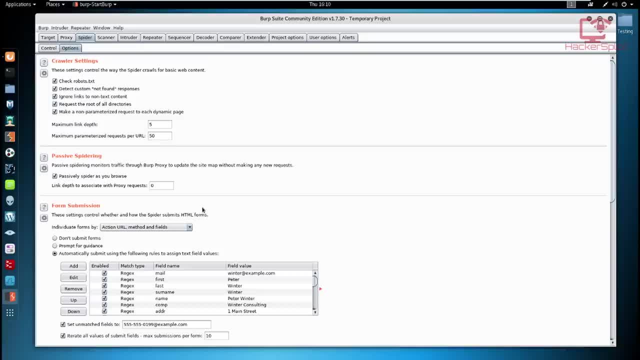 three theory and haven't talked about it. But if you're interested in learning more about spidering, and you're interested in learning about doing anything, but remember it's very, very important to understand what exactly is happening behind spidering. And in the next, 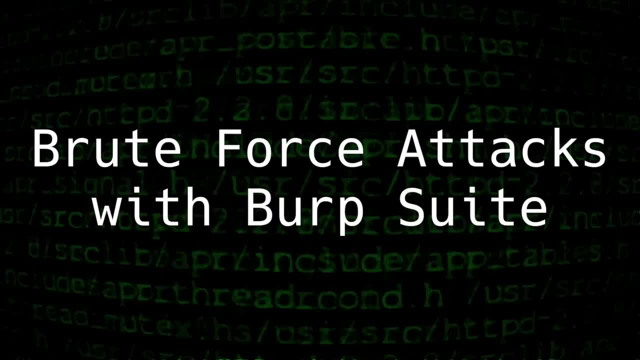 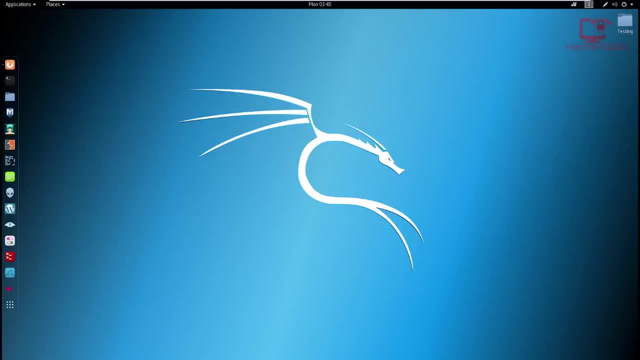 video, we'll actually get started with the spidering process. We're going to get started with brute forcing with that, Alright. so our vulnerable web application of choice is going to be the damn vulnerable web application, as we discussed in the previous video, Alright, and I'm going to be using meta exploitable to as 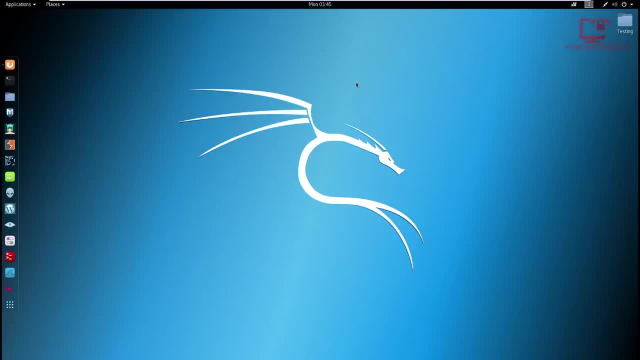 our as my server By default. you can install meta, you can install the damn vulnerable web application on your Kali Linux and you can host it on your local, on your local server, And you can. you can then perform your attacks, But I like running it from an another virtual machine. 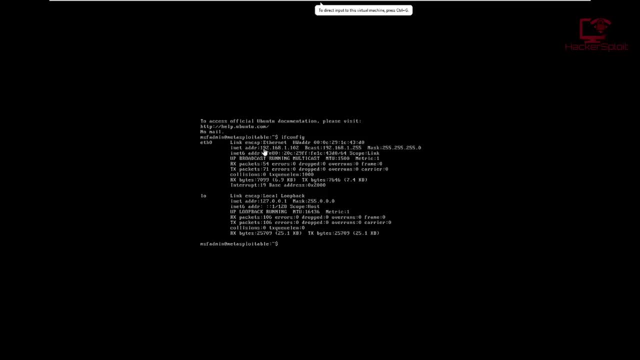 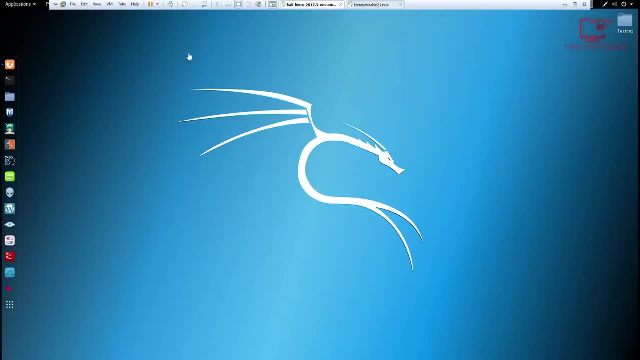 And, as you can see, I'm running it on the meta exploitable to virtual machine And by default it's connected to my local network and it's bridged. So you can see that my local IP address is 192.168.1.1 or two. Alright, so I already have the damn vulnerable web application. 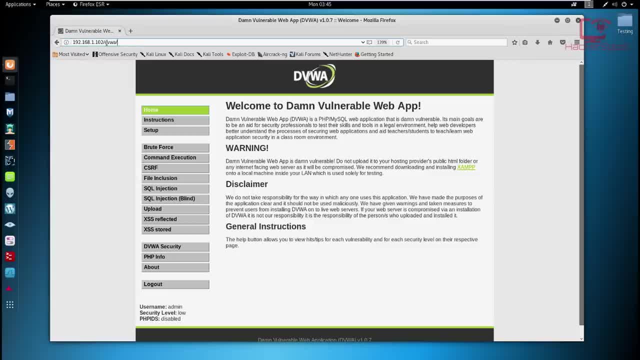 open. As you can see, it is running on the that IP address of the meta exploitable to virtual machine under the damn vulnerable web application. So for those of you asking why I'm using meta exploitable to instead of meta exploitable three, it's because meta exploitable. 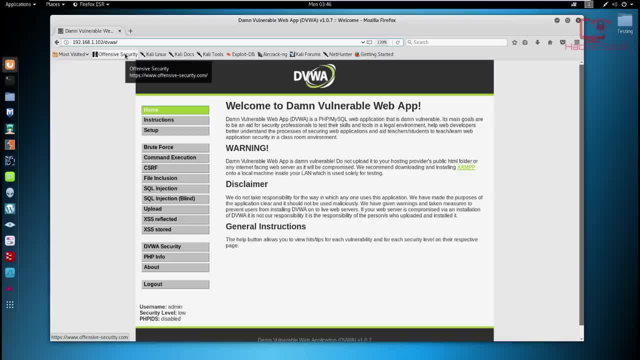 to has a much larger choice in terms of vulnerable web applications, And it's really good for practicing, Alright. so make sure you're logged into your damn vulnerable web application you need. the default username is admin and the password is password. Alright, it's really very. 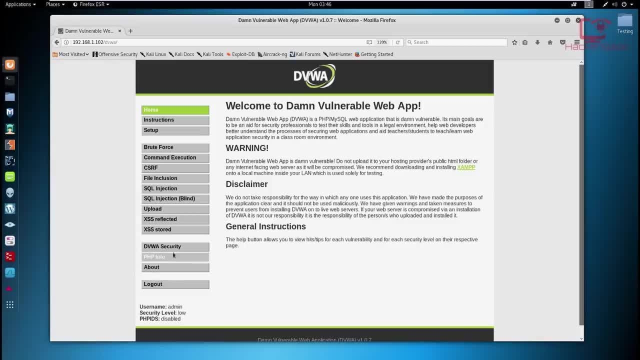 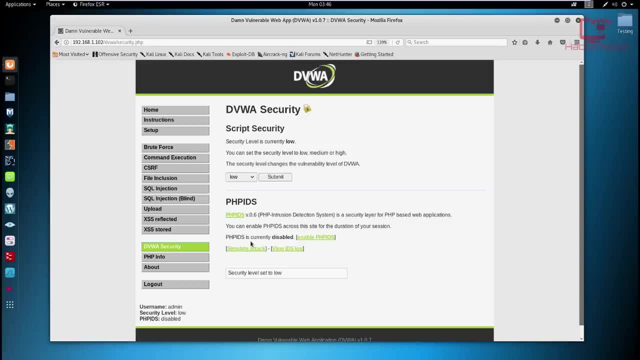 simple: Alright, by default. in this video we're going to set our security level to low. If you don't know how to do that, you can go into your damn vulnerable web application security And you can set that to low and you can just hit Submit The. 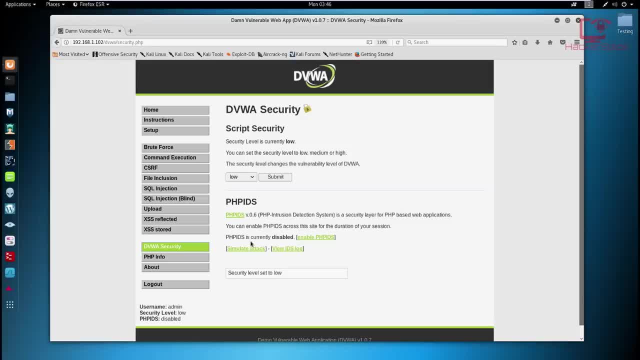 reason we're setting it to low is because most logins are. you know, if you look at the real world, if you're talking about big sites, this attack may very well work on sites that are older or sites that have not been updated or sites that don't have good security. you'll be shocked to. 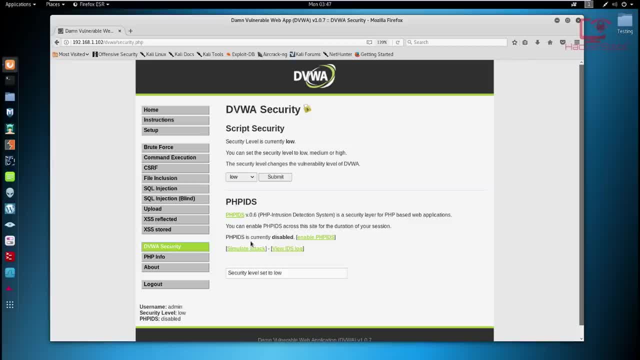 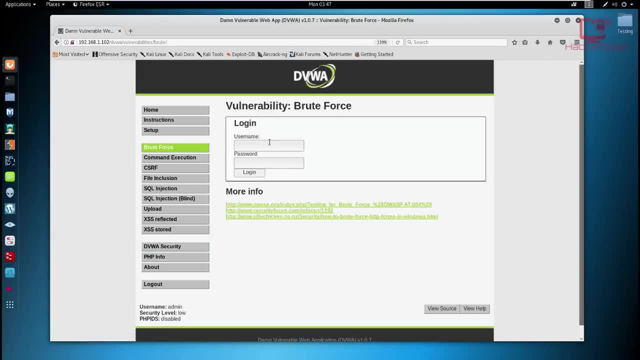 find some really big companies that actually don't have any login protection, or brute force protection, for that matter. Now, that being said, what I was talking about is, if we go into brute force, you can see that we have a lot of security. So we're going to go into brute force and we're 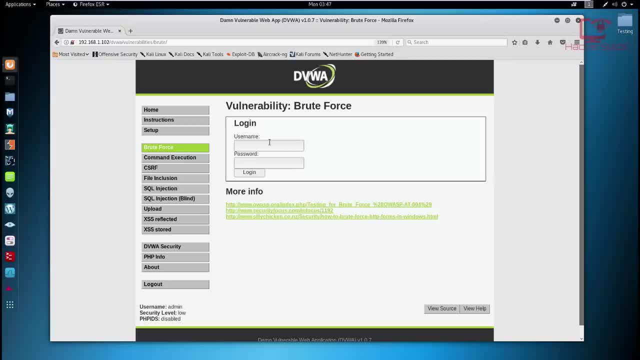 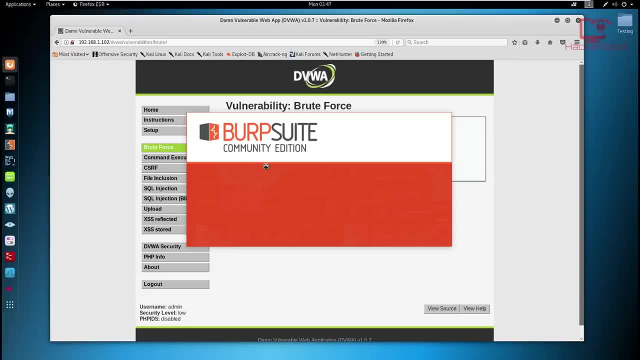 going to have a login prompt here. Now I've forgotten the username and password and we're going to be brute forcing it live, All right, But before we do that, we need to actually start our birth. Alright, so start up that suite And you can see. I'm using the community edition and it is. 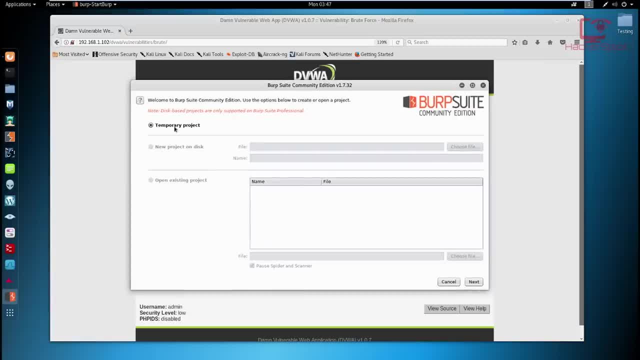 the latest version. Alright, so make sure that yours is the latest version. obviously, for obvious reasons- And we're just going to start a temporary project because I don't use the pro version- And we're going to hit: use the BEP defaults when a startup right. give that a few seconds to start. 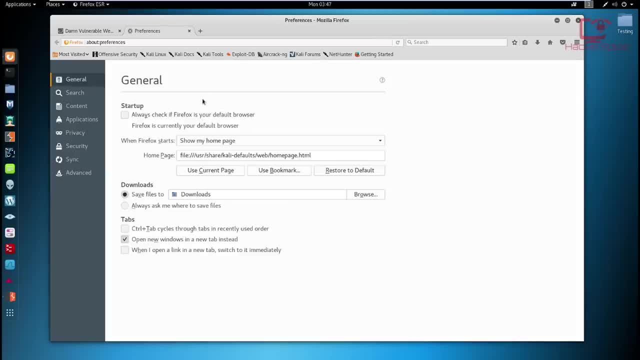 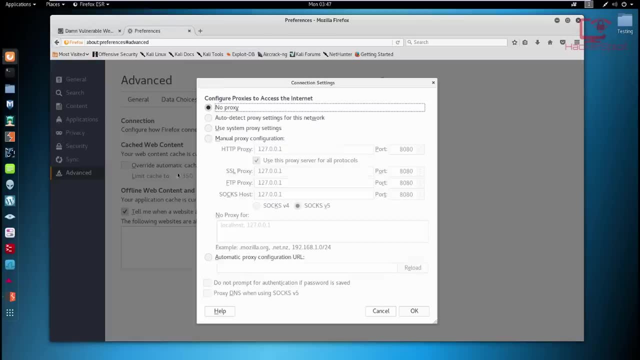 the to start up, And now you want to make sure you you're using the proxy. So we're going to go into preferences and advanced And whoops, burp is opened up. let me just go into my proxies, network settings, And we 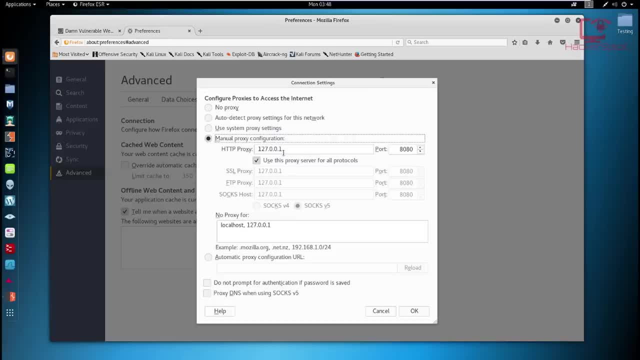 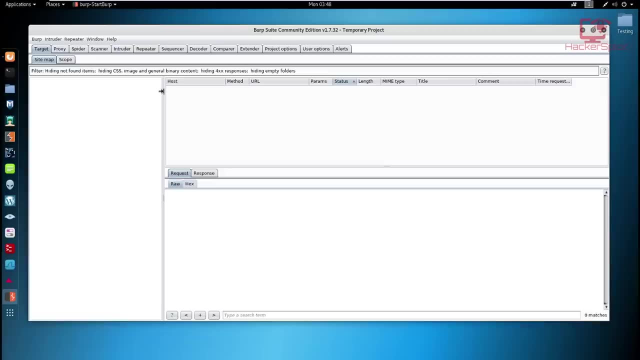 make sure that it's using the manual proxy configuration, which is the localhost 127.0.0.1.. And the port is 8080.. We're going to hit OK, Excellent, Now we need to move into burp back again And we want to make sure that we go into proxy and the intercept is set to off. All right, 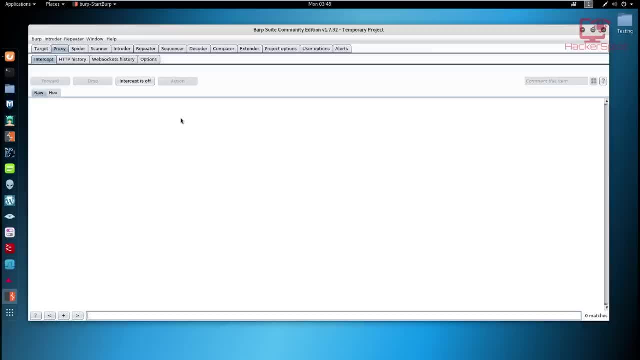 the reason we're setting the intercept off Is because I just want to show you something first. Now, by default, intercept essentially just means that you're not intercepting the request, the request and the responses being sent from the web application to your browser. Okay, so we have already set the proxy for the browser. 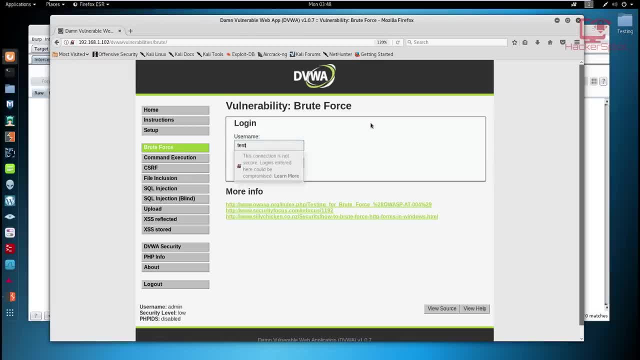 but we're not intercepting. So if we just test a random username like test and we say a password like 12345, you can see if I hit login it's going to tell me that that is incorrect. Now, if I set the intercept to on to see the request, 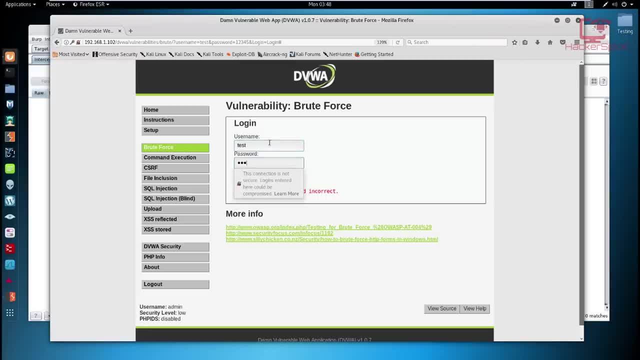 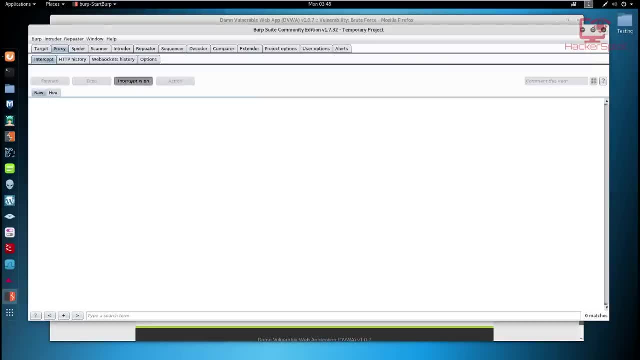 let me just turn it on And we can now reload this So we can say test and the password 12345.. We can see that now it's for some reason- let me just forward that I'll have to actually just turn that off- And we now say: log in And for some reason that is not allowing us, because we have 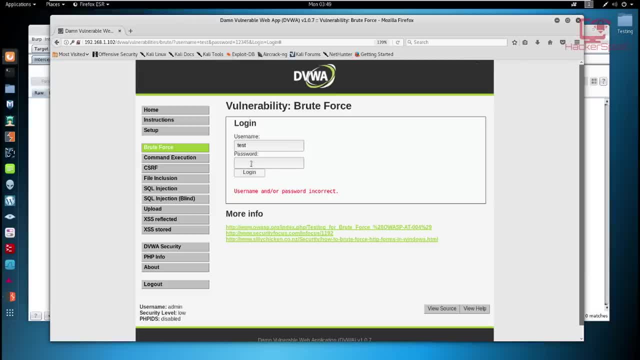 to reload, Alright. so now, if I hit intercept on, and whoops, let me just open up my browser and hit the password 1345.. Log in for some reason it's going to. you know it's going to. you know it's. 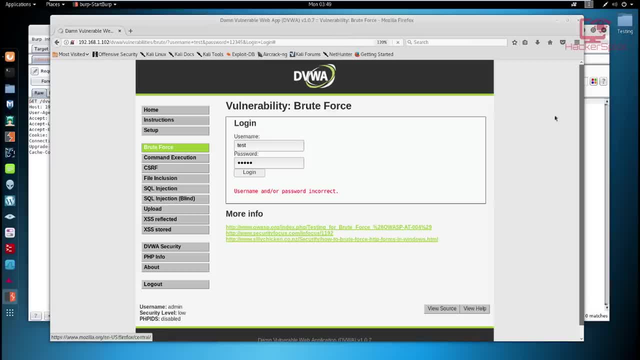 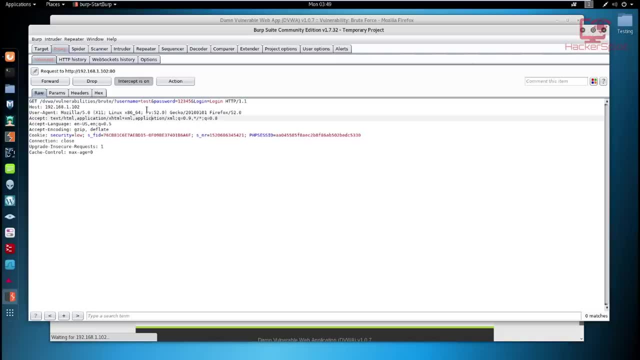 going to reloading here. I probably there we are Alright. so I've reloaded the page And, as you can see, now the intercept is on And if we go back to burp, you can see that we got the get request being sent by the web application. Now let's inspect it for a while Now we'll be looking. 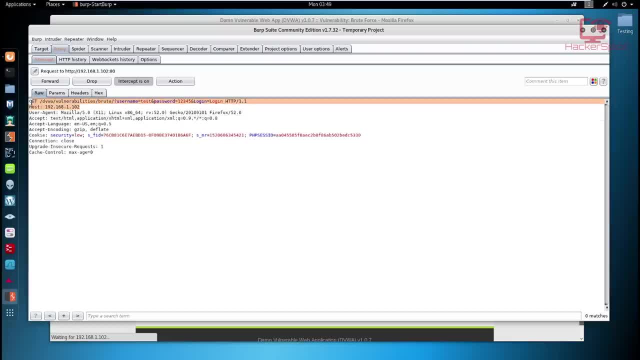 at what all of this really means, But by default, the most important thing right now is the get request. Alright, so you can see that the get request has two values here. It has the username and the and the password. Now the values are again, are not? 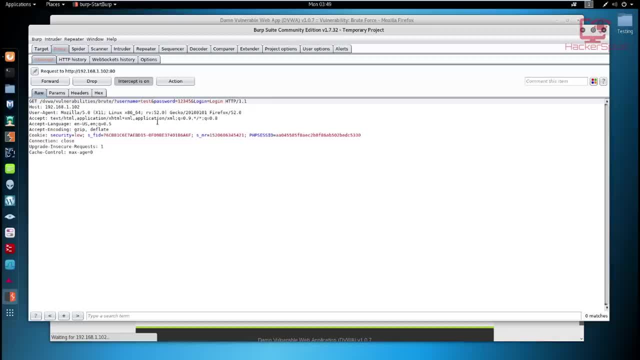 important. we're going to be brute forcing the values, but it's very important to get the fields that we're using here. Now, what am I talking about? If you look at the cookie, you can see the security is low And if you want to edit the value, and for the package you can set it to high. that 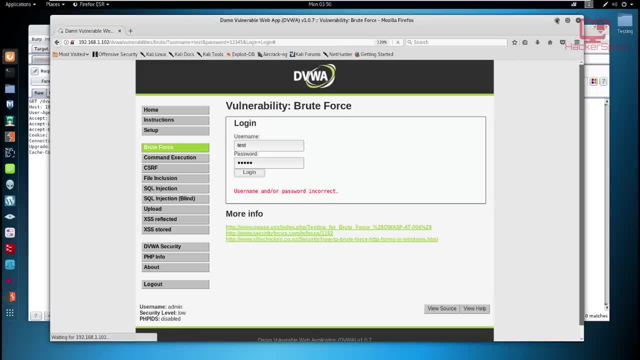 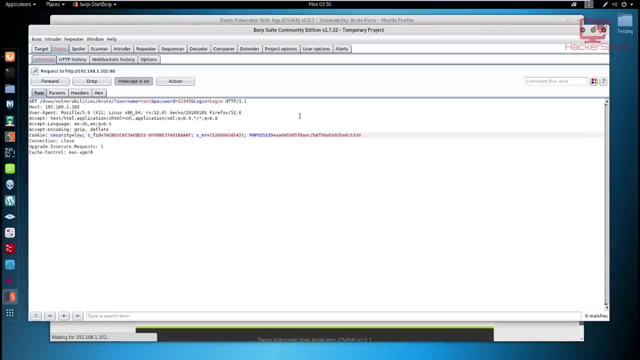 is basic stuff. That's good stuff, right. But now we want to brute force this login, Alright. and how do we do that? you can see, the first thing we need to do is we're going to be using the intruder. 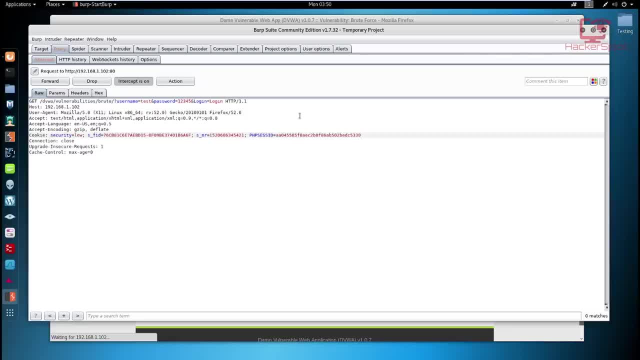 Alright. so if you're a bit confused about what the intruder is, don't be worried. the intruder is essentially allow, allows us to edit the parameters, it allows us to edit the requests and then obviously, edit them and manipulate them so you can get the desired results. Now, the great thing about the the intruder is it. 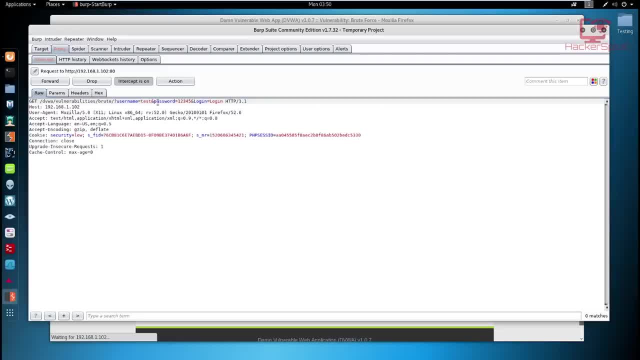 allows us to perform attacks like the brute force, etc. etc. All right, But now what we need to do is we need to send this request into the intruder so that we can send our own response. Alright, so we're going to right click and send to intruder. So we just send it to intruder. 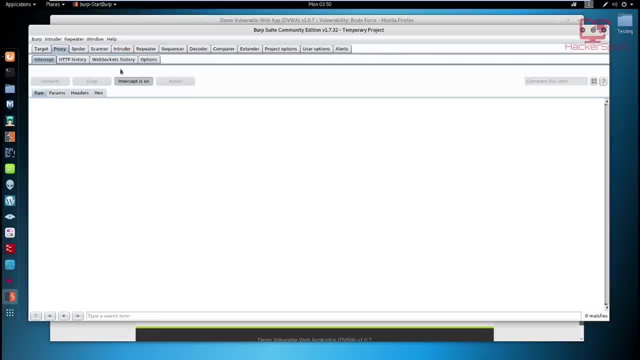 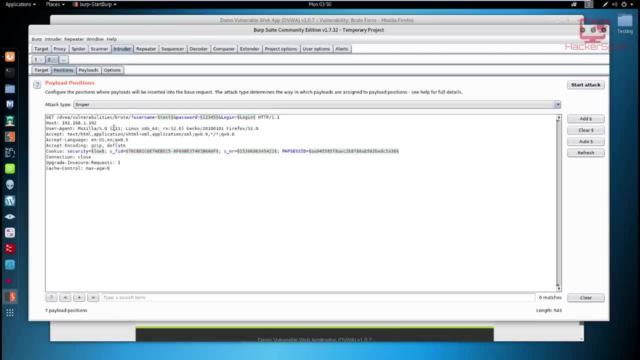 And once it's sent to the intruder, you can just hit forward. All right, we don't need, we do? we don't need that get request anymore. So now you want to go into the intruder and you want to go into your positions And, as you can see in your positions, you have got. you have got the get. 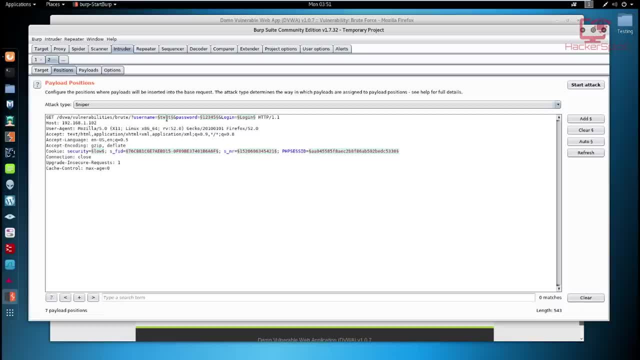 request that we were, we had just intercepted, And now you can see something really interesting. it's highlighted for you all the different payloads, okay, all the different fields that we can brute force for. By default, we have the username value, the password value, the login. 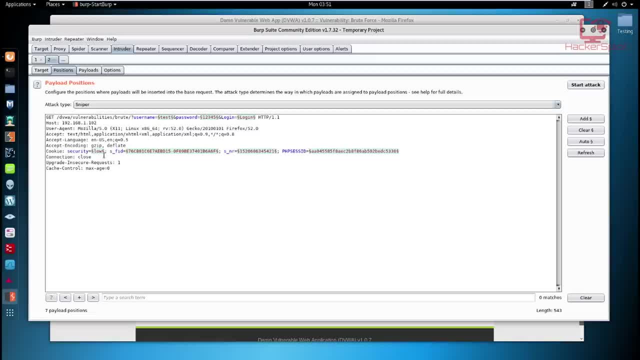 value. we have the F, the SFID Value. we have the, the cookie value. no, no, no, we don't need all of these. the only values that we need are the username and the password value. So the most important thing you need to do right now- 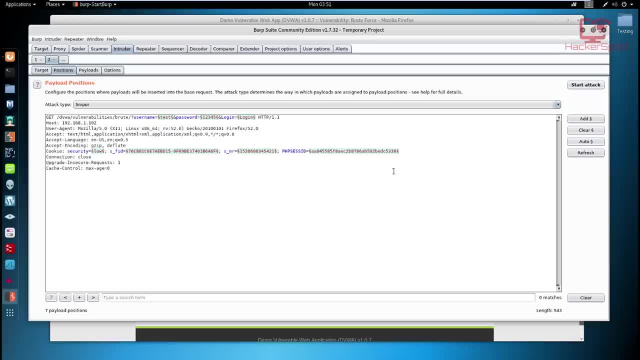 is you need to clear, just hit clear, All right. Oops, sorry, not that clear, I beg, I beg your apology there. I'm sorry, I didn't mean that. what I'm trying to say is: I'm sorry, just clear. 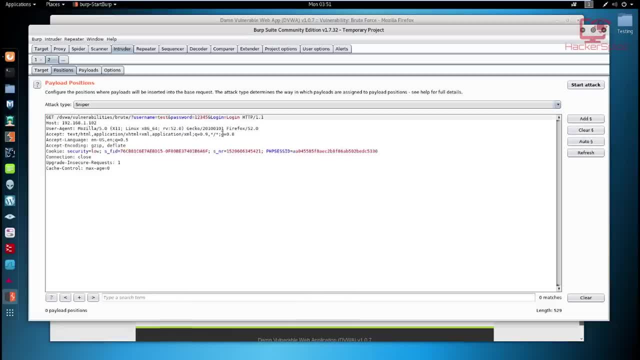 just hit clear And, as you can see, now no values are being selected to be brute force again, So now we need to select them manually, But that we're going to be using the, the cluster bomb attack type. Alright, the reason we're using the. 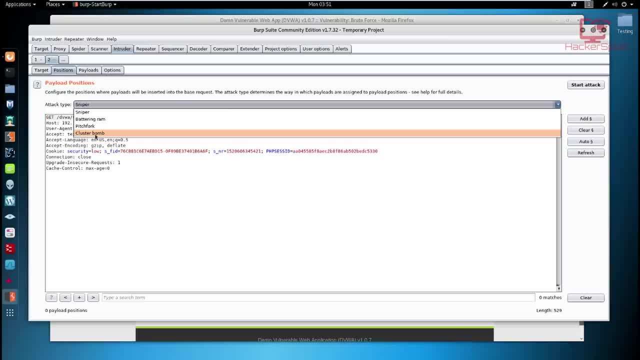 cluster bomb attack type is because we are going to be using two values. we are brute forcing against two values, remember that. okay, and these need to be set in in combinations. So that means it's much better to use a cluster bomb because essentially you're clustering two values. that 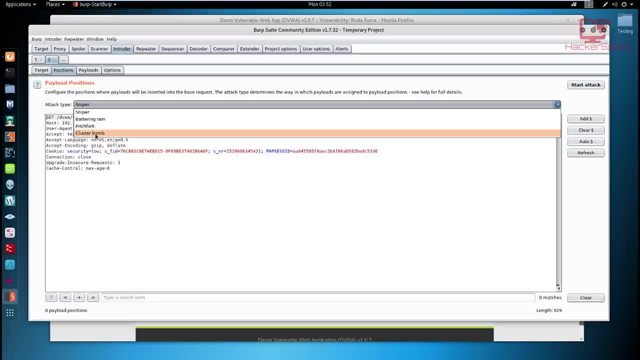 need to be, that need to be tested against the login, the login application or the login form together. Alright, so in a combination. so we need to select a cluster bomb And now we need to select the values, because those are the, those are, that is. 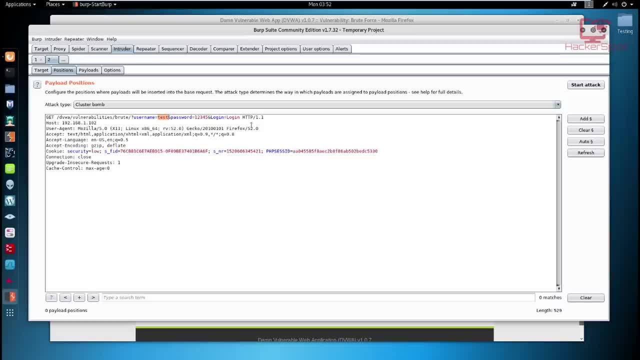 what we want to brute force again. So just highlight the value. It doesn't matter what the password or the username is, just highlight it. And you want to hit Add? Alright, so just hit Add And, as you can see, we have selected that. you know, I'm going to the password. 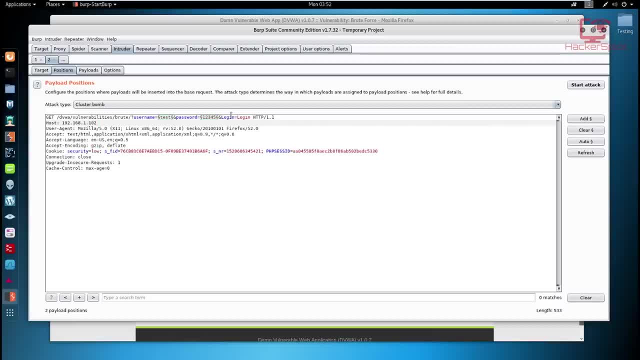 and you want to highlight that as well, And you just want to add that, As you can see, now, once we have added that those are the two values we're going to be brute forcing against, make sure that none of the others are selected, none of the other values. Once that is done. 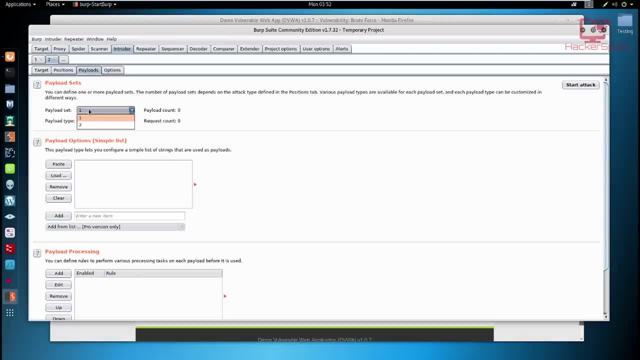 you're, you're almost there Now. now you want to go into your payloads. Alright, now, in your payloads, you want to make sure that your payload set is set to two, which is your username and your password. So let's start off. 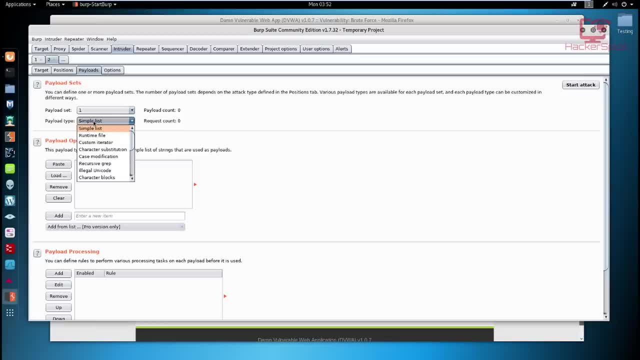 with your payload set as payload one, Alright, as your payload type. make sure that that is a simple list Because you can see we're only targeting usernames and passwords, So we don't need, you know runtime file or we're not changing anything you know dependent on Unicode. 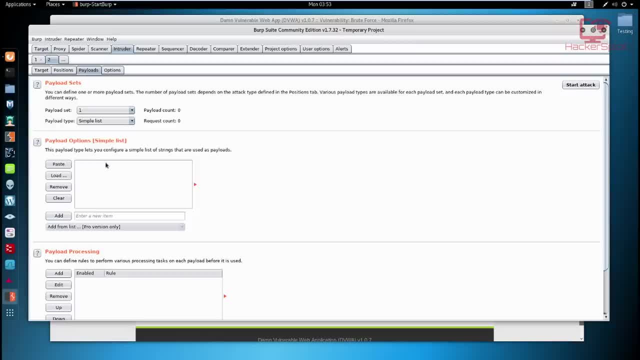 etc. you get the idea. Okay, so simple list. and now you're going to your payload options, which is where you select your user list or your password list or your word list. Now we are not using a word list, But if you want to, you can. if you're performing this on a real site, which I 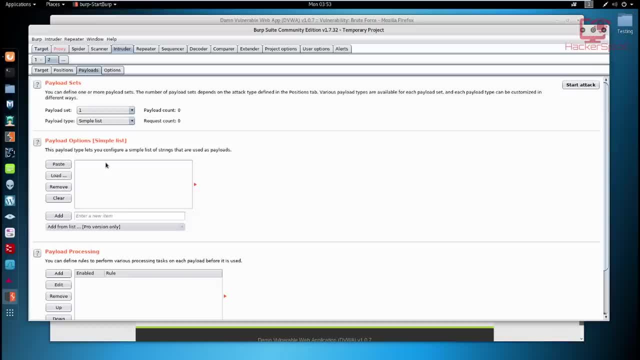 don't recommend unless you have written permission. Now, since we're using this in our penetration testing lab, we are going to just add the default usernames. As I said, the security of the site is low And it's not really a complex brute force to crack. Okay, so what we want to do is we want to. 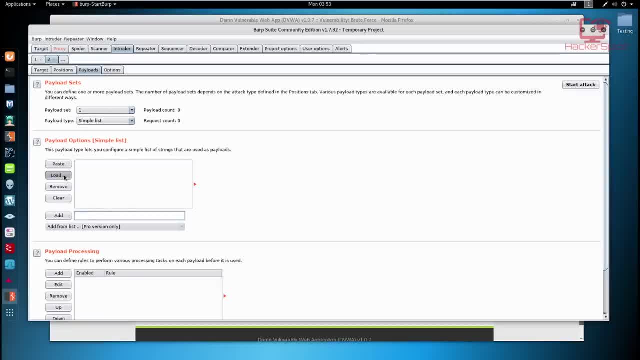 make sure we have set payload set to one for our usernames. So now we can go into load where you can load your default usernames and your passwords or your word lists. But by default we're going to add our own, Alright, so we're going. 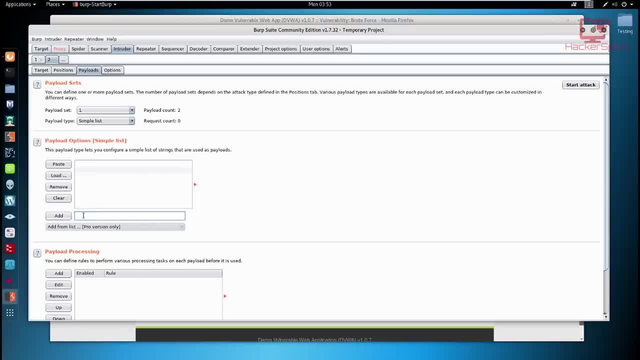 to say: whoops, some, we're just gonna say we're going to type in and now like the commonly used usernames, Alright, so something like admin, administrator. oops, for some reason actually, let me just remove these blank values there. admin, now administrator, administrator. let me just type. 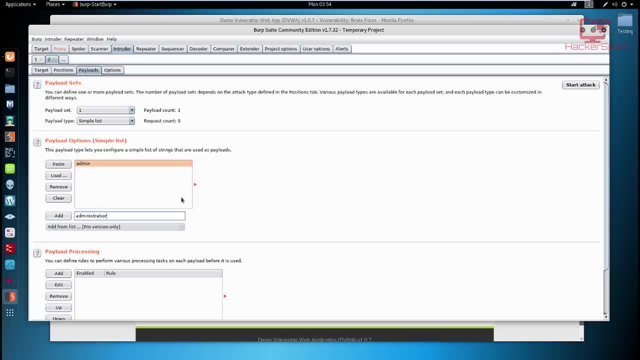 that back in Administrator, like. so, administrator, for those of you telling me that my typing is bad, that's because my microphone is right in front of me and I can't really see what I'm typing. Administrator, let's see what else. what are the default ones? like? we have root, we have password. actually we're. 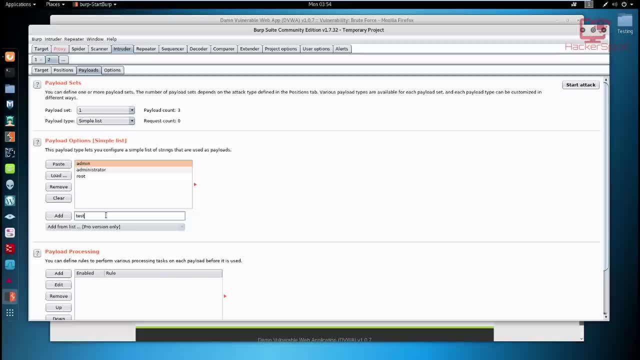 not setting the passwords right now, So we can just type in the default ones like this: Alright, so we can say: test, you know the default ones, user one, whatever you think could be the most commonly used ones, Okay. or if you know what the username is, that is even better. So we're going to add all the usernames. 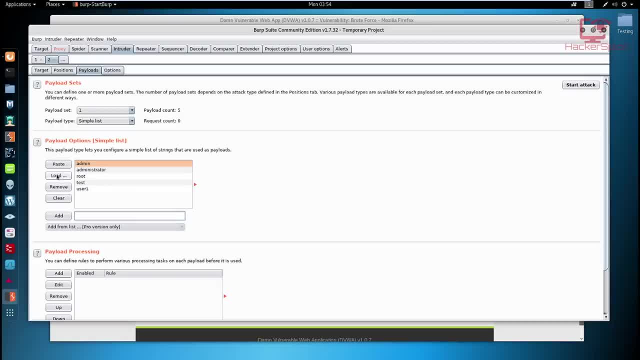 Alright, so we've added the usernames that we want to use Now by default. again, I'm saying you can use a word list if you want to, just going to load and select the word list. Now we want to select our passwords. Alright, so we can go into the payload, set two And, as you can see, now we 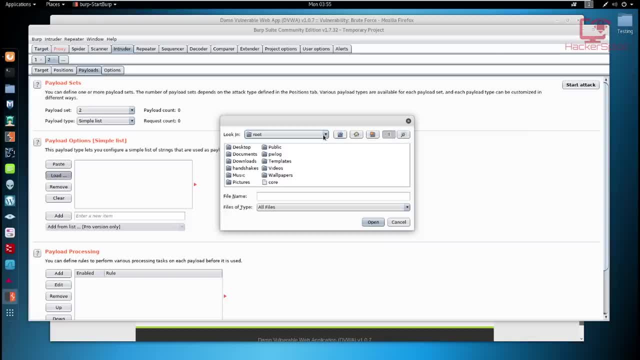 can add our own values. Now we can use the default word list that come with Kali Linux. So if I go into my route and I go into user share and we select word lists, let me just find where we're word lists are, if I can find them. there we are word lists And the ones that work great for me. 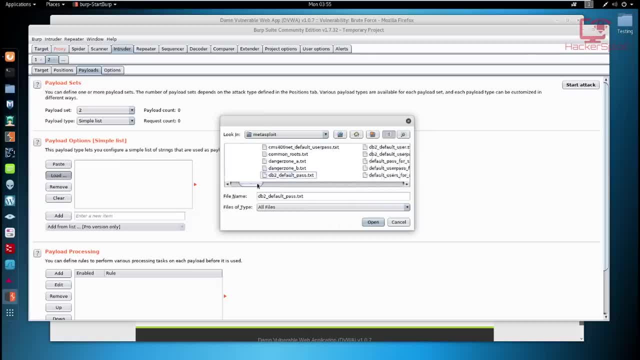 are in the Metasploit folder And you can look for the default passwords. As you can see, you have your database default passwords. you have your default user passwords for services. that's also great. It has a great list of of default usernames and passwords that you can use. But for me, 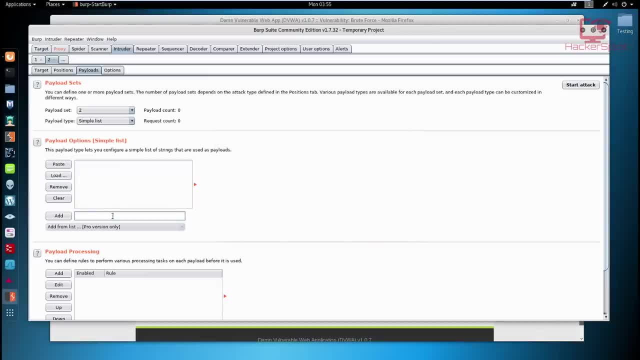 I'm not going to use this because we are sticking to the basics Now. now you want to add your own password So we can select again some randomly. you know commonly used passwords, So password, you can say password. Let's see what else. admin. you know admin again. whoops, let me just remove. 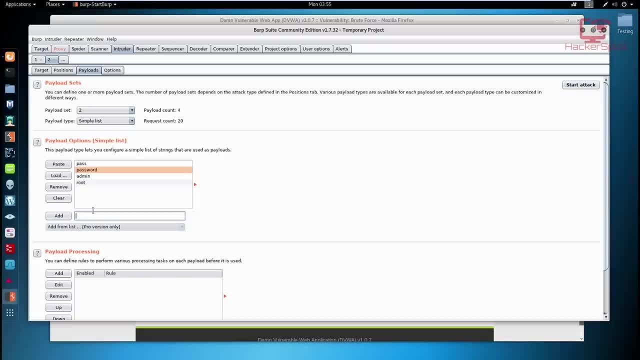 that one admin route you can use route, Let's see, let me think 12345.. That's also one that I've seen many network administrators using, 12345.. And you, you get the idea. Alright, so I've set our. 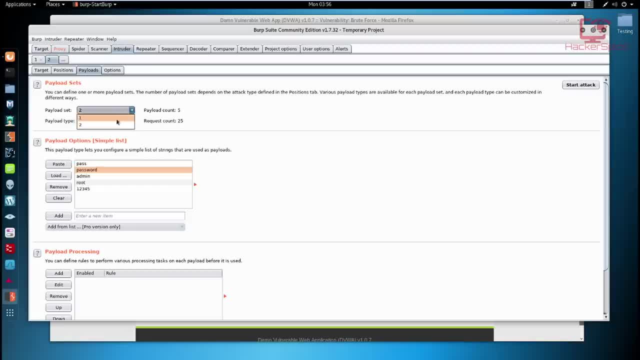 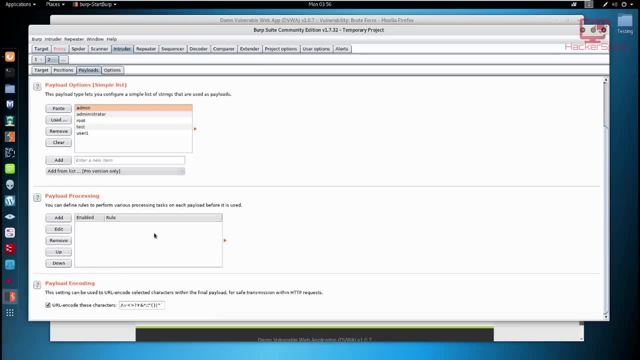 two payloads. payload one is set for usernames, Payload two is set for passwords. Excellent, All right, Now we have selected our payload types. we've selected, we have added our payload options. we don't need to look at payload processing. that is advanced. Once that's done, what you want to do is going to intruder. 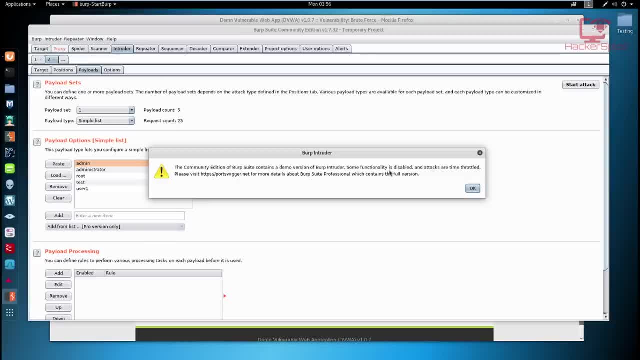 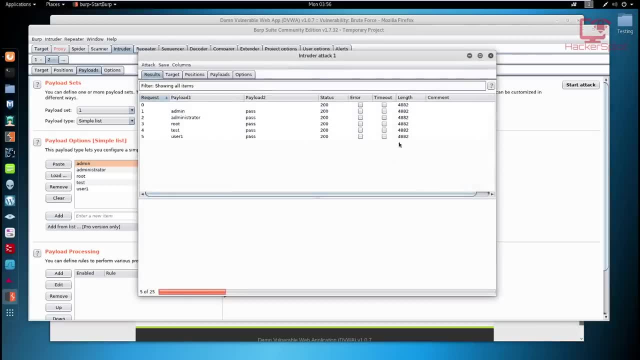 and start the attack. All right, And now it's going to tell you that the community edition of burp contains a demo version, But it's essentially telling you that the process is going to be slow. All right, so we're gonna hit. OK, And it's going to start at the attack, As you can see. 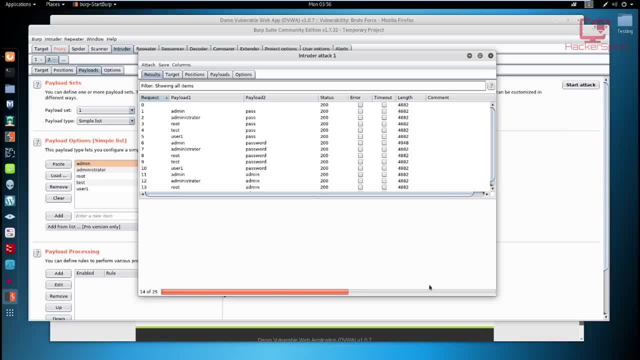 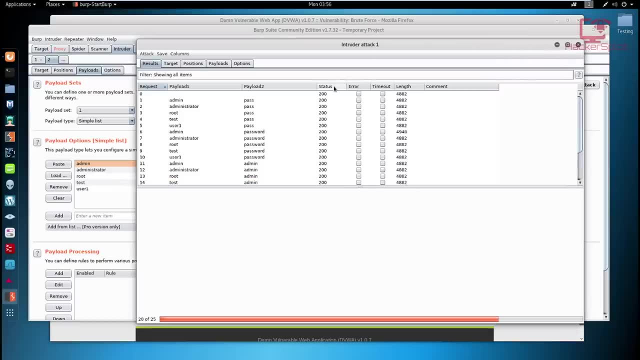 it's going through all the combinations And, as you can see, there are combinations that we have here are 25.. And it's going to go through all of them. Now, one great thing that you need to do here, or one important thing that you need to do, is you need to understand the these, the status. 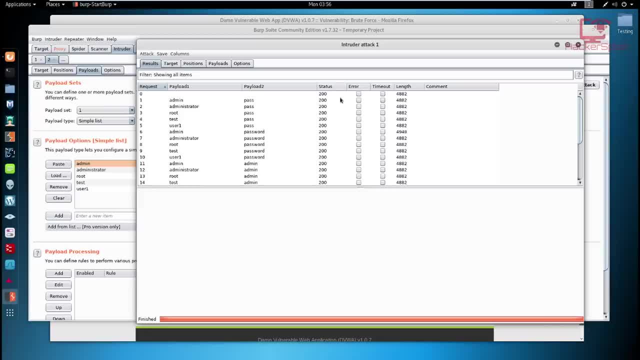 codes that the server or the web application is sending back. Now that's a good way of understanding what password is correct and what, what username is correct and what password is not correct. Okay, so if we look now at the, at the results, as you can see that it's finished, it's gone through the. 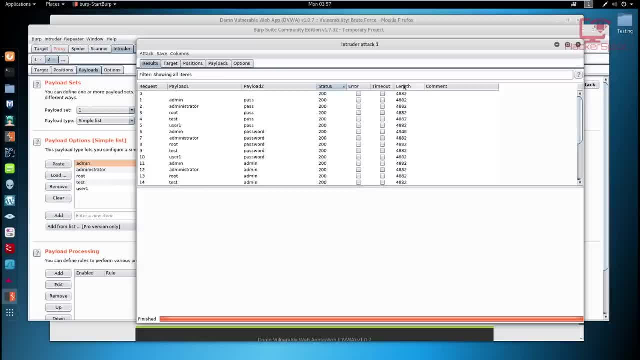 brute force attack. we check the status: the status is still the same. we have a status to 200.. If we look at the length, all right, the length is going to be still the same, But you have to look for things that are not, that are not matching. So, for example, you can see that the length here 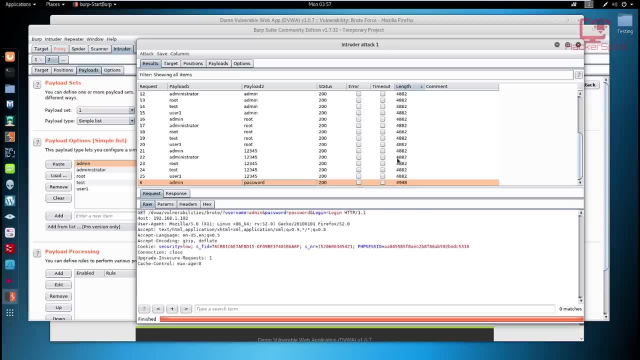 that was returned was 4948. And it's not. it's not following the format of the others, So that means that this could be the username and password. don't worry about the status. the status will still remain the same regardless of that. But when we'll be looking at advanced server penetration, 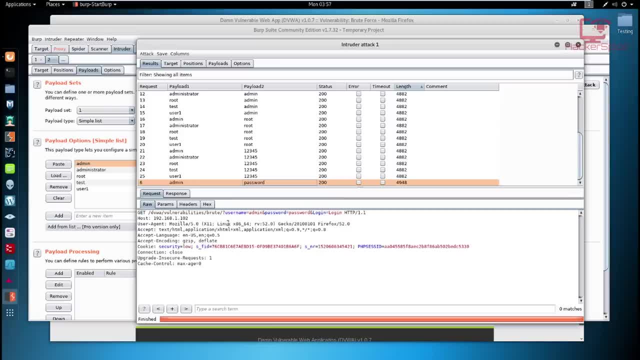 testing. that's something important. So you can see that the get that we've got here is very important. Now, if we look at the, if we look at the response that will be sent right there, you can see the, the response, And if we render it, you can see that if it was successful. 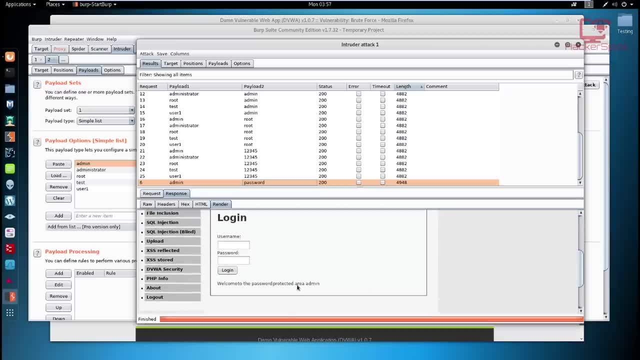 it will tell us that we've logged in successfully, So let me just browse down all the way, as you can see. welcome to the password protected error admin. And there you go. that is the username and the password. It is admin and password. Now, again, this was really simple. Again, you can you. 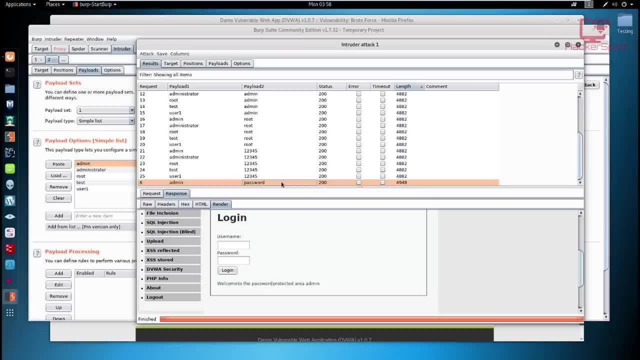 can increase the security if you're practicing on your own, But you can see that this really works And this is how to utilize burp for advanced stuff like brute forcing. Now again, most of the advanced websites nowadays have great content management systems that have the security. 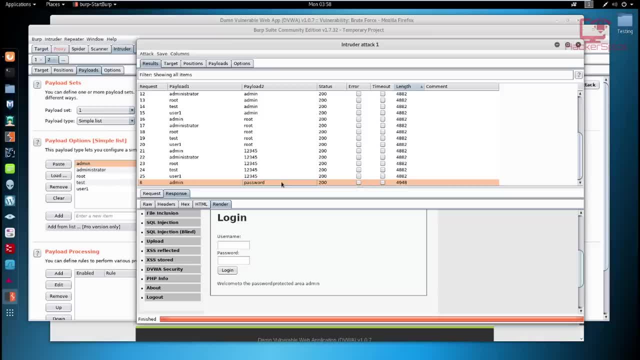 plugins that essentially prevent you from brute forcing or lock you out. But most of the older sites you'll be you'll be actually quite shocked to find out that their brute forces, their login forms- sorry- are not protected. Now we have already logged in And you can see that the 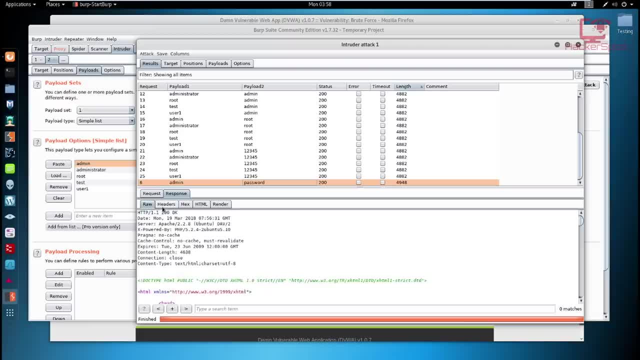 default username is admin and the password is password. Okay, so you can look at the raw, the raw HTTP here. you can look at the request and the response. You can look at them and you can inspect them, If that's what you do, And you can look at the headers. what's being? 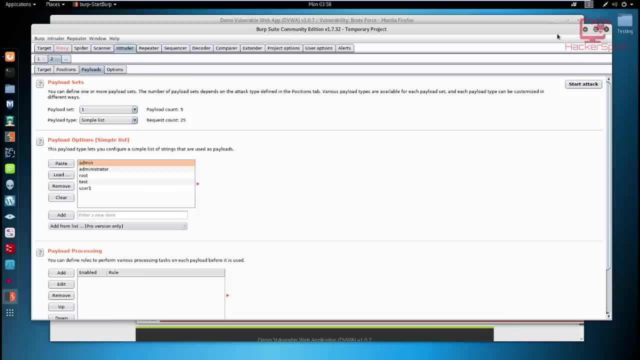 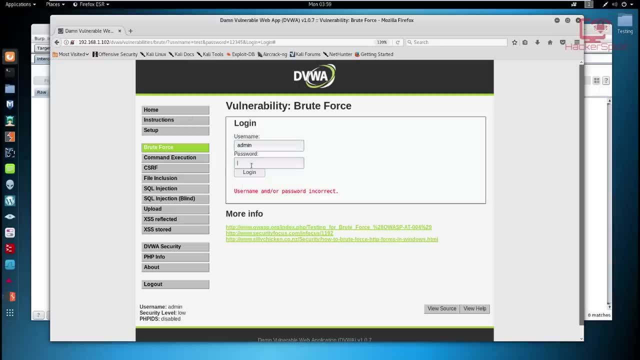 sent all that good stuff, But that was going to be it for this video. And now, if we just go back into burp, let me just go into my proxy And I'm going to disable intercept and we can try and log in here. So we know that the admin, the username is admin and the password is password. So let me. 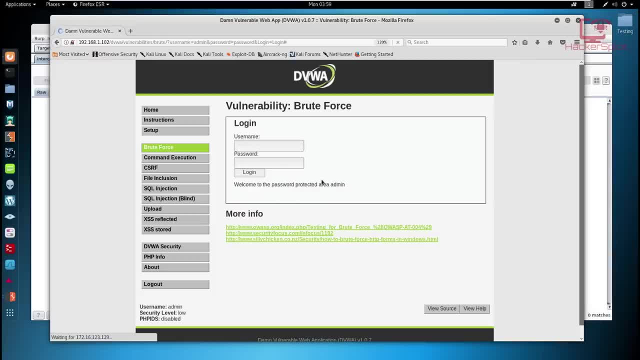 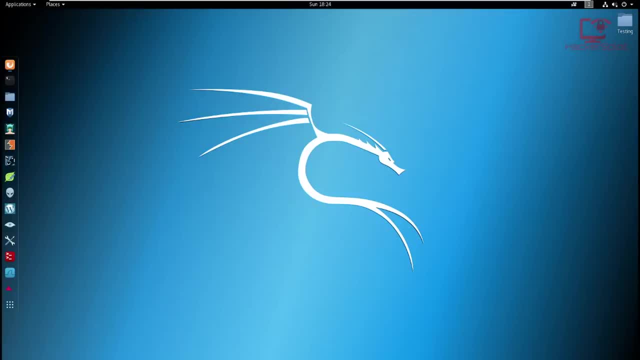 log in And welcome to the password protected admin area. Fantastic, In this video we're going to be looking at selecting our burp suite, our target in burp suite, adding it to our scope and then finally spidering it as my vulnerable. 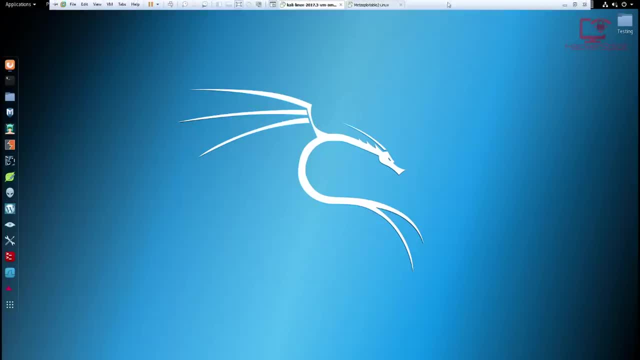 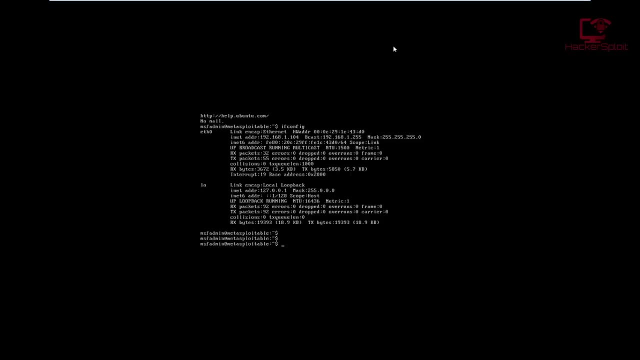 operating system. I'm going to be using the Matilda day, which comes pre installed on metasploitable, So you should download. Well, I would recommend that you download metasploitable to. it's a fantastic option for any of you who are just getting into penetration testing and offers. 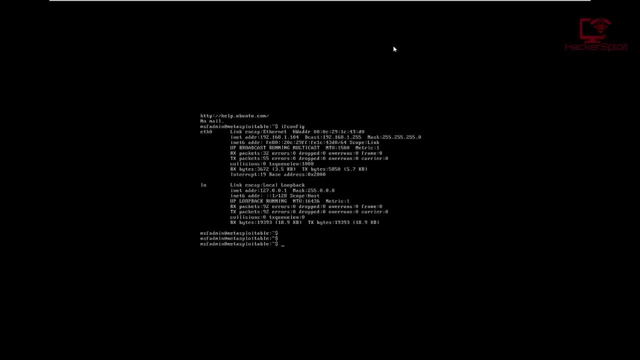 multiple vulnerable web applications and vulnerable systems that you can practice with. So, again, it's something that I really really recommend. That being said, as you can see, I have the metasploitable to virtual machine running And I have already looked at my local. 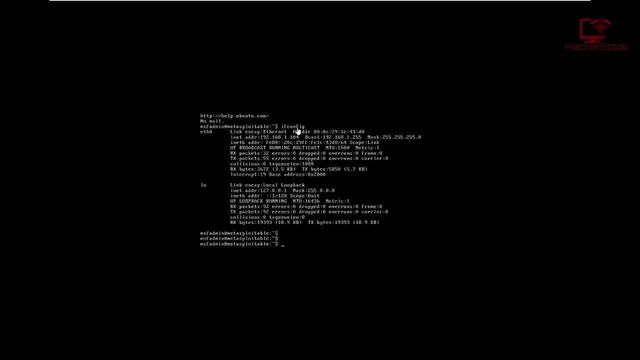 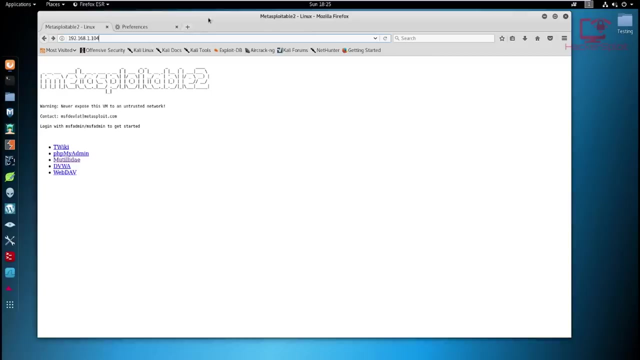 IP address. you can do that by typing in if. config. that will display to you your your current network interface and your local IP address, Because we are doing this in our virtual penetration testing lab. All right, so let's go back to Kelly Linux now, And I'm going to open up my browser. make sure you. 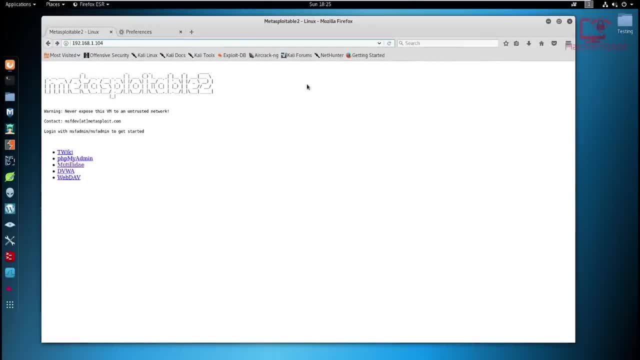 get your IP address And, as I said again, we're going to be using Matilda day. So if you don't know what Matilda day is, Matilda day is simply a vulnerable web application And the reason I'm switching off, I'm switching from the damn vulnerable web application- is because I want to 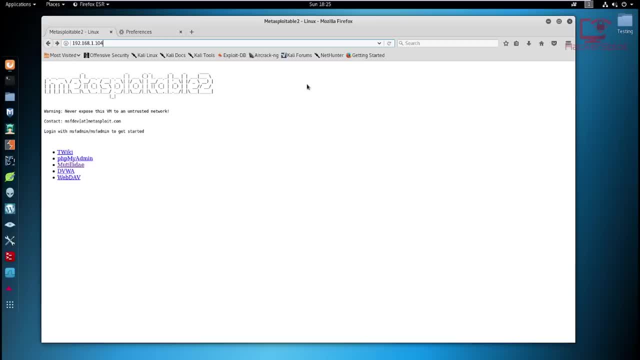 show you a few. I really want to make it a bit diverse in terms of the web applications that we use. All right, so let's get started Now. Now I already have the IP address of my virtual machine opened up here in my browser, as you can see: 192.1, 68.1, point 104.. So if I reload this, you can see: 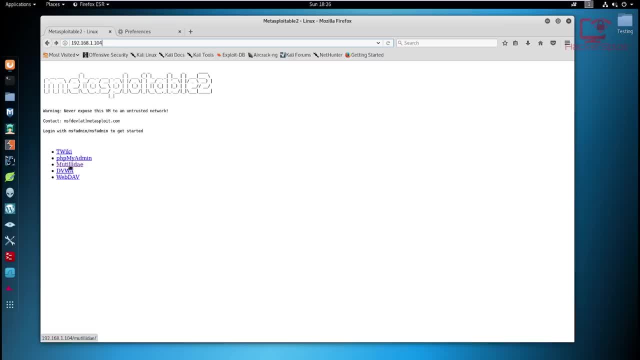 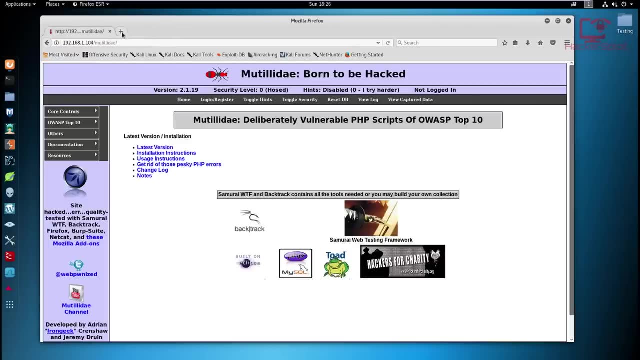 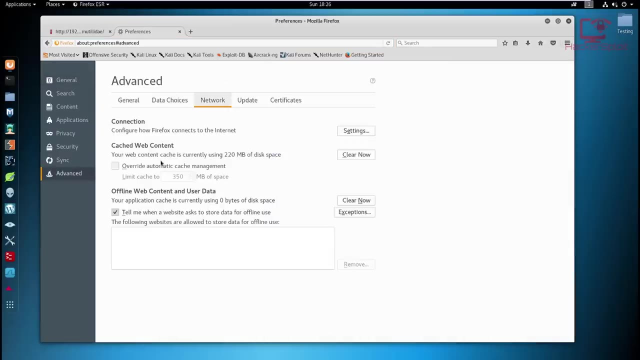 that it indeed is the metasploitable to server And I can just go ahead and click on Matilda day. Alright now. what I should do now is going to my preferences. you can do that by opening a new tab. So let me just open a new tab here, going into preferences and then selecting advanced and 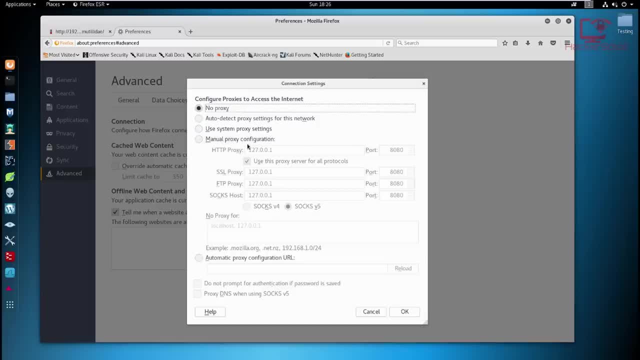 network and finally settings. And then you want to make sure you select a manual configuration And then make sure it's using the localhost proxy, which is 127, point 0.0. point one, a port 8080, and hit OK. Once that's done, we know that burp suite can intercept, not that we want. 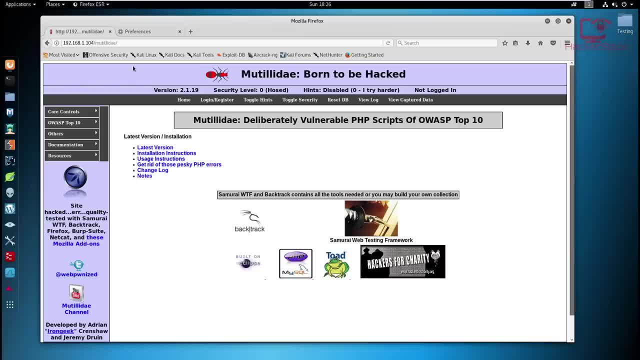 to do that in this video. we just want to. we want to have a look at, we want to map the web application. Alright, so we're not going to change anything in Matilda day, but I'm going to be showing you some pretty interesting things in this video. So now we should start up, sweet community. 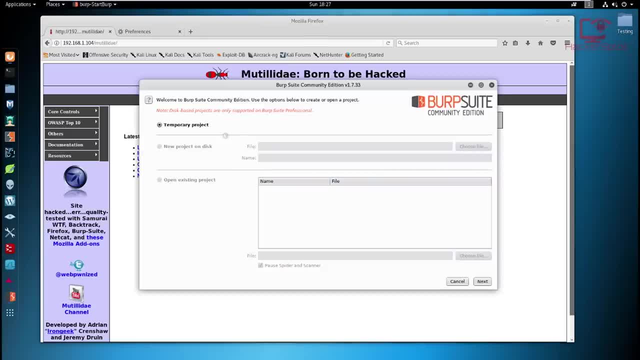 Now I'm going to be explaining something At the end of the video that is really important, And it is in regards to the community version and the professional version of burp suite and what, what the differences are and why you will need at some point to get the professional version. Okay, so I'm going to select a temporary. 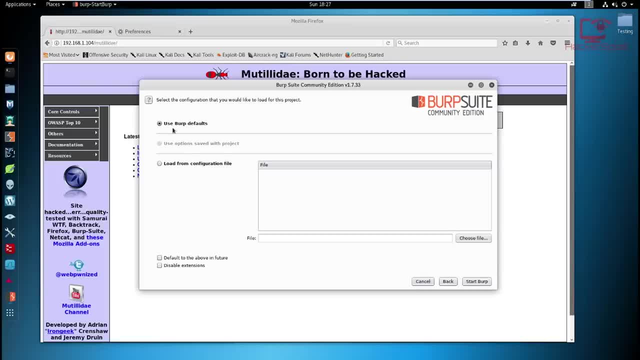 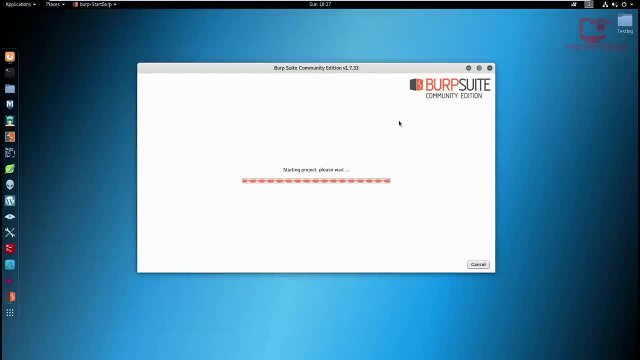 project. I'm using the community version as of right now. hit Next, use the BEP defaults And I'm going to start up. Alright, so it's going to start burp suite And let me just minimize the browser here, So give that a few seconds to start up. 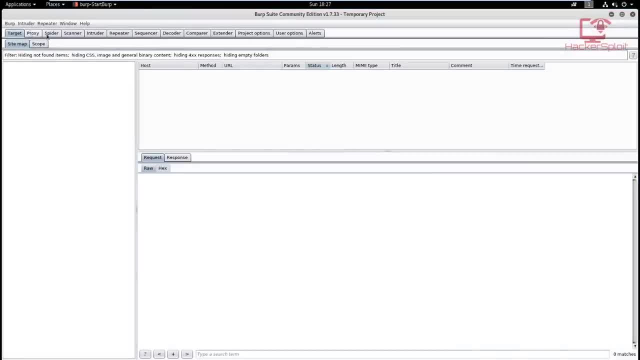 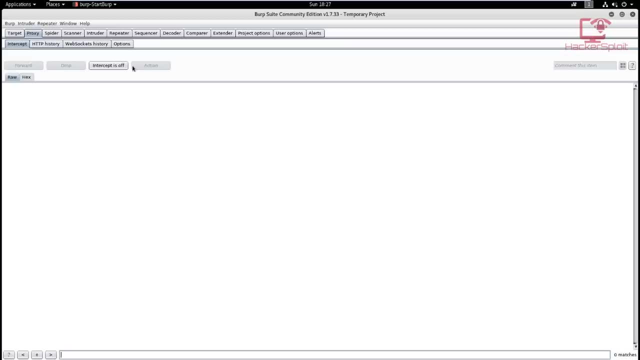 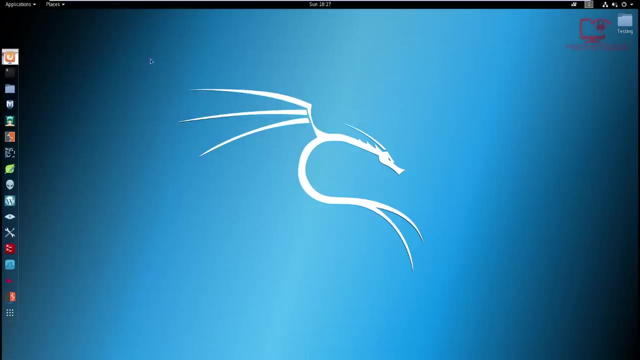 And it starts up. what you want to do immediately is turn off the proxy. we want to stop intercepting because we are not intercepting any requests or we are not intercepting any responses. So go back into your target And now we can get started with with actually reloading the page right here. So 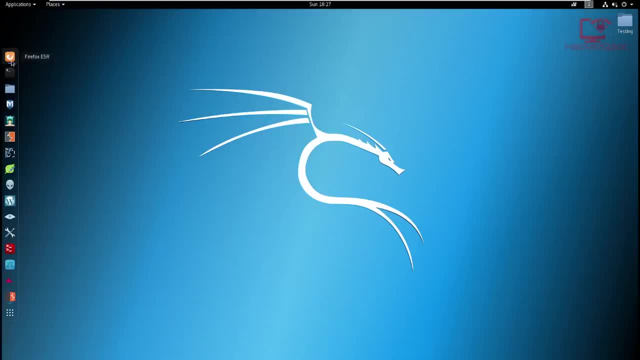 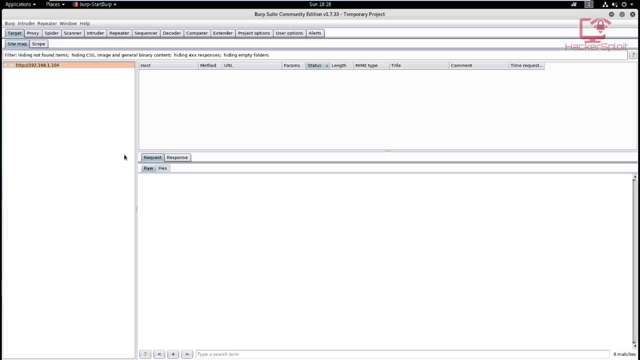 let's reload that And we should be able to see what's going on And we should have the site map. Alright, so let me just open up the burp suite here. Fantastic, Alright. so now you can see something very interesting has happened here In our target. 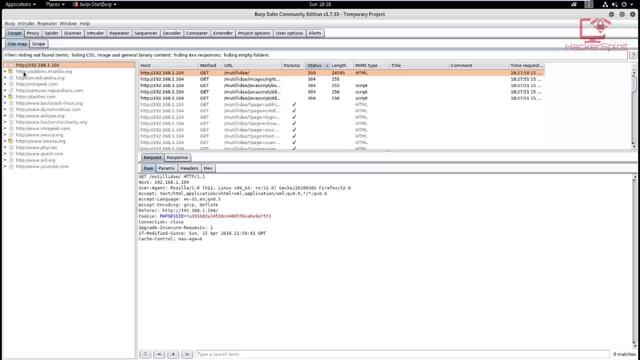 and site map. we have the files that were discovered here. Well, essentially, we have the web server. that then has the motility folder, which is our target. Now, before I get into any of that, the site map will show you the current site map. Obviously, a site map is essentially sorry about. 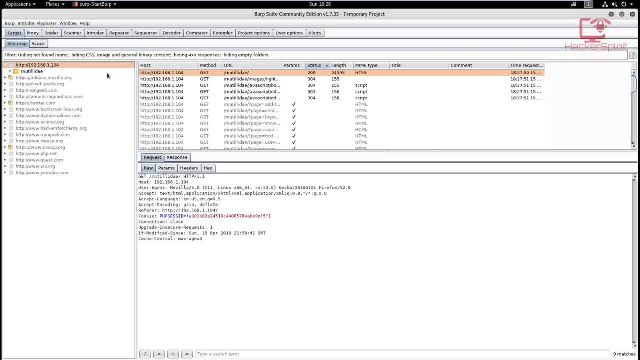 that A site site map is essentially the structure or the format of the web page and how the web page was constructed and how it will function regards to every other piece of content. Okay, So the first thing that we need to do, or we'll be- 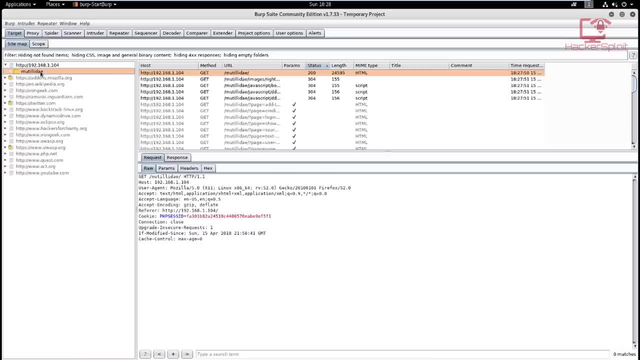 looking at is actually selecting our target, which, in this case again, is motility, And you can do that by right clicking and hitting Add to scope, Alright. so you might be asking: what exactly does scope mean? Well, a scope essentially allows us to define our automated spidering And what this 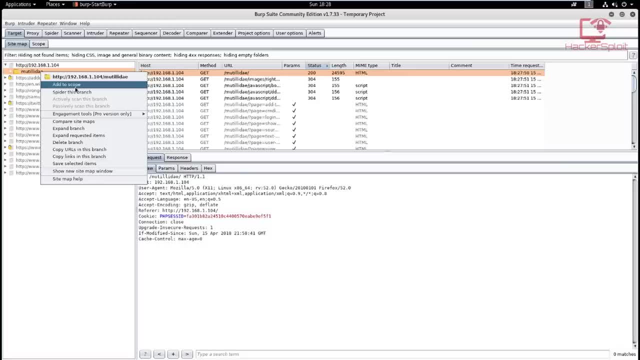 means is we are focusing our only on our target. we're not going to focus on the reference links, like you can see here. for example, we have Twitter as a reference link, track, dynamic drive, Eclipse, etc. etc. you get the idea. So scoping is essentially selecting our 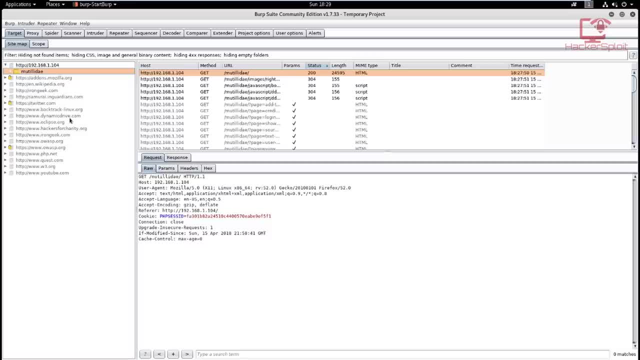 target, isolating it so that we only see what we need to see And the, obviously, the results that we want to see. So I'm going to right click on motility And I'm going to hit Add to scope. All right, So now it's going to say: you've added an item to the target scope. do you want? but proxy? 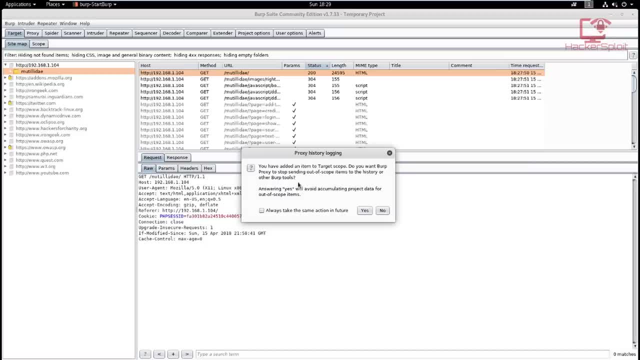 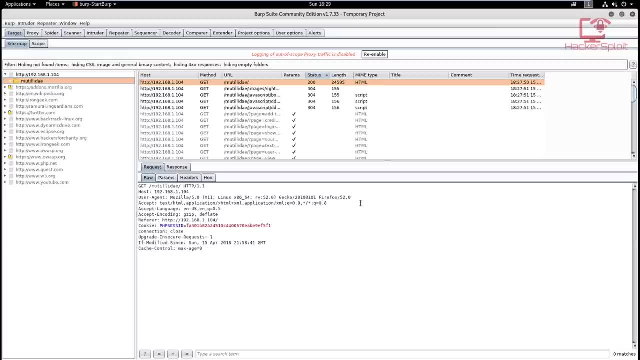 to stop sending out scope items out of scope items to the history of the other tools. Yes, Again, we want to make sure that we are. we clear out all the junk that we don't need. Now, you might have noticed. well, that's essentially. 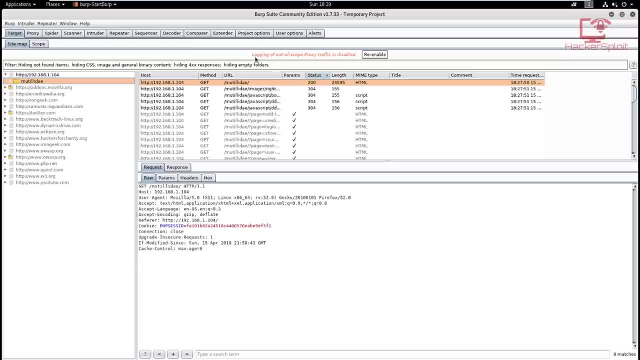 happened, but nothing has really changed And, as you can see, it's going to tell you here: logging of out of scope proxy traffic is disabled. Don't worry about that, Just leave it as it is. If you want to re enable it, you can go ahead, But right now you don't need to do that. Okay, so we've. 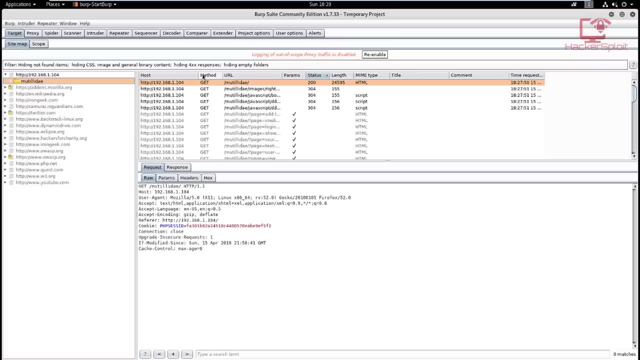 looked at how to add our target to the scope. Now let's look at spidering. spidering is essentially the the first and the most important step of web application penetration testing. All right, it is, it deals with or it is in. it is in relation with: 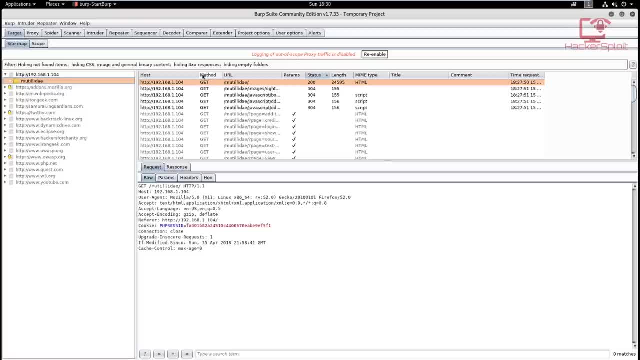 footprinting And this is why I bring the comparison from penetration testing to, obviously, web application penetration testing. it is to deal. it essentially deals with crawling through the website and then it records all the files, the links and the meta, the methods that it can get. 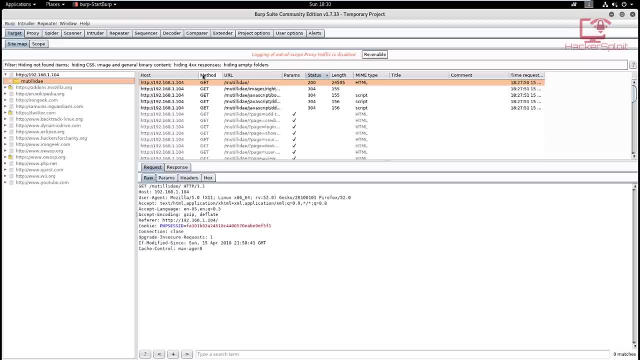 And that helps us build an idea of how the web application is structured, how it works, And then, finally, we can learn how we can break through it. What we need to do is we need to spider our target. we have added it to the scope, which is: 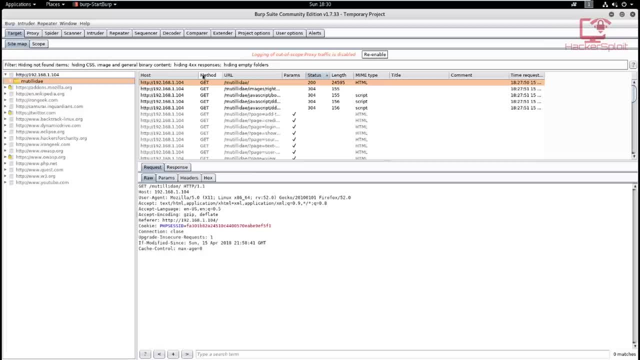 great, And now we need to spider it. So what we're going to do is we're going to, we're going to use spidering, And this will help us identify all the links and the parameters that we need. Again, as I 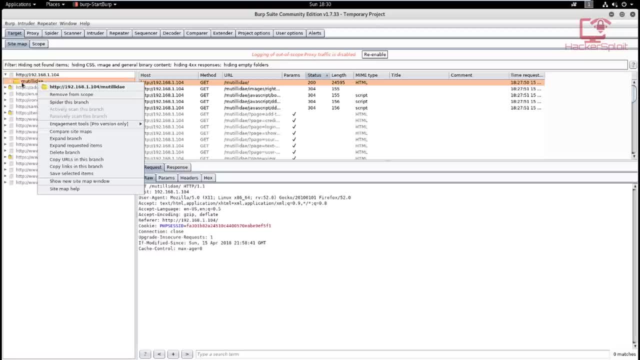 said, it's like footprinting. So what you want to do is right click on your target, which in this case, is motility, And you want to hit spider this branch. Alright, so I'm going to spider this branch, And now something interesting is going to start happening. As you can see, it's going to 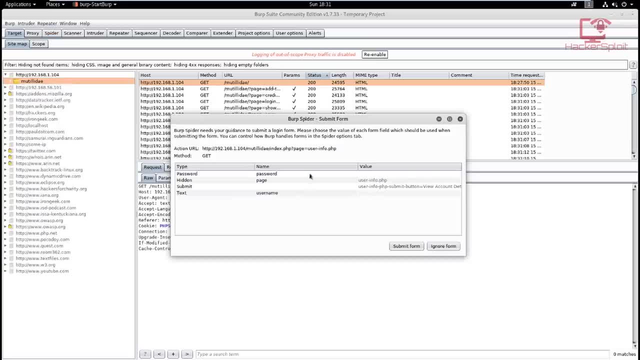 start getting all the links, all the resources that it can, And it's going to prompt you with here, a submit form. Okay, now what you can do is just ignore the form. there'll be quite a few. essentially, these are default login forms where it's asking you to. 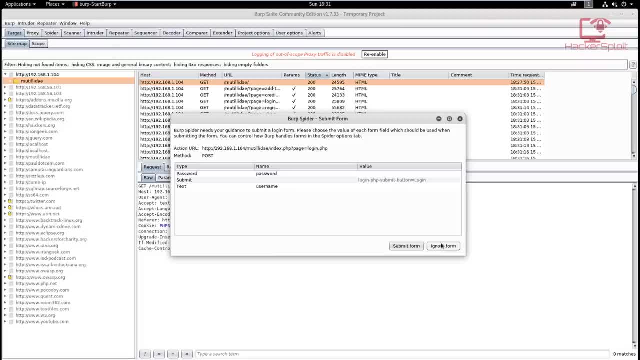 enter credentials that you might want to enter. let's say you you're performing white box penetration testing and you have the details. you can again log in like this and perform internal penetration tests, But we're going to assume that you do not know your penetration. 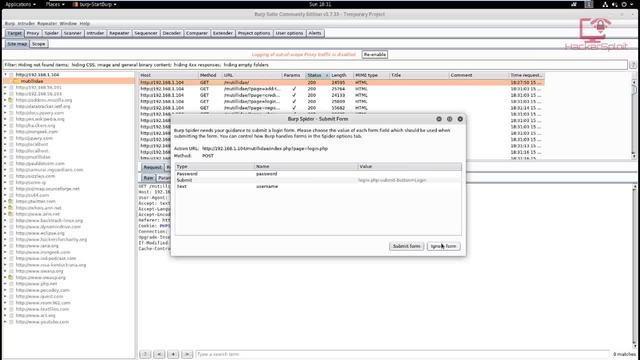 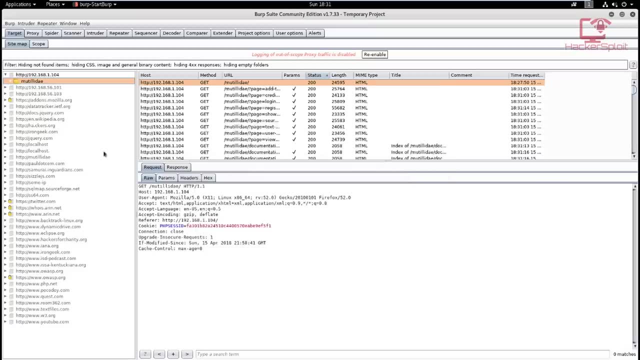 you're essentially performing a penetration test on the security, So I'm going to ignore all of these forms. Okay, And, as you can see, there's another one right there And the spider ring is probably continuing. Now, if you want to view the status of the spider ring, you can go into spider And, as 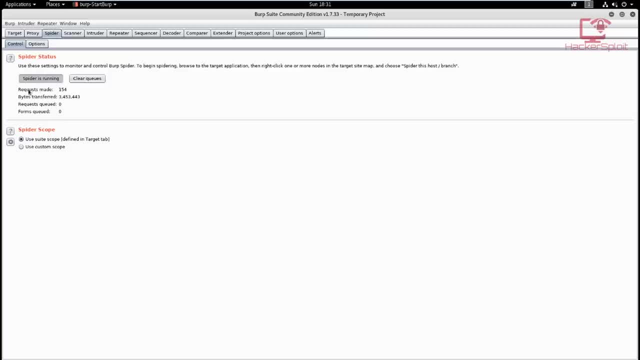 you can see. you have your status of the spider ring And once it's done, you will see that the requests made will stop changing and the bytes transferred will also stop changing, So we can stop the spider. Now you noticed something that we were faced with, those form login prompts. Now 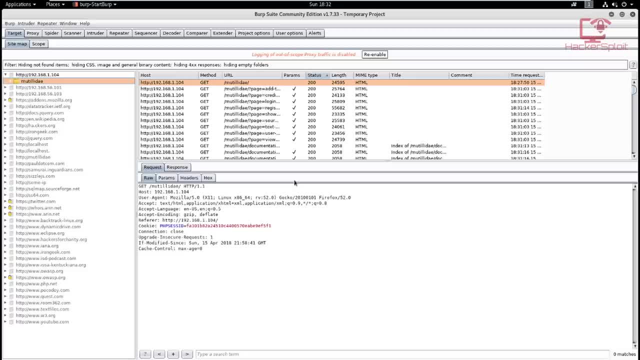 you can choose to enter them as it prompts or as your prompted, But the better way of doing this is to actually you can actually do this automatically And you can do this by going into spider And you want to go into options And you want to go into your. 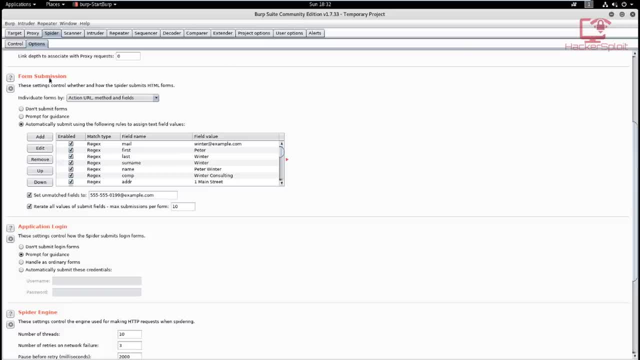 application login. All right. Now, if you look at the form submission, it is essentially what it's doing is it's going to use the default form submissions that you would find in a database. So, for example, you have mail- first name, last name, surname, name, address. you get the idea. So those 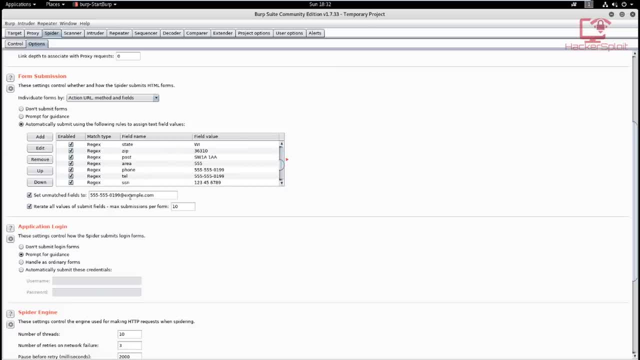 are default values that one would, one would be expected to find. Now we're looking at the application login. as you can see, its option is set to prompt for guidance. we want to change this to automatically submit these credentials. Now in here you can enter default credentials or if you have an idea of what the 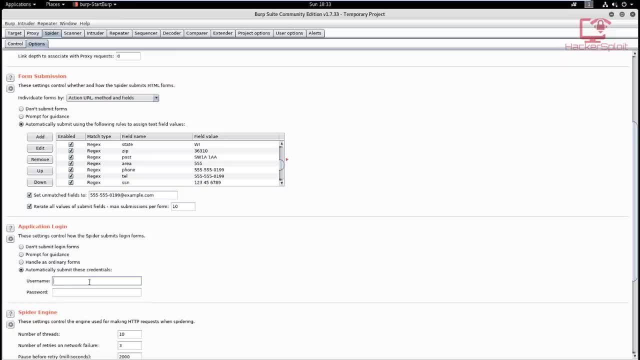 credentials you might expect to find Now. this is where creativity and sheer information gathering comes into play. So if you knew the default, you know usernames and passwords. you can enter them here. Now, what I'm going to do is I'm going to 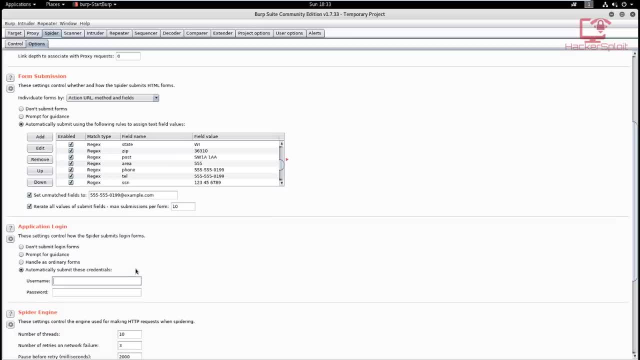 enter a string. that is well. I've used it before in performing SQL injection And we'll talk about SQL injection because it is very advanced. If you know SQL injection, or you have, you have an idea or experience with the databases- you might understand what this string means. Alright, so for. 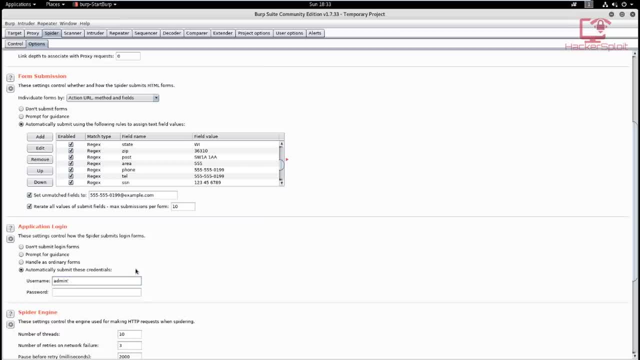 my username. I'm going to change that to admin quotation mark and say: or one equal one and two dashes. All right, space and a dash. Now you don't need to worry what this means. for now, please do not stress about this. I will explain. 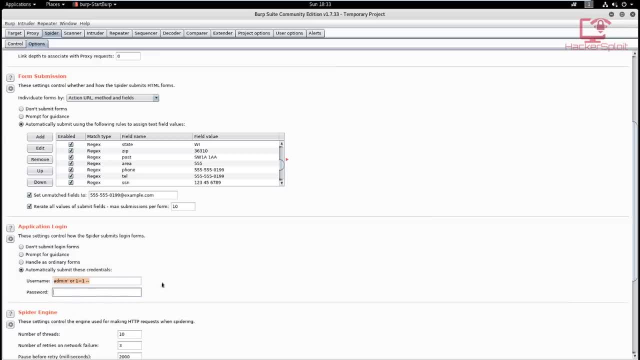 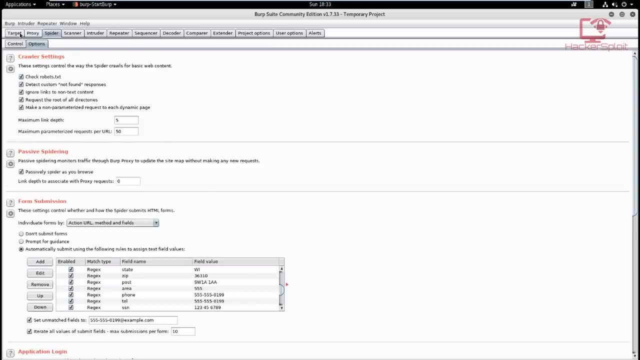 it when the time is right. Alright, so leave the password as it is And don't worry about that. Now we had- we don't need to change anything in terms of these tabs. we talked about these tabs in the theory section And now we can go back into our control and target And, finally, we can spider. 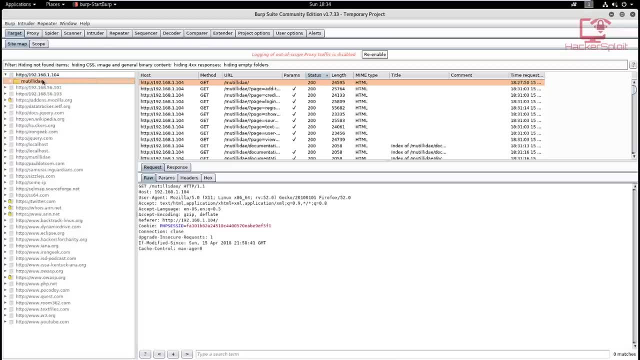 the application again once more so that we can enter the. we can essentially process the strings that we, that we just entered in terms of the username. So I'm going to right click and spider this branch. Okay, so it's going to start spidering And if we look at the spider, you can 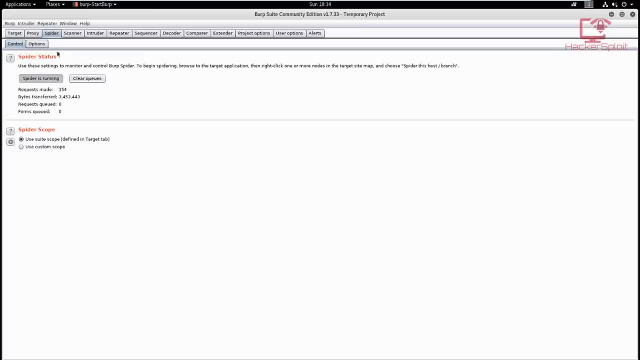 see that the the spidering is complete And you can essentially clear the queues if you want to clear, clear them, like so, And you can keep on running it, depending on what you want to do. Okay, so I'm just going to pause it. And now we have essentially spidered the web application And you 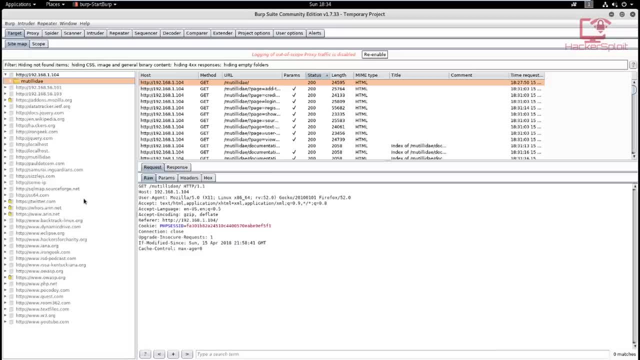 might be asking. Well, I've seen a few reference sites. that's not helping much. you know we don't need twittercom Or, you know, sizzle js. this might give us a basic idea of what types of sites are linked to the web application, But in reality, 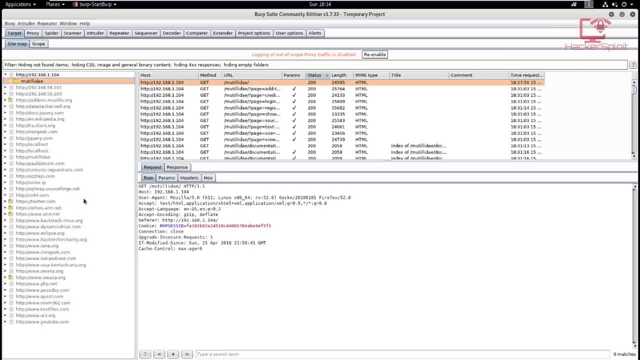 you can see we have hackersorg, not not very important information at all. Now, what if we click on the motility folder? Oh, look at that, That's really interesting. Now, that is very, very important. What has happened here is it's given us the structure of the web application. 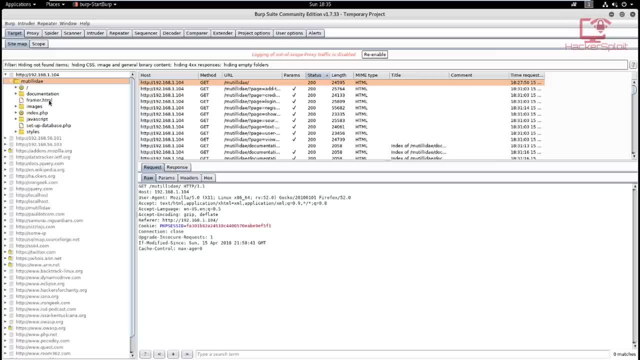 this is vitally important Right now. again, as I'm saying, you can look at how the website or the web application is structured. Now, as I'm saying, you can look at how the website or the web application is structured. So in documentation you can see, you can go ahead and read the. 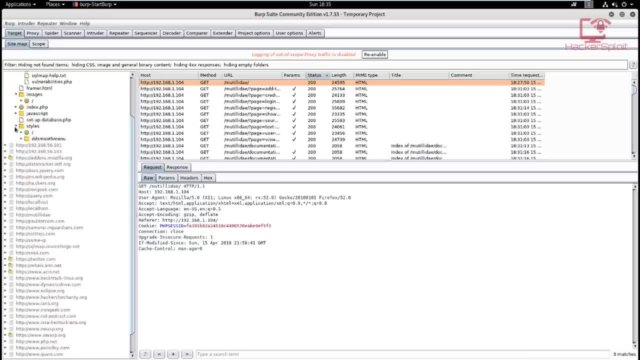 documentation. you can look at the images that the website has, the styles, So you can inspect the entire site and understand what exactly is going on here, or get an idea of what the person who developed the website was thinking. And then finally, out of experience or as we'll be looking, 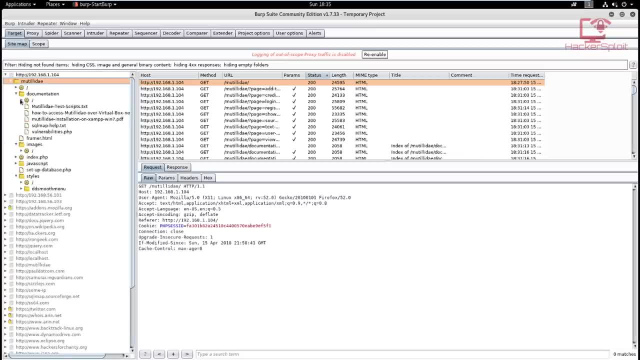 at. out of knowledge, you can actually understand how to exploit a system, And that's. we will be talking about discovering hidden files. hidden files like admin pages, login pages. you know that really juicy stuff And we'll be talking about that in the next video, And that's. 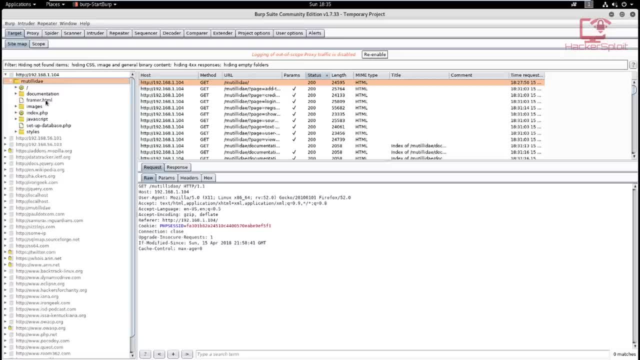 because burp suite Community Edition does not support or have allow you to use that feature. So what I'm going to do in the next video, I'm going to be using burp suite Pro and also show you an alternative program- I'm sure you've heard of it- That also works on Windows, Of course. 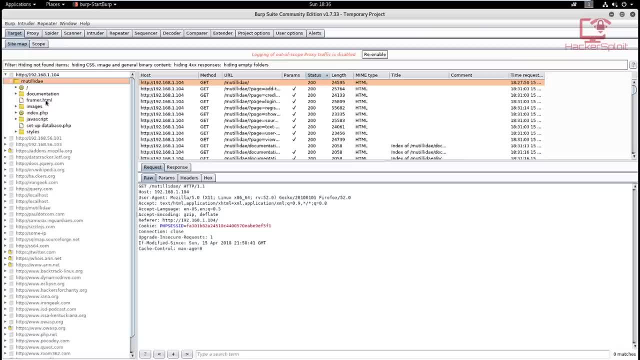 burp suite works on Windows, but I'm not really a Windows fan when it comes down to penetration testing. So, that being said, we have, essentially, spider, the application, we have the structure of the web application, And now we need to look at something also very interesting, as we have. 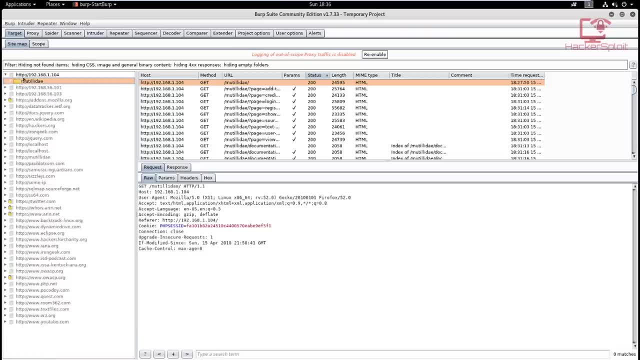 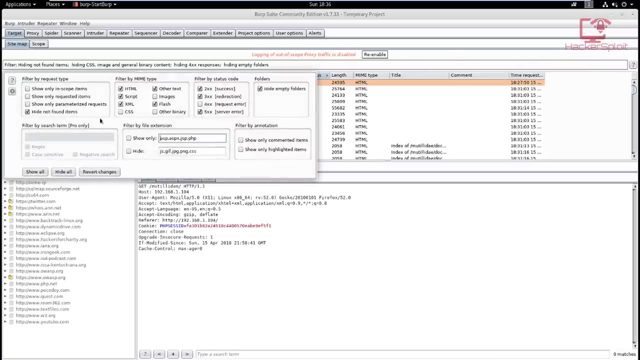 already talked about it. Let me just complete, Let me just show you how to get rid of all of these reference links and to essentially show the items in the scope only. So what you can do is just click on filter right here, this little bar. here is the filter bar. So click on it And it's going to show. 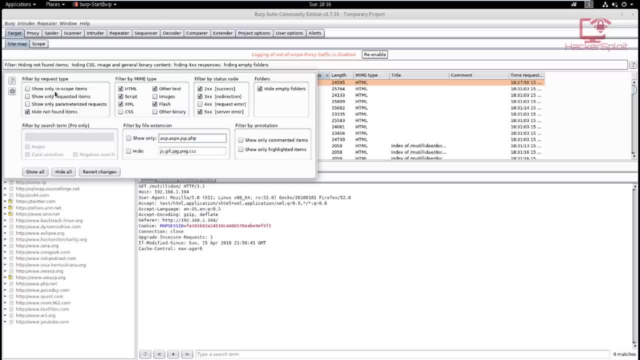 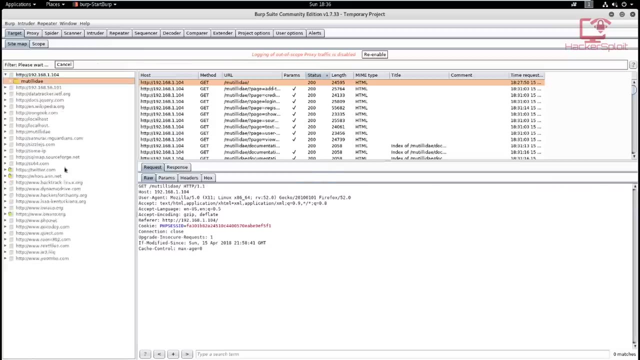 you bring up this small little window and you want to focus on the filter by request type and make sure you check show only in scope items. this will essentially filter all the results to show you only links, resources or files that are within the scope. So once that's done, just click back on the filter And, as you 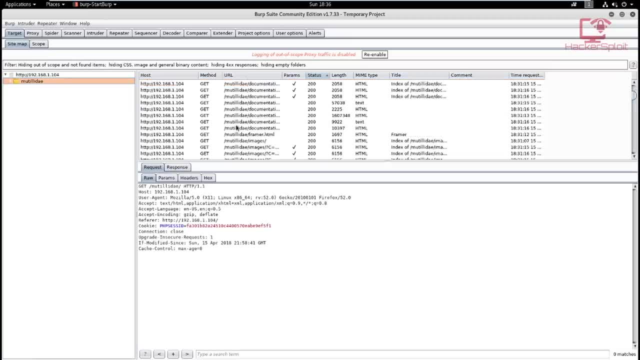 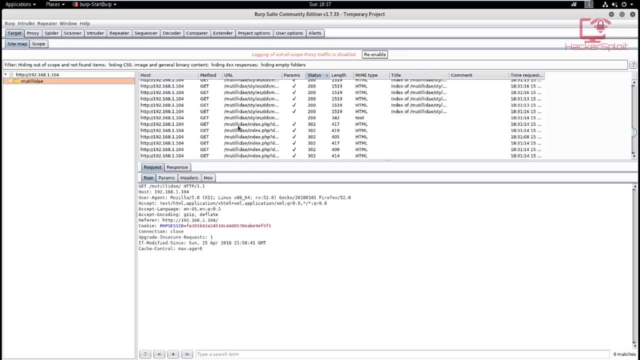 can see. it has got rid of all the junk that you do not need whatsoever, And now you can essentially look at the, the requests and the responses and analyze them, accurately defined to your scope, And this will essentially, it will stop confusing you. I've seen many beginners make this mistake where 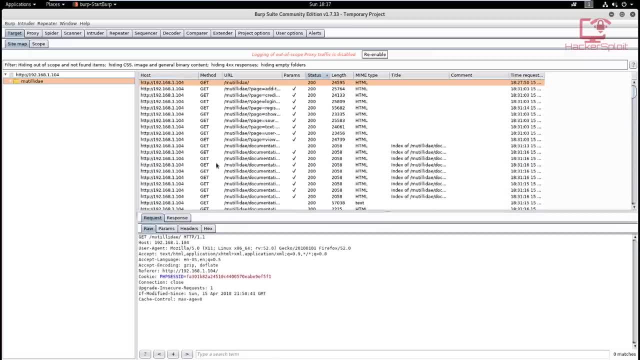 they don't define the scope, And this is what I'm going to do, So I'm going to go ahead and find their scope. they do not know what their target is and they're getting links that are not even relate to the website that they're they're trying to perform the penetration test on Now. 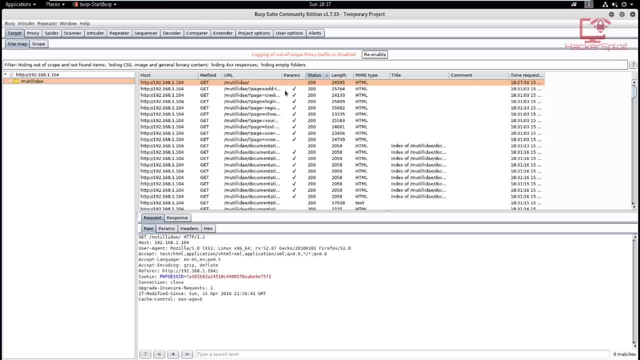 since you know this knowledge. this will help you get a solid foundation And again you can start logging out of skip out of scope proxy traffic when you want. Again, that's very nice that they add that button right over there. Alright, so now you only have the files that you require, or the 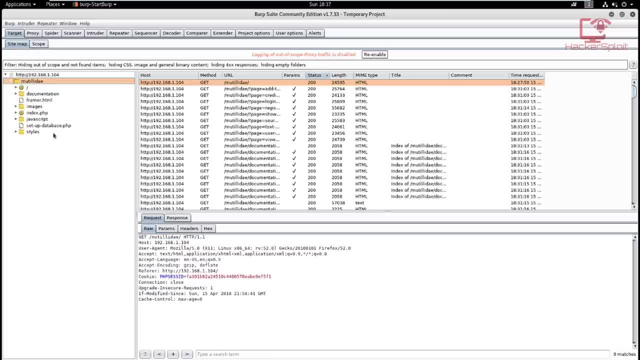 files that you're currently performing the penetration test. only Now I know this. this video was slightly it. there was not a lot of action, But again, it is very important that you get this. in the next video, we'll be looking at how to how to discover hidden files or files in general that you 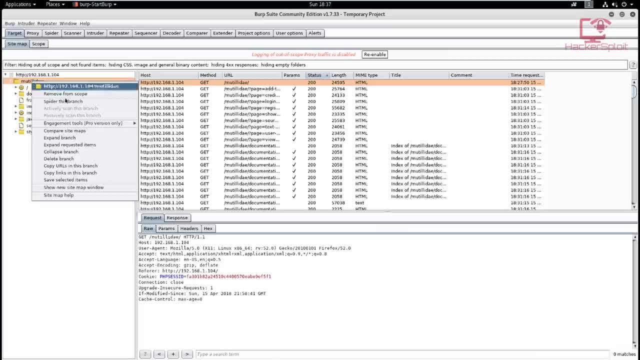 are not supposed to find. Okay, and that can be done by right clicking and going into engagement tools. As you can see, it is defined to the professional version of that suite And we will be going into discover content, where I'll be explaining to you how to find things like the login. 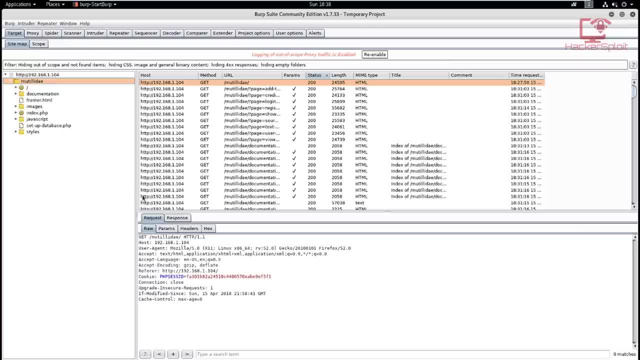 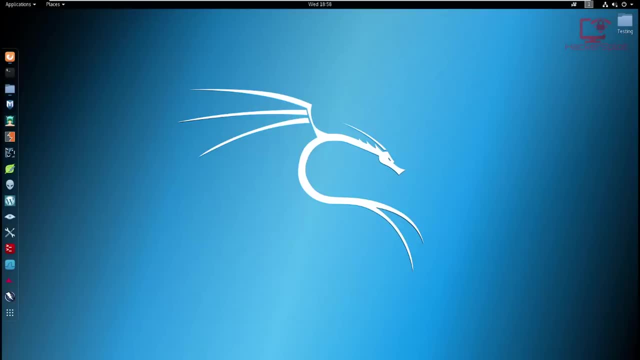 page or the configuration page, some things that web developers, you know, actually just may try to hide them, but if it's actually found, can really exploit the website or can lead to the exploitation of the website. We're going to start looking at how to. 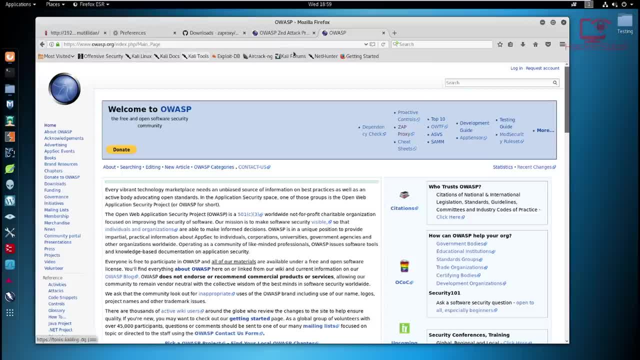 discover hidden files. But before that, I just want to take you through a few things. Alright, so let's start off with what OASP is, or OWASP, Alright. so what does that mean? Well, essentially, what it means, or what it stands for, is the open web. 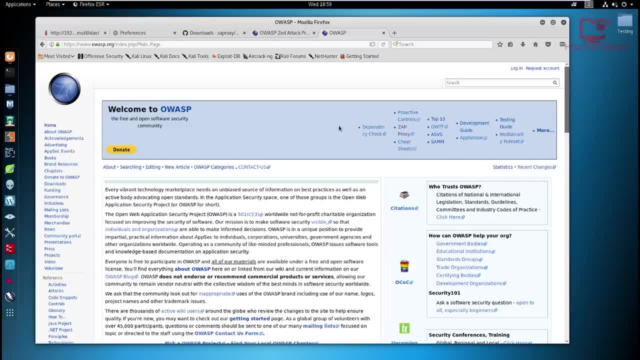 application security project. All right, and its goal? Well, essentially, it is a nonprofit organization whose goal is focused on improving the security of software. All right, so its job is to improve the security of software. Now this project, the OWSP, or the open web application. 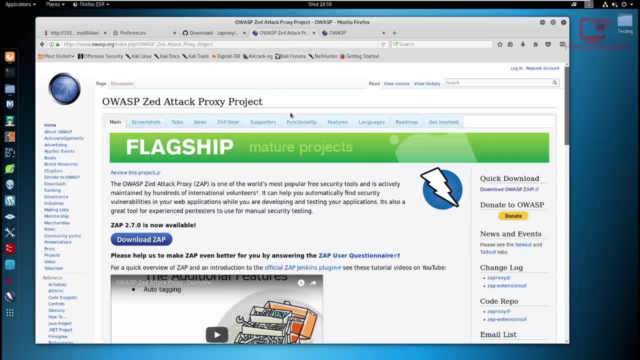 security project created a tool called the Zed attack proxy, or, as you know it, the zap. Many people like calling it zap And I'm sure most of you have heard of it And you might have been there. you might be leaning towards burp suite a little bit more, but I can guarantee you that zap. 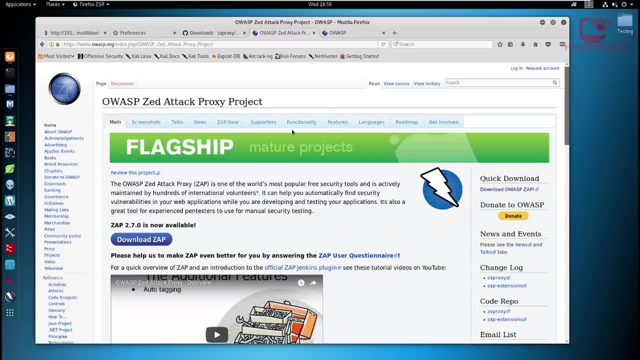 is one of my favorite tools And I use it because, firstly, it's free And for the people, like for the students I teach, I usually tell them to start with zap, Because if you get zap, you'll automatically get burp suite And you only need burp suite when you're moving into an enterprise. 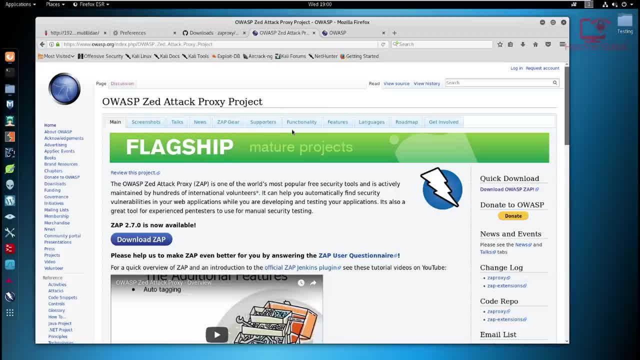 environment where you know, burp suite is the recommended tool And it is the tool that you must use to adhere to to certain rules and ethics. That being said, zap is a fantastic tool. it's absolutely free. as you can see the OWSP Zed attack proxy, which is 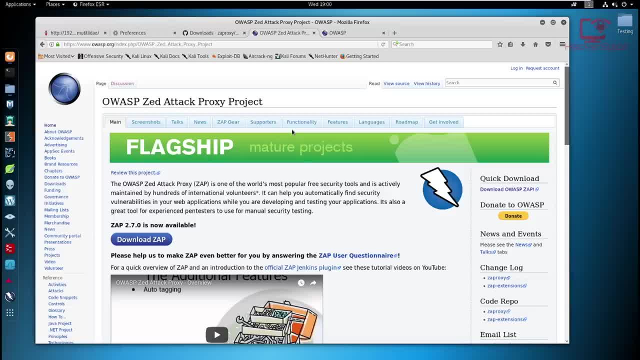 you know, abbreviated as zap, is one of the world's most popular free security tools and is actively maintained by hundreds of international volunteers Alright, so it helps you find security vulnerabilities in your web applications while you're developing and testing applications. So, again, if you're a web application developer, this is also a fantastic tool for you. 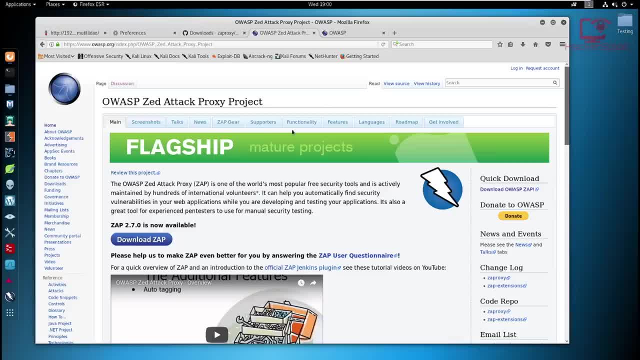 And, as I said, it's going to be a fantastic alternative to to burp suite. All right, that's not to say that burp is bad. burp is more of an enterprise. Enterprise developed software in. as I've mentioned in the in the first video of the series, burp is focused on professionals. Now, 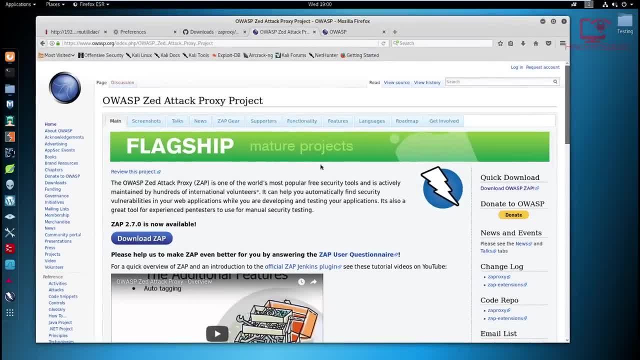 that's not to say that zap isn't, but you'll get the idea Alright. so I'm going to be making a separate video on installing zap And I'm going to make a video on how to get accustomed to the interface, because it is slightly different And the language or English used for the interface is. 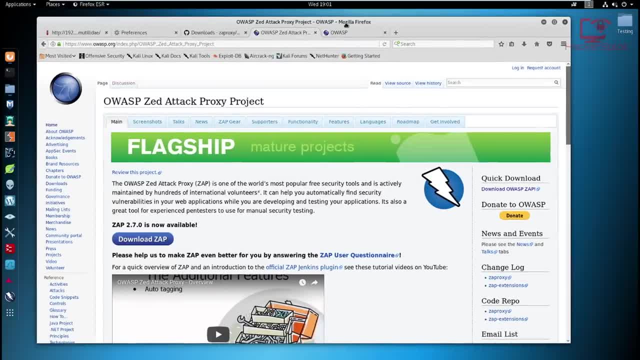 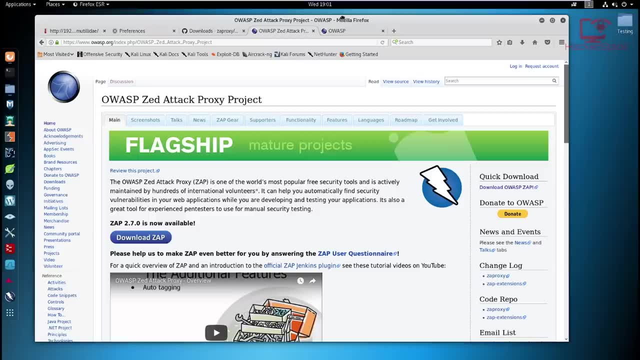 different, But it is quite different. So, again, getting used to it was also something that is quite helpful, because we'll be needing some of the enterprise features and only a tool like zap will be a great alternative. However, if you do have burp suite Pro, go ahead it'll. it'll just be. 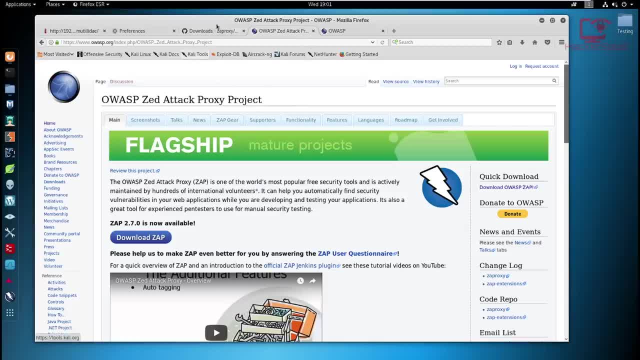 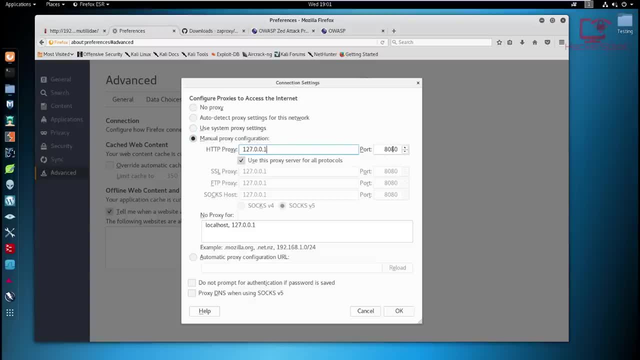 the same thing. As I mentioned in the previous video, it's really very easy to to follow up where we left. Okay, that being said, it runs on the same network proxy. it runs on the localhost, So make sure you're running it on the localhost. 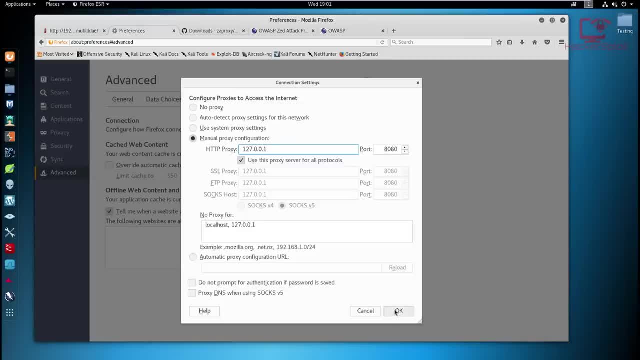 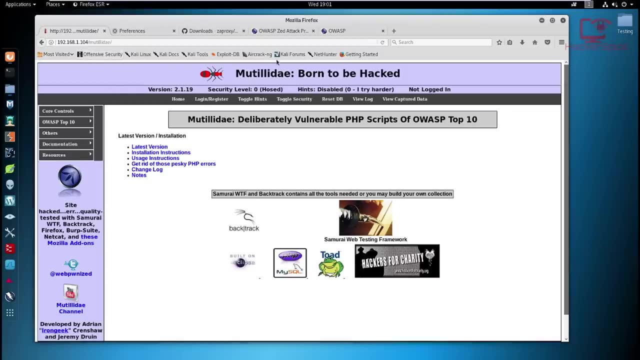 On port 8080.. I'll be showing you how to change the port if you so feel you want to. That's also another great thing about as a zap is it allows you to change the proxies. So I have motility opened up here and it is again running on my meta splitter ball to virtual machine and it's running. 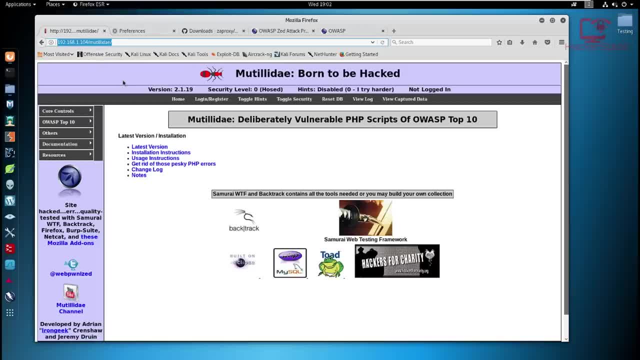 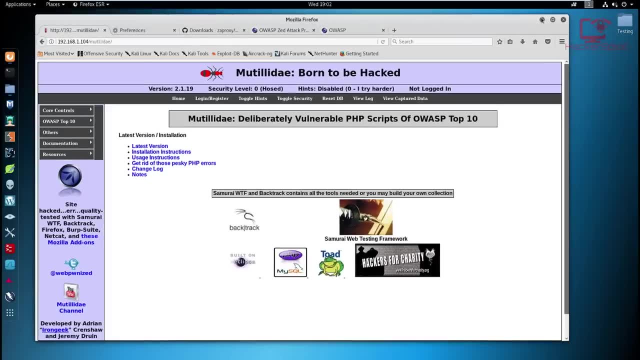 on the IP address. my local IP address: 192.1, 68.1, point 104.. As you can see, motility Alright, so that's working perfectly. So let me just leave those other tabs open, because again, there's no, there's no real harm, Okay. 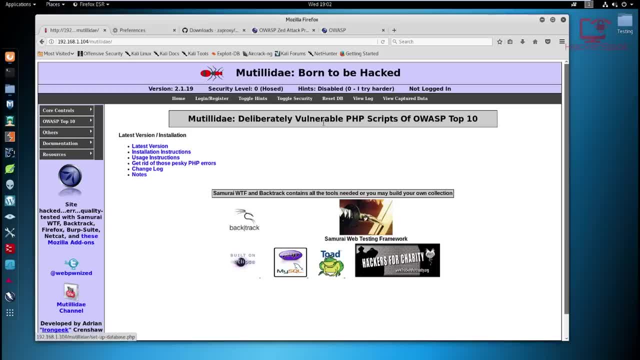 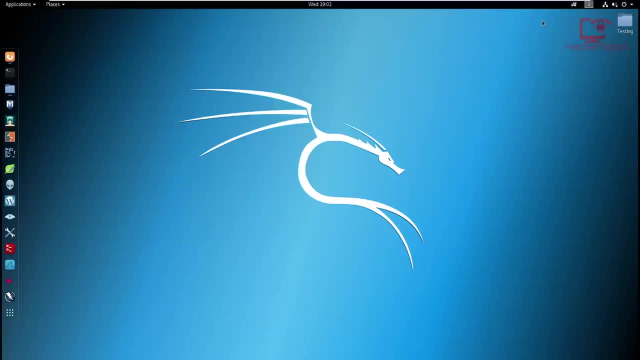 so, again, you can configure the material day security level if that's what you want. you know to do to make things harder. But I'm just going to be showing you the focus of this video, which is how to find hidden files. Now you might be asking: why do we need to find hidden files? Or why do we? 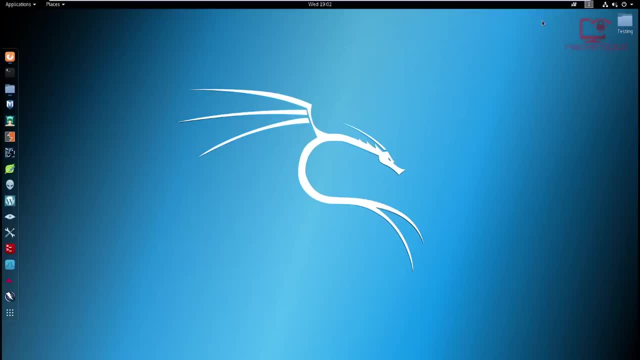 need to discover these hidden files or hidden files. Firstly, are the files like admin login pages, you know, maybe a robotstxt, But that's not really something that's hidden nowadays. it could be a txt containing maybe usernames. you know something really weird, or you know- pardon my English, or 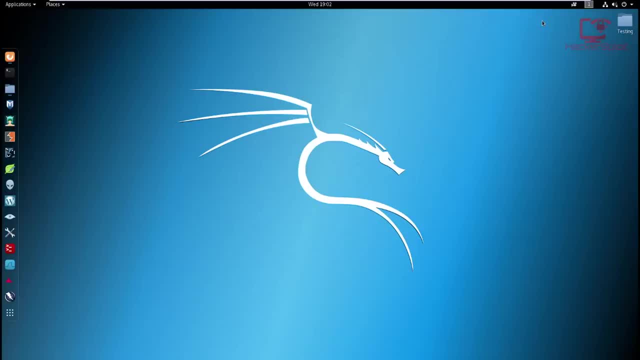 pardon my language, something dumb that the web developers left behind or, you know, just not configured correctly, And you'll see what I mean in a few seconds. Alright, so again, these are the files that are hidden, and you will not find them after spidering your web application or website. 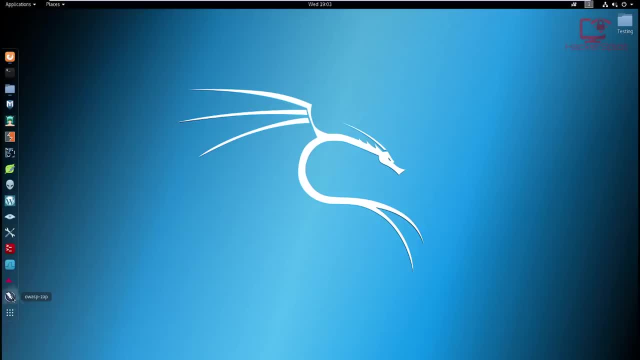 Alright, so let's get started with zap. As you can see, I have the logo right here on my it's added to my favorites. Let me just launch it. Give it a few seconds and it should start up. there. we are the zap. give it a few seconds again. 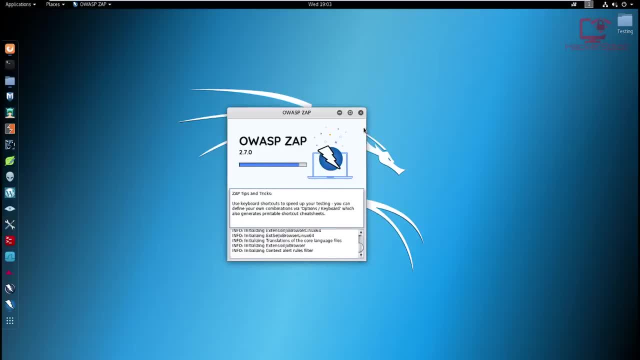 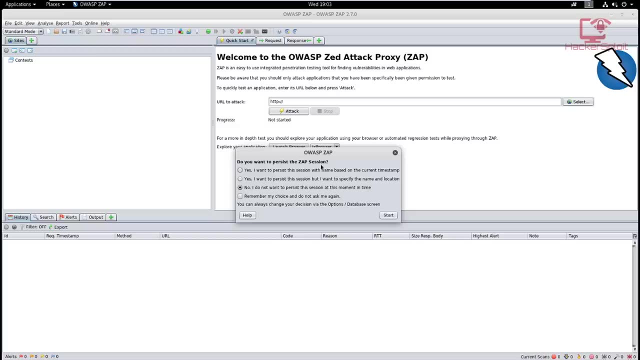 and make sure you update it. usually, the updates for the modules very, very regularly, So make sure you update them to the latest version, as they improve the speed and so on and so forth. Alright, so it's going to prompt you here. do you want to persist the zap session? That means, do you want to? 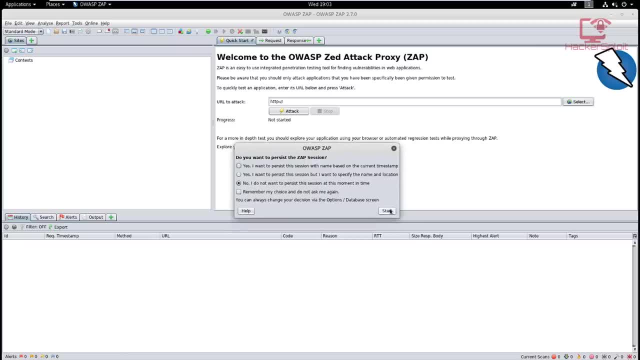 save this app session. I do want- I do not want- to persist at the session at this moment in time, So I'm going to start Again. don't worry if you're not familiar with the interface. I'll be going through it in another video, because it deserves. now you might be a 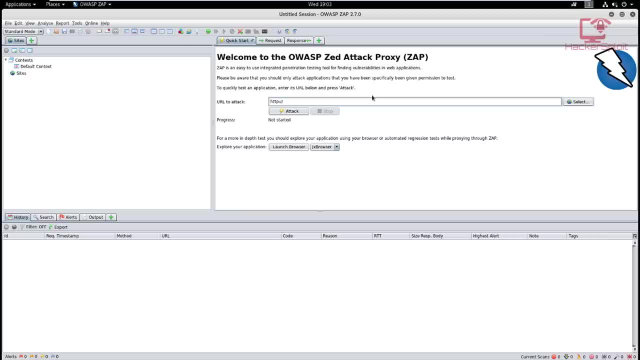 little bit overwhelmed, But do not worry, do not start going to, you know URLs to attack that may seem really really tempting. But again, you know, let's take it nice and easy. So let's talk about the proxy, how to change the proxies. So to do that, you can go into your cog right here, as you can see. 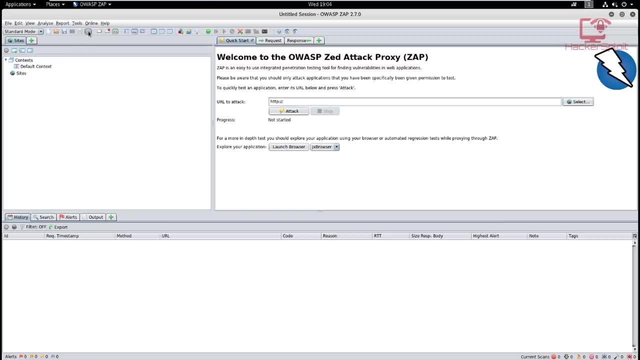 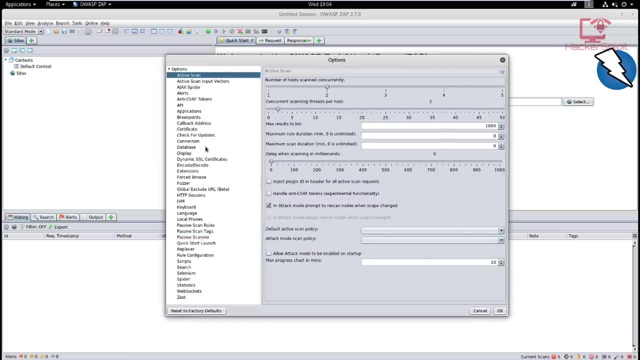 or you can go into tools and go into options, Alright, but I like going into this little cog here And once you press on, click on the cog, let me just enlarge that. you will see that you have this huge menu And again. 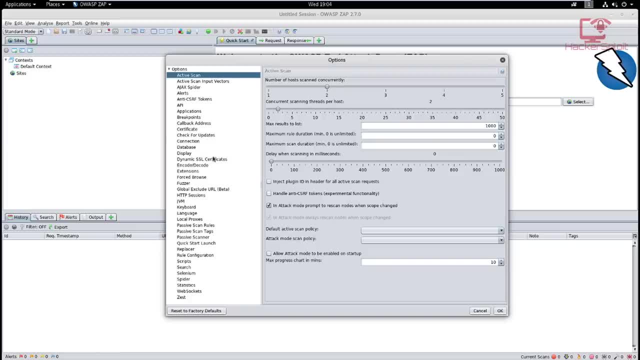 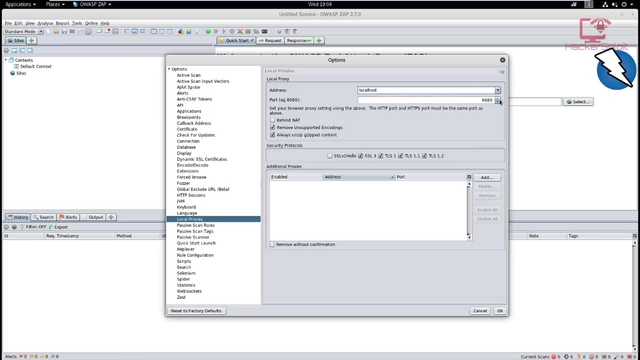 as I said, zap is a really advanced tool And in some cases can totally replace burp suite. Now, looking at the proxies, you want to go for the local proxies. right here It's obviously starting with L, So local proxies. and make sure that the address is hosted on localhost And you can change. 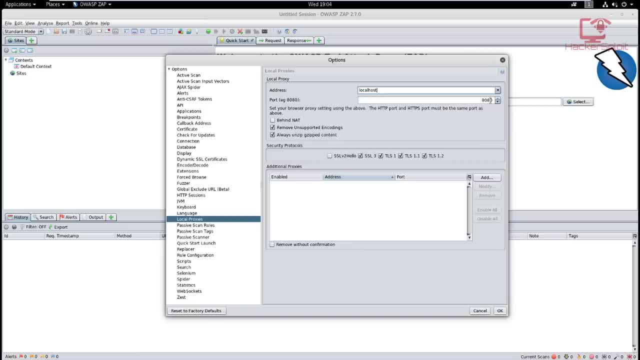 the port if you're using burp, suite and stuff like you're, just if you're using both the applications at the same time, or you're running something on localhost already, So you can change it to something like 8081, whatever you feel is comfortable for you. Okay, so that's how to. 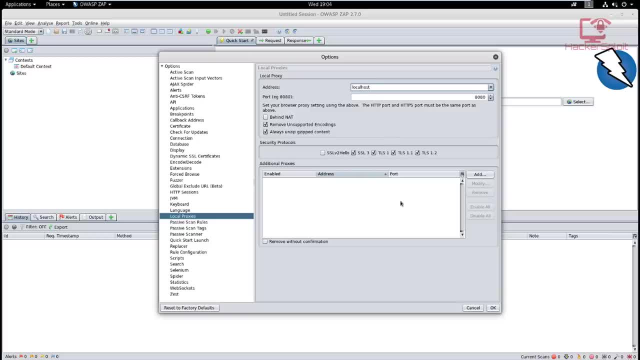 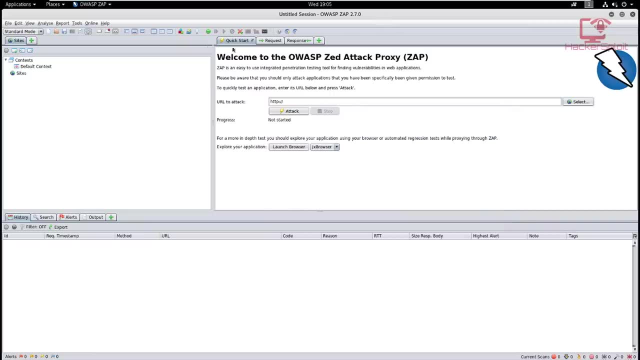 change your proxies And if you're running behind a NAT, you can also check this, and you should be good there. If you don't find that the proxy is working, So just hit OK. All right, Now you see that there's no trail. we're not going to be looking at intercepting right now, But 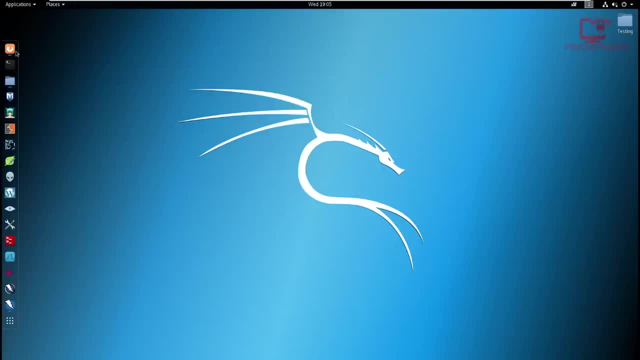 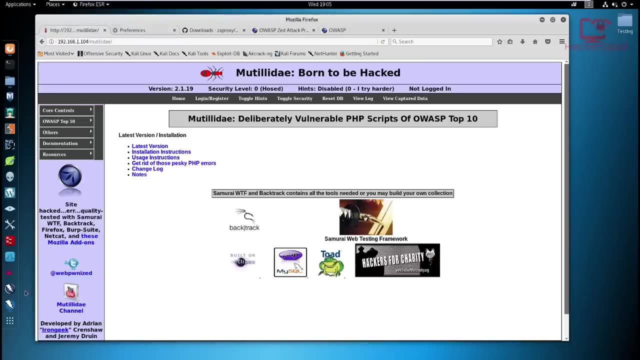 we'll be looking at that in a few, in probably the next videos, the advanced videos with SAP. All right, so let me just reload the motility page And, as you can see, I'm running the proxy. So I'm just going to reload the page And, as you can see, we're not intercepting actively. 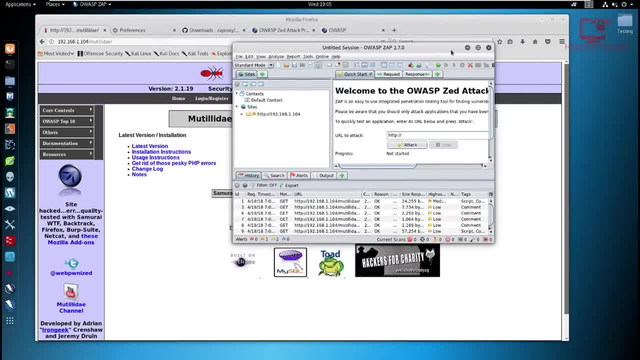 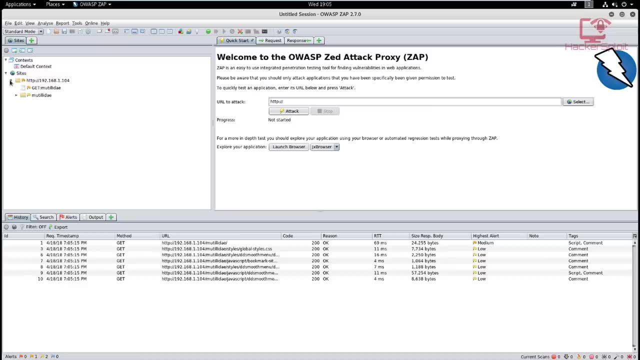 So what's this? Well, we got some files here. Let me just reload the page one more time. And there we are. we are getting some results. So we get the IP 192.168.1.104.. That's the server, And if we 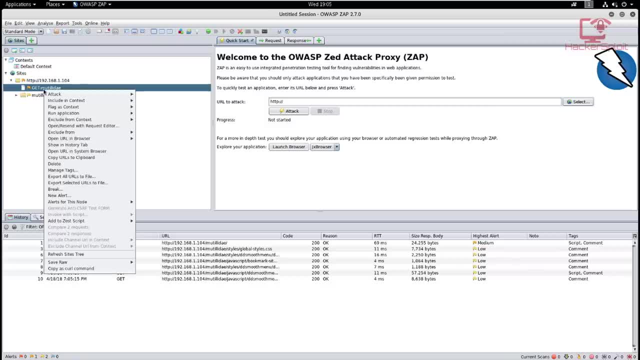 just click on this, we get the IP 192.168.1.104.. And if we just click on this, we get the IP 192.168.1.104.. This drop down here we get the get request. So you can analyze the get request, if that's what you. 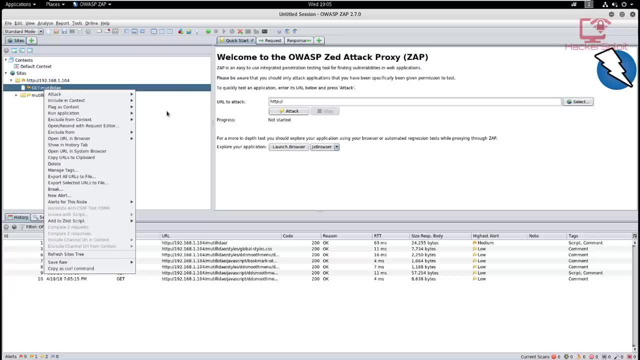 want, So you can right click and then analyze. All right now. we'll not be looking at that right now because I want to focus on finding the, or discovering the hidden files. So what we'll do is we want to click on the motility folder Now, one of the great things I like about SAP. 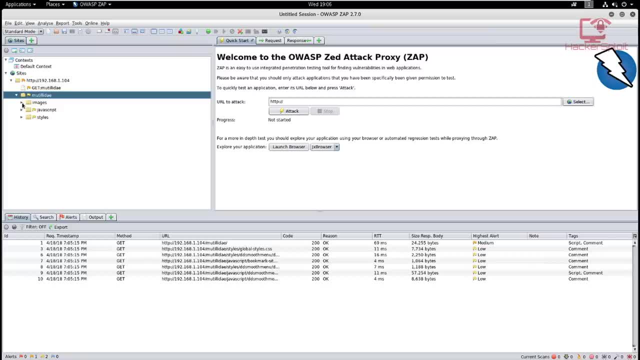 is. it already gives you the file structure or the website structure immediately here. All right, you can see. you have your images folder, which has the images there. you have JavaScript styles and your all the resources in regards to the website that it could find. naturally, All. 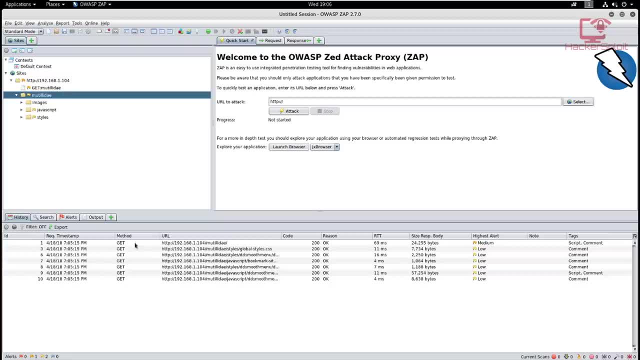 right. So if we, if we just look at the bottom here, you can see that it it's showing you a timestamp with the method, the URL, and it gives you the, the code, which means the pages. In this case, the 200 code means the page was found, you have the reason, you have the RTT, the size. 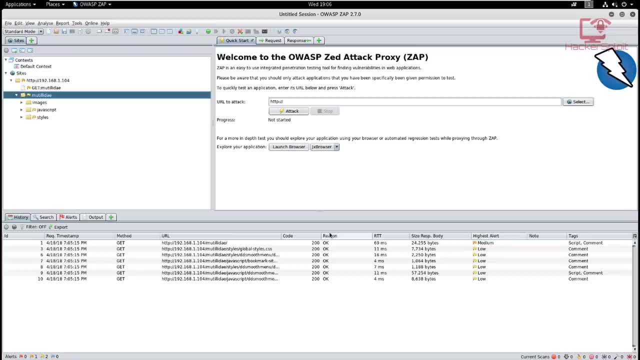 the alert. as you can see, it's telling us we have a high alert here. Now, don't worry about that. Again, these are things that you know will be, will really be tempting, But again, let's take it slow, Alright. so the first thing you want to do, or you need to do, is to right click here and you. 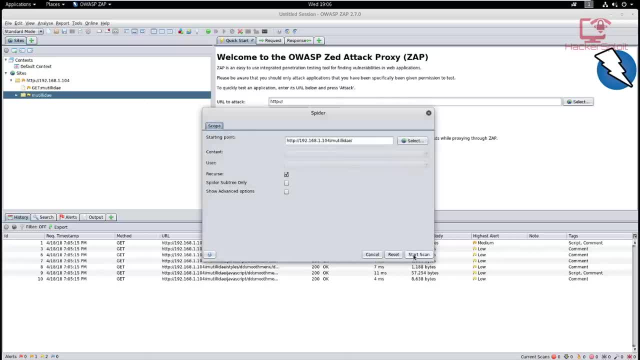 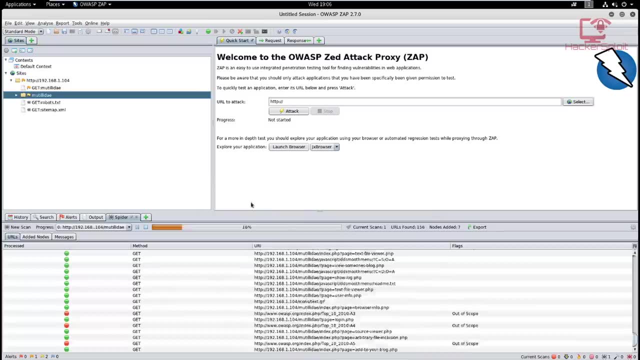 want to go to attack and hit spider- Alright. so we want to spider the website or the web application and start scan. do not touch anything here, just make sure it's using the appropriate server address and just hit scan- Alright. now it's going to spider the entire web application. 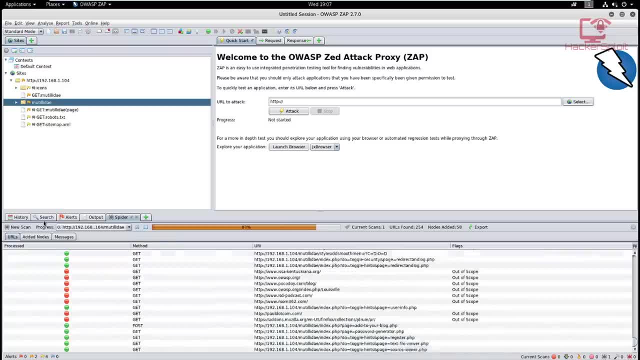 it's going to go to the server and it's going to go to the server and it's going to go to the server and it's going to give you a little progress bar here. you can pause it or stop it, which is also great to see At the bottom. you should have also noticed that you have your tabs. 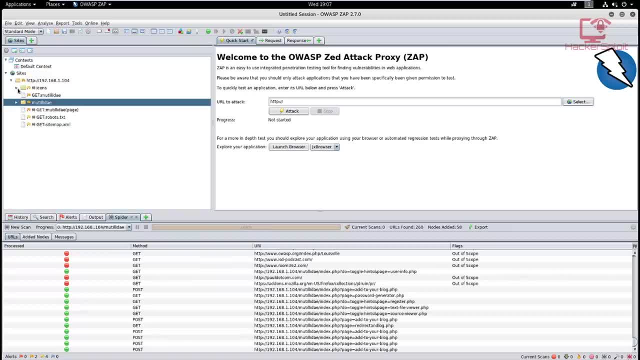 here that work really, really well And, as you can see, the the website now is completely spidered And if we just check all the files that we can find now, you can see that we have some more JavaScript files And essentially what's happened here is the entire site has been has been spidered. 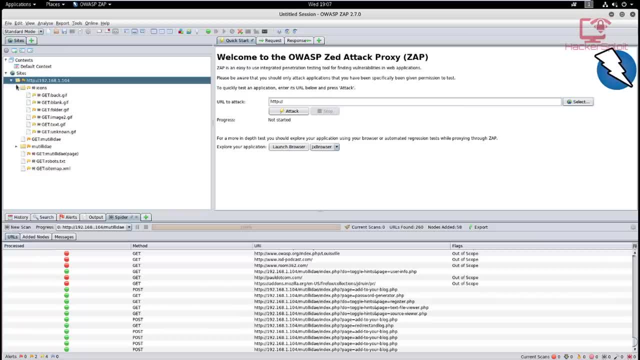 Okay now we already did this with burp And the. you know you've you're probably going to have a lot of problems with that, But anyway, you're probably really bored of this right now. So what we're going to do now is we need to. 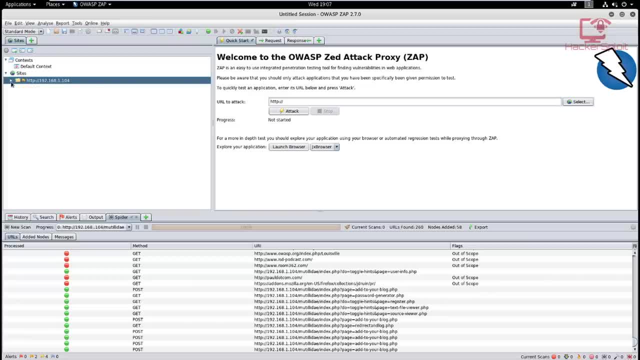 we need to start discovering the hidden content, right? So let me just close all of this up There. we are Fantastic. Now let me just open that up And let's go to Matilda. Oops, my bad, Sorry about. 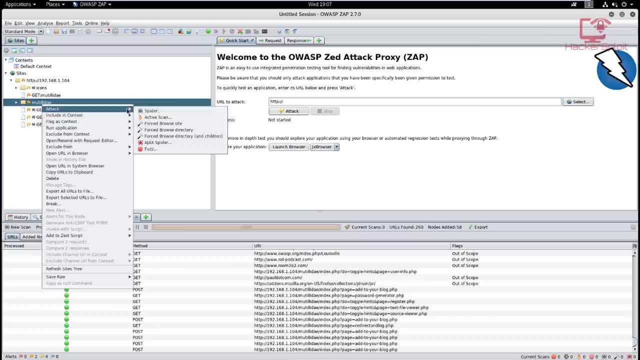 that guys And we want to right click on Matilda day and you want to go to attack and you want to go to forced browse directory And children. that's very important, for browse directory will not display everything. We'll also be looking at fuzzing, but that's for later. Alright, so you want to make sure you hit. 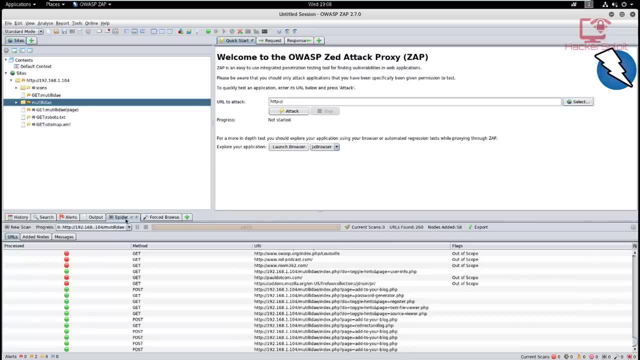 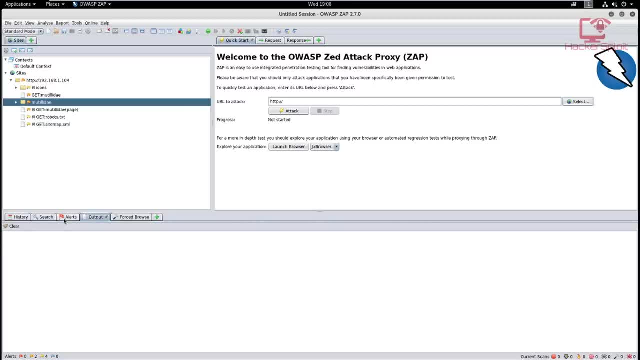 force browse directory. just click on that And it's going to open the up this tab here. So you can see we had the spider tab open, which you can close if you're not using it, which is also great. I really like the management of zap. you then have output for your outputs- alerts, As you can see. 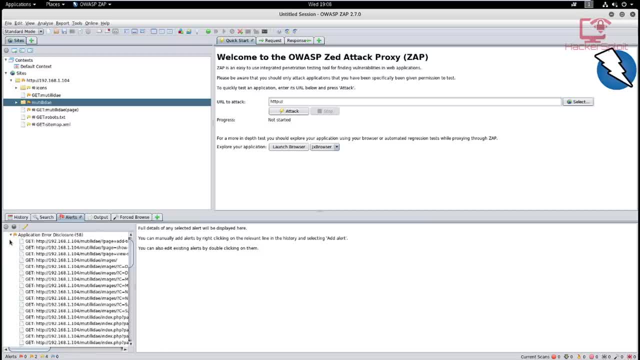 you have some alerts here that will alert you on some potential vulnerabilities. So, for example, application error disclosed. you have some cookies, a no HTTP flag, So again awesome stuff. There We have the get requests are all that good stuff, which is again focused on a different type. 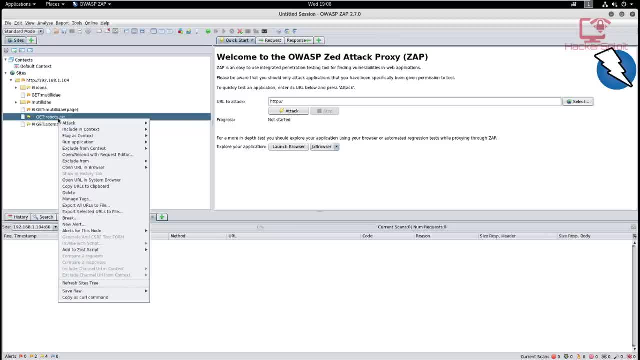 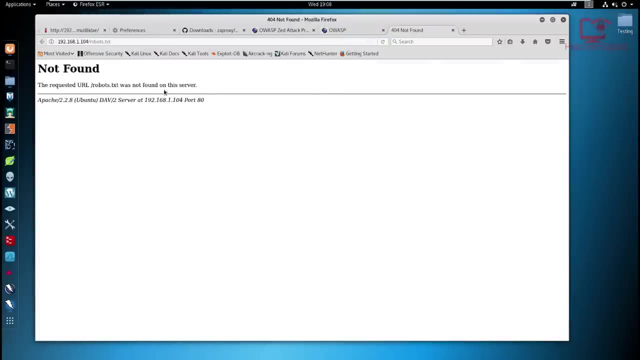 of attack. And, as you can see, by default we've got the robots dot txt here which you can analyze, if you want to, by right clicking and going ahead and doing that, So you can copy the URL to the browser. So, again, copy the URL to clipboard, All right. And if we just try and explore this, let me 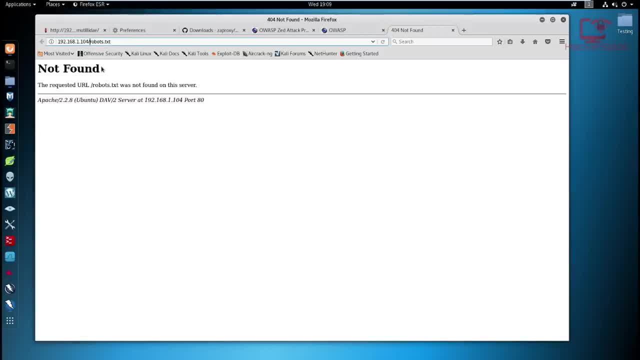 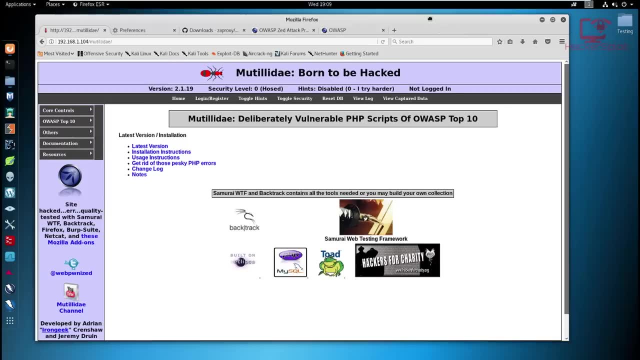 just paste and go here. As you can see, we're for some reason we're not actually getting robots to txt. We use the motility, motility day, or actually you know what. let's not do that right now, Because I. 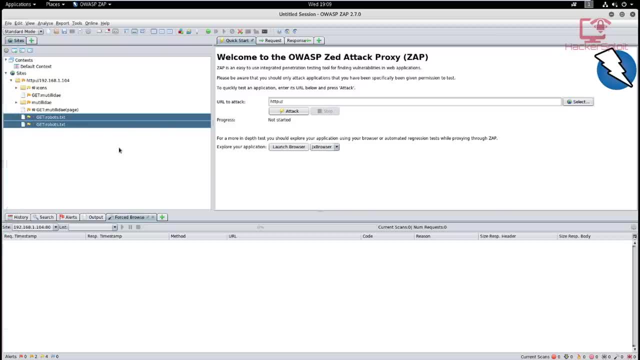 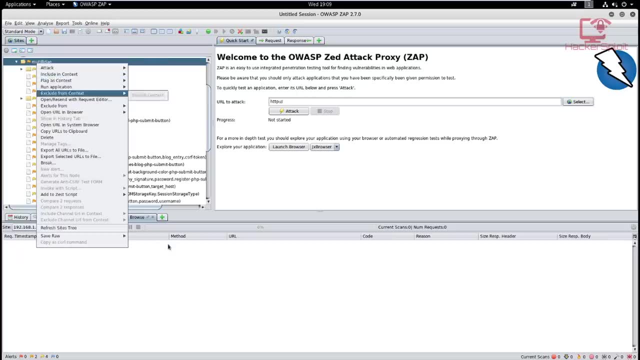 really want to stay on topic here, So I'm just gonna go back into that Again. I always love going off top fourth topic for some reason. Okay, so make sure you click on motility day and you want to right click on it. And now, oh sorry, we already did the forced browse, So right click go. 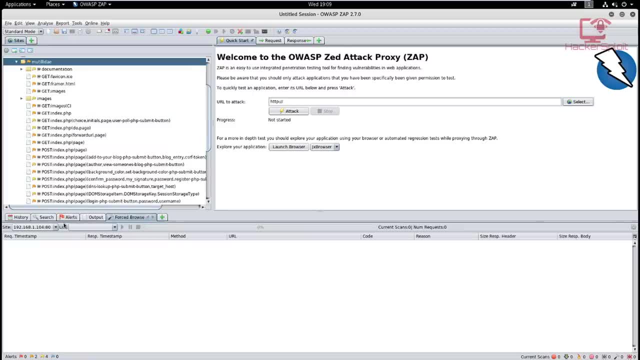 to attack and forced browse directory and children. All right, now it's going to open up this tab here. It's going to make you choose the site. As you can see, you have your site IP here. Now you need to select the default directory list, So it's going to use this list here, this default list that comes. 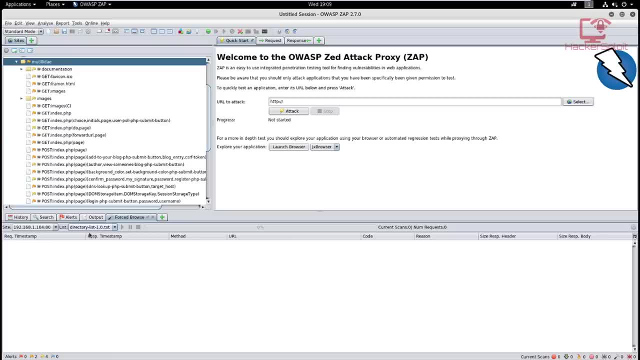 already with zap And now it's going to try and use it in a sort of a brute force way to try and detect the hidden files and folders And once it gets the result, it's going to enumerate them. Okay, so now you want to right click again on it after you've selected the list, and hit attack And 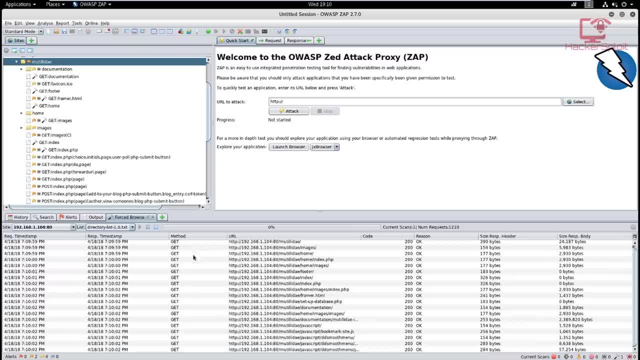 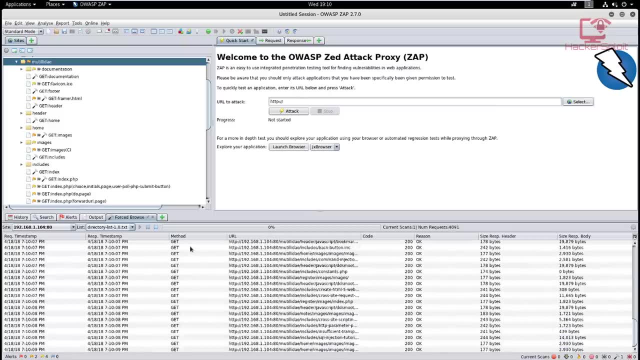 you want to go to force browse, directory and children And once you hit that, it's going to start the process. Now again, this is going to take a long as well- not a long time, depending on this: the the size of the website. if the site is huge, then again it's going to take a while And 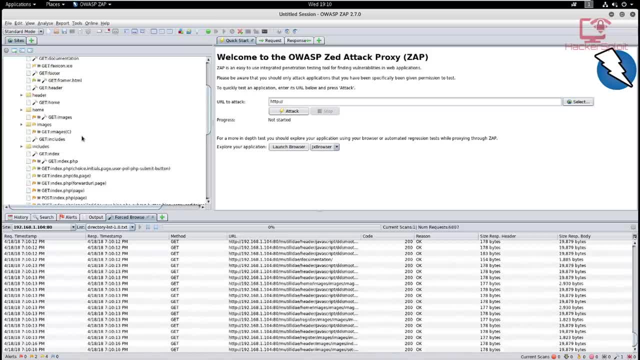 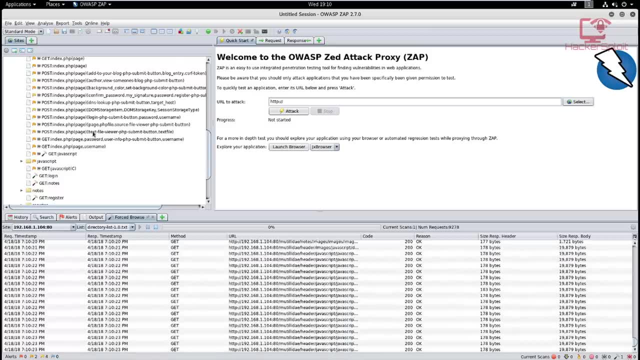 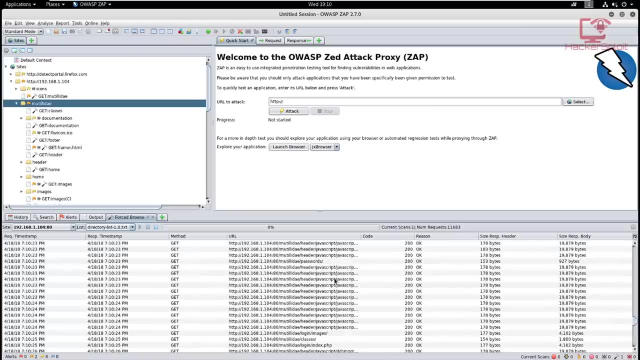 as you can see, immediately, we're getting some, some hidden files. So let's, let's wait for this code to complete, And I know motility day has some very, very interesting files here that I'm sure we'll be happy to get. Alright, so just let it go through this. As you can see, you can check the. 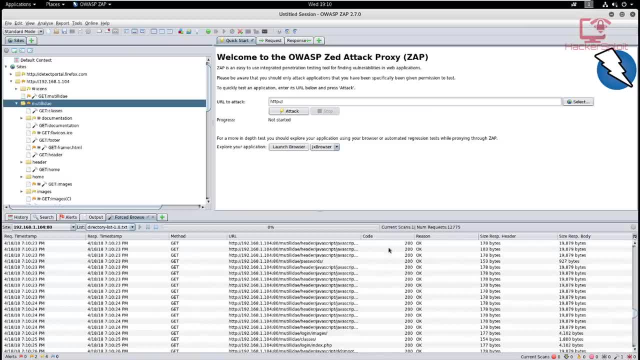 progress as you're going here And again, the, the. if you look at the status code, you can see 200 means the pages were found, So you can just go ahead and look for things that are irregular, And I'm sure we can find something here that we 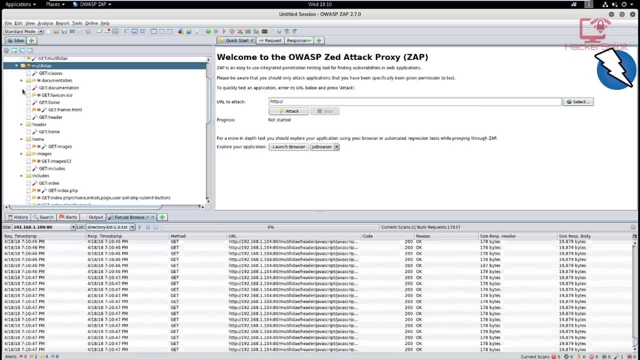 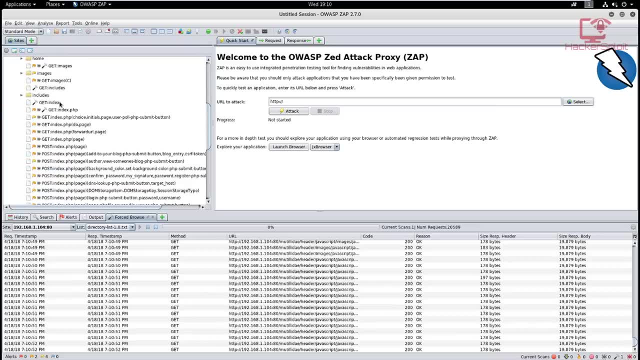 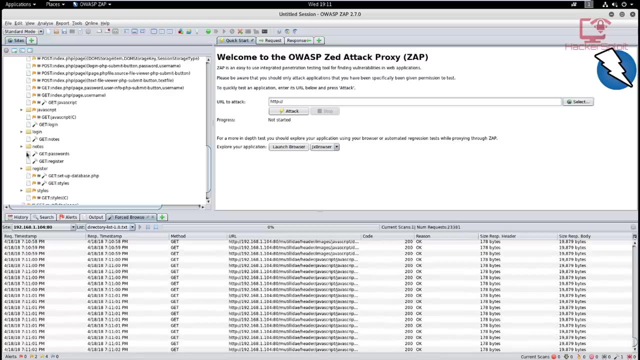 haven't found before. Or you can look at the at the file for the, the website directory here. So motility day, let's see if we can find something that is really really interesting here. So we have the includes, we have the get index dot PHP, the get request story for the index dot. Oh. 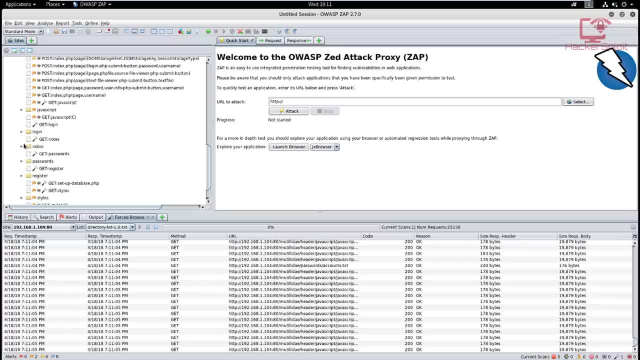 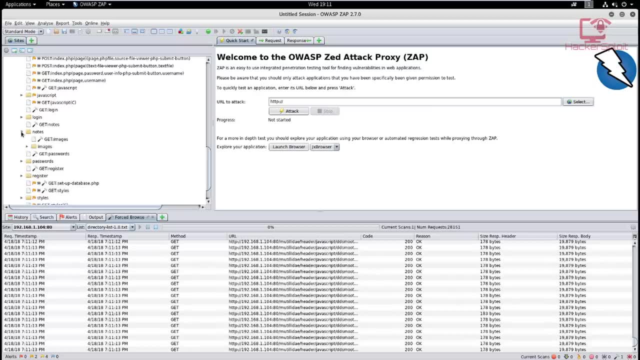 something interesting here. we have a notes folder. Aha, now we're talking. now this is where stuff gets really exciting. Alright, so we have whoops. where did it go? There we are So in notes. we have some very interesting files in notes, So we have a get passwords. Now what happens? What's? 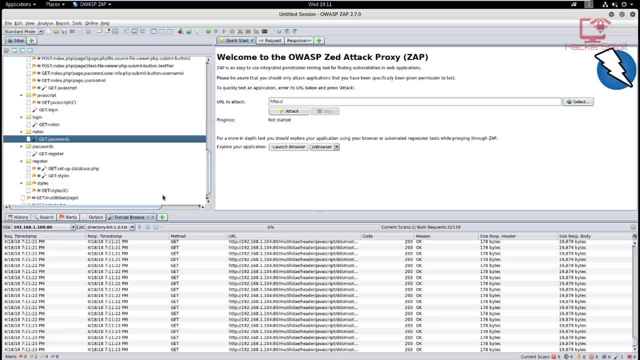 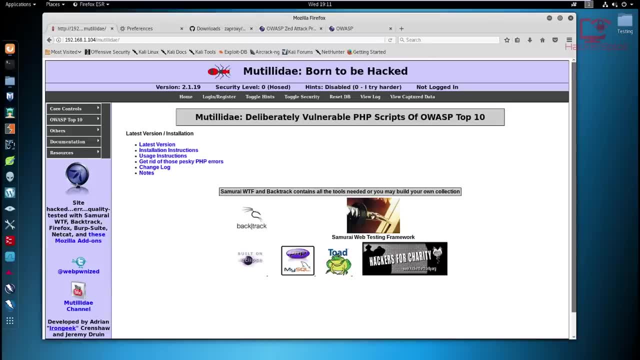 this about, Alright. so what if? what what if we just open this URL in the browser? Alright, so let me just try and open that in Firefox. I just want to see what it's going to be all about. So hopefully it's going to open up in my browser. If it's not, I'll have to copy the URL, probably because I 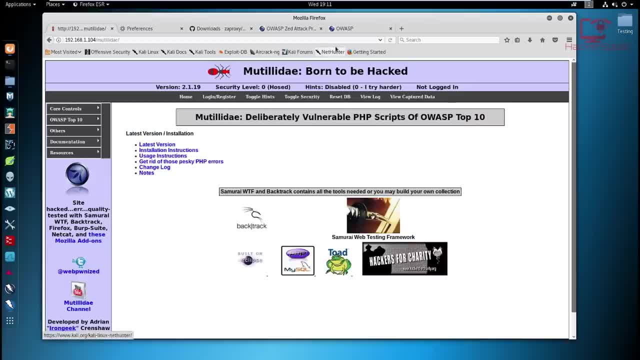 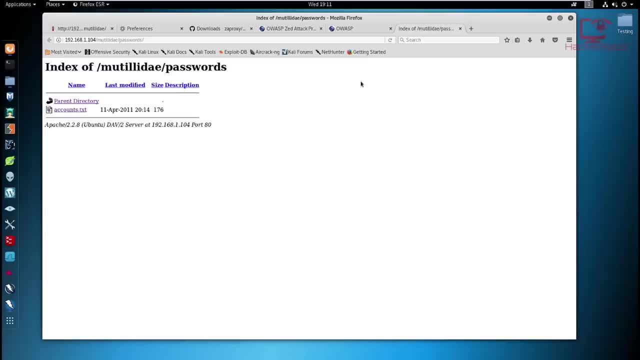 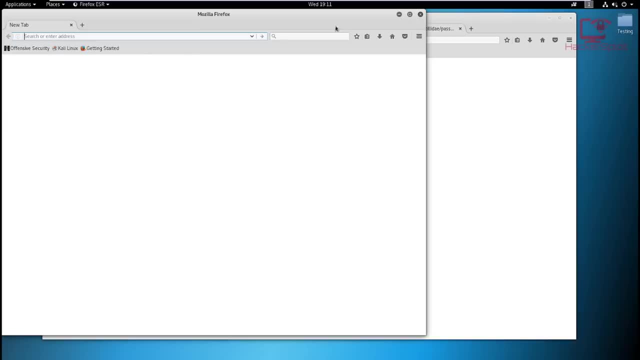 haven't set any any default, Alright, so copy URLs to clipboard And let me just paste that in there. paste and go There. we are motility and passwords: Alright, so you can see that this folder or this file was hidden And we have an interesting txt file here which, again, is quite 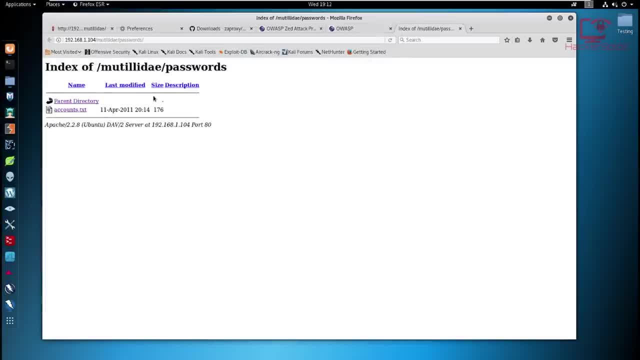 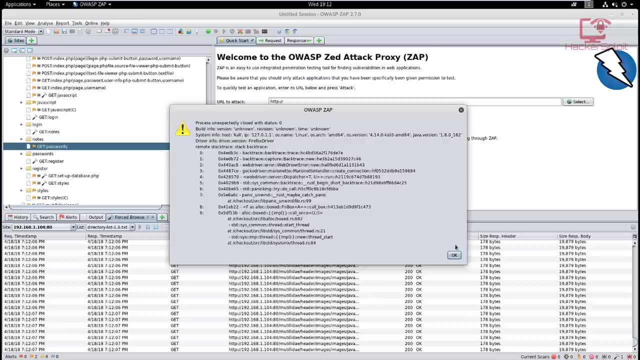 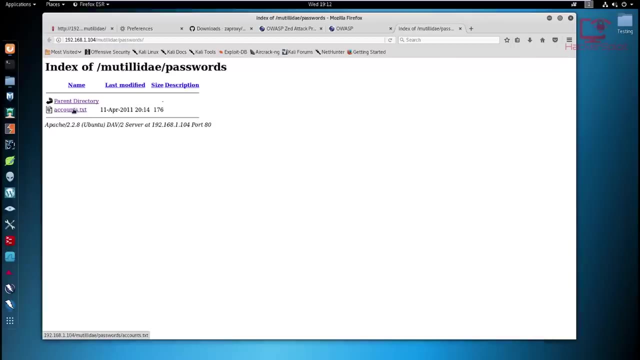 scary to go. we did open Firefox. Well, don't, doesn't look like we need that instance. So as, getting back to the topic here, for some reason process unexpectedly closed with Alright, so that looks like we have a Java error there, So let me just go back over here. So again, we found an. 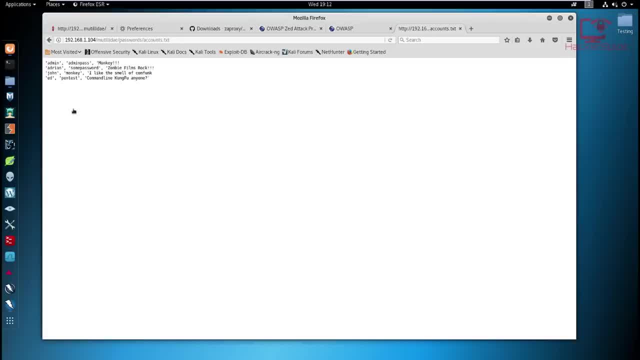 accounts dot txt file. what could that be carrying? Let's click on that, Oh boy. So again we have accounts here, And well, I'm pretty sure you wouldn't know what this means. This is just bad practice from the website. 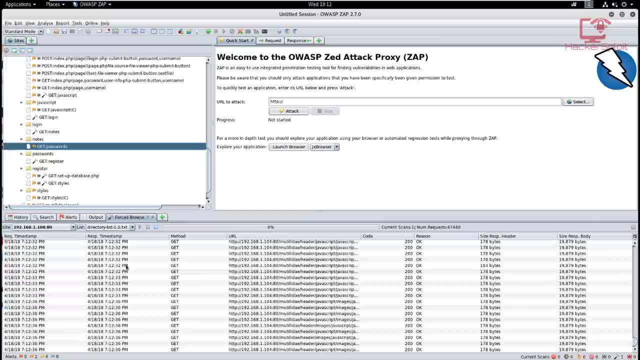 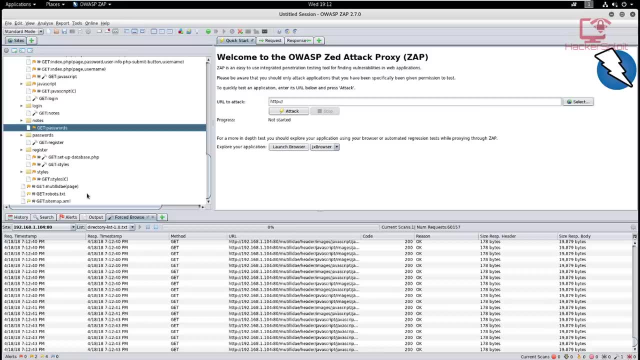 developer where he wrote notes And essentially these are the accounts. Now let's see what else we can find. Let's see accounts. nothing interesting in accounts because we now have the account, So that makes our brute force much easier. You then have let's see if we can find any passwords. if 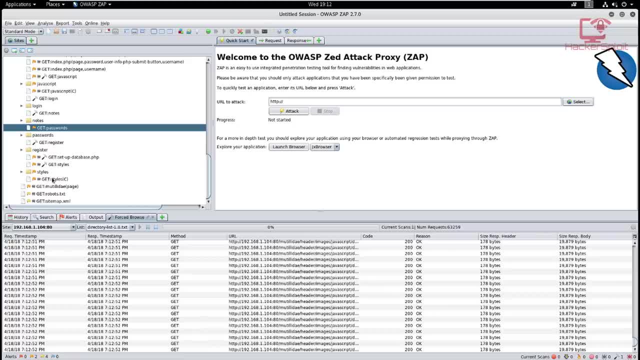 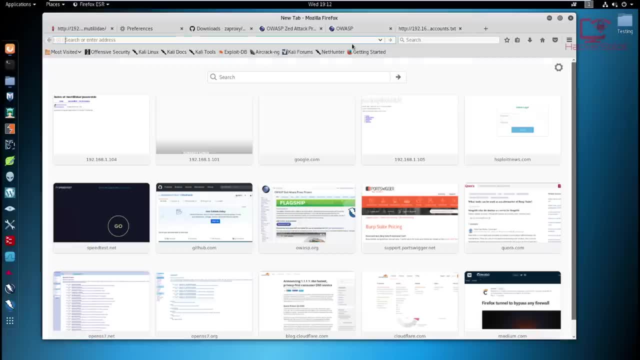 they were ever saved here. I'm pretty sure they're not, But we can look for some interesting files. Yeah, that can be really interesting. You can look at the sitemap if you want to. So let's also copy that. Let's see if it gives us access to the sitemap Also. very, very. 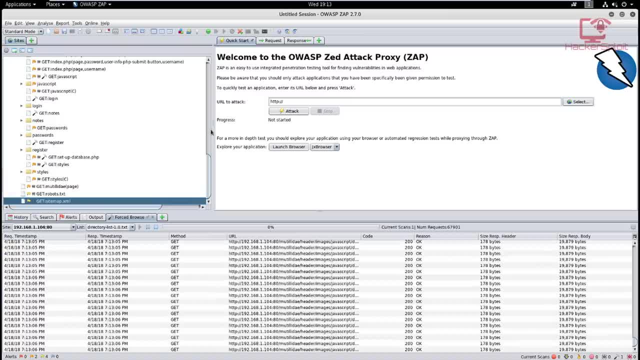 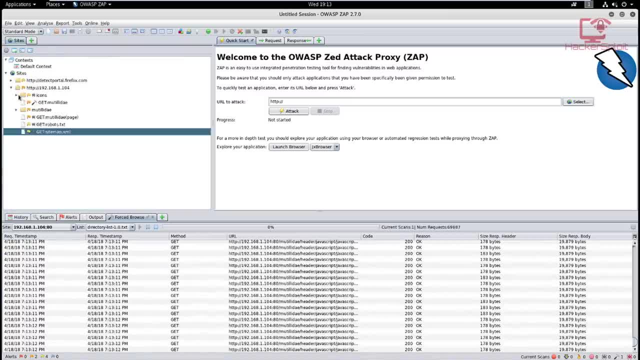 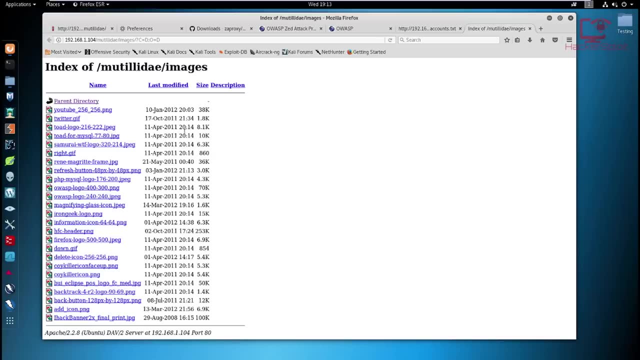 process it. All right, let's look for some other files here. Let me just open that motility again. So we have the get images. Let's see if we run the get images. Let's see what images we can get. Again, I'm going pretty amateurish on this. I'm just clicking on everything, But I'm just trying. 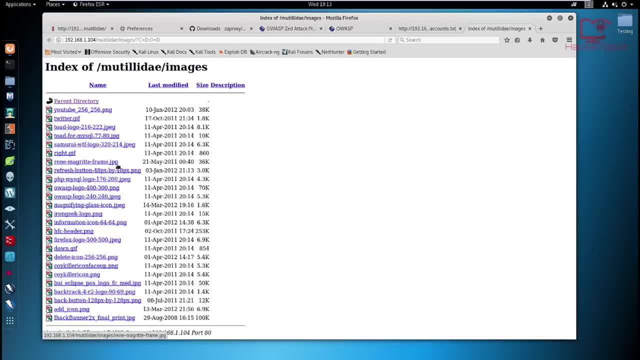 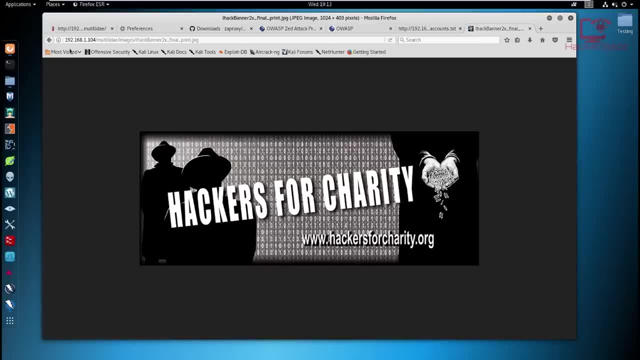 to show you the amount of files that you can find, As you can see immediately. you can find the refresh button. you know all the different things that you can find, So let's go ahead. and all the icons related to the website. You have the I hack banner. Oh yeah, hackers for charity. 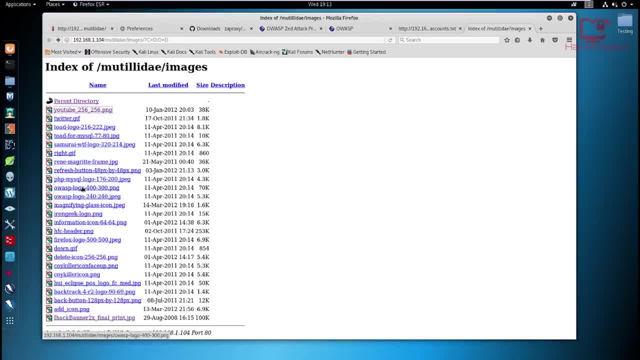 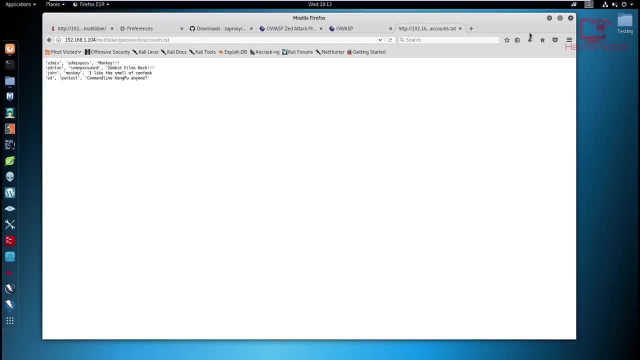 man. So I'm talking about YouTube. Oh my God, what an old logo that is. You have the OWSP logo- pretty cool, pretty cool, And yeah, so you get the idea. So this is how you actually go to website. 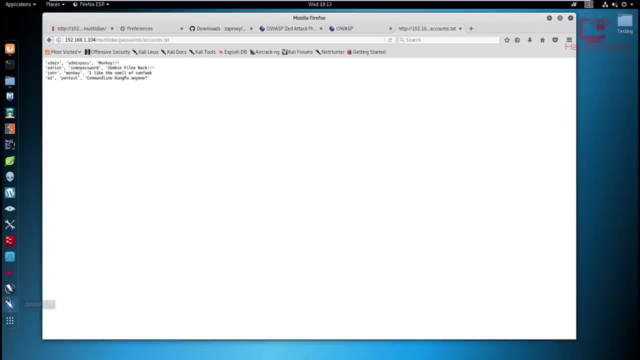 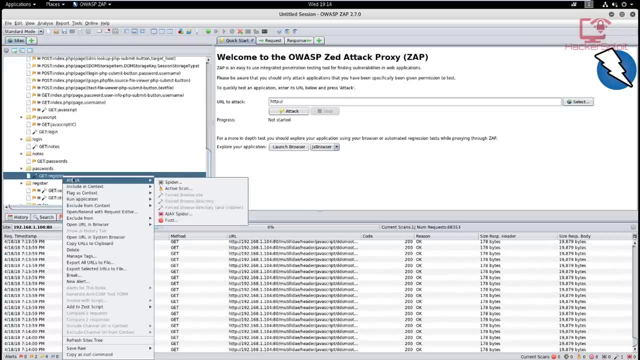 and find files that could contain, you know, stuff that is quite interesting, to be honest. So let's see what else we can find. I'm just going to go through one more resource here that we've found. Oh, we have to get register. Oh, now that's what I'm talking about. Copy URL to clipboard. 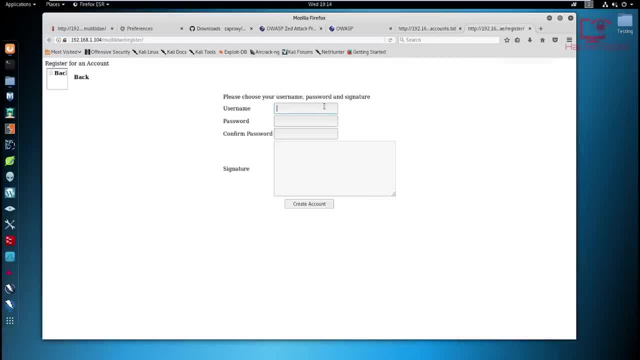 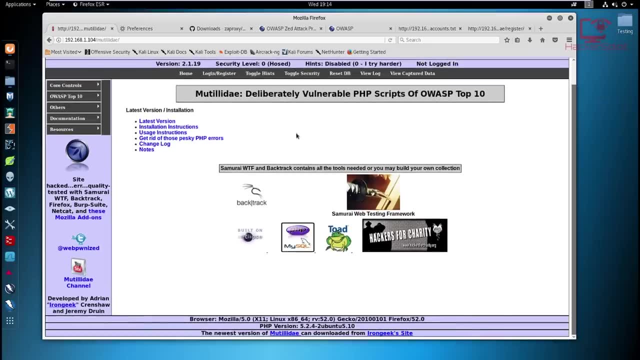 It's actually. this is actually quite fun. This is why bug bounty hunting is Oh yeah. Now this is what I'm told: we can actually register. We can actually register ourselves on the website. Now again, looking at the website from here, it doesn't look like we can. can we even register? 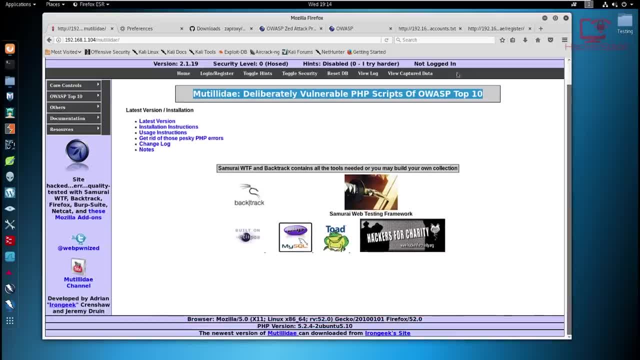 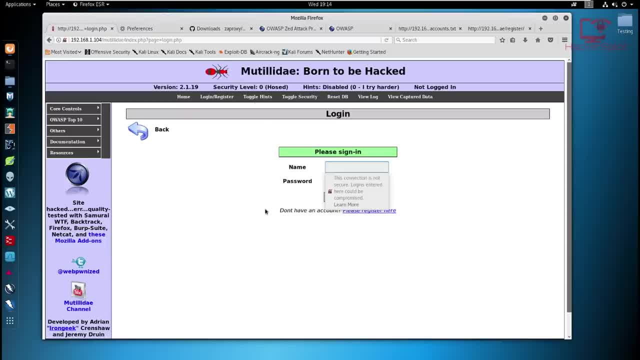 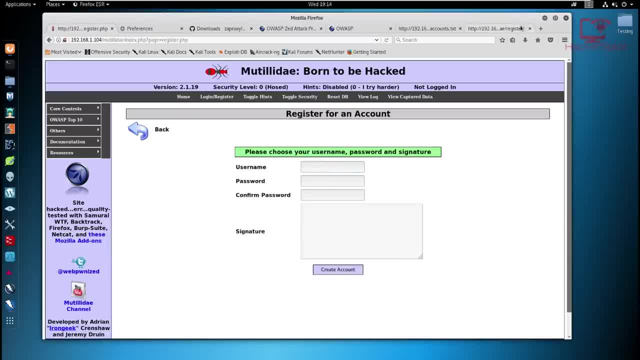 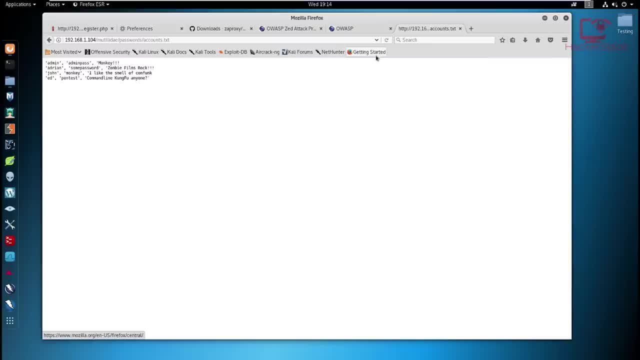 render and register. Sorry about that. We can register there. So yes, it is the register, It does exist. So that wasn't actually a hidden, but it was hidden. It was hidden to the woman when we spied at the website. So that means indeed it was hidden for obvious reasons: because the brute 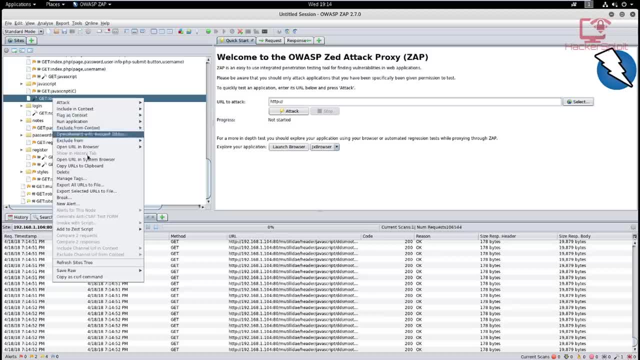 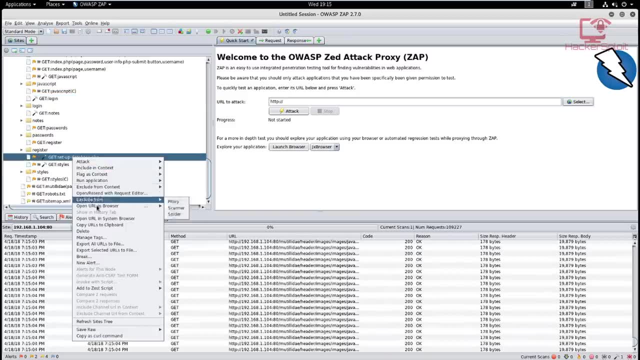 force. for example, if you find the lock in which is again here and again if this is hidden, you can imagine the the damage that you can do. So, again, you can log in from their setup database. Now that's interesting for some reason. 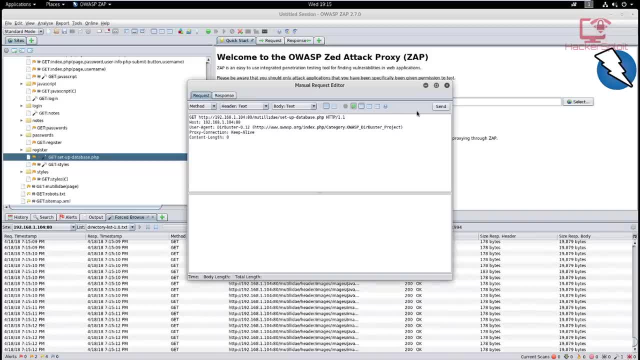 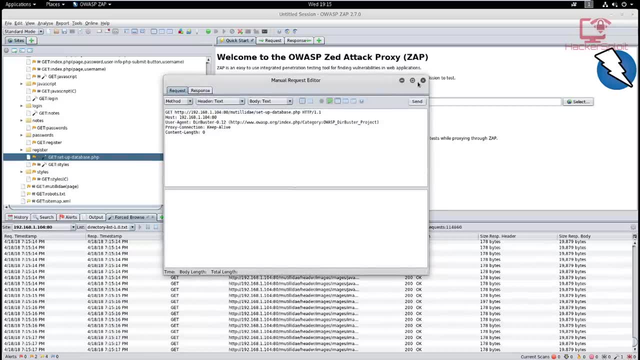 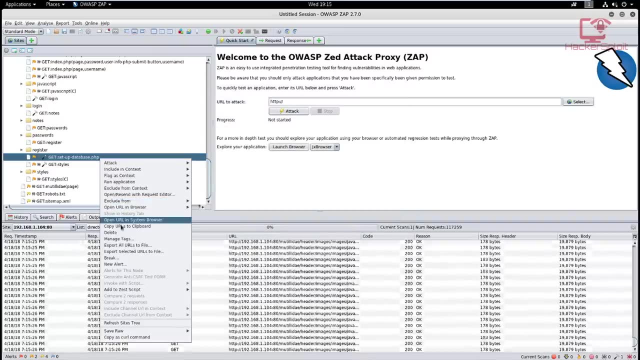 you're letting me copy, Alright. so looks like we got set up database here. So, yeah, we can. Okay, I do not want to manually edit the request. No, I do not want to manually edit the request. For some reason, my keyboard is being pressed here. Well, that's weird man. Copy URLs to clipboard, Alright. 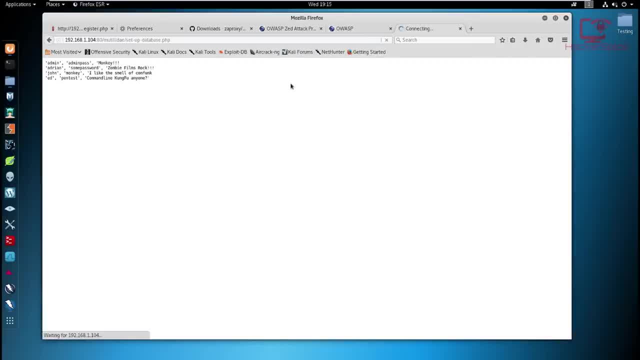 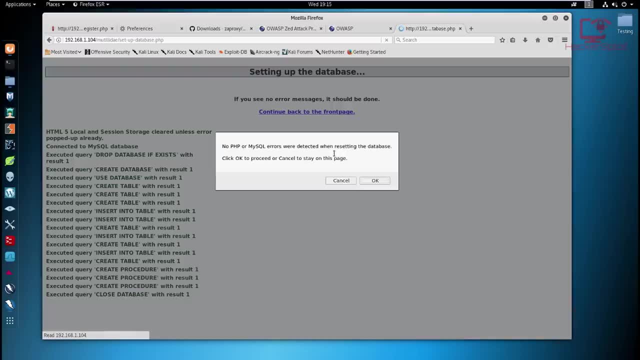 sorry about that. My spacebar was being mashed on by my tablet in front of me, Right, So let me just there we are. So no PHP MySQL errors were resetting, So essentially reset the database and you can see the damage that this. 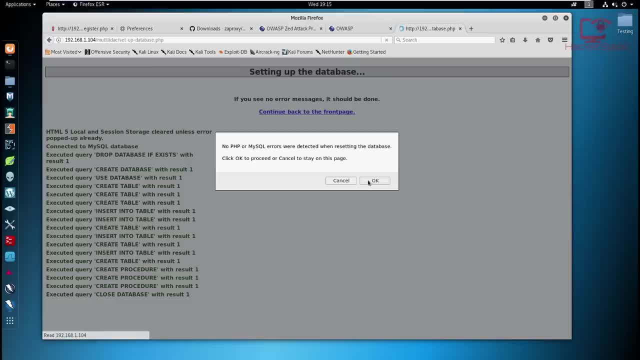 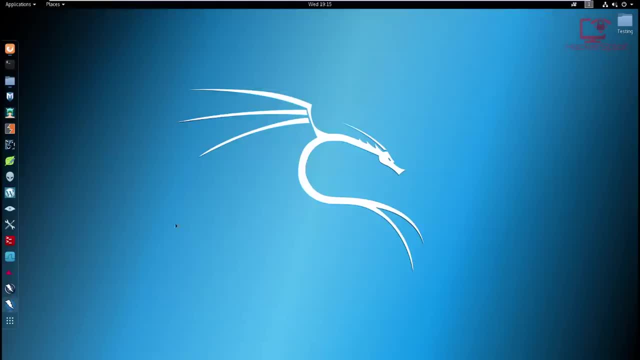 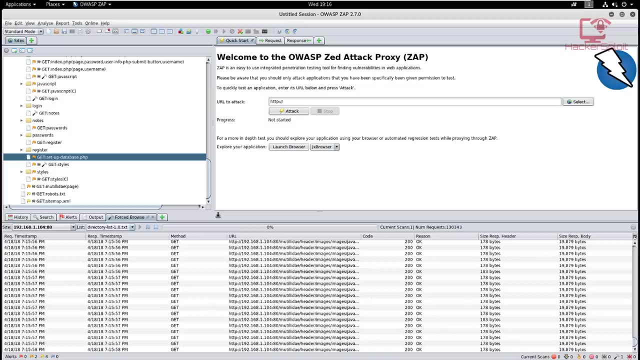 can do. So, again, that is some good stuff that you can have fun with. When, especially with motility, you can increase the security and find what other files you can you can find, you know, with zap. Again, zap is a fantastic alternative that you can use If you know, if you're not ready to invest in. 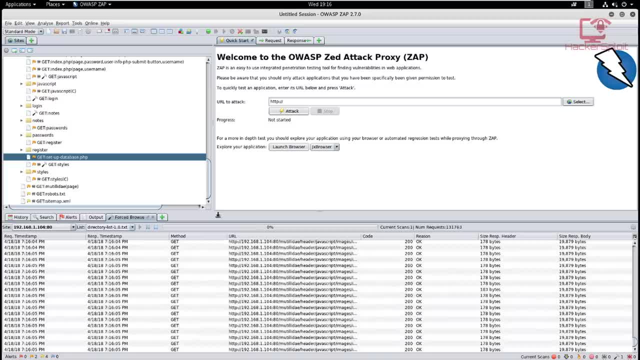 burp suite. that's totally fine. I used zap for I think about three years, especially since 2014.. I think I used it in till about I think 2016 or 17. I'm not too sure, And it worked great for me. 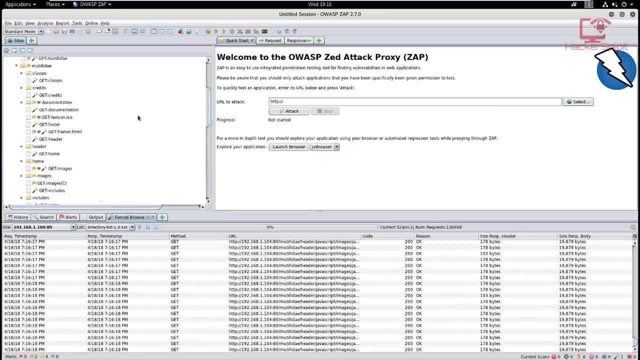 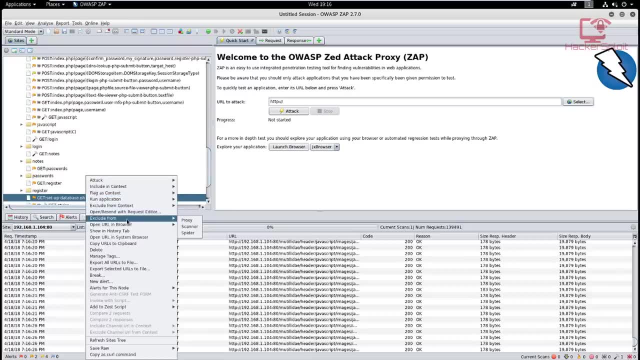 I really enjoyed it And I'm just getting back to, I'm just remembering how all the tools used to work. It was actually quite a user intuitive interface, Because I just remember, right clicking means you can copy the URL, you can inspect it, you can change the request, you can attack all. 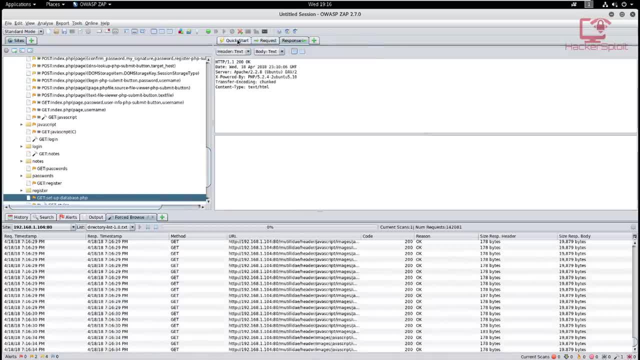 that good stuff And you know it's not that easy, But it's not that easy. But it's not that easy And it's sorted out really really well. All right, and you can look at the requests here, you can. 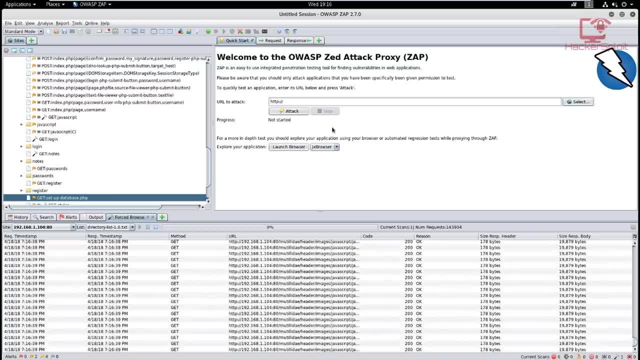 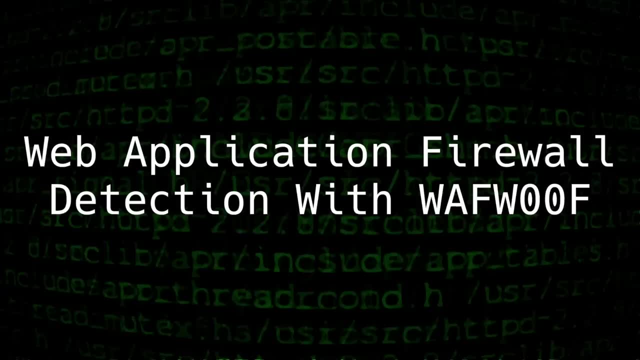 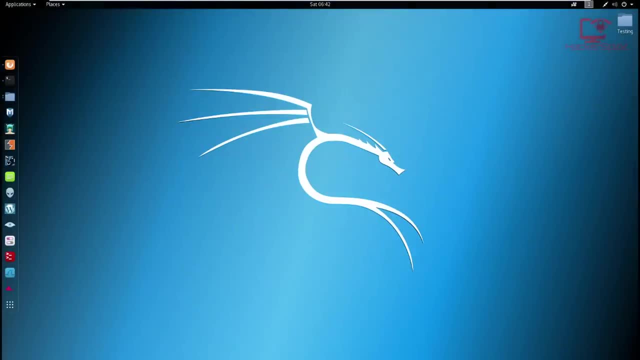 change them to whatever you want and then send them. you can intercept them. See, it essentially does whatever, but a suite does. We're going to be looking at web application firewalls, or wafts as they're called Now. this may be a new term for you And do not worry, this is now. 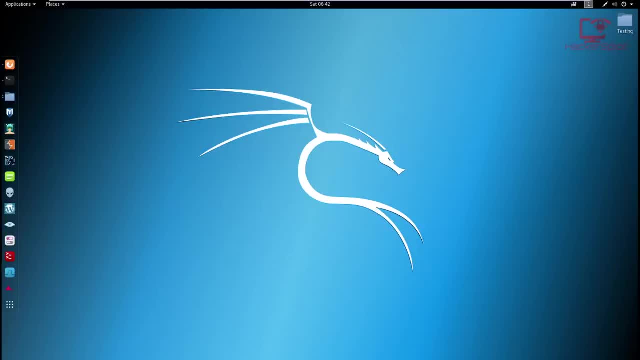 when we move into a more professional level- And again this is what I'm I've been talking about- is most people out there, or most documented documentation out there, won't cover the most important industry standards. you know now when I'm talking about web application firewalls. 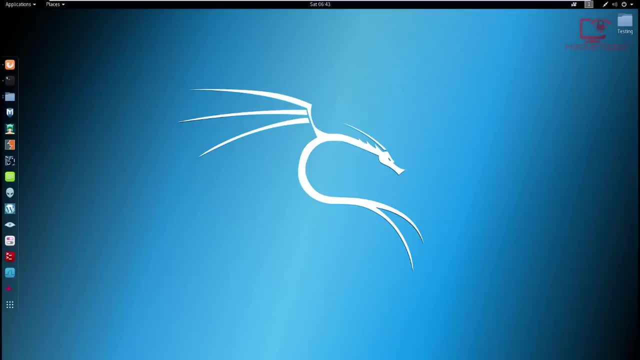 what I mean is is: these are the protection or these are the mitigation procedures put in place to protect a web application from attacks. obviously now, as a penetration tester, or if you're looking at it from a white hat or a black hat perspective. from white perspective. 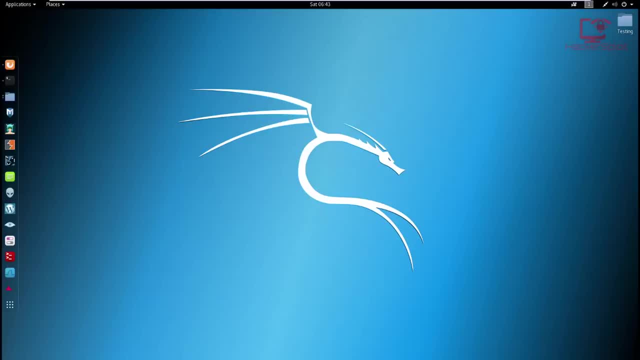 it's always important to have a web application firewall, And I'll probably make another video showing you how to set it up. it's really easy and it's free, And it'll probably remove about 20% of attacks. Okay, so that's if you're a white hat. Now, if you're a black hat and you're, 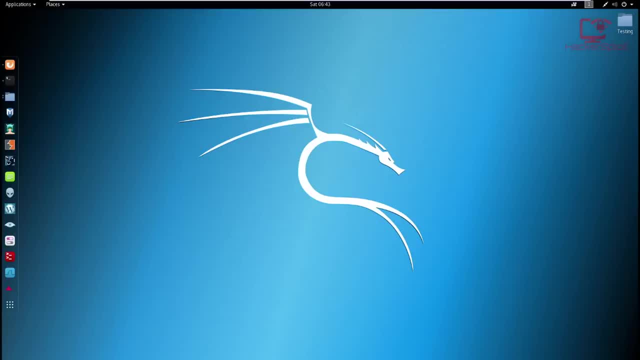 targeting or you're performing a penetration test legally on a website or web application. we usually what the employer will tell you is they'll give you a scope of the project And again they might give you the source code, etc. etc. you get the idea you have your white box testing. 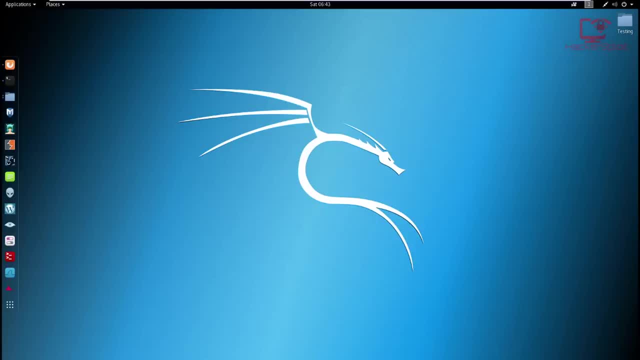 black box and gray box And you're going to be able to do a penetration test. you're going to be able to do a penetration test. you're going to be able to do a penetration test. But, coming back to the firewall, most of them wouldn't know that there is a file And that's because the person who set 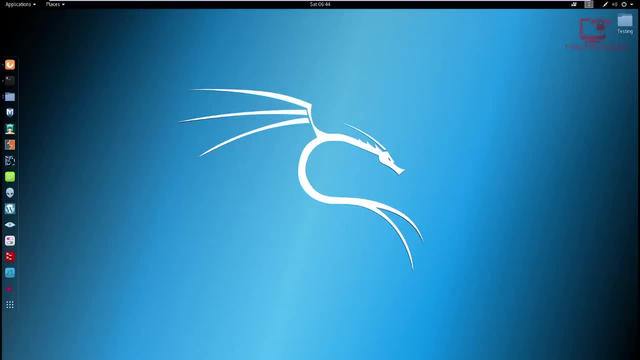 the website up for them in terms of hosting or the web application for them will, in most cases, on a professional level, have a web application firewall. Now you might be a bit confused And you might be saying: Well, why is this important when performing a penetration test? Well, 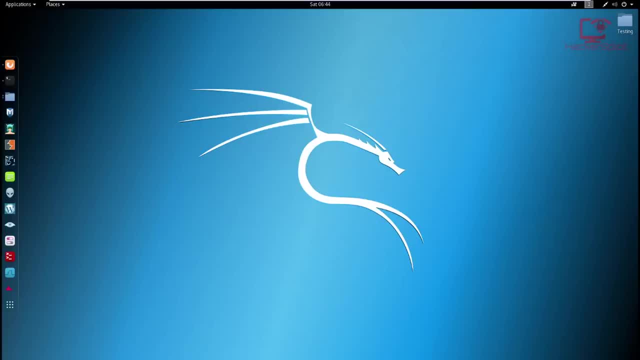 this is important because, firstly, it's something that most pen testers overlook, And if you know this, you've got an ace up your sleeve Alright. so, essentially, what's happening is if it's being used, if a web application firewall is being used. 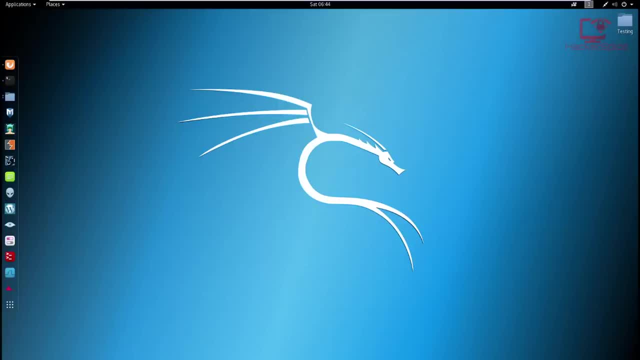 you obviously first need to detect it, And I'm going to show you how to detect it in this video, using a special tool that I don't think you've ever heard of, But it's also industry standard. So this is a real, real secret. I don't know, for some reason, it's not just, it's something. 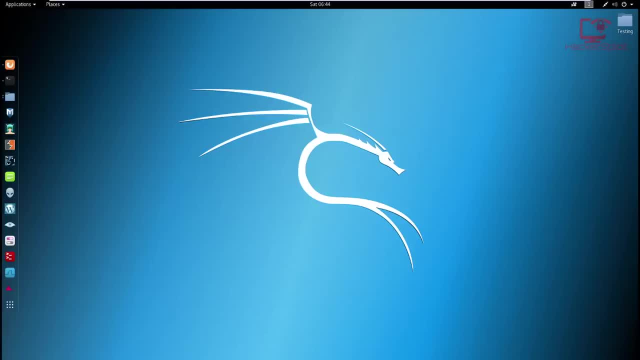 that just hasn't caught up yet, But hopefully after this video you'll know about it. Alright, so essentially the purpose of a web application firewall is it protects the web application, you know, from a firewall point of view in the sense that it. 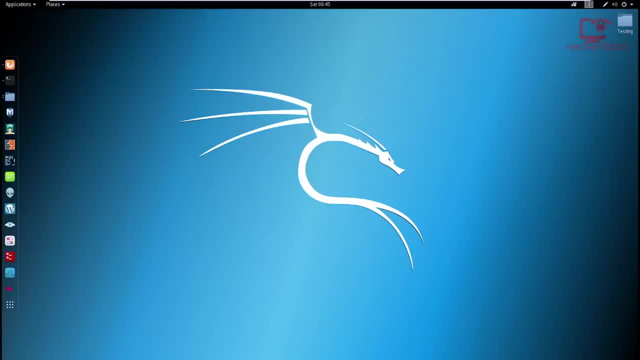 blocks attacks as one would expect them to come. Now, what does this mean for you? Well, this means that you will need to, you will need to manipulate any type of data that is going to be encoded, Alright, so what this means is, if you're, if you're performing a penetration test, 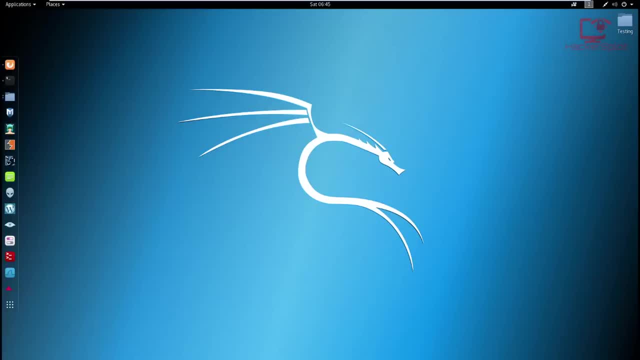 that involves you manipulating data and sending it back to the web application, then you need to encode it in a specific way to buy the data. So you need to encode it in a specific way to buy past the firewall, Otherwise it will be blocked by the firewall, And I'm sure most of you have. 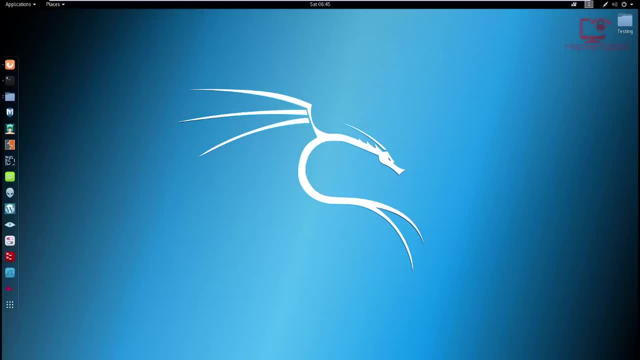 actually done this before. If you're just amateur penetration testers and you've just begun, you'll find that, for some reason, your requests aren't being processed, And that's because there are. there's a firewall setup to prevent these malicious requests from being processed. Okay, 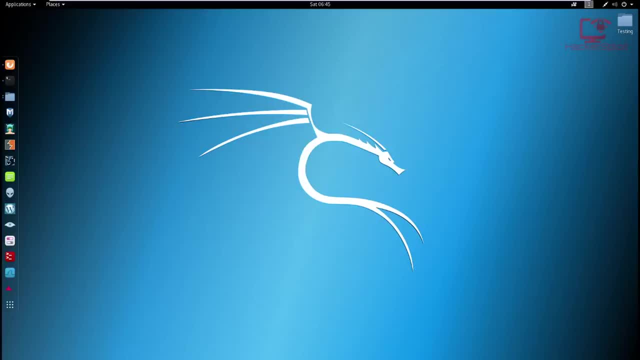 so, again, web application firewall is really important. Now, looking at the tool we'll be using, the tool has actually a very, very funny name. you, for some of you, might find it hilarious: It is called WAF wolf. Now, for those of you have heard of it, you pretty much already know how to. 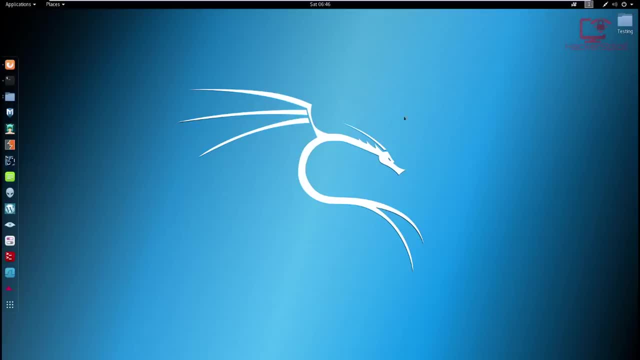 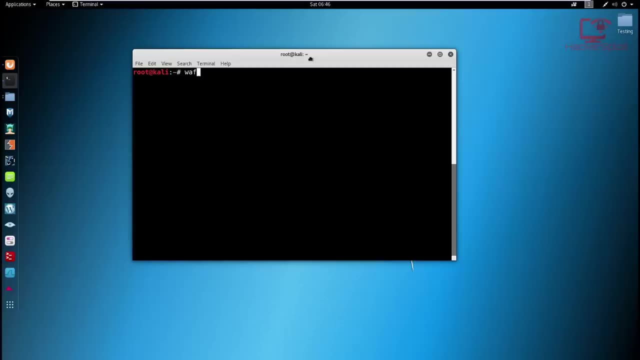 detect a web application firewall. but it's really very, very simple. Alright, so just open up your terminal And what you want to do is you want to type in WAF wolf, Alright, so this is how it is going to be spelt. So it's WAF wolf with a two, with two zeros, And the syntax is pretty simple. 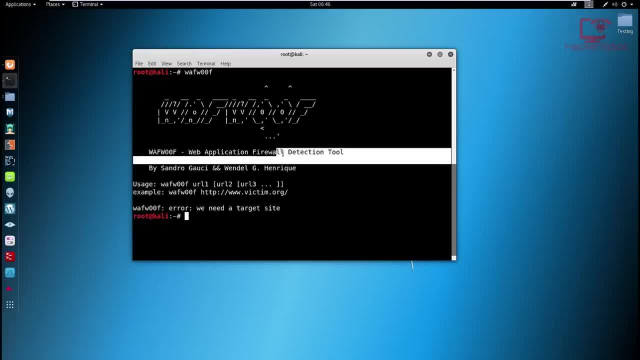 If I just hit enter as you can see WAF wolf, a web application firewall detection tool. Alright, let's go to the author. it's actually it's a tool that's been there since the- I think, almost the last version of backtrack and the first version of Kali. So again, quite an old tool When I say old. 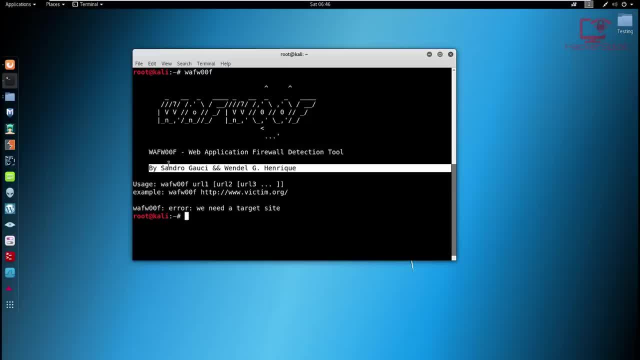 I mean, you know, I mean that with respect, given the fact that it's really, really useful and I've used it a lot because it saves you a lot of time, And what I'm talking about is: so, let's say, we want to scan a website. okay, In this case, I have my WordPress server running here And 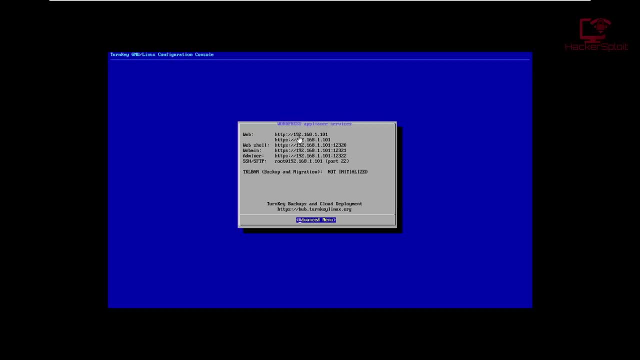 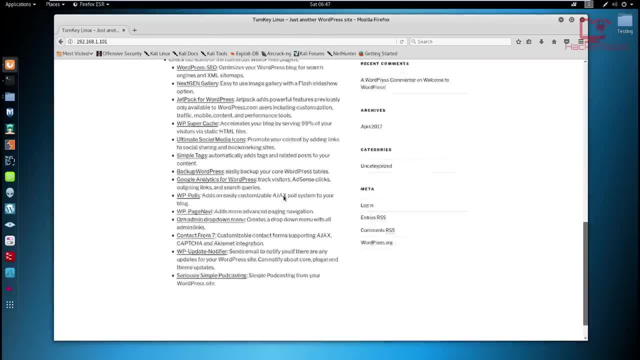 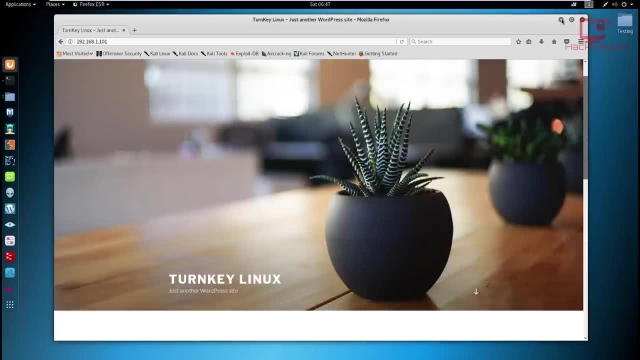 browser And, as you can see, it's a WordPress site And this site is vulnerable, And this is what we're going to be performing later on the penetration tests on, But for now, we want to find out whether it has a firewall. Now, by default, I know it doesn't have a firewall. 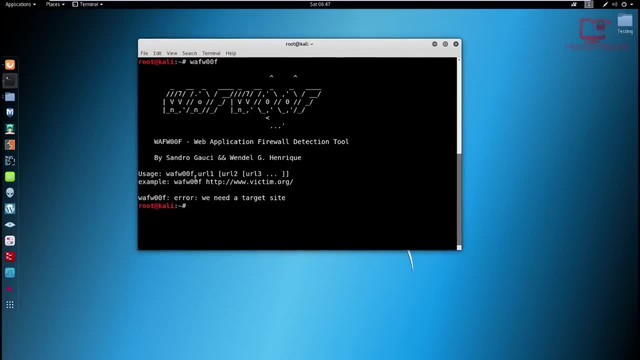 But let's see what WAF wolf would tell us. Alright, so the syntax is very simple, As you can see. you just type in WAF wolf and you enter your URL or your URL, So you can enter as many as you like. Okay, so it'll give you an example there of how to go about it. make sure you enter. 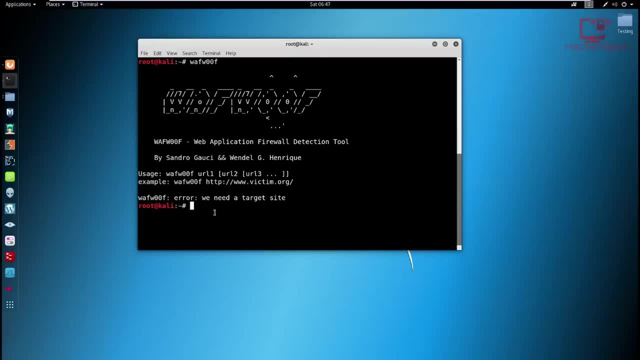 your HTTP or HTTPS protocol And we just let's try that out. So, WAF, wolf, and we specify our protocol, HTTP in this case, and the IP address 192.1, 68.1, point 101.. All right now, in this case, 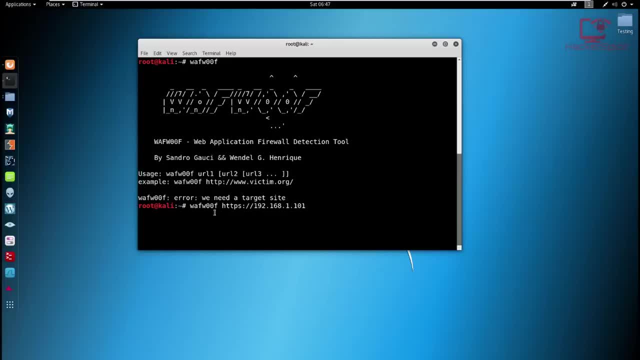 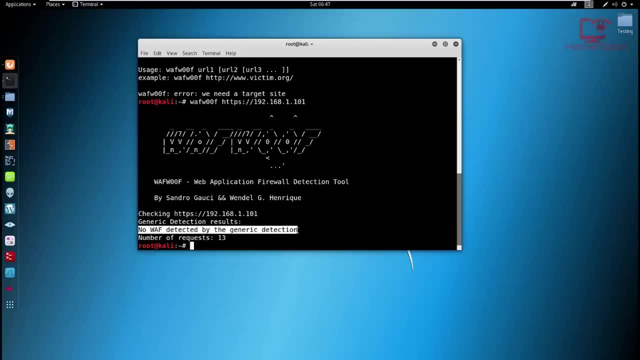 I'm pretty sure that it won't detect any web application firewall. So let me just hit Enter And, as you can see, no web application firewall detected by the generic detection. Alright, now this is very, very advanced And this tool is an industry. 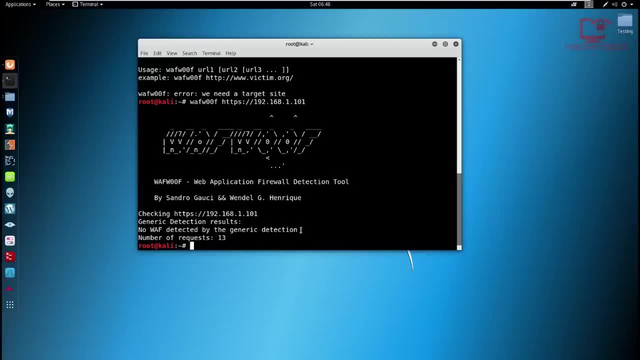 standard, And if it does tell you that there is no web application firewall, then by all means I can guarantee that it does not have a firewall. Now let's look at one of my sites that I currently own. It's a site that I use. it's actually my web development company that obviously we use for web. 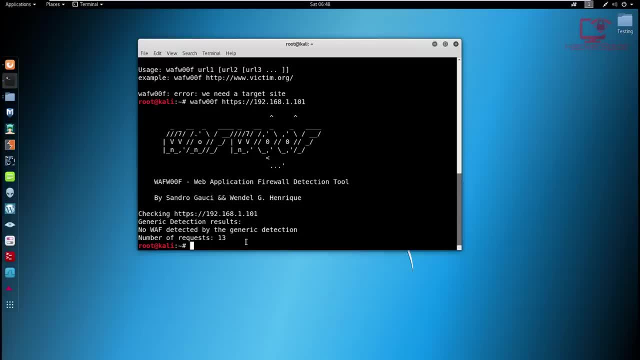 development. Now I've protected this site with a web application firewall provided by Cloudfair. Now, for those of web developers And when you're performing your hosting, you know that using Cloudflare is awesome because it allows you to optimize your site for speed, it allows you to purge assets and make 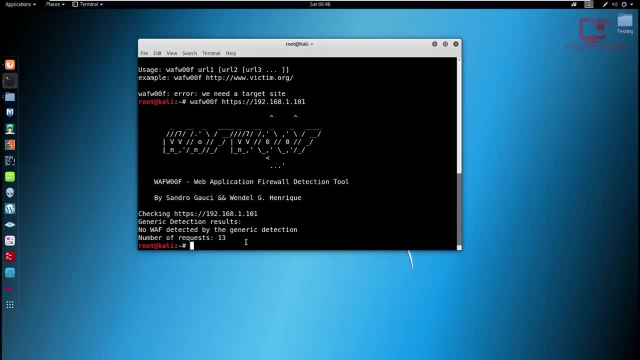 your site faster, protect it and again, protect it from DDoS attacks, etc. etc. all the good stuff. So let's see if it will actually detect this. So I'm going to type in waft wolf. I know that. 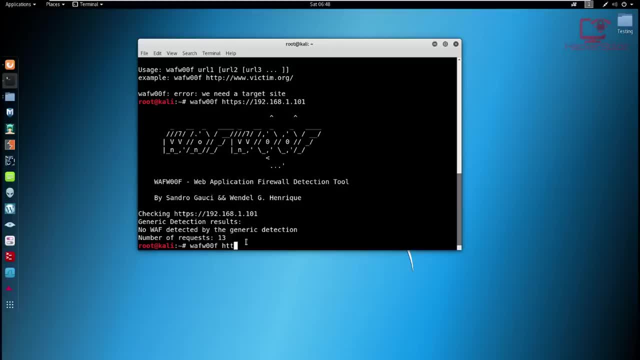 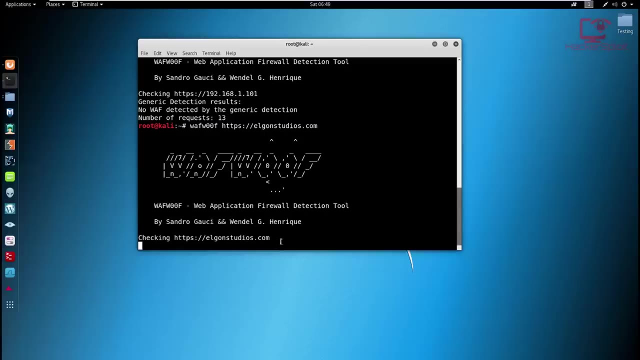 name is really funny. The protocol is HTTPS, HTTPS, like so, And I'm going to specify the site, which is Elgon studioscom. All right, Elgon studioscom. And if I enter, as you can see, it's going to start checking the site. give it a few seconds. it shouldn't take any much, you know. 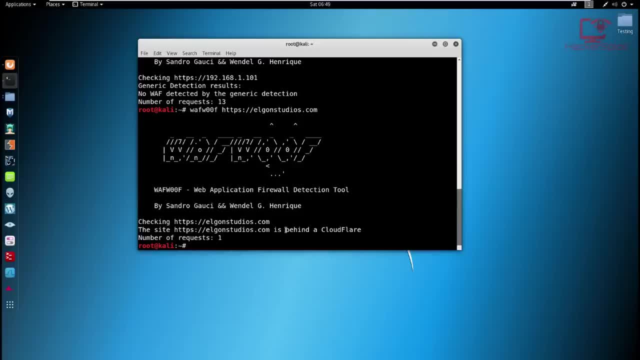 a lot of time And, as you can see, the site Elgon studioscom is behind Cloudflare Right Now. what this means is that most of the most of the attacks that involve manipulation of data will be in some way blocked, And you know you won't get your response back the way you wanted it, And 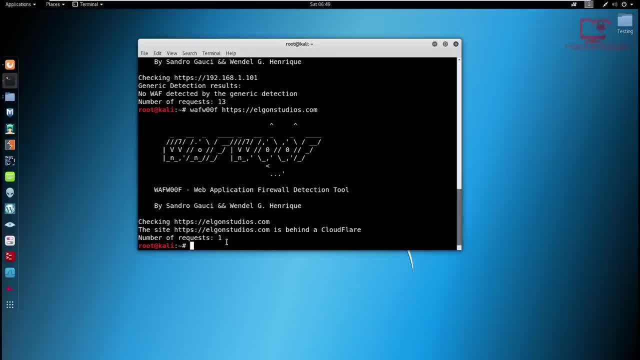 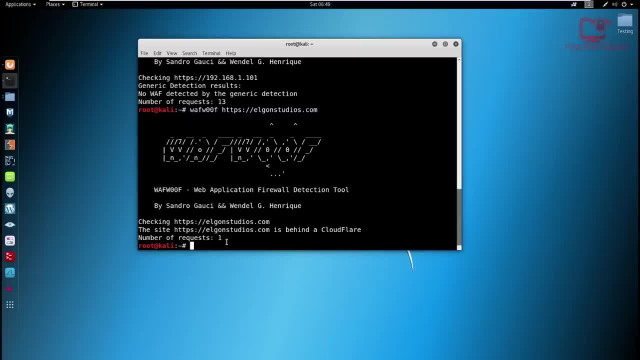 your, your requests, that you're going to be sending to the web application, And that's what we'll be looking at as we increase the security level using the, the damn vulnerable web application. All right, so I thought this is something that I really need to share with you. again, it's going to 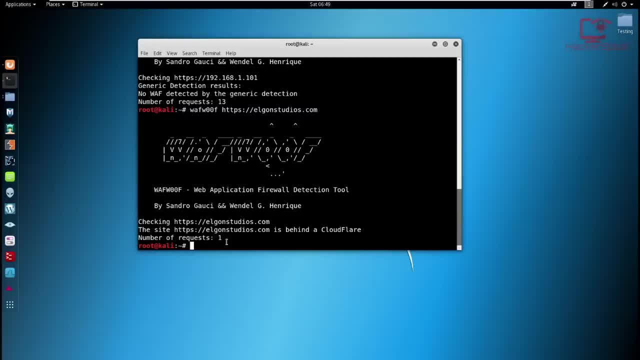 really help you And I promise you this is something that you know. if you go for a job interview or you're performing a penetration test for a company, this is something that most of the network or systems administrators are very keen on. they want to know whether you really know. 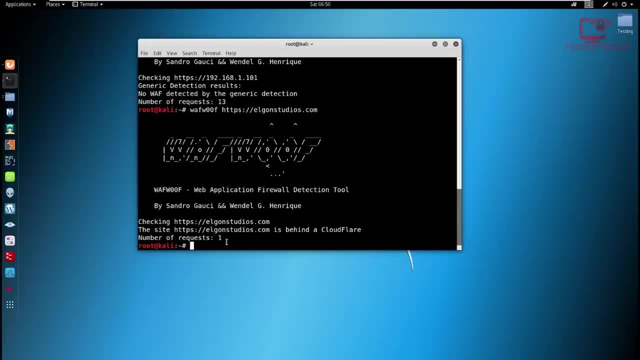 your stuff and whether you're really up to date with how to detect. first of all, because information gathering is really important And, as you can see, this tool is fantastic. And once you know there's a firewall, you then have a better idea of how to target and you won't be wasting. 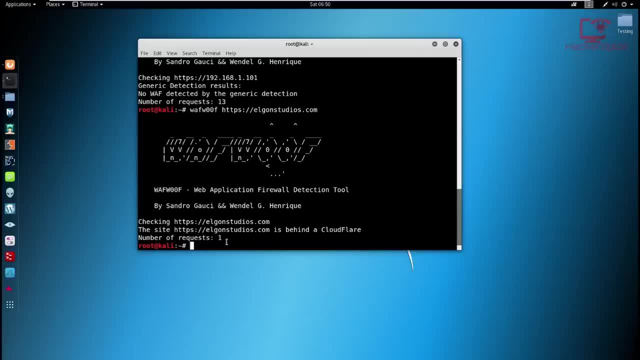 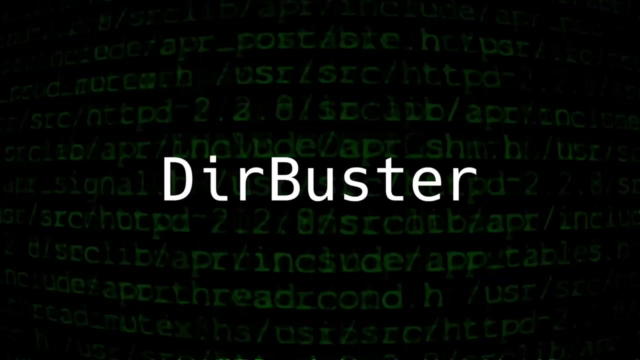 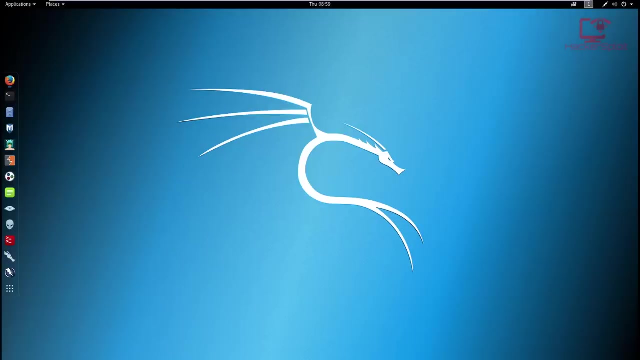 time Again. that's something that most of the amateurs or beginners do. they waste a lot of time trying different commands, And that's what we're going to be talking about in this video. I'm going to be showing you how to use the buster to discover directories and files on a website or 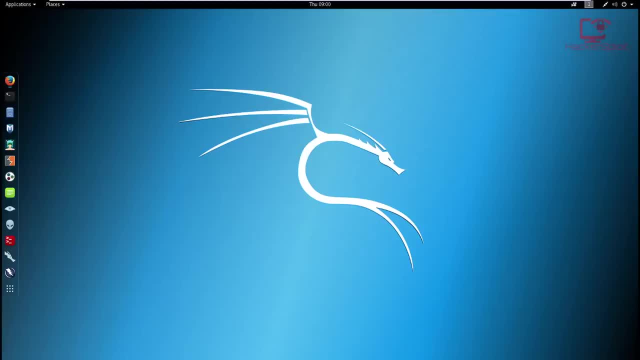 a web application. You might be asking yourself: what is the buster? Or if you haven't heard of the buster, let me explain it to you. Alright, so the buster is essentially a tool that was developed by OSP, the open web application. 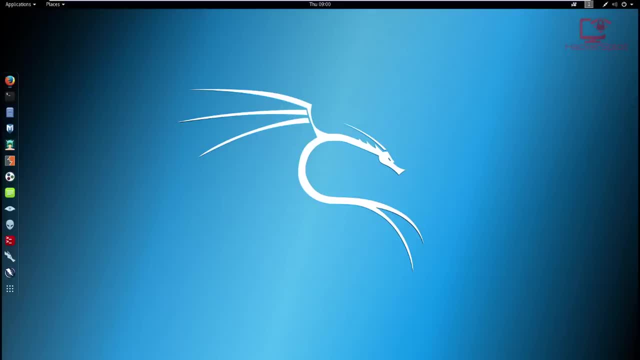 security project and essentially uses a brute forcing to find commonly used directories and file names on servers. Alright, so this tool is extremely useful for those of you who are doing CTFs, For those of you who are bug bounty hunters, because essentially, it allows you to understand. 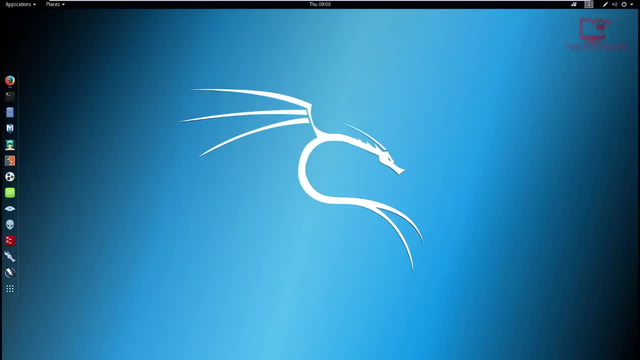 the structure of a web, web application, And that's what we're going to be talking about in this video. So let's get started. So the buster is actually a tool that's connected to a website or a site in terms of the files and directories and how they are structured. Alright, so why is this? 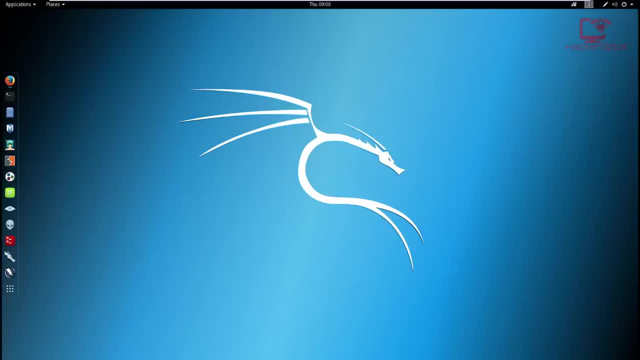 important. Well, this is important because this will help us understand how we can attack a site or what type of attack vectors we can. we can, we can find, you know. so, for example, if I had a web application- and I'm going to demonstrate that right now- and I scanned it with the bust, 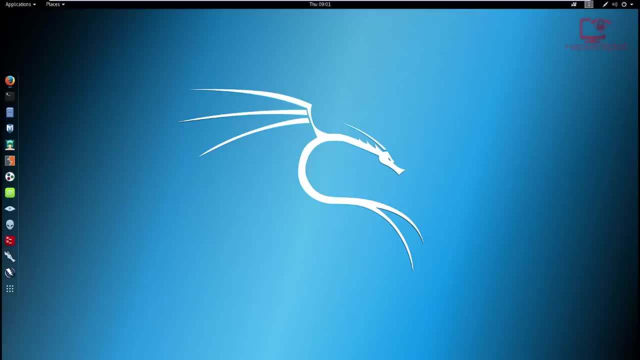 and we found some hidden directories and hidden files. we can use these as attack vectors, Alright. so, as I said, it also allows you to find hidden files we can also put in here. you know, that's where we've seen things likeор Blizzard, that's where we've seen things like that. where 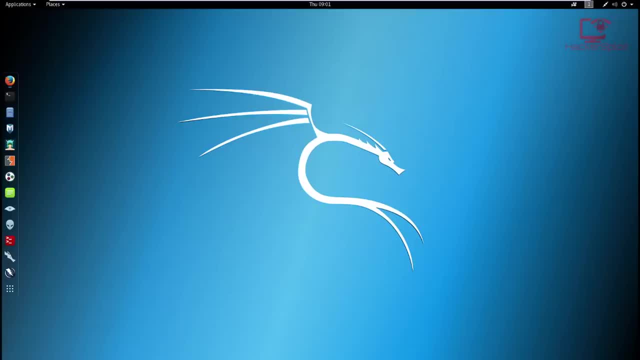 we've seen things like this, where we've seen things like this, where we've seen things like this. I said it also allows you to find hidden directories or or files that are hidden from the public, So these can also lead you to to finding additional resources that could have. 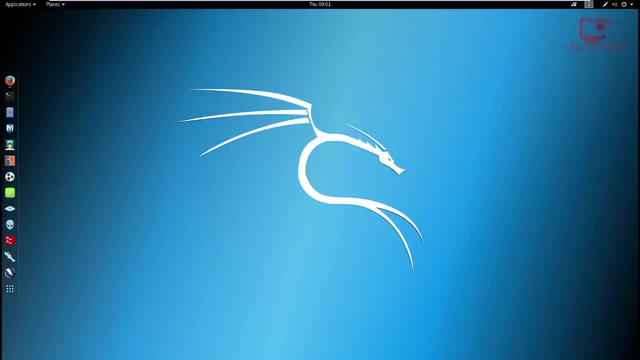 been hidden away by the devs that like, for example, admin pages, etc. etc. All right, so how does it work? Well, really simply. once you start up the buster- and again, as I mentioned, it uses brute forcing, So I'll explain where word lists come into play- So you open it up. 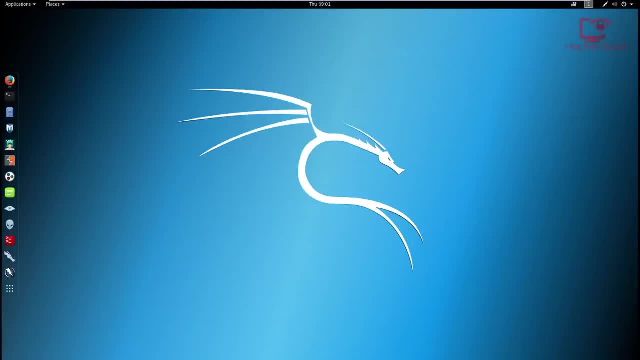 and you select the URL of the web application or the website and you specify the port. the port is is definitely going to be HTTP, So either a port 80, or port 443.. And then you select the word list. Now, in this case, Kali Linux already has a dub dub buster word list that. 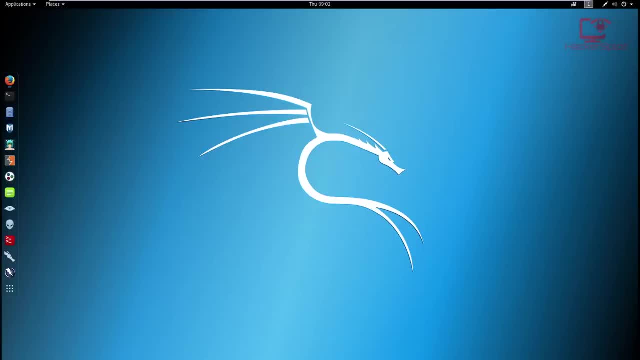 that are designed. it has three of them that are designed for different types of scenarios, And I'll explain them as we move along. All right, And essentially how it works is, once you start the brute force, you're going to have a list of all the different types of scenarios that are designed. 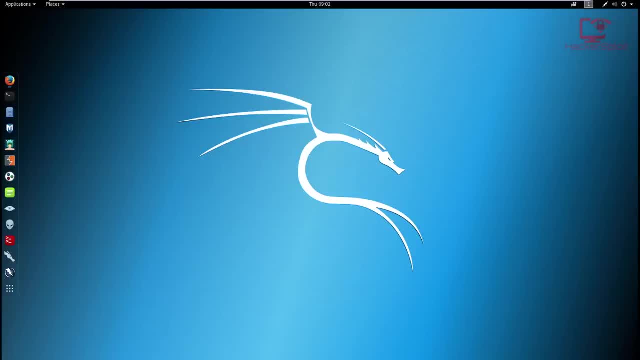 for different types of scenarios And I'll explain them as we move along. All right, And essentially how it works is, once you start the brute force attack, it will send HTTP, get requests and it will wait for the response from the server or the web, the web application, If it gets a 200. 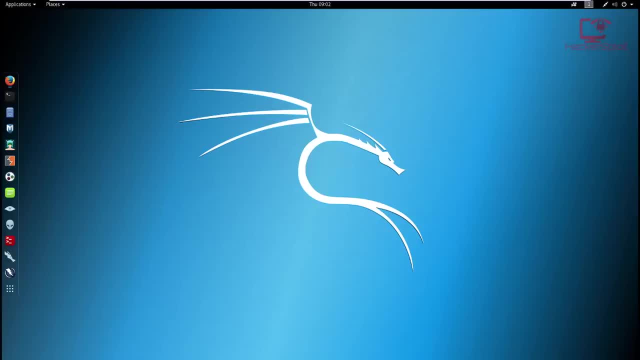 response. that means that, yes, that directory exists. All right if it gets. if it gets a bad response, meaning like 400, or 403,, meaning no access, then it will. it will. it will know that that directory or file doesn't exist. So it's essentially testing directories on the server. 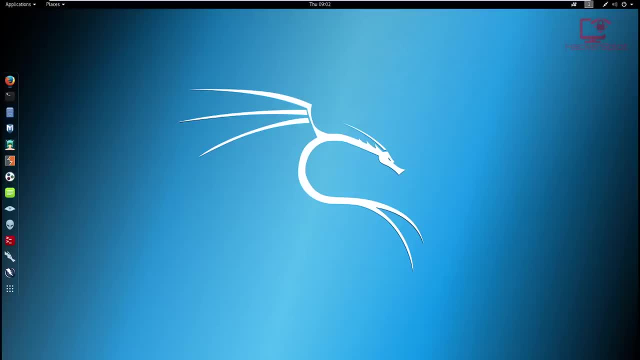 against this, this word list. So it will check. for example, is there a temp folder? if it sends a temp request to the server, it gets a response, a positive response, then it knows it's there and then it will enumerate them. Alright, so let's start off. 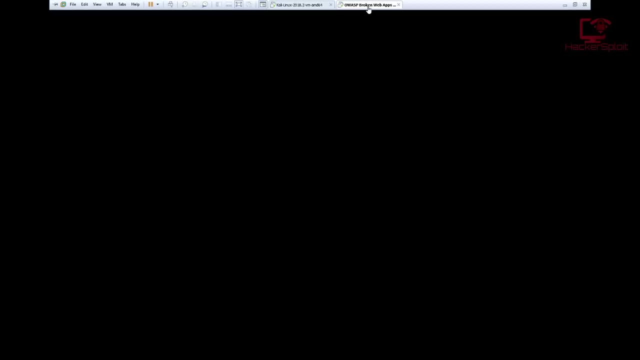 really, really simply. So I'm on calendar. Next, I have the OS broken web application right here And I'm going to be demonstrating a two scenario So you can see I'm running that here And that has a lot of vulnerable web applications. But the whole idea is to 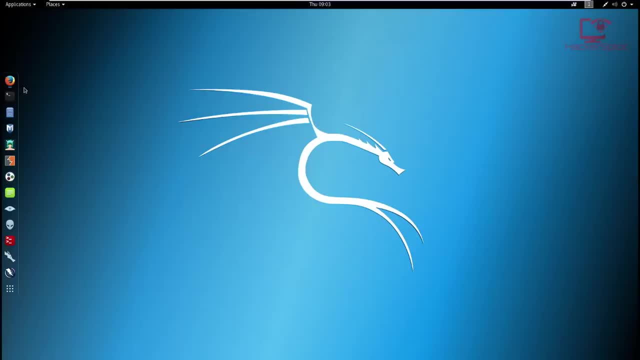 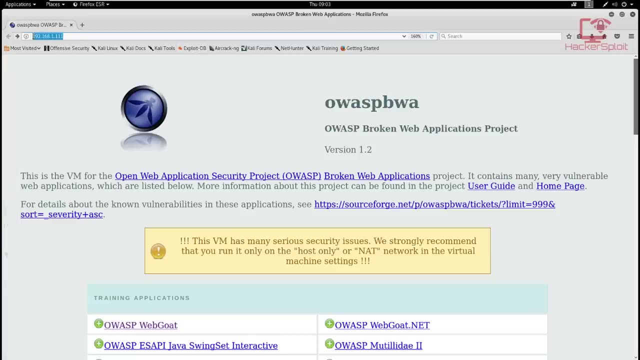 demonstrate how directories can be found All right and why this is extremely important, especially for a web application penetration tester. Alright, so I'm going to put up Firefox And, as you can see, I have the open web application project right here, the OS B WAP. 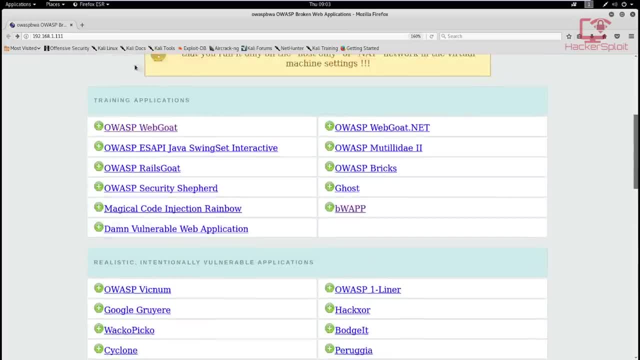 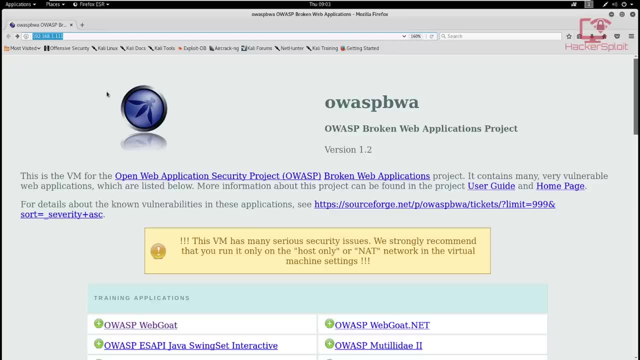 as they call it, and it has plenty of of ways of me testing this. But what if I was to just test the entire server? Alright, so this is a web server. What if I was to test the entire web server? Well, 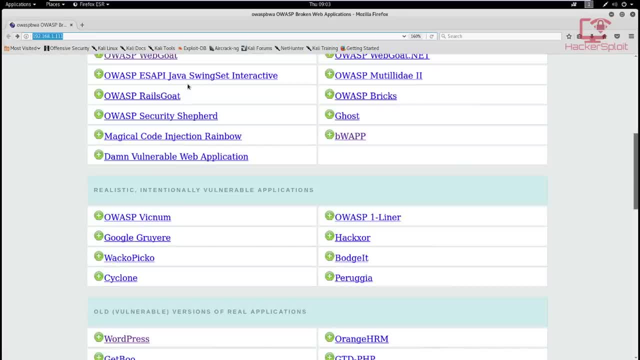 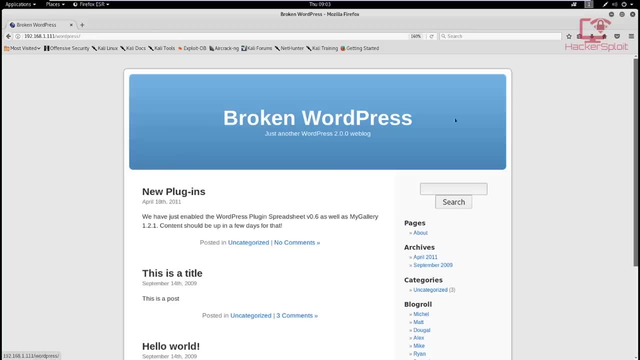 I'm guessing that they're going to be a lot of files and directory. So what we can do is we can start off with a perfect example of how this will work- is, let's say, you're targeting a WordPress site, So I'm going to open up the broken WordPress. Now, of course, this is a very old one And we're not. 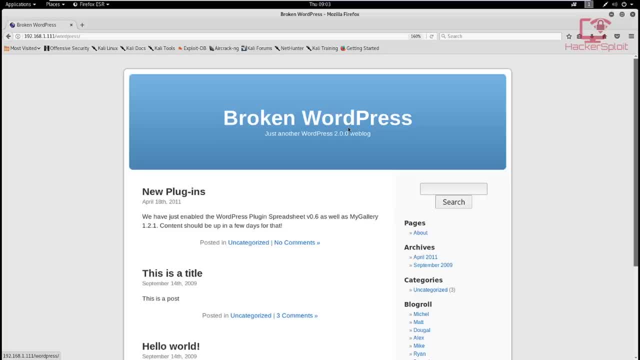 really exploiting anything, But by using this example it will let us understand how we can enumerate the different directories and folders you know on this WordPress installation, Or if you are target targeting a WordPress site. this is the way you do it, So I'm going to copy the 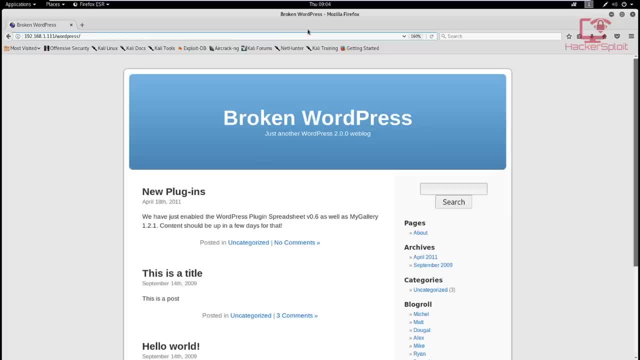 URL with the with the directory right here. So it's- we know it's- in the WordPress folder because that is the root directory of the of the web server And we're selecting the WordPress installation. But for the website you'll select the URL right. And as for the port, 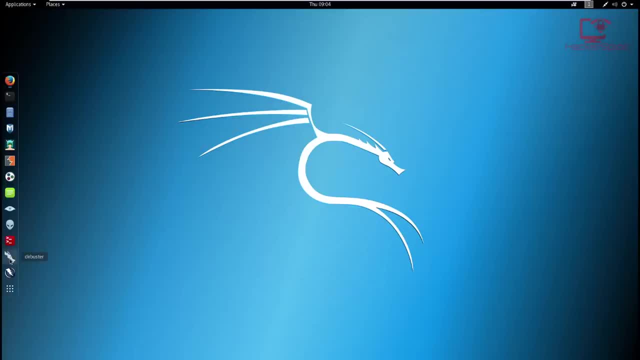 we know that this is the default HTTP port, which means it's port 80.. Alright, so I have the burst right here. If you can find it, just, you can use the Start menu and type in the buster it's going to be like. so just just click on it and give it a few seconds to start up. So again. 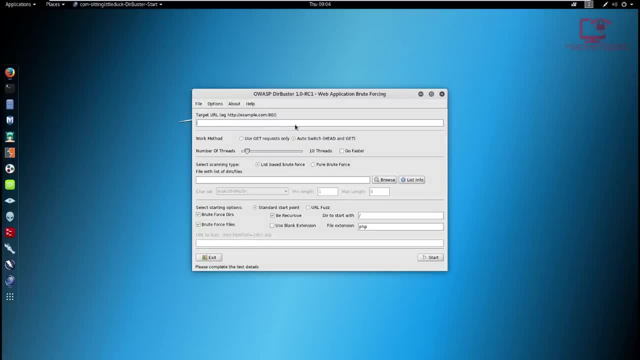 it was designed by the OS team, So it works really really well. And again, something that I'm sure if you, if you are a web application penetration tester or you do do the CTF challenges, then you'll you'll know that use this tool a lot. Alright, so we in here. 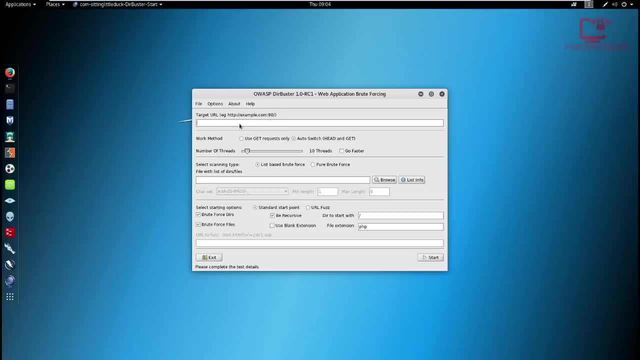 we have the target URL and that's where we would paste it. Alright, so we can paste it right here. So Ctrl V and that is the URL Now in the work method. if you want to, if you want the scan to, 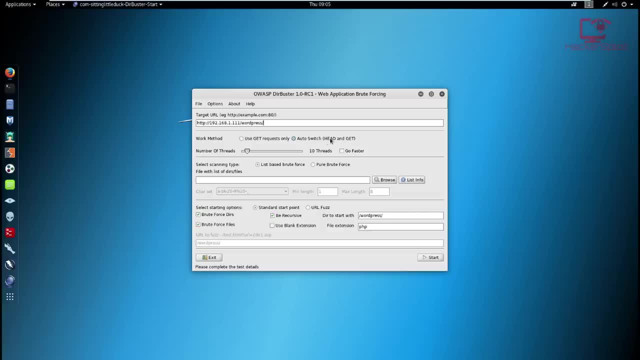 be faster, you can use the get requests, But what we can do is auto switch them from the head and get, and that will give us a more robust or a more accurate response rate. Alright, so in terms of the number of threads, this is how fast you want. You want the scan, or the brute force, to 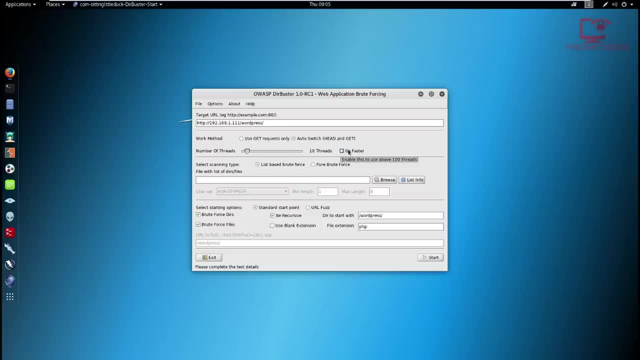 be. so the faster the better, depending on your hardware, And of course you don't want to overload the server. So I'm just going to go hit, click on, go faster. That's probably works the best for me, But if you want it to run faster, then that means it's gonna- it's gonna have multiple. 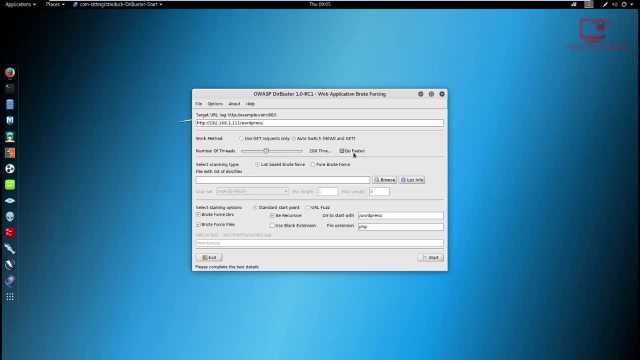 requests and threads being sent from your computer. Alright, so I like keeping it at just threads, which is go faster, And because I'm testing my own web server, I can you know I can pretty much increase it to whatever I want. So usually if you're talking about a bigger server, 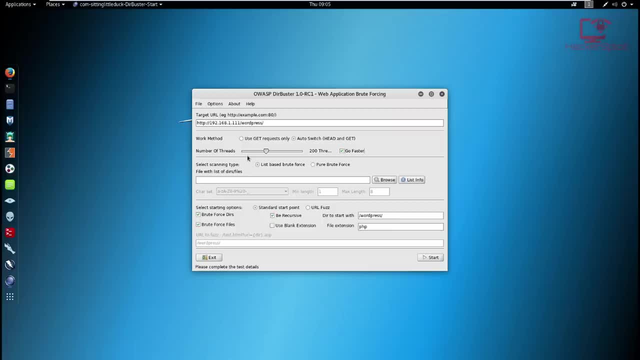 or a bigger web application, then it doesn't really matter how many requests or how many threads you use. it will not really affect the performance of the web server. But if I was to run it at maybe a maximum speed, you would see that the web server would be lagging out you. 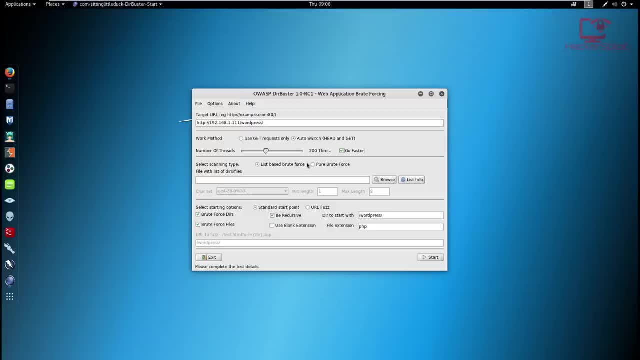 know out of the amount of requests that are being sent, Because you know you have to understand it from a fundamental point of view. we are requesting the different web pages and the server has to process them. So if the, if the server is not running on on. 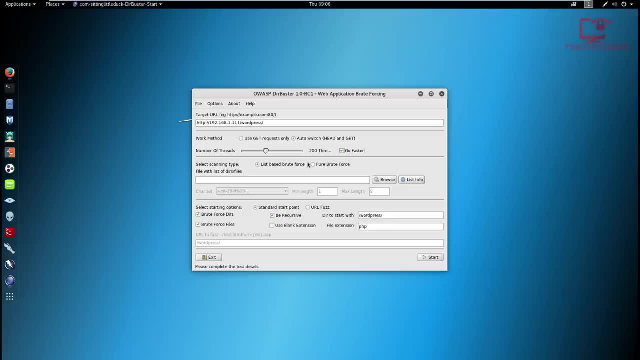 you know, good resources. like it's running on one gigabyte of RAM, it's very easy to make it lag out And to actually cause some sort of a denial of service just because of the amount of requests. But in this case we're performing it, you know, with with an ethical perspective. 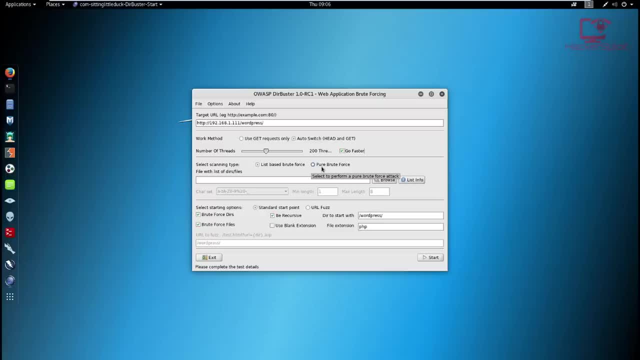 So now you want to select a list based brute force or you can use a pure brute force, but I don't recommend that. that doesn't really work- And you now need to select your word list, your dev Buster word list. Now by default on Kali Linux and on parrot OS. these are found in the 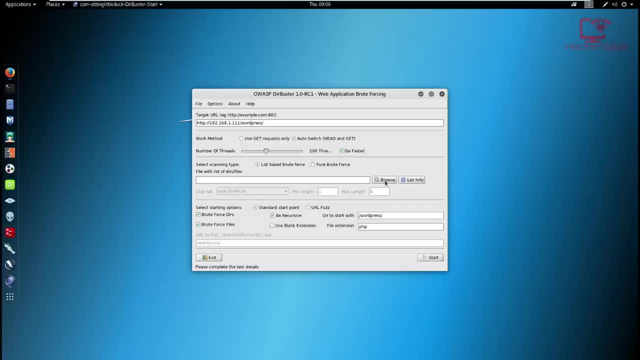 user share folder on the underword list and you can find the dev Buster word list right there. So I'm going to show you that right now. So I'm going to browse, I'm going to go to my route and I'm going to go into user And I'm going to go into share And let's go into word lists here. 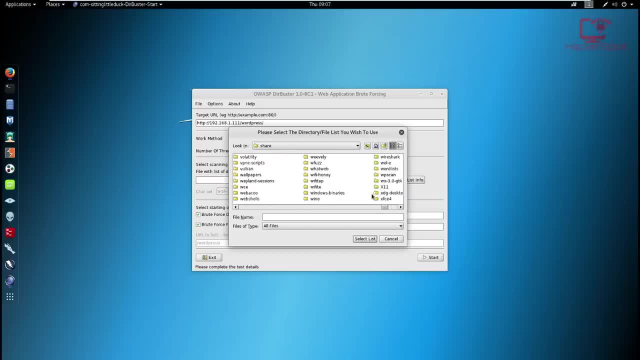 Let's see if I can find it. It's obviously with a W. Where it? Where is it? Let's see, Let's see. Let's see, Where is word lists? Sorry, if I can see this there. There we are. 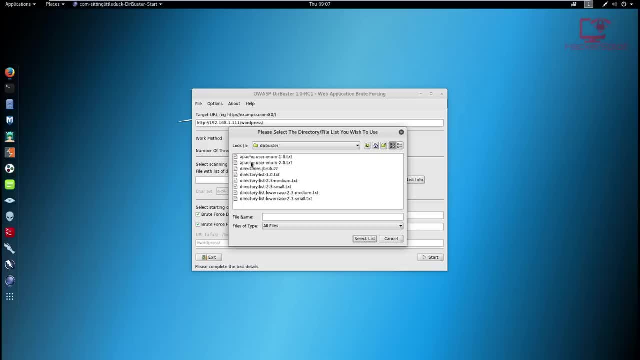 Sorry about that word- lists. And you now want to go into dev Buster? Alright, so there is going to be a folder called dev Buster, And now you might be a little bit confused. Well, really, you don't need to need need to be confused. That's why I'm here. So, as a beginner, you might be wondering. 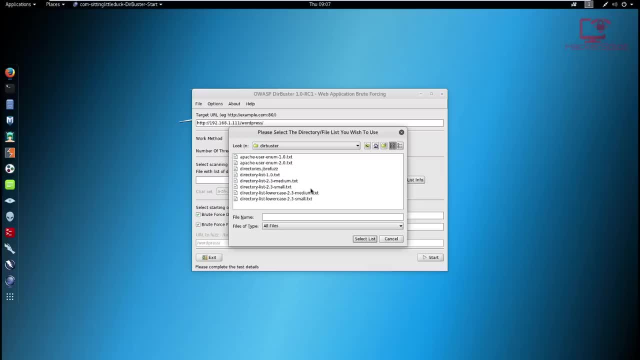 like which one is better. Now, as an advanced penetration test, I know which one is the best. In most cases it's going to be the medium, the directory list 2.3, medium dot txt. Now, if you're scanning a very small web application, that that's not that really. 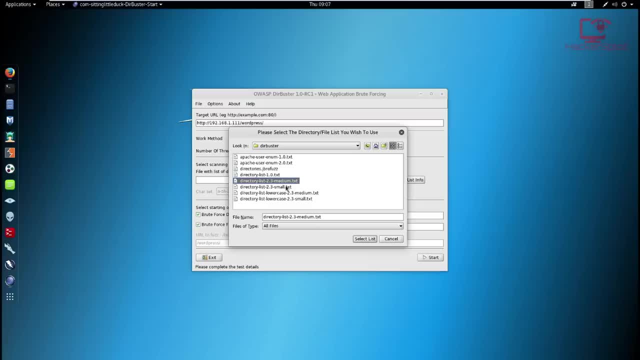 complex, like a simple HTML site- you know HTML CSS, whatever you want to call it- then I would recommend the small one. But if you're scanning a big site, like a WordPress installation or a Joomla installation, then you should use the medium one. this will work 99% of the time. 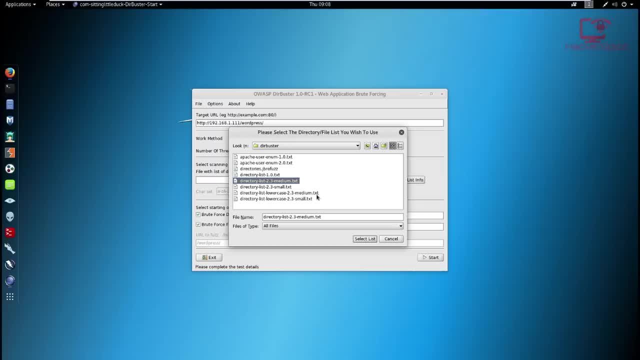 unless your your, your requests are being blocked by either a web application firewall or by the, the host. So I'm just going to select list, All right, And now, in terms of these other options, you can see it's, it's going to essentially brute, brute force the directories, the files. 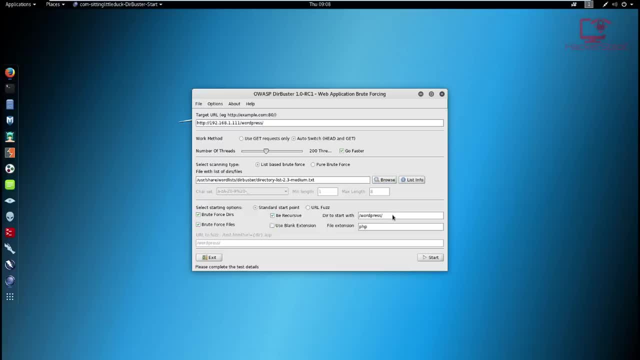 it's going to be recursive, which is great, And the directory: you must specify the directory if it is. if you are trying to perform a scan, that is directory sensitive, All right. And standard start point, just leave it like that. And you now want to hit start, Alright. so once you start, 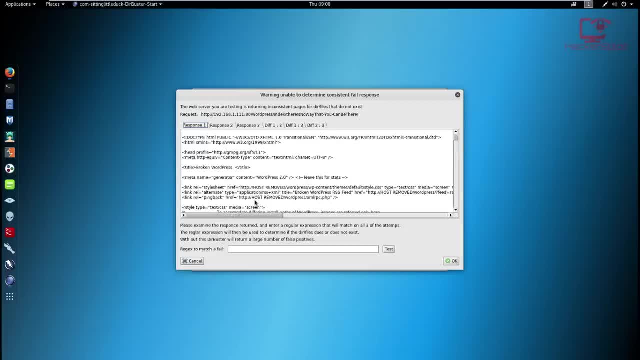 it's going to start brute forcing the web server against. it's going to start sending the requests And if it gets the responses, the positive responses, it's going to. it's going to understand that, yes, that directory does exist. Now you can see. we. 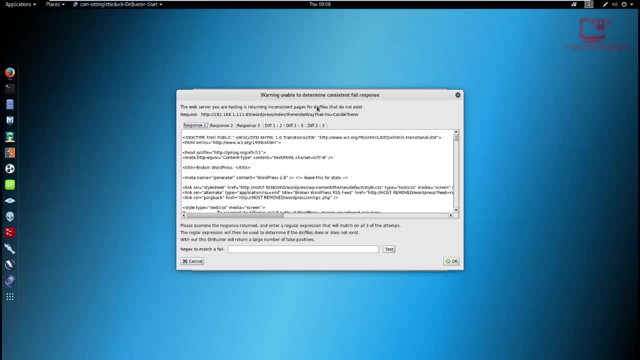 have a response that is being sent here And it's going to tell us, tell you, that it is unable to determine a consistent fail response, which means some directories and files are being you're getting a negative or you're getting a no access response, meaning that that directory doesn't. 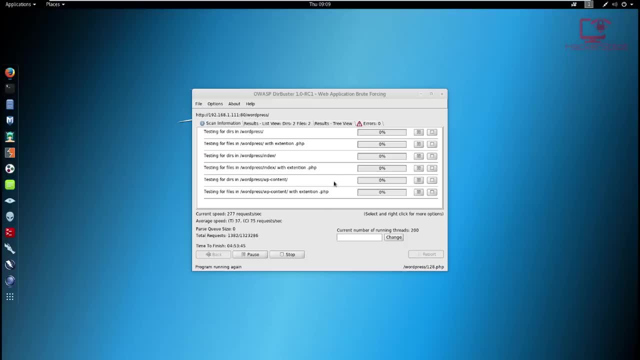 exist. So what you can do is just hit cancel to these ones and hit Yes, And it's going to continue scanning the other ones And, of course, down here you can see, since it's performing a brute force. you can look at the current speed, which varies. 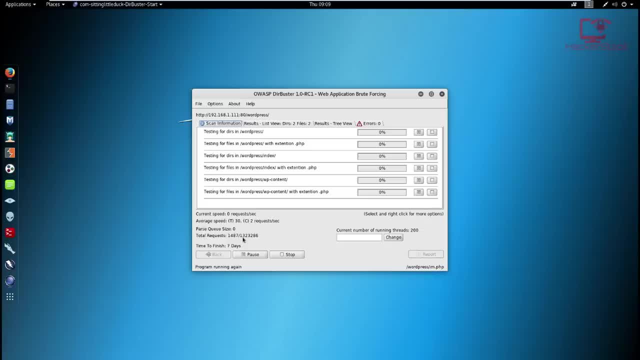 dependent on the amount of directories, the average speed And it will tell you the total amount of requests done out of the amount that could be done, depending on on the word list that you have selected. And finally, you have the time to finish and of course this will vary depending on a lot. 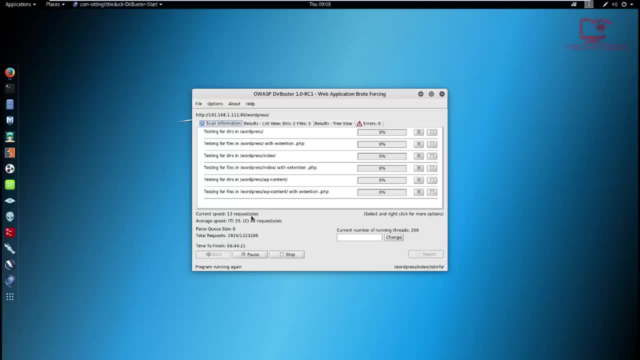 of factors, But mostly it depends on the, the, the speed of the scan that you've selected, And the and the word list. So you have your scan information here it's going to tell you what folders and files it's testing And in here you can see the results in terms of directories and. 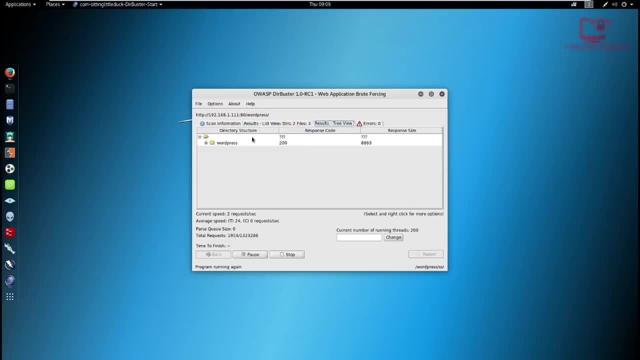 files that it was able to find And, in the results, this is going to give you the directory structure as to how files and folders are being structured on the web application. Now, by default, right now, you can see the amount, the files and folders that it has found, for example, 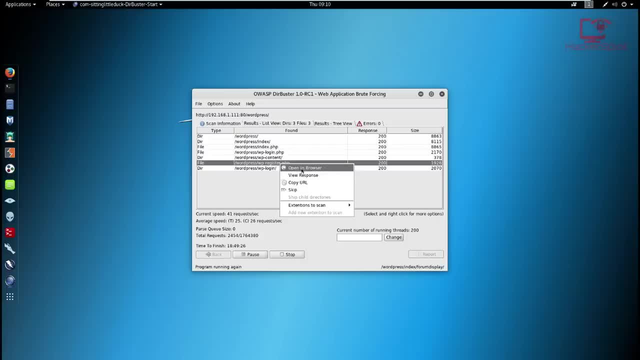 the WordPress register dot PHP. So if we open the folder, we can see that the files and folders that it has found are, for example, the WordPress register dot PHP. So if we open the folder, that if you right click on it you can open it in the URL Or you can view the response that it. 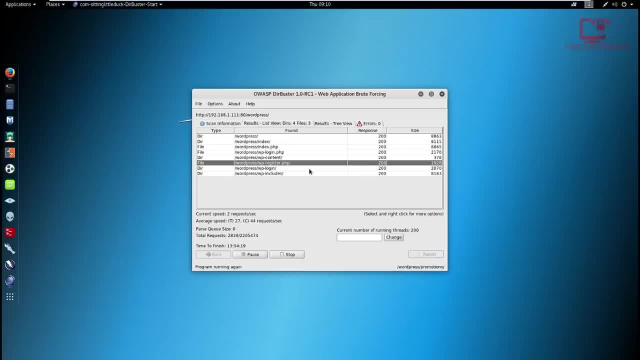 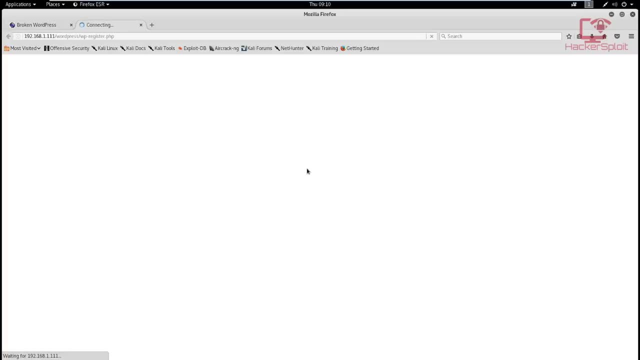 gave And you can copy it. you understand, you get the basic functionality here And then you can open it in your browser. So again, you see, with that we are finding files that we otherwise wouldn't have known existed. Now, of course, for a default WordPress installation you would have: 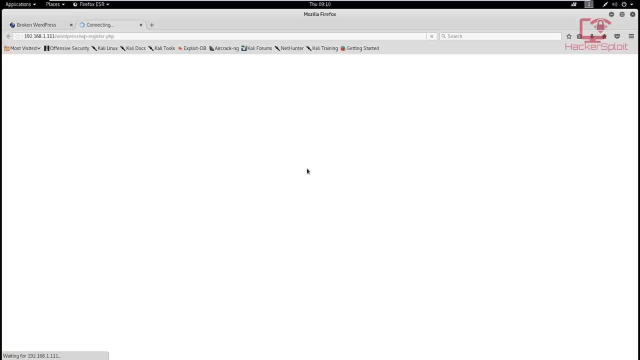 guessed that this does exist, But remember most people for most other installations on configure configurations. this can be a great way of finding files and folders that you didn't know existed. And again, discovering them is very, very important And this can give you different attack vectors. for, for example, if I went to the admin dot PHP. 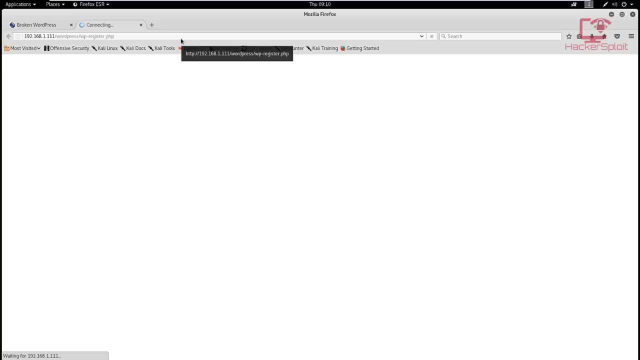 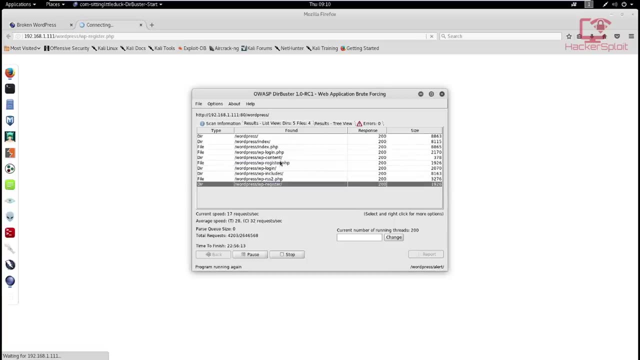 and it forced me to log in. that might be a good place to start brute forcing If I had credentials. if not, you can choose select another attack vector. So let me just move back here. you can see we have the register page here, which we just clicked on. let's look at the 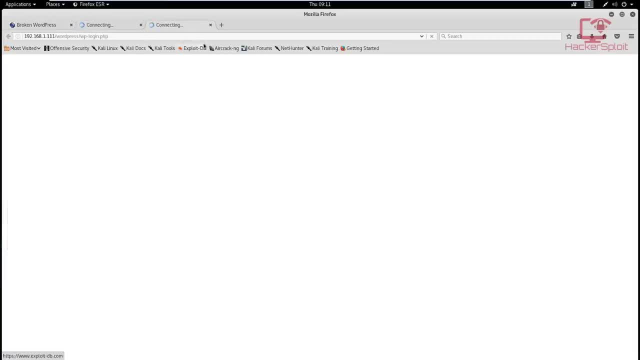 WordPress login dot PHP. So I'm going to open that up in the browser Now. you can see the server is not responding. So I'm going to open that up in the browser. Now you can see the server is not responding, And that's another point that I wanted to point out. if you want to be, as you know right now, 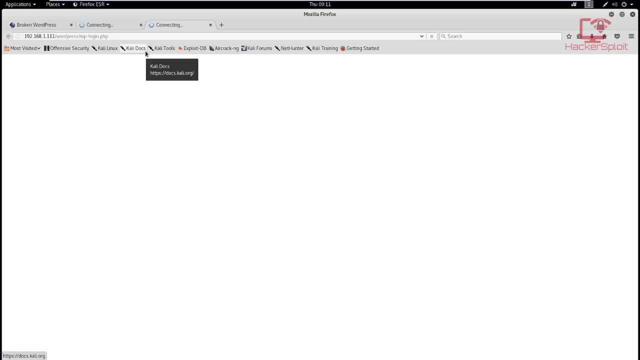 we are being as promiscuous as possible because we it's not really a web application that is delivering service to other people, but because it's hosted on my local air network. So in this case you can do a performing a type of denial of service, And that's because the server I've 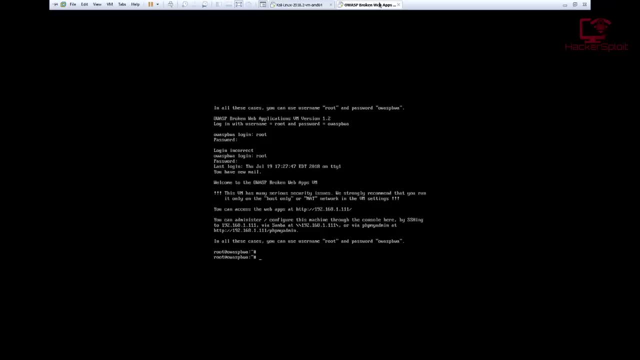 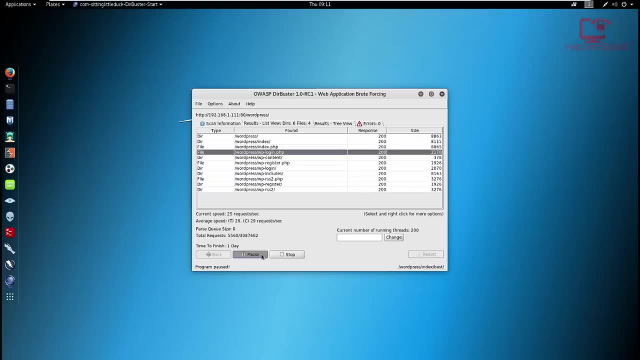 allocated very, very minimal resources to this virtual machine, So that's why it's kind of lagging out Alright. so that's something to take into consideration if I was to to pause the attack, Like so if I was to just pause it. remember you can pause it and you can. 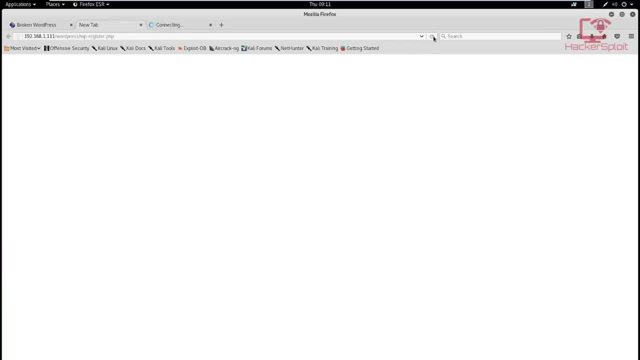 stop it And let me just go back here And let's see if we can reload these pages. they should be able to to be reloaded quicker Now let me. let me just load that up And we can close this one. 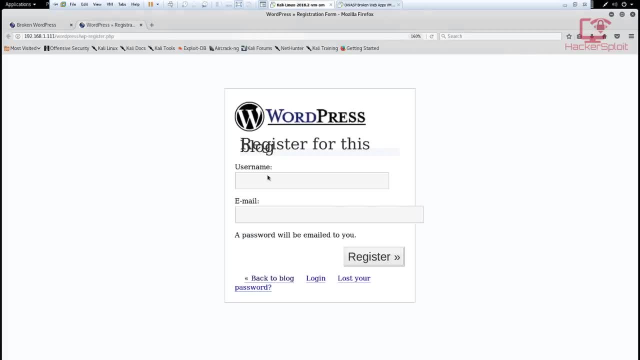 Let's see if the WordPress register page does open up, If this virtual Yeah, there we are. So you can see, even though this is a very old WordPress installation, that we were causing it to lag out, So always keep that in mind that. 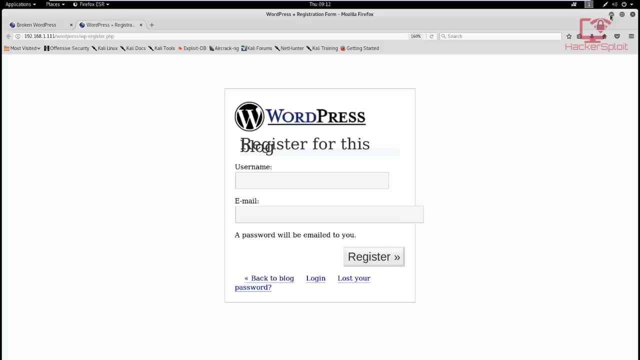 the amount of threads that you select can affect the performance of the website or of the web application And you don't want to cause any any impact to customers if you're performing the test on a real world working web application or website. Alright, just something you might want to. 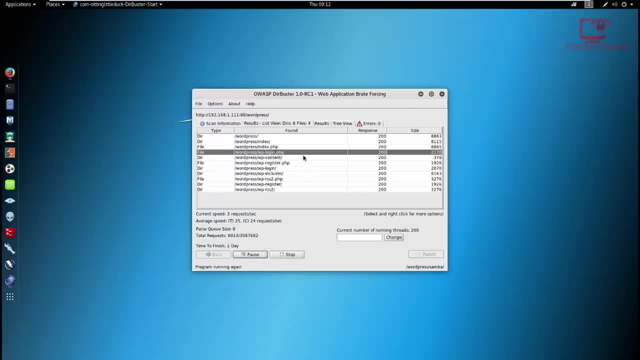 take into consideration. So we're going to resume it And, of course, I'm not going to expect to find anything weird here, Although this WordPress installation is designed to be vulnerable, So you can also change the number of threads running right here. 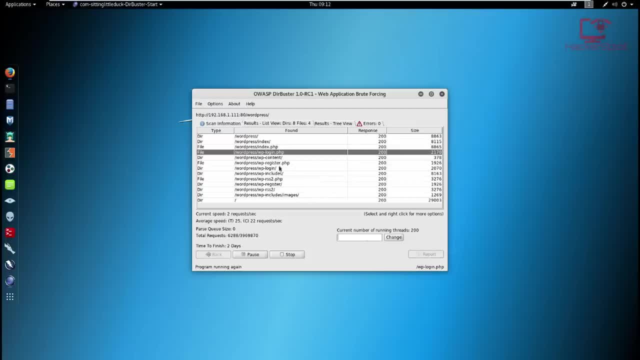 So if I wanted it to run, you know, maybe on 10 threads, which is quite slow, that means you'll get the enumeration process will take longer. So it's all about balancing your resources and understanding what you're trying to look for Now. of course, this can be a very, very useful tool. 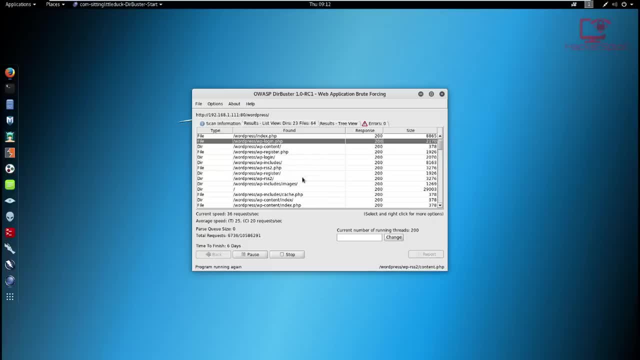 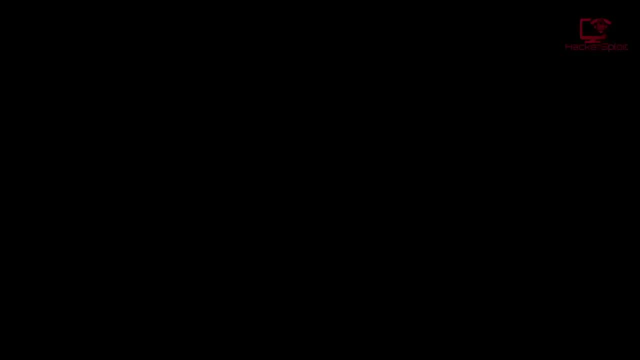 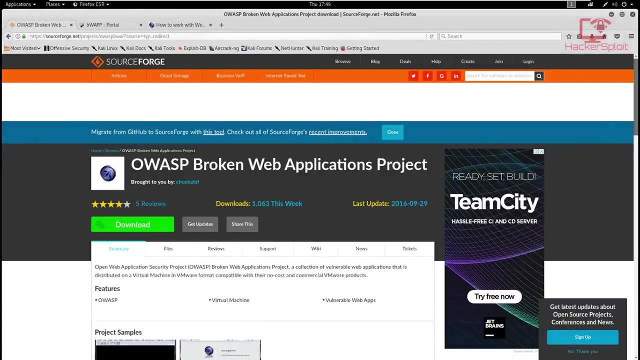 when doing bug bounties or- or CTF for that matter- especially hack the box. We are going to be looking at something that is extremely, extremely important and something that should be understood completely, And that is cross site scripting. All right now, before we get started, I'm just going to explain what we're going to be. 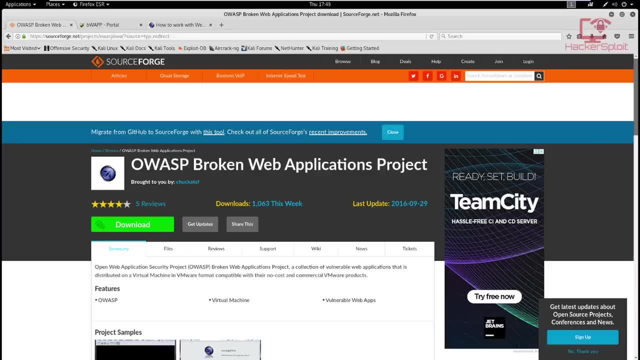 looking at, explain what we're going to be looking at in this video. we're going to start off with explaining what cross site scripting is. I'm going to be showing you the environment that we'll be using for testing any of these, any of these attacks, just because they allow us to illustrate. 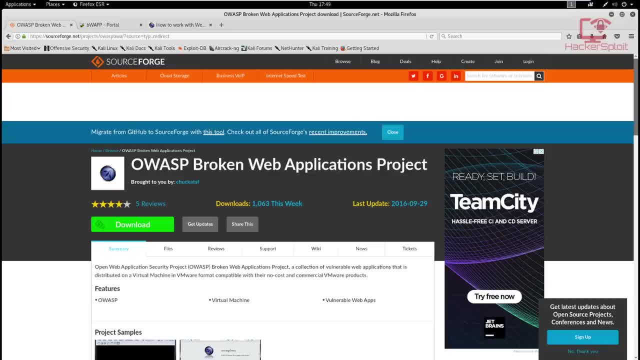 or they allow me to explain how everything works, because that's what we're going to be looking at. That's the most important thing. for me is that you understand what you're you're listening to and you have a good representation of what's going on. Alright, so I'll be explaining. stored. 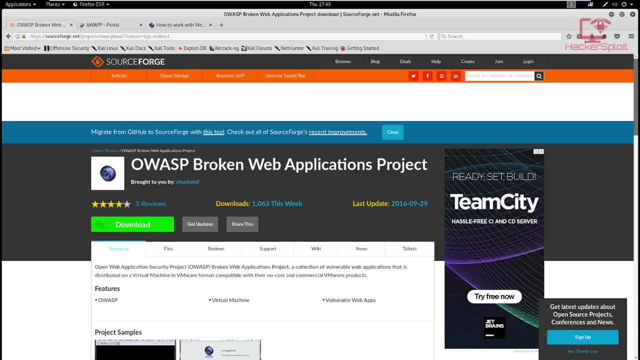 I'll be explaining reflected stored and DOM cross site scripting. Alright, so let's get started with me explaining what environment I'm currently running. So you can see that I'm running Kali Linux right now, But I am going to be using the OS broken web applications project, So I'll 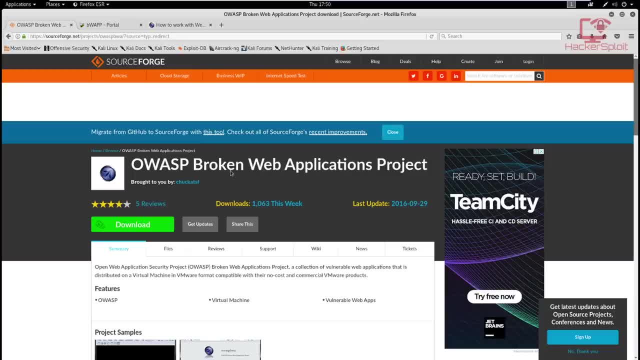 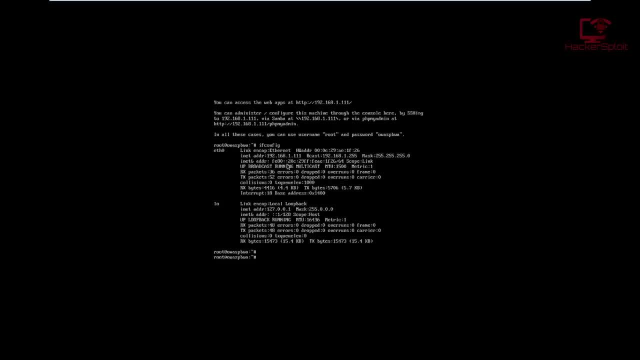 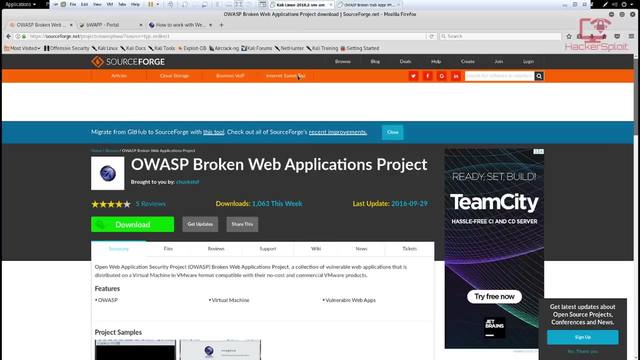 in the description section. it is essentially a virtual machine that you can easily just run on VirtualBox or VMware. I'm currently running it here. As you can see, I just got the local IP. It's 192.168.1.111.. All right, so I have that running And I'm running this on Kali Linux And 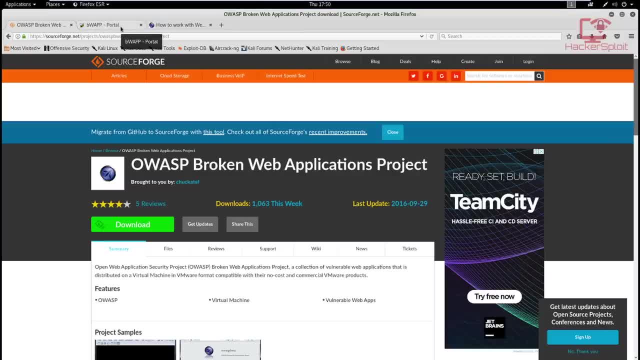 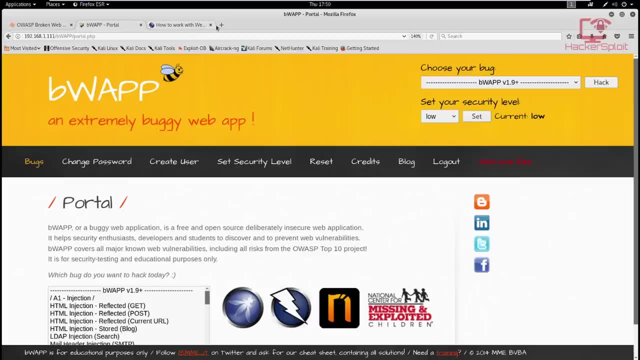 I already have opened up the URL in my browser So you can see from here I've opened up bwap And I've opened up web. go to, because that's what I'm going to be going to be using to explain each of these cross site scripting attacks. So if I was to do that, 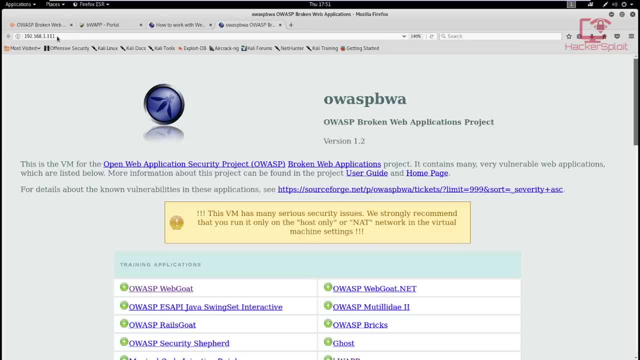 if I was to just open up 192.168.1.111,, yours could be different- it should be different- depending on your IP configuration and subnet. then it'll take you to the OS BWA or the OS broken web applications project. The latest version as of recording this video is version 1.2.. 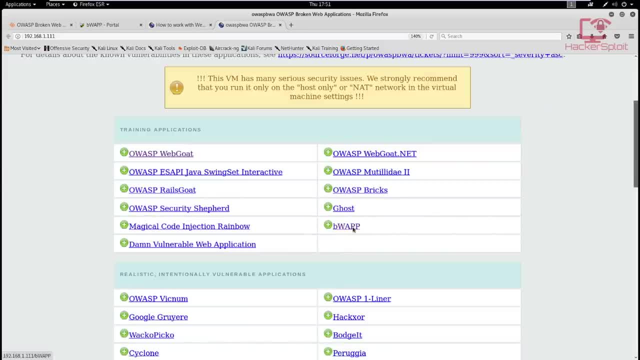 So we will be using web goat and B web or the broken web application project For for this demonstration. So the default credentials for web goat are going to be guessed, for the username and guest, for the password And for B web it should give you the prompt. 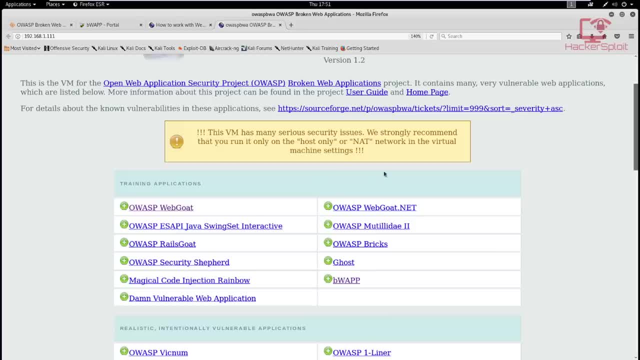 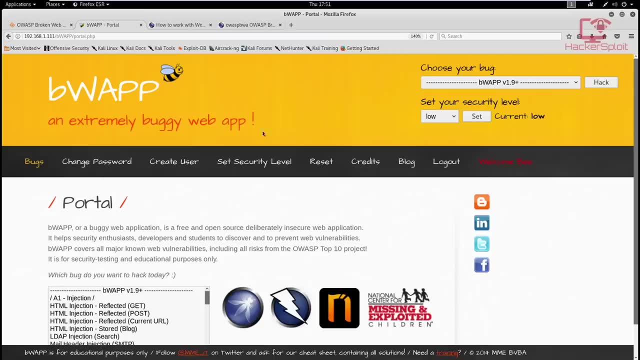 right over there. I think it's going to be a bug app or something like that, But, irregardless, it will tell you what it is. Alright, so make sure you open that up and you have that all set up. So I've logged into B web and I have a web goat started up right here. Alright, so let me. 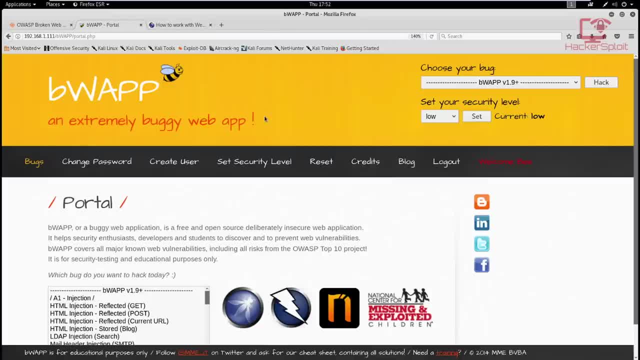 get started, And we are ready to go Now, before we even move on into performing these attacks, it's very important to understand what's going on here with with cross site scripting, what it is, how it works And what are you exactly taking advantage of. All right Now. 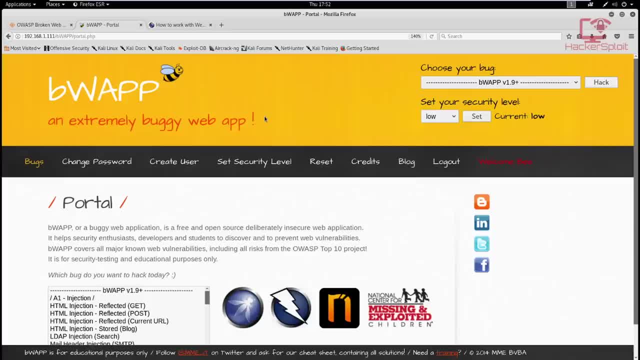 this is where a lot of people make mistakes, And if you want to be a successful web application penetration tester, you need to understand. you know from a fundamental level what's going on here. Alright, so let's get started. What is cross cross site scripting? Well, simply put, it is the 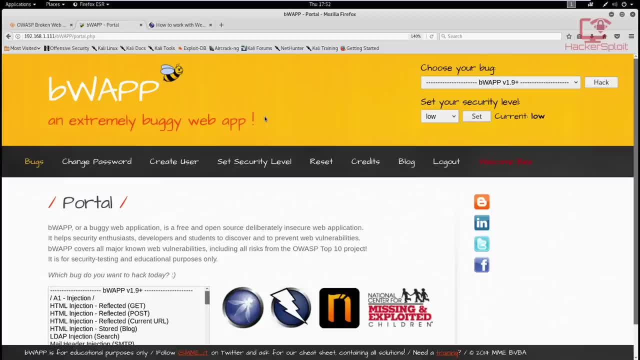 process of injecting a script into a, into the parameter in a URL to attack a user of the site or to potentially attack the server side of of the website or the web application, right? So it essentially is the inject, the injection of a script into the parameter of a URL. All right. 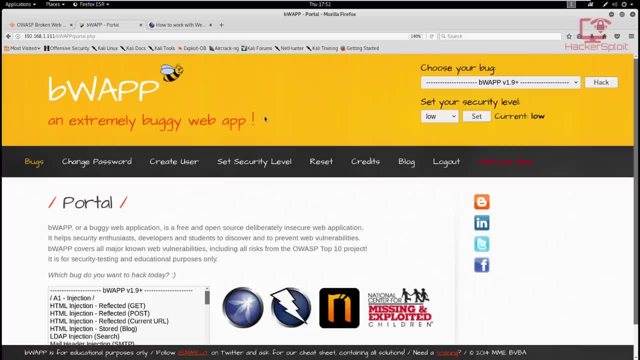 that's essentially what it is Now. of course, this may be quite confusing, but don't worry, I'll explain what's going on here. So let's start off with with first of all explaining the the three types of cross site scripting. All right, the first one is reflected, and then we 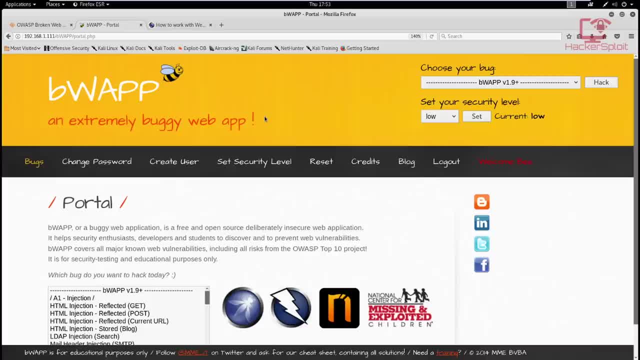 have stored and DOM. So with reflected, what's happening here is the, the data is inputted and then, you know, reflected directly back back on the screen. So I'll explain this in a second. Alright, so if we are to look at this from a fundamental perspective, I'll show you how to. 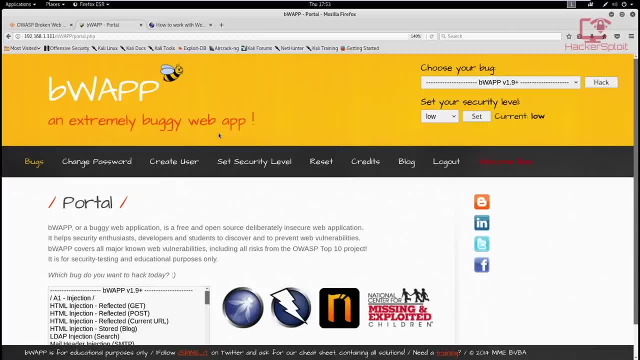 access this. you know how to navigate the view app. just give me a second. let me explain what's going on. So, essentially, what's happening with reflected cross site scripting is that the input is going to be stored in the parameter of the URL. All right, and I'll explain how this differs with. 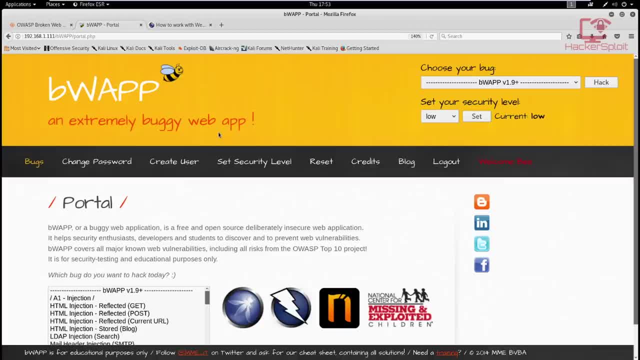 each type of attack, because many of you will point out and say: Well, it's not only to do with parameters, And don't worry, I'll explain all of this. Alright, so we can essentially manipulate the, the parameter of the URL, so that we can essentially run a script. Now, what type of script? 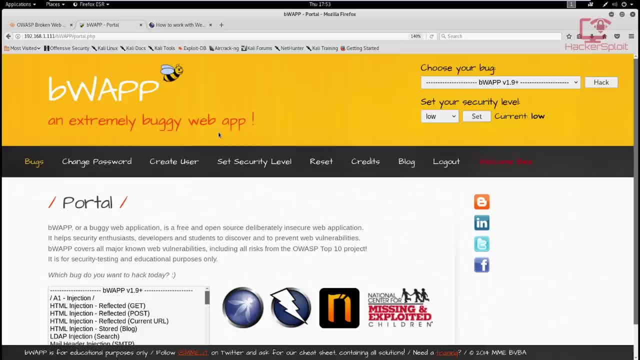 we can run a malicious script that is based in JavaScript And I'll explain that right now. So you can see, with our portal you don't want to touch anything here. you can set the security level, But for now I recommend setting it to low, not that that's going to hurt anyone's ego. 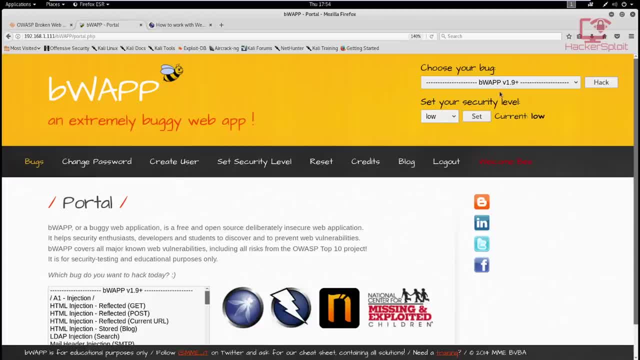 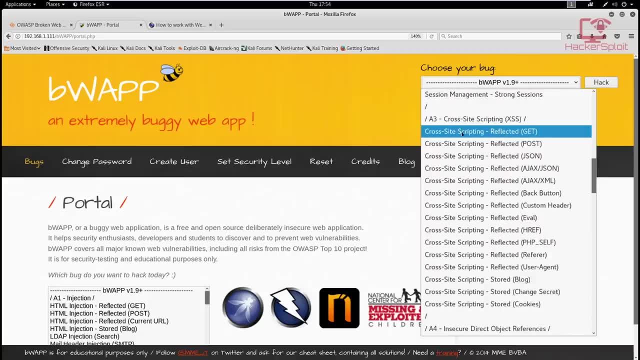 Because, remember, you have to be humble to begin and you need to understand what's going on first. So we will open up the choose, the bug section here And we want to go down into cross site scripting And we want to go into reflected, which essentially deals with the get, the get requests. 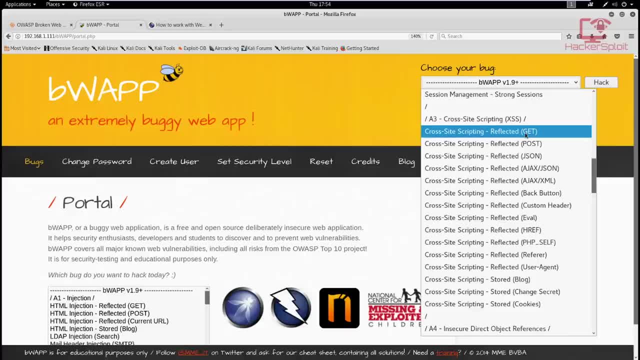 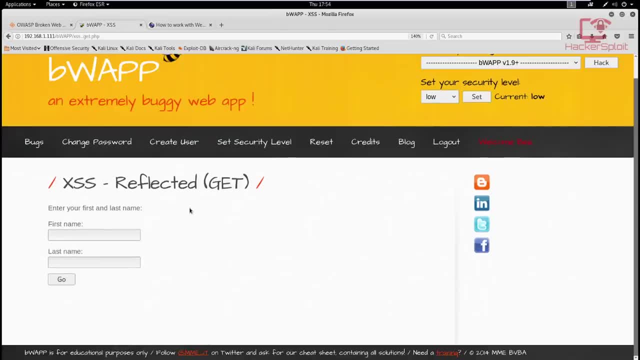 So we're going to start off with that And this will really make you understand what's going on here. So if I click on that and I just hit hack, alright, so now it's going to give us a prompt here And you might be asking: well, what's, what do you mean? What exactly is going on? if I was to 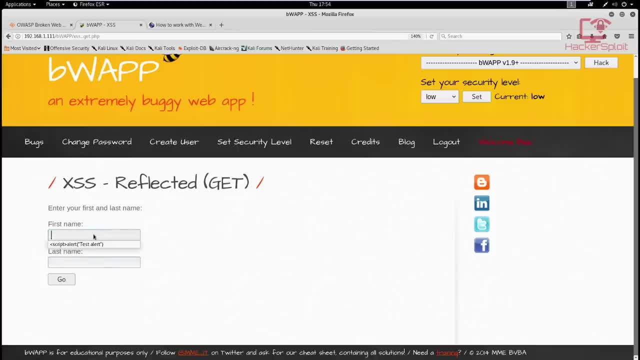 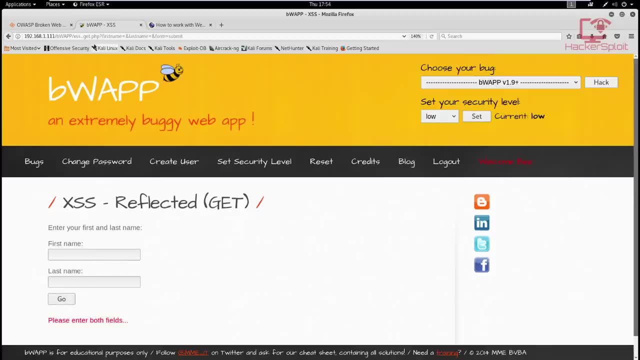 not enter any details into the, you know, into these fields right here. So, for example, you can see I just had a suggestion there. that's because I was testing it out. But if I was to hit go, you can see that in the URL we do have the input here. So you can see the values can be edited. 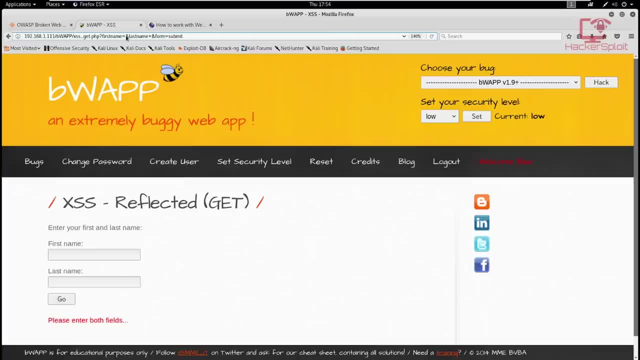 directly into the form. So you can see: first name has the no value, And then we have the last name, which again has no value, And you can see that it is submitting a form. So what we can do is run some JavaScript code in here. 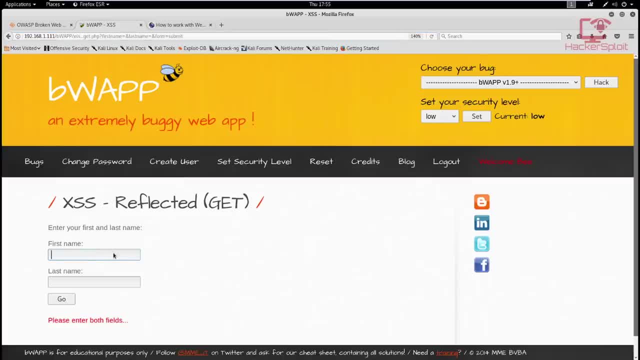 And the most common way of explaining what's going on here, of course, not running a very malicious code right now x essentially explaining and demonstrating that it does work- is- I can run a piece of code here Now, of course, when you put this into a practical perspective, 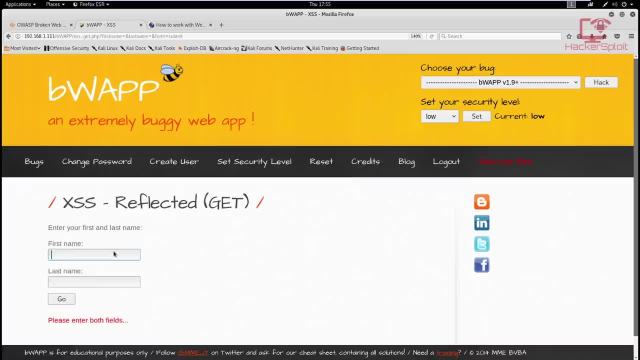 many sites are going to filter the content that you can enter in these fields or the these forms, And we'll, essentially we will not allow you to run JavaScript code. you know, obviously to protect, to protect the site from these type of attacks. But what you can do is 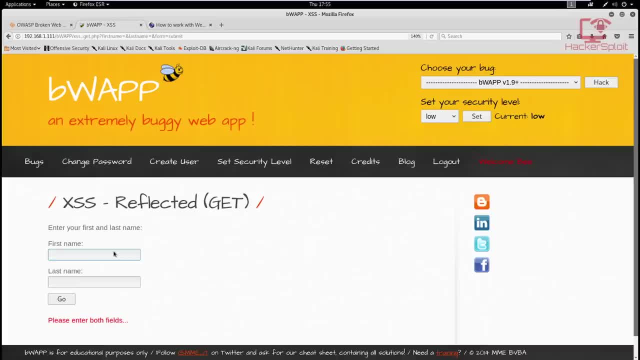 encapsulated, to encode it in a different type of language or, as I said, I'll show you everything or how all of this works. So this, right right now, being the current security level, as low we are, it'll not. it'll not essentially encode, it will not verify or validate what we're entering. 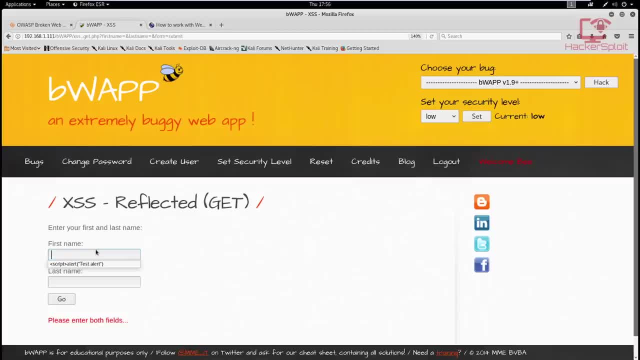 In here what input is being given. So if we were to type in a script here so we can say script and you can see the recommendation, their script, that's mine. So if I was to type in alert, and this is JavaScript, so I'm pretty, I'm pretty sure you can, you know what's going on So we can. 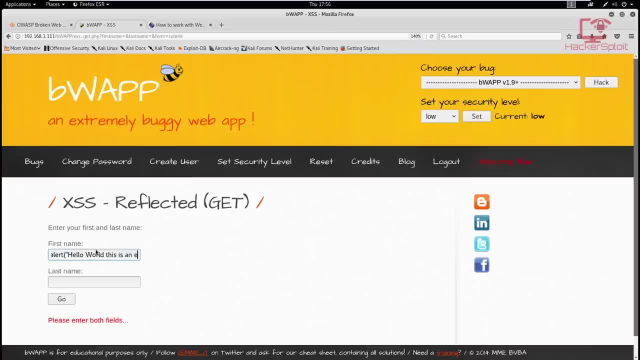 say Hello world. This is an example of reflected XSS or cross site scripting, And we can close that up right now And then we need to close the script, So we can do that in the next field or the next parameter. 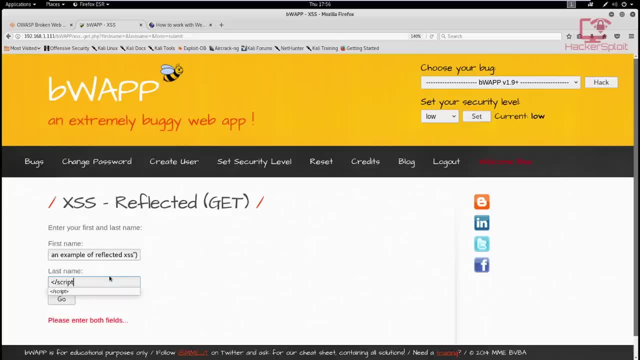 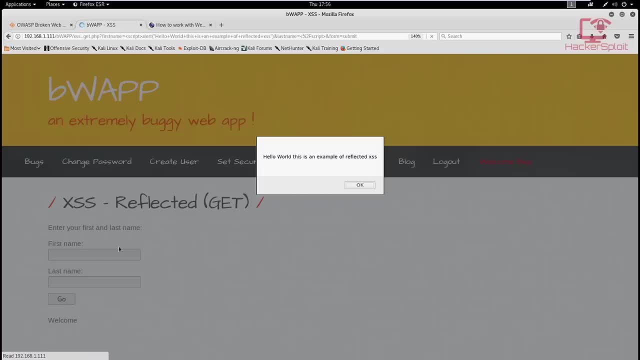 Most people like doing it from the start, But this is just to show you how robust this can be. So I type in, I close the script, then I hit go And, as you can see, it gives us the alert, which is what. 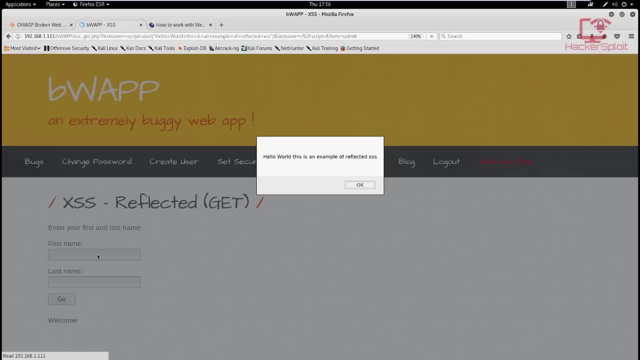 we and we, which is what we used as our form of of me showing you that it does work and it will be processed, the input will be processed and will be sent back to you, you being the client, And we can just hit OK. And that was an example of 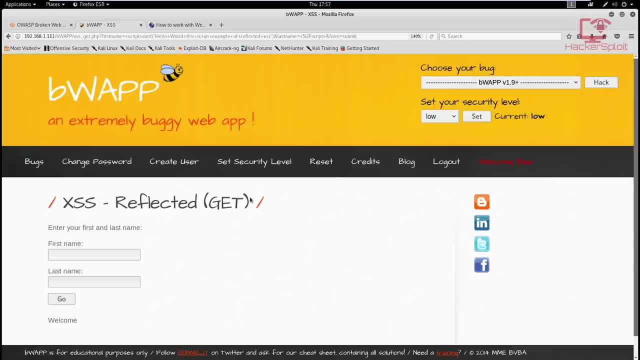 reflected XSS cross site scripting using the get method. Now, of course we can. I can replicate this many, many times using the other types of cross site scripting, for example with the post, etc. etc. we'll be looking at all of that, But for now we need to understand what's going on here. 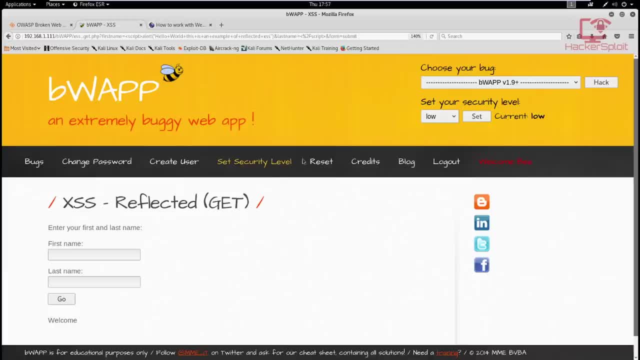 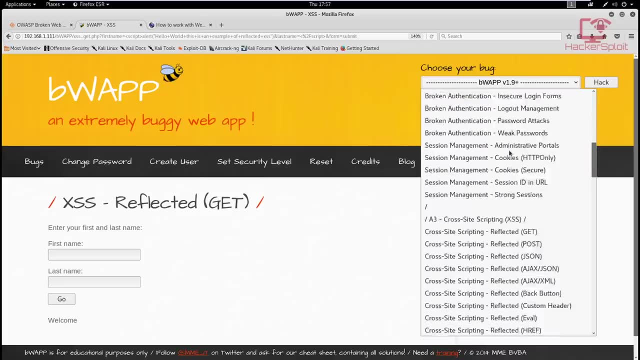 Now. next, we need to look at stored cross site scripting. This is probably my favorite because of the potential that it does have. Alright, so let's go into the choose your bug menu here, And we want to go into cross site scripting And we want to go. 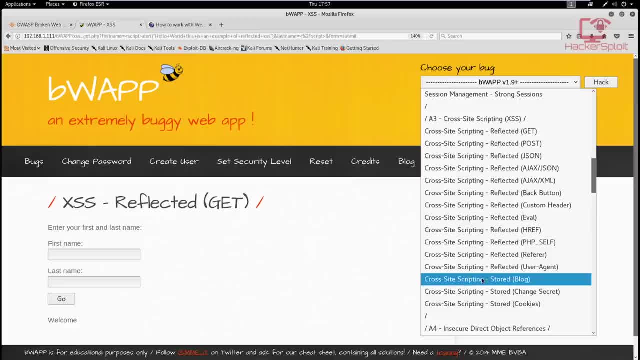 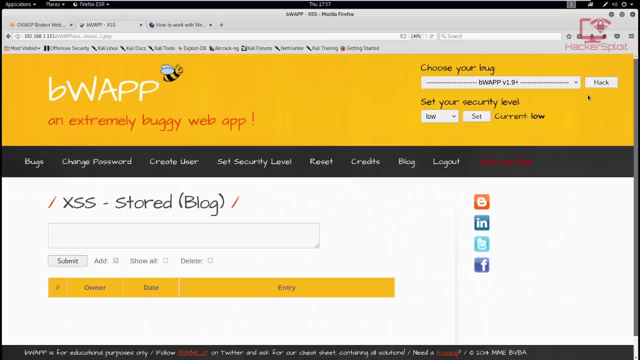 we want to go for the blog cross site scripting, stored cross site scripting, and we're going to select blog and I'll explain why in a second. Alright, so first let me explain what stored cross site scripting is So essentially, with this, with the cross sites scripting attacks, 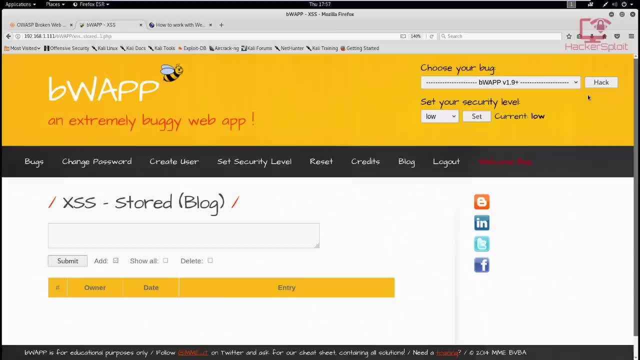 more specifically, the stored attacks. essentially, what's happening is you're attacking the input And you're essentially attacking the input that is to be stored, or you're attacking the data, or, essentially, I like to say, you're attacking the data. you're attacking the data. 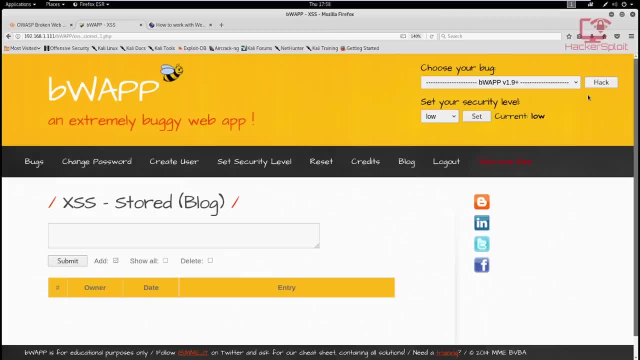 explain this really simply. So you're attacking the input that is to be stored on a database. So what you're doing is you're essentially injecting malicious code that will be saved into a database, or that is going to be saved by the server or the web application server, And then you can. 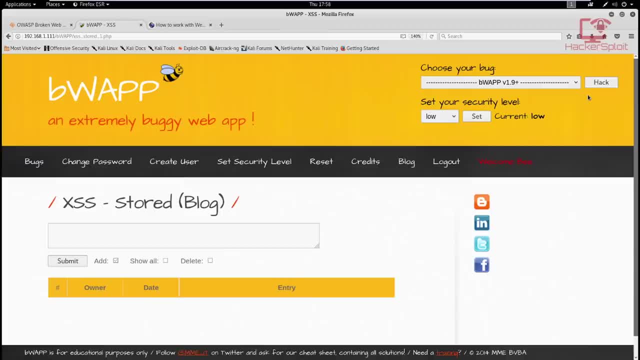 definitely you, since it's being stored, you can access it later on or other users can access it And, for example, if it's running malicious code, it can trigger different things, like opening the webcam of a user, stealing different types of information. I'm not going to go into. 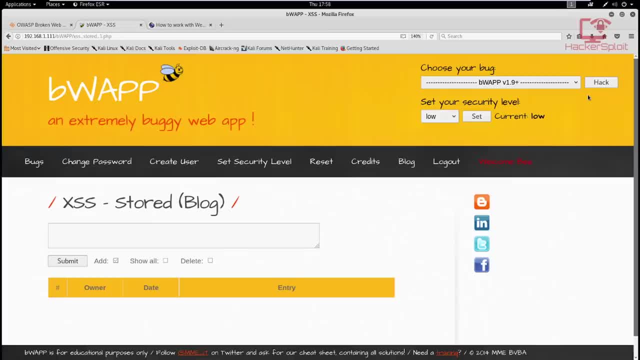 what you can do with it. But you can really do a lot of stuff, a lot of malicious stuff, with code. Alright, so let me explain what's going on here. So, with the stored cross site scripting, you can essentially inject malicious code into the database again. that then that, when accessed, 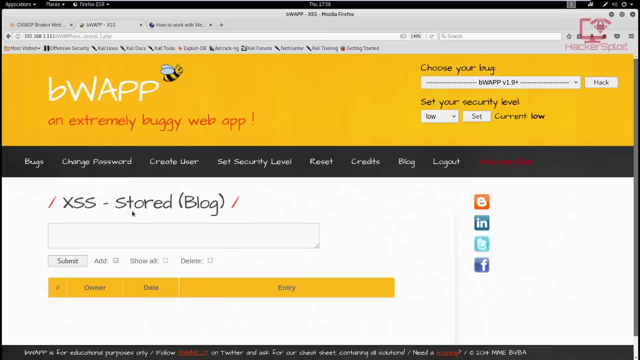 runs this malicious code Alright. so, if you can see, this is an example of a blog. let me explain what I mean. the best places to implement stored cross site scripting is in places like comments, you know, forums and again, as you can see right here, blog in the form of comments that you know. 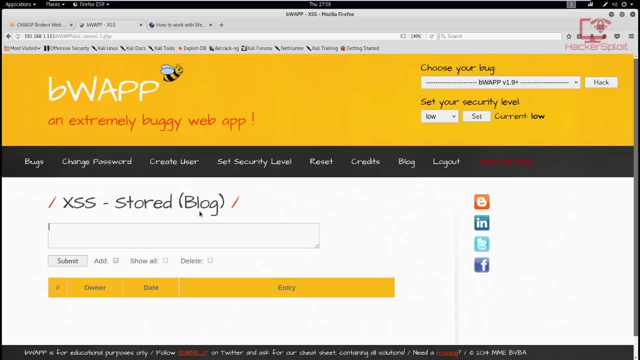 or pages that can be accessed later, or data that is being stored in directly into the database- any database, for that matter, as long as it's being stored, okay. so we can type in here something like hello And we can submit that to the database And you can see it's getting stored. 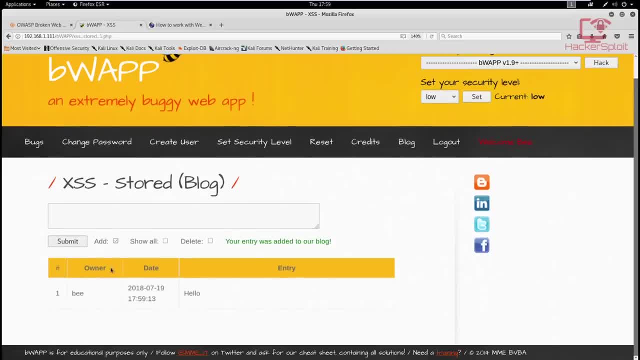 And you have the different tables. you have the, the number, the owner, the date and the entry. So now we can also run a scripting. For example, let's suppose that we have written something like that: we're going to type in the directory and that's going to be stored, So we're going to type in the directory. 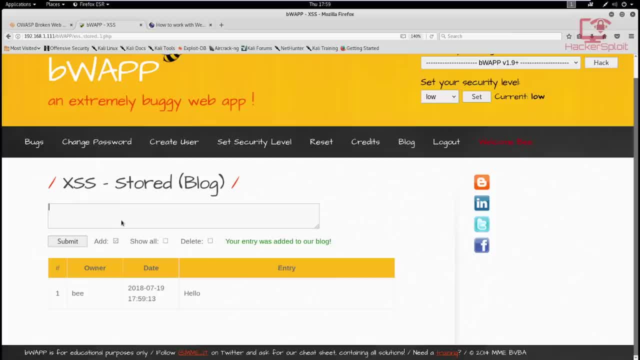 we're going to type in the directory that's going to be stored and then we're going to type in the directory in here, Alright, so what if we were to enter JavaScript and again this data, given our security level, is any of the data that we're entering is not being validated. So you can. 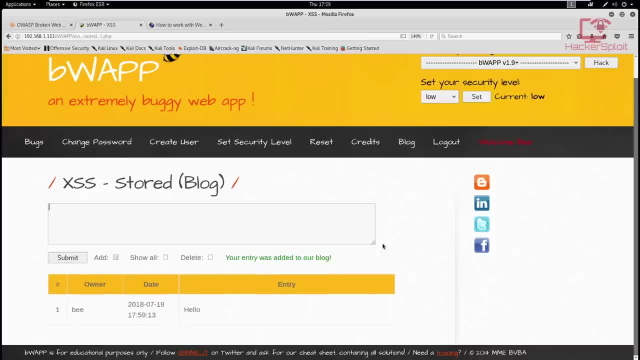 essentially enter it raw. Now, in reality, if you go and try and enter a script in, the data will not be accepted because again, they are protecting their site against that. that's one way of mitigation, very basic. I'm sure you know what I'm talking about, Alright, so enough of me rambling. 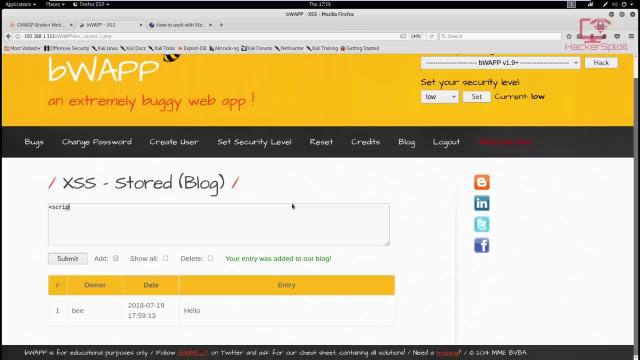 on. So if we are to enter the same script we entered, we are to say script, and we then say alert, for example, we can. you can use any type of JavaScript code you want here And you can experiment. you know you, these web applications are there for you to experiment and test your. 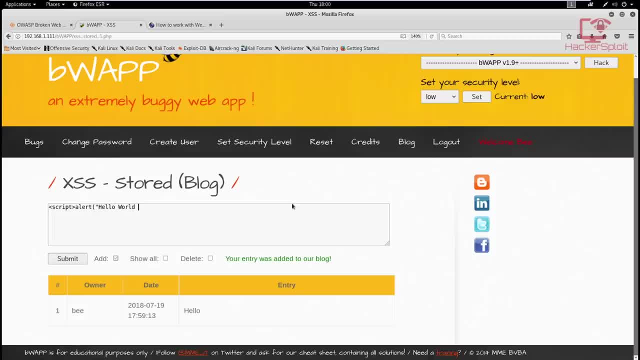 skills out. So for us to say, Hello world, this is stored out, store cross site scripting and we just close that up there. And of course we have to close the script Because we know that that will not execute if we do not code it correctly. Okay, so now we can. we. 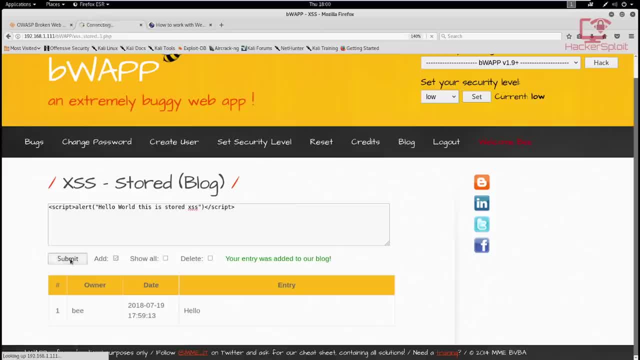 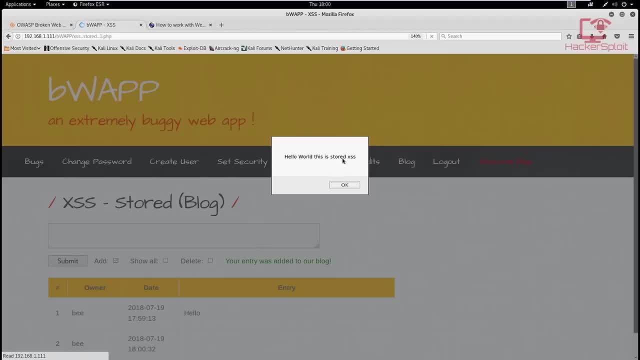 can add that, And if I was to just hit submit right now, you can see that it's going to store and be that being the latest blog post you can see it's going to tell you it's going to execute the script and it's going to say: hello world, this is stored cross site scripting. So an example of a blog. 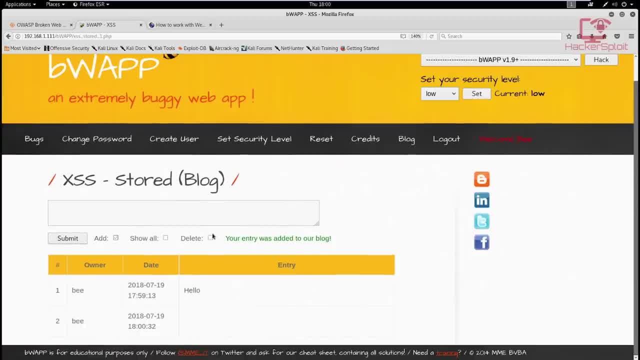 if you're to post this on a page or a, you know, to make a blog post- and inject this script in, anyone who opens that page will essentially run that malicious code, And whatever that code does can then, furthermore, you know, cause damage to the user or to the server, depending on what you want it to do. So 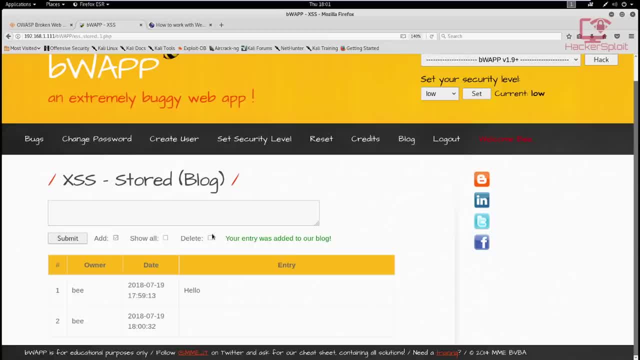 it's all dependent on what the attacker is to do. Remember what I told you in the first video of this series: it's all about your mindset and your, your, your willingness to break things and to find out what does and doesn't work. Okay, so that was an example of stored cross site scripting. 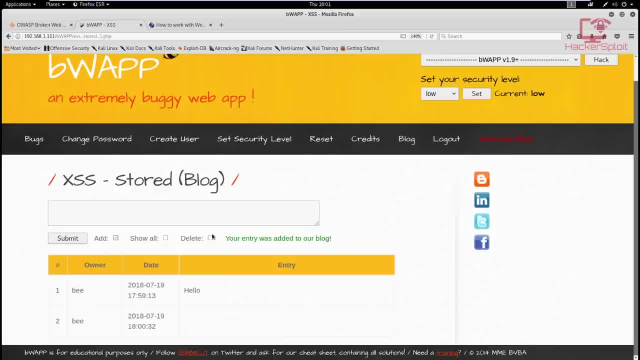 And, as I've mentioned, the most important thing to understand is this: in this scenario, the data is not being validated. if it is being validated- and I'll show you that in a second or probably in the next set of videos, we'll increase the security level And I'll show you. 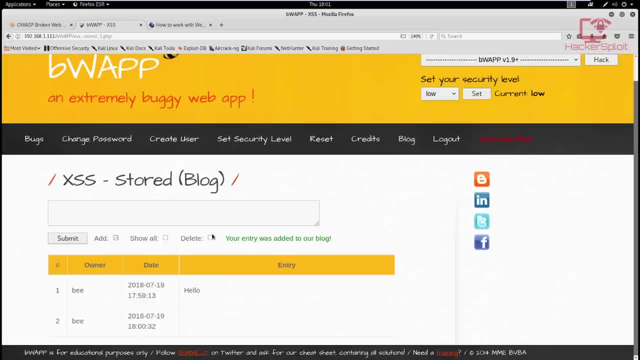 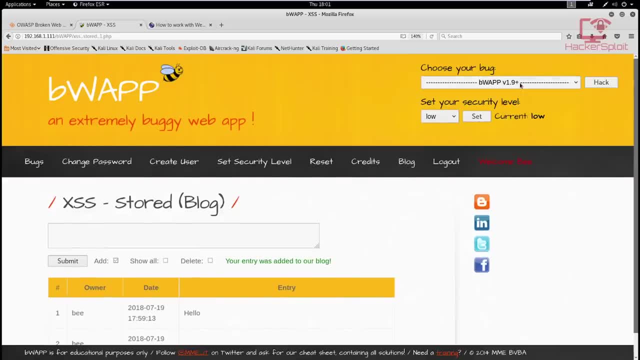 how to get you know past this. you can see how things change as you move along in terms of security levels. So I was going to use the B WAP. This is my first time using it, So I had to get a bit of an introduction. So I had to get a bit of an introduction, So I had to get a bit of an. 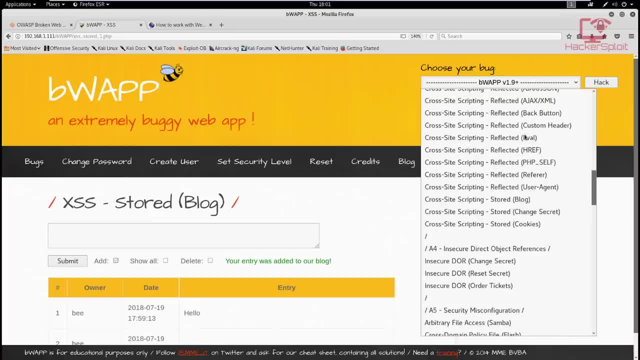 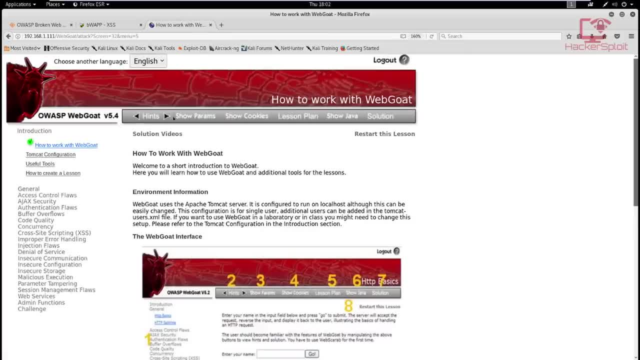 use web goat. they are the only ones I know who actually allow us to run it, So I've zoomed in right now. by the way, the credentials are guest for the username and guest for the password. So essentially I went through cross site scripting And again they didn't have the, the DOM in here. 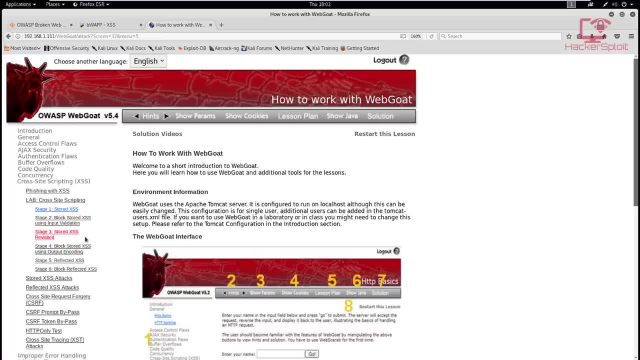 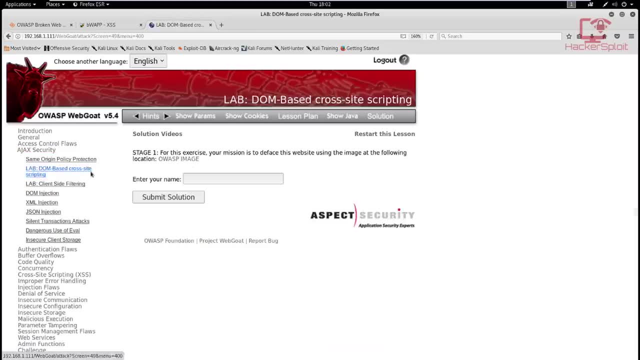 all they were focusing on is stored and again reflected, So I found it to be in the AJAX, or AJAX or whatever you want to call it, and we have the the DOM based cross site scripting. Let me explain why it's saying: this is based in AJAX security. This is: 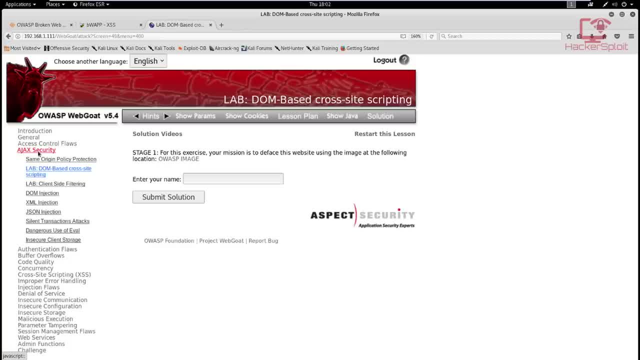 because DOM cross site scripting focuses on the client side, So any data or input that is entered- whether it be a malicious code, etc. etc. is going to be processed by the client, not the server. So any of the attacks will be based, of course, on the client. Now let me explain. 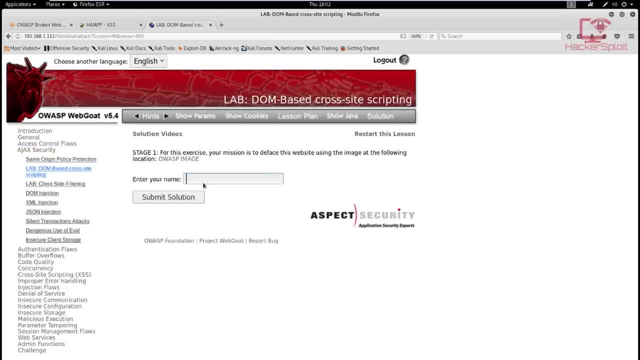 what I mean. If I am to run, remember, JavaScript, server side, client side, I ax, for example. so if I am to run, for example, a JavaScript code in this entry here, so script, and again I type in alert, just being the example, and I say: hello, let's keep that simple And I close. 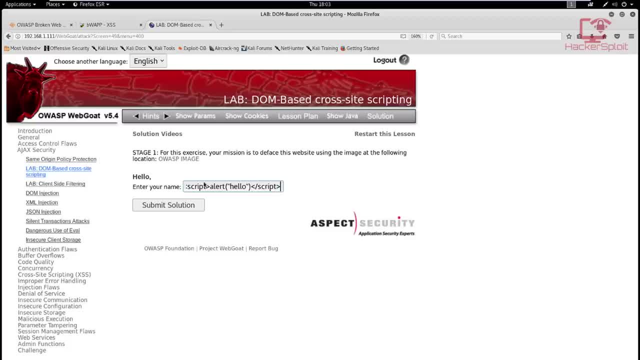 the script here you can see that we will probably not be left with anything- will not get any result. That's because it's being processed by the client, not by the server. So, no, no result or no data will be reflected back to us. If it was, you know if it was reflected cross site. 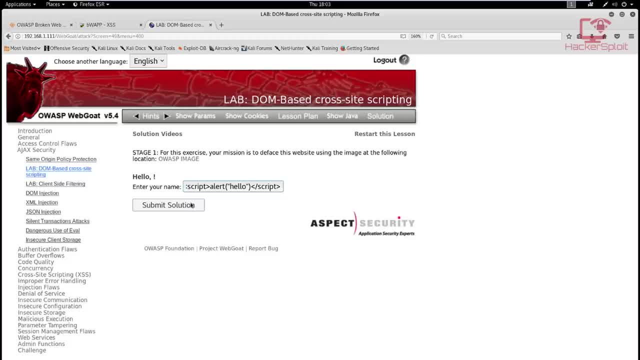 scripting it, the server processes it and then is reflected back to the client. So if I was to submit here, you can see that nothing happens here And that it is going to be taken as code. Now what if we were to enter or use a language that that a client can understand? So let's say 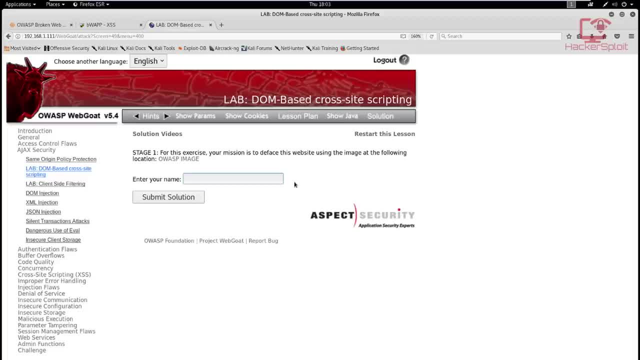 we were to say: let's see HTML. what if we were to use HTML? so again, say in here IMG, for example. that's a very. this is the way we learned it. So I'm GSRC And we 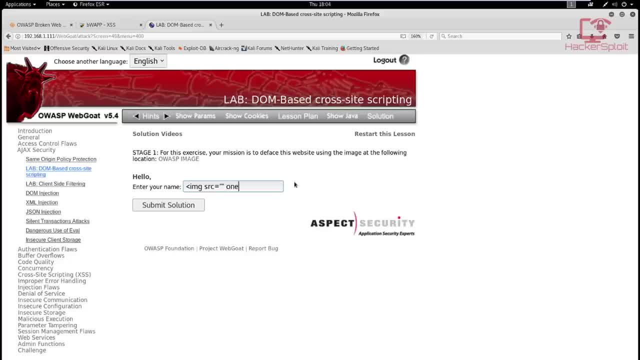 don't have an image source. So we can leave that like that And then we can use the on error in case we get an error of image, which we will get because the image has no source. on error, we can say: that is going to be, that is going to be equal to alert, And then the alert we can then put in. 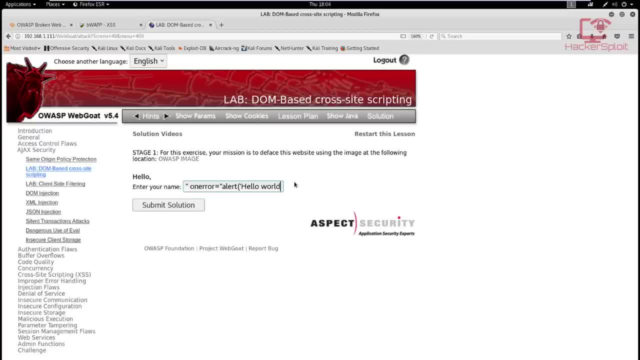 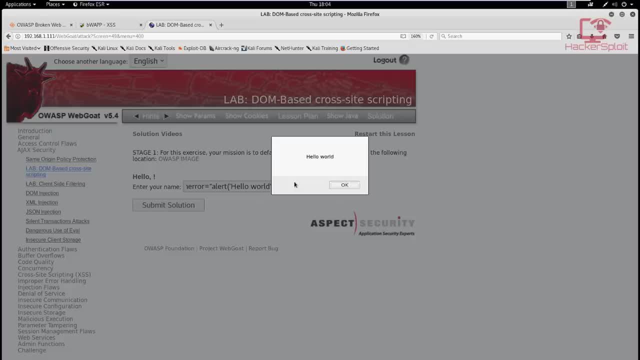 here we can say hello, oops, Hello world, And we can close that up. And once you have closed it, you can see that we can. we can close that there And there you are. So it is going to be processed by the client and you get the. 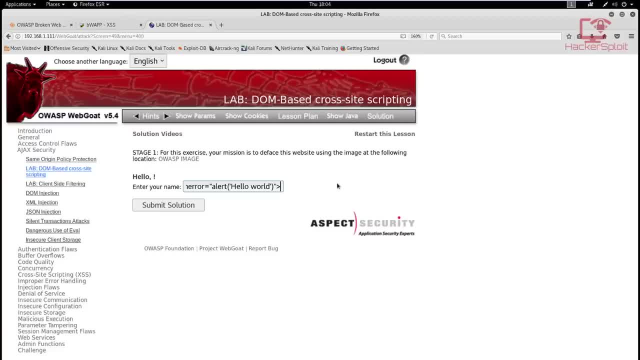 the dialog box or the alert with the message Hello world. So you can see that with DOM based cross site scripting, It is all being processed. all the input, whether it be malicious or not, is being processed by the client, And a X is one of the these languages that can be used, So you can also 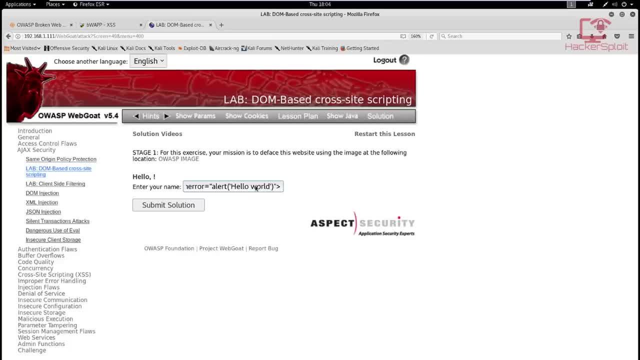 incorporate a X if you wanted to, or test it out. Remember, it's all about experimentation and understanding. I hope that you've got an understanding of what cross site scripting is, how it can be used to manipulate data, whether it be on the client side, on the database, and how you can. 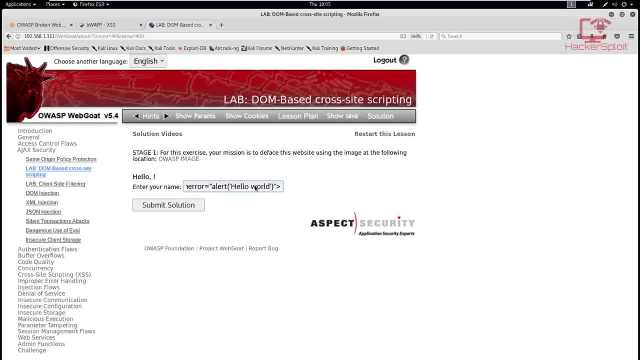 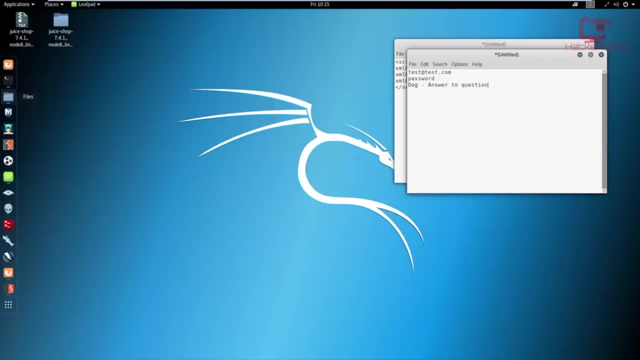 easily just transfer data with, you know, bad security in place. Of course, this is the. these attacks will be very uncommon now, But again, this was focused on more on an explanation point of view. You are going to be looking at cross site request forgery, or CSRF. Now this is an extremely 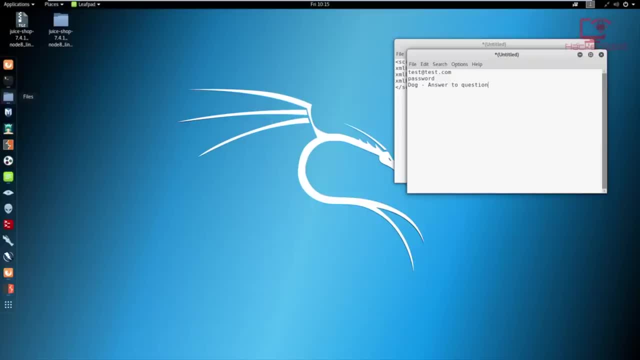 important topic, and a big one, that I cover it correctly. So, for the purpose of this video, I've set up a very unique environment that in, at least in my opinion, will demonstrate how to utilize or how to perform this attack. All right, now I'm just going to give you a brief overview of the 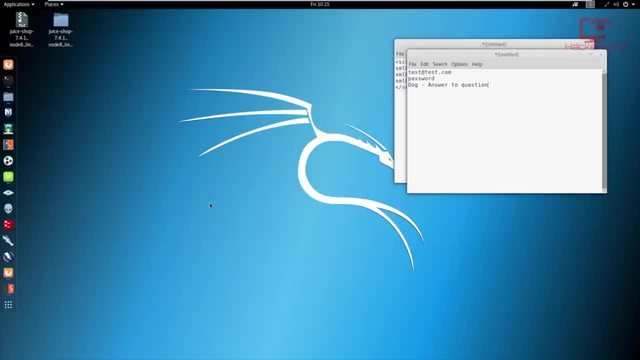 environment that I have Now. of course you can see I have a few files open here. Don't worry about them right now. Just just remember that we'll be using them later on And I'll be using them really, really well to explain. 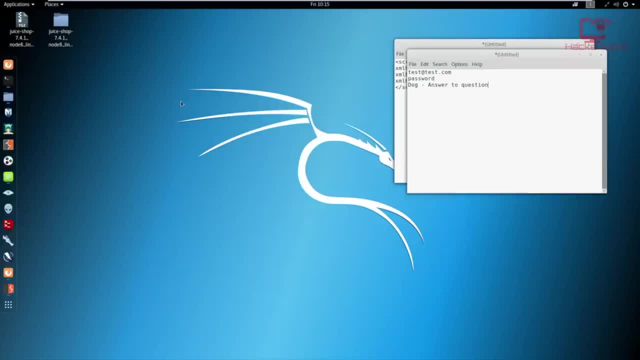 what's going on here So you can see as my target or as my vulnerable system, I'm going to be using my vulnerable web application. I should say I'm going to be using the OS juice shop. Now, not actually, no one actually recommended this to me, But I remember that I performed this during a CTF challenge, that I 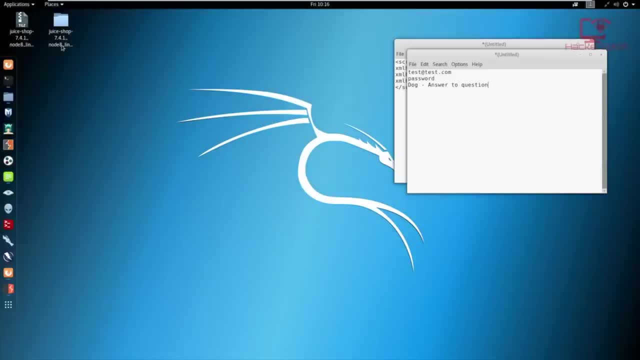 went to earlier, I think late last year, I'm not too sure exactly when, but the whole process was involved with exploiting this web application All right, And in my opinion this really outlined or really showed off how to perform all of these various 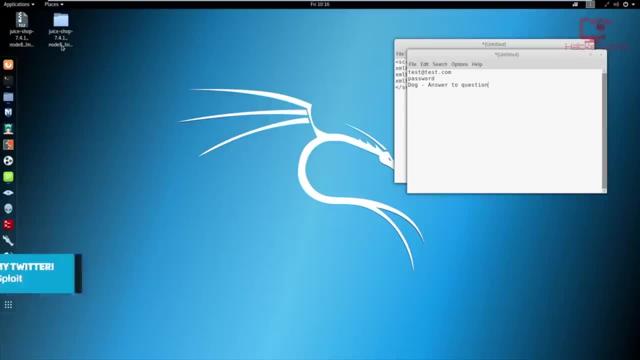 web application attacks. In this case, we're going to be focusing on cross site request forgery. All right, so I have the juice shop running. It's. it's based on nodejs And it's running on my local host. 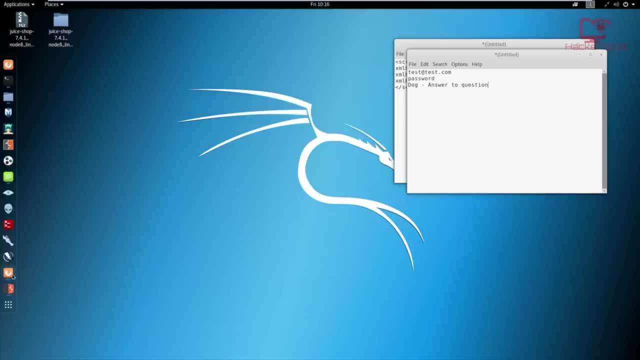 Let me just show you that right now. There we are. So I haven't logged in or done anything yet, And that's I'm going to do that with you. So I've set it up. it's running on my local host. Let's get started with this. 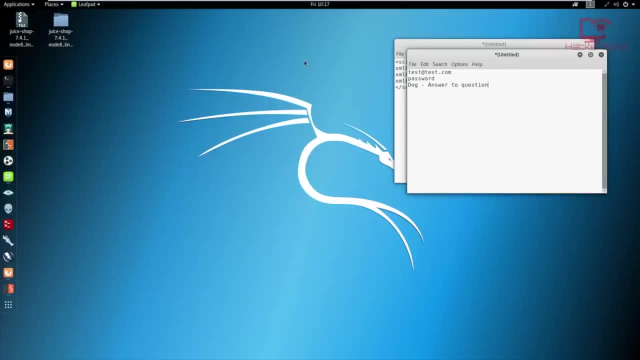 really really simple but sometimes complicated topic. Alright, so cross site request forgery- CSRF. Now, from the name you can already tell that it's split into two, into two sections. you have your cross site and your request forgery, So from that we can get a basic example of what's going on. here. we have cross site scripting and 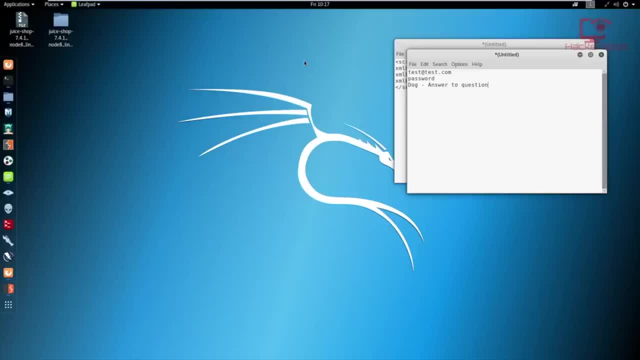 we are going to be forging requests or we are going to be manipulating requests. Hmm, interesting. So we are. we are kind of understanding what's going on here. Now, the technical explanation for what CSRF is is: it is an attack. 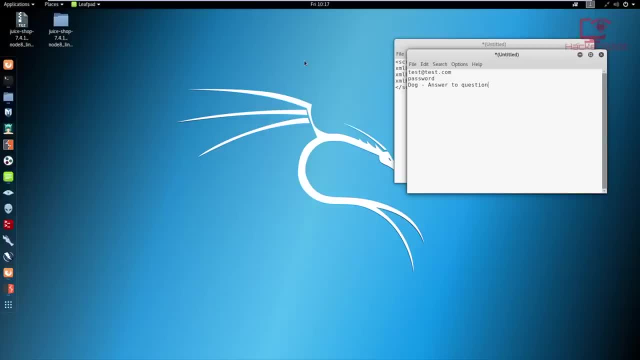 that forces an end user to executed unwanted actions on a web application in which they are currently authenticated. Alright, so let me put that really, really simply, right, it's an attack that will force an end user to execute unwanted actions on a web, on a web application. these actions can be anything, But in this case we're going to be. 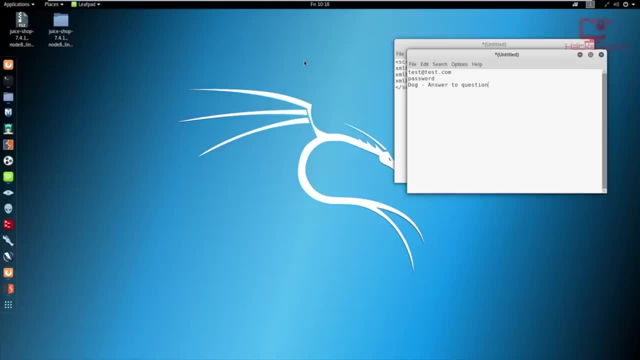 looking at changing the password, And they have to be currently authenticated to that web application, which which means they have to be logged in to that web application for this to work, Because if they're logged out then you get the idea it really doesn't help or it doesn't work Alright. so we use cross site scripting in this case to perform the 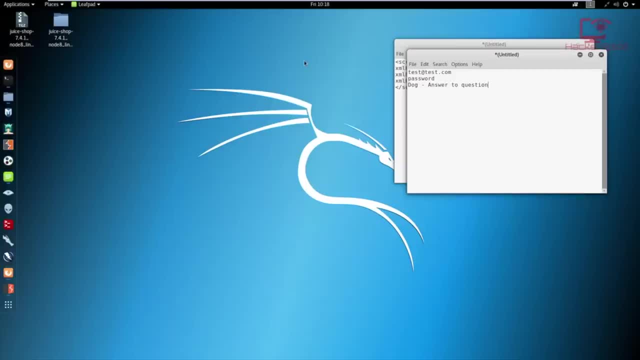 request forgery and to get either desired or undesired results. In our case, we're going to be looking at how to to change the password of any user that's logged into the to this web application. And how will we? how will we be doing that? Well, we are going to be using CSRF, But the first thing you need to 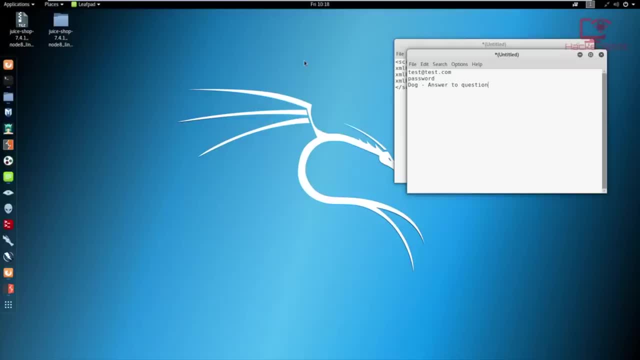 understand is how an HTML form works. All right, And this is very important because, first of all, a client will request a page from a server. All right, the server will then respond and give the, the client, the HTML form. The client will then send back the, the form with the data, back to the server. the server will then authenticate and 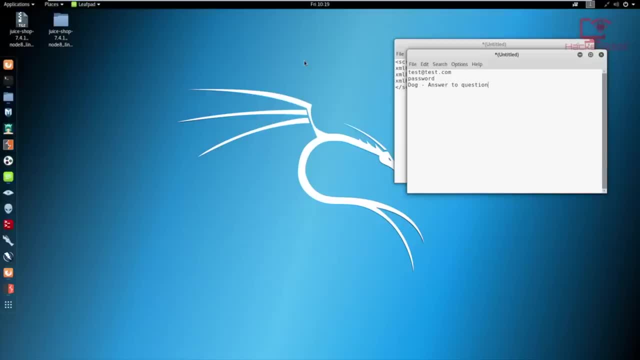 authorize the user and then will will perform the requested action And, based on the request and the response, we are able to forge or to change the request and get a desired response. if you're looking at it from an attacker's perspective, All right. so 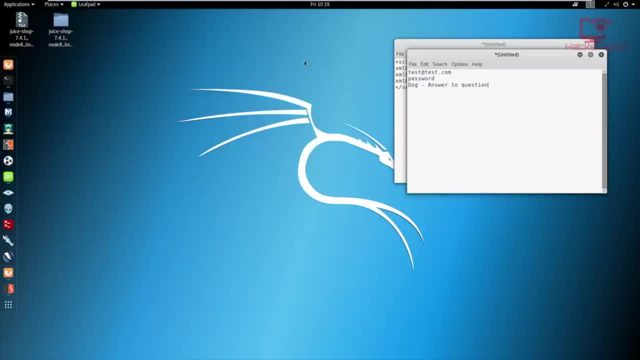 the way CRS, CS, CSRF works. sorry about that. That is, the attacker will manipulate the victim into submitting the attackers form data to the victims web server- essentially, essentially performing these, these requests. In our case, as I've mentioned, it will allow us to change the password of any user on. 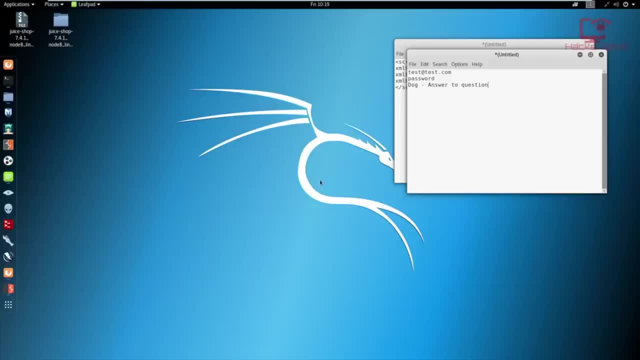 this web application, In this case the OS juice shop web application. All right, So now you might be asking: well, if I'm a bug bounty hunter or I'm practicing to become a bug bounty hunter, how do I go about? 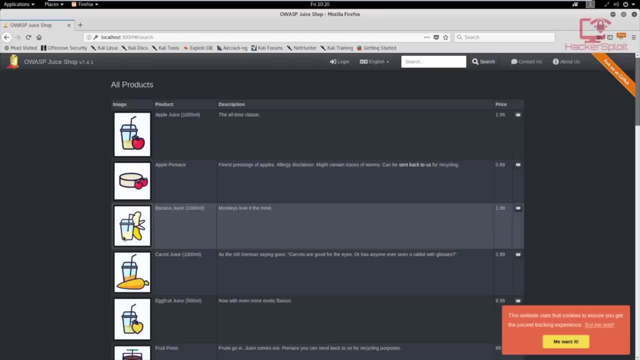 finding this vulnerability? Well, that's a very good question And that is the question you should be asking yourself when performing any penetration test. Now, coming back to my environment, I'm running burp suite, the Community Edition. you you'll just need the. 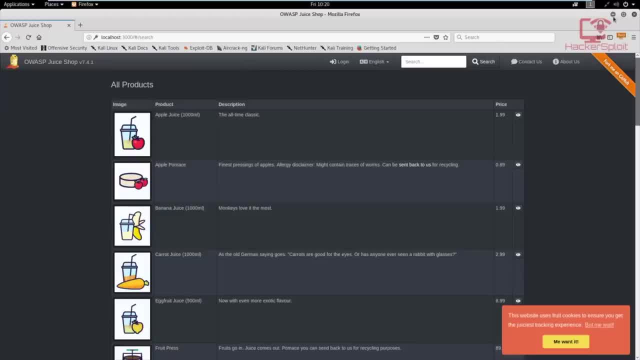 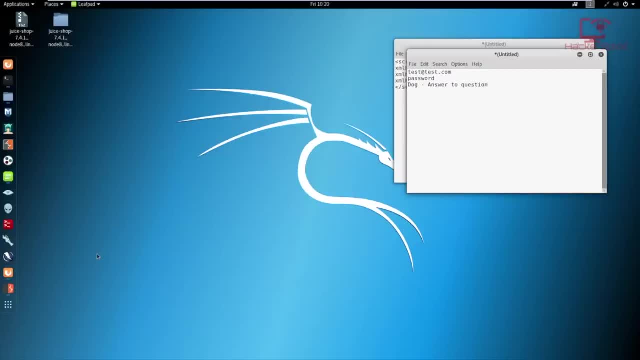 Community Edition For this one. we're not performing any advanced techniques here, because we're essentially just changing. We're just going to be changing the request to get our desired responses. But once we move on to the advanced stuff, I'll then be using OS. 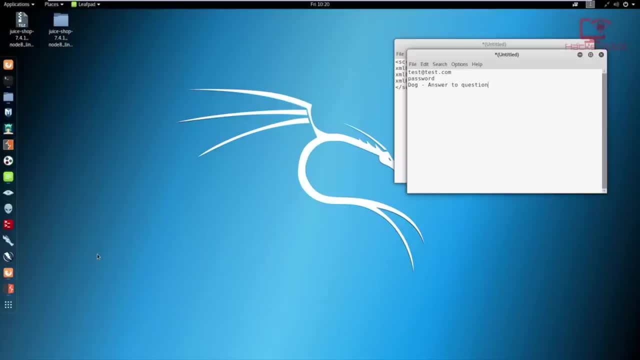 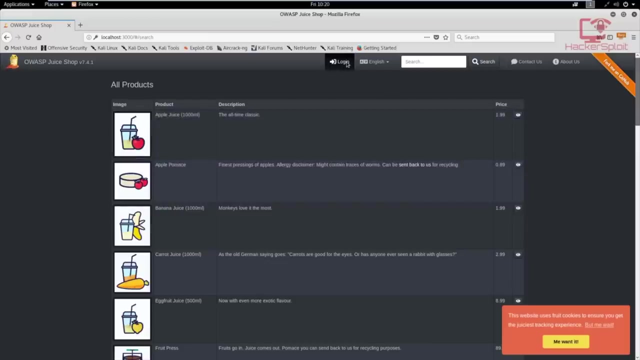 zap for our attacks. Alright, so, keeping things really, really simple, we the way to look for these vulnerabilities is to target the login pages, which we have right here. we then need to. we can then create the account and login And then, finally, we will be creating. 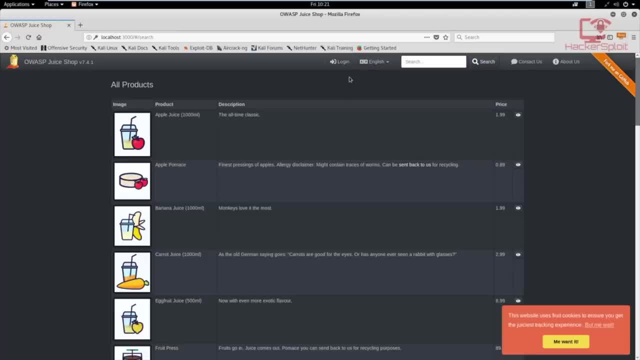 our own, our own script to perform the cross site scripting, And that will allow us to submit the data. or, if we send the URL to another user of this web application who is currently authenticated, it will allow the, it will allow us to make them change their password And then we can log into their account. Alright. so this? 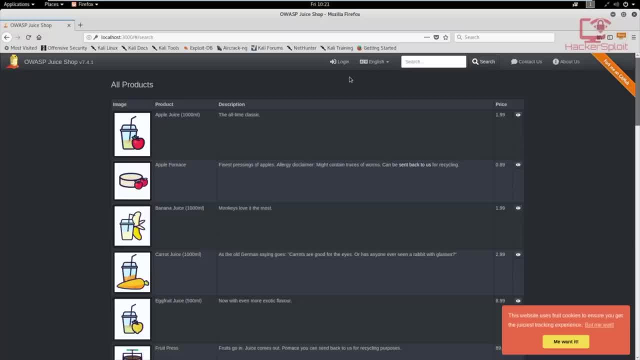 vulnerability is very common on sites with accounts. you know, sites that have emails, passwords And, as you probably would have guessed, there are a lot of sites that utilize this functionality. But remember, most of the sites out there will be protected from. 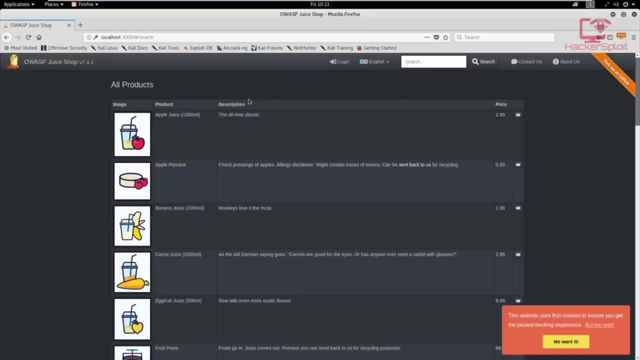 this vulnerability, So it's up to you to find these vulnerabilities. Alright, so, as I've mentioned, we will be using OS juice shop as our target, And the reason is is because it will explain what I want to explain really, really well, All right, and we'll be using the burp suite. 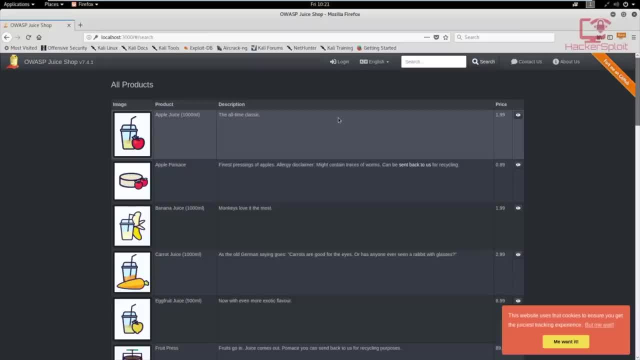 community edition. Now, as you can see, I'm currently running the burp proxy. I'm not intercepting any traffic. if I open up burp suite, I'm not intercepting any traffic. if I go to the proxy and intercept, I'm not intercepting anything. So it's currently just I'm just going. 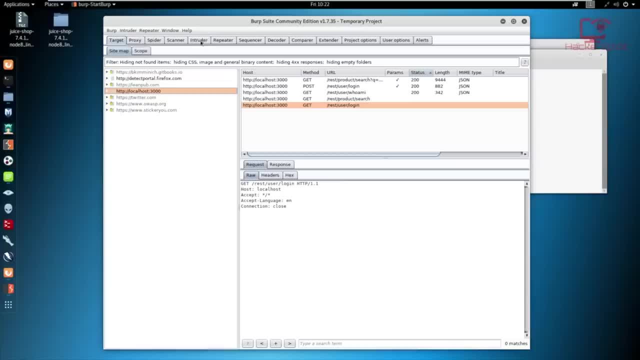 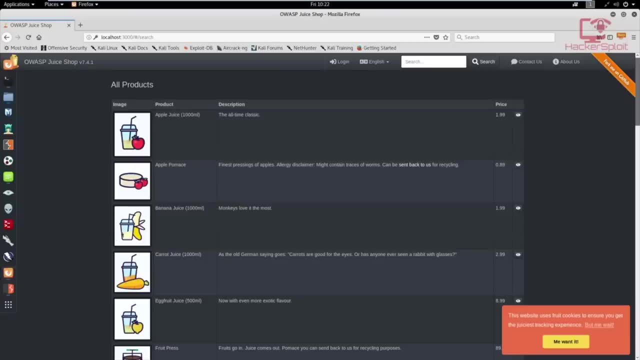 through the burp proxy and all traffic and data is being logged through the burp proxy. So when it comes down to this little data that I've saved here, I've already created an account. The reason I've done that is to save time, because I don't 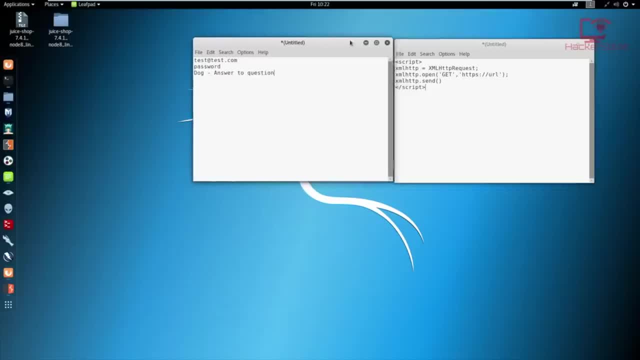 want to explain everything about it. So I've created, I've created a user with the email of test at testcom And a password of password. So really simple. Again, there's nothing really complicated here. And if you want, if you're wondering what exactly does, 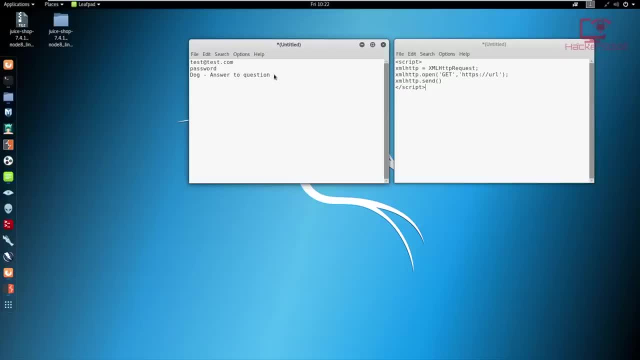 this mean? Well, this is a security question with the answer. So the the question was: what's my favorite pet? And I wrote in dog, So hopefully that doesn't scare you into thinking that I've gone completely crazy. And then in here we have the script. that will be. 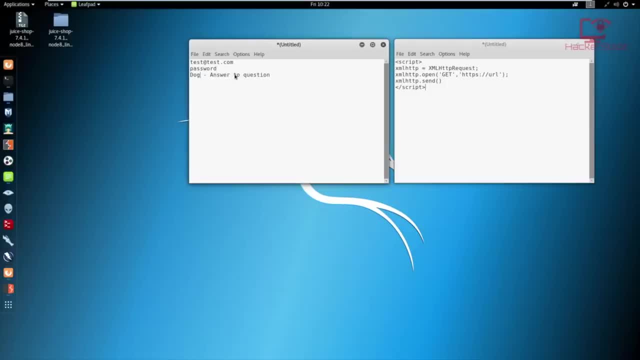 using or will be utilizing to perform the CSRF on the site. I'll get to this in a second. We don't need that right now. So if I want to log in, I know that the, the email is test at testcom And the password is password. Alright, so let me do that right now. we need 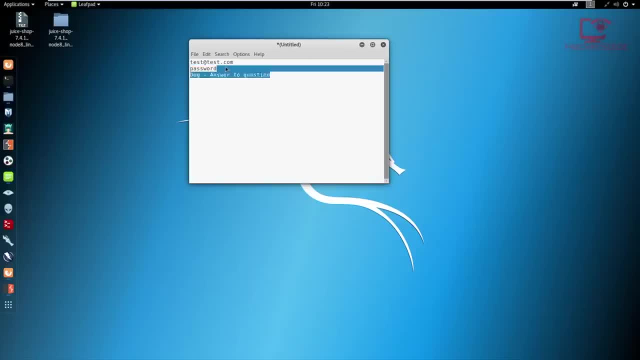 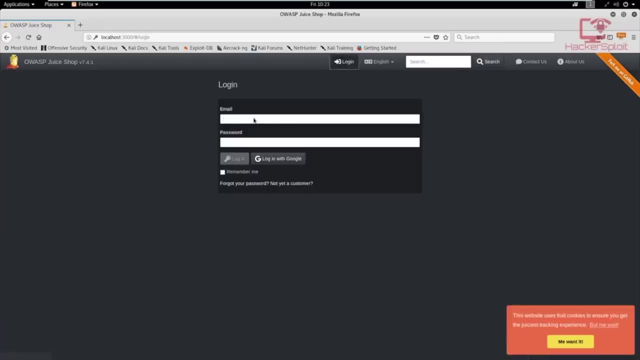 to authenticate. So let me log in, like so, And I'm going to hit test at testcom, All right. so let me do that. All right so now, and I'm going to write the password, which is password, and I'm going to hit login, Alright. 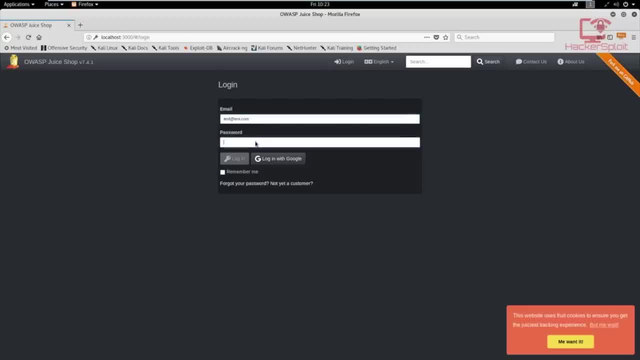 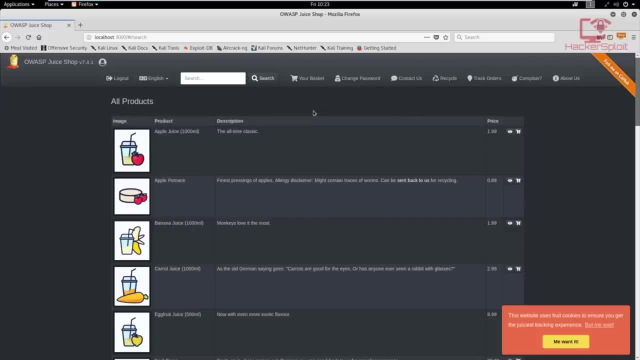 and I'm don't want to save the password, And they also have logged in now. Now, as I said, this is very. this vulnerability works really really well when you're talking about changing passwords because, as you can probably guess, an attacker would would be looking to exploit this. 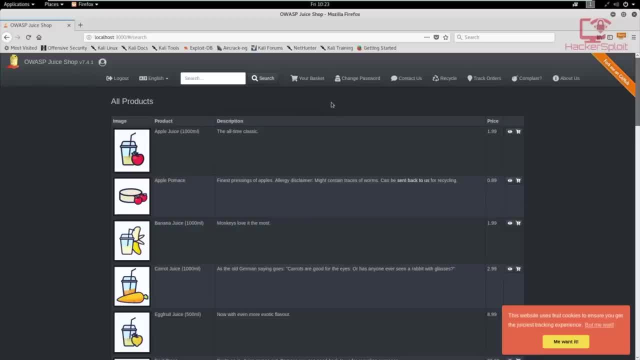 functionality, Because imagine if we were able to send a request to get request to our target with the URL, encoded URL. of course, we can also use link shorteners if we wanted to do that And, essentially, if they authenticated it, it will allow us to make them change their password. 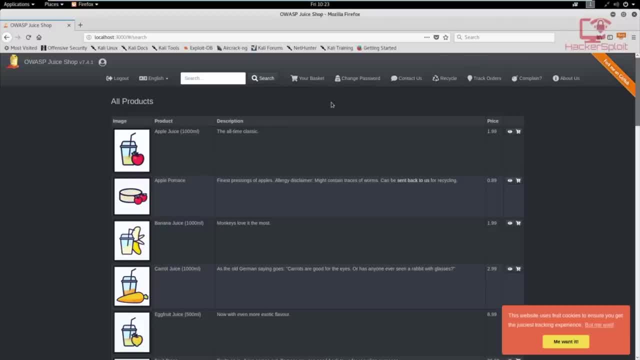 simply by clicking on the link changing the password to whatever we specify. Alright, so how do we do this? Well, the first thing we need to do is we need to look at how the get requests are being sent, And we can do that using burp. So we are just going to change our password. 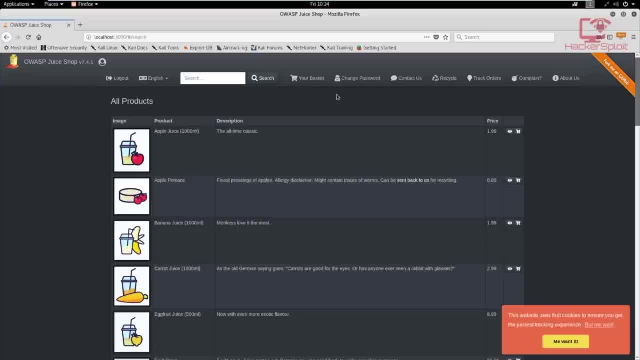 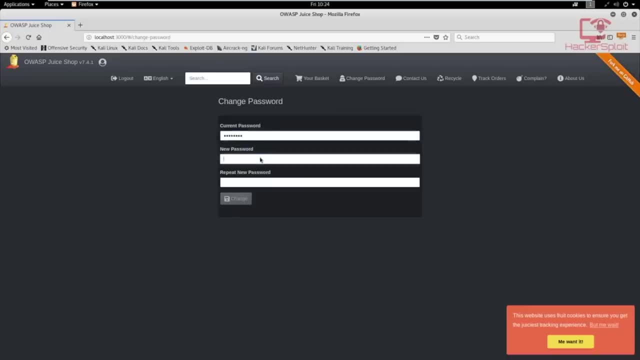 So our current password is password, And what I'm going to do is I'm going to change my password into password- Oops, sorry, Password 123. And I'm going to repeat it. So pass word 123. And I'm going to change Alright. 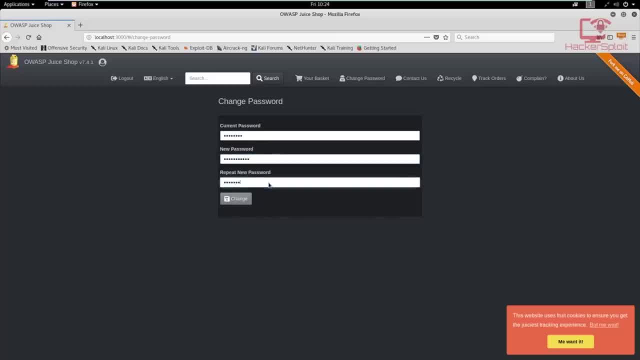 so the password was successfully changed. Okay, now let's look at how this was processed in burp, or how the request was sent in burp. So I'm going to go into burp, our proxy and HTTP history, And I'm going to go all the way to the bottom And, as you can see, we have the get request right over. 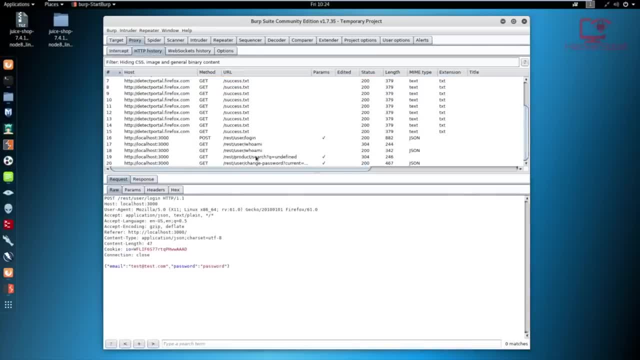 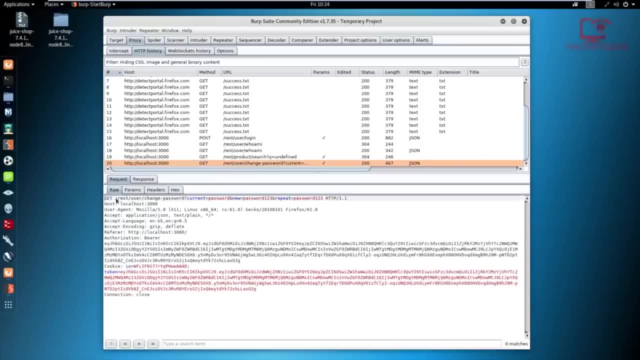 here. Okay, so the get request is very interesting. you can see we have the get request and it's targeting the. the following URL: And these are the parameters. So change password. the current password is password. new password: 123.. And we've repeated it. Alright, so now let us perform the. 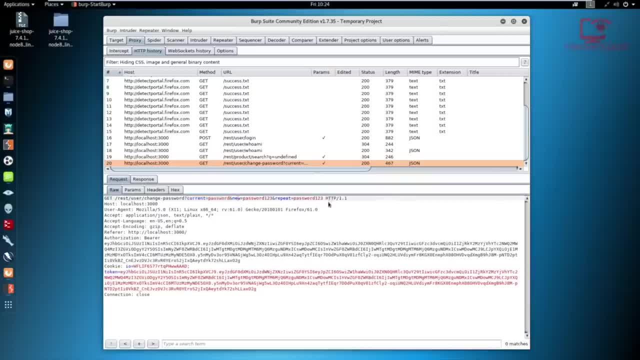 forgery here. So I'm going to send this in to the repeater. Alright, so I'm going to click on repeater And in here we can manipulate the request and see what responses we get. Alright, in case you, you did not know about that. But again, let's start off really, really simply, So. 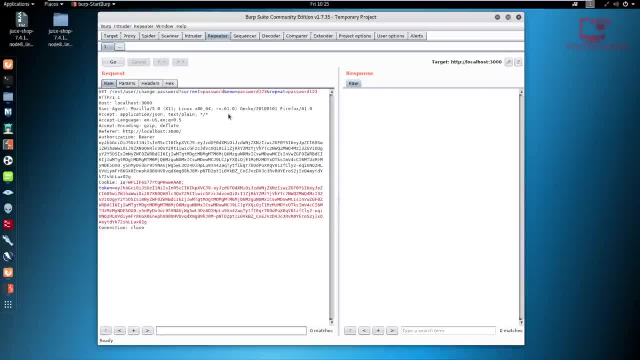 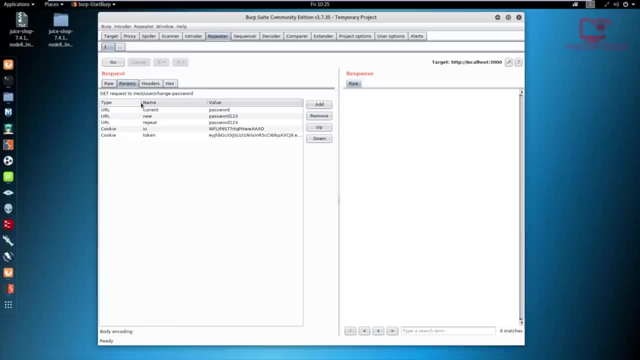 we are going to be working with the raw request. we don't want to work with individual parameters- although you could change it- but we are going to be manipulating the request entirely so that it performs what we want to do. Alright, so what we can do first is: we can test, So let's change. 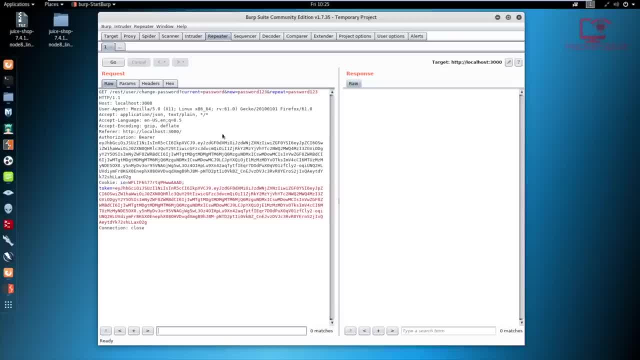 what if we were to change the current password to something like: let's see test, let's change it to test And then we hit go. you can see that the response we get is a is a 401 error, which means we. 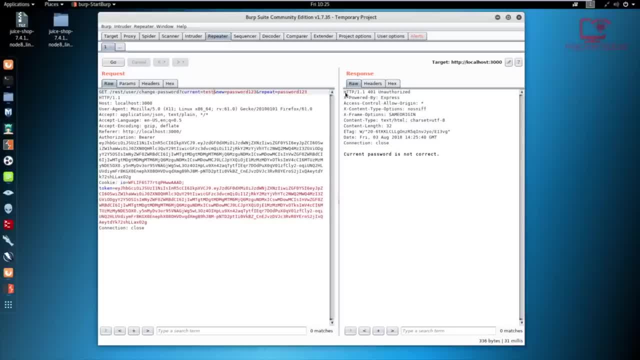 are an authorized user, And then we hit go And then we hit test, And then we hit test, And then we hit make that, and it will give you the message right here: The current password is not correct. All right, that's good. That is good from a web application perspective, which means that this: 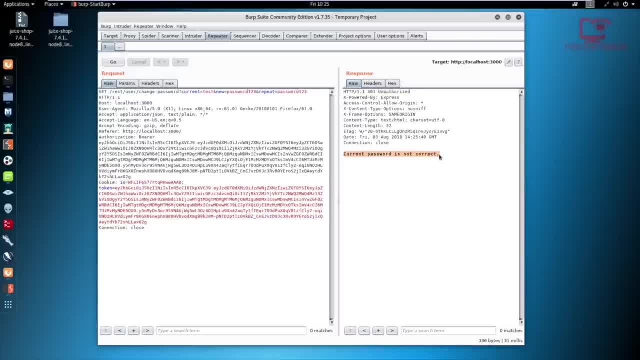 web application is performing validation And it's not going to allow us to not to just go in and start manipulating any requests and making changes. So from a security perspective, the web application is doing really, really well, All right. What if I was to change the new password? 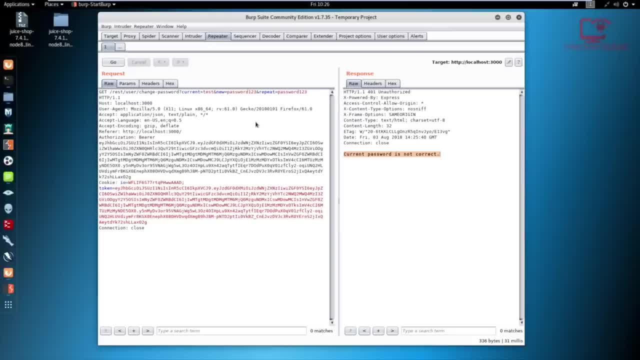 Let me change this back to password, to the current password. So let me change this back to password, to the current password, which is what we set, And I changed the new password to password pass 123.. All right, and I hit go Again. we get another run again, the 401 unauthorized error telling us. 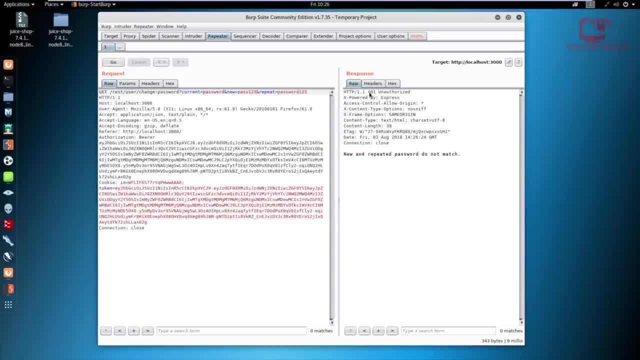 that the new and repeated password do not match. So, yes, the current password is correct And the the only thing that we're getting an error is the new password and the repeated password are not correct. So interesting. what if we want to change the password into password one, two? 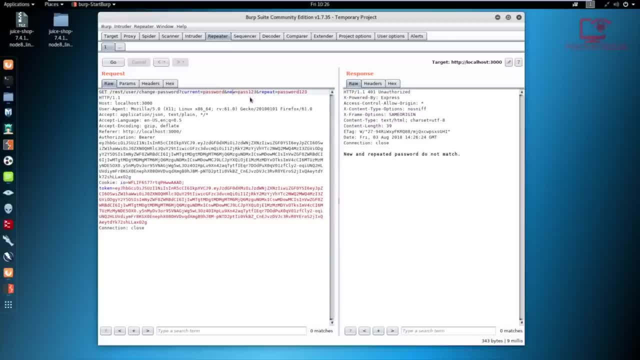 three and we can repeat that again. So we want to confirm this, or password 123.. Actually, hold on. So I'm going to say password 123.. And now let's see what this tells us. this should verify it, But 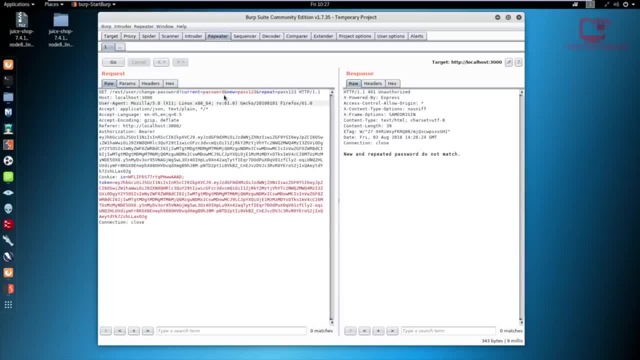 let's see if this works, So you can see. yes, that does work, And we know that this works because that's what we did. That was the original request. But what if we do not know the current password of the user? Remember, we're going to be targeting other users of this web application, So 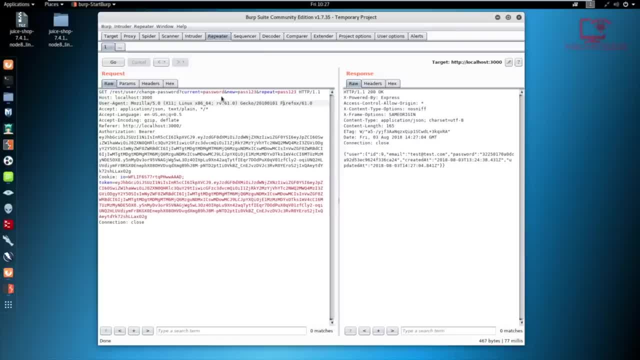 what if we get rid of? and this is very, very this is the way penetration testers go about it- what if we get rid of stuff? So what if we get rid of the current password? All right, and now essentially, the get is targeting change password, with the question mark here essentially requesting 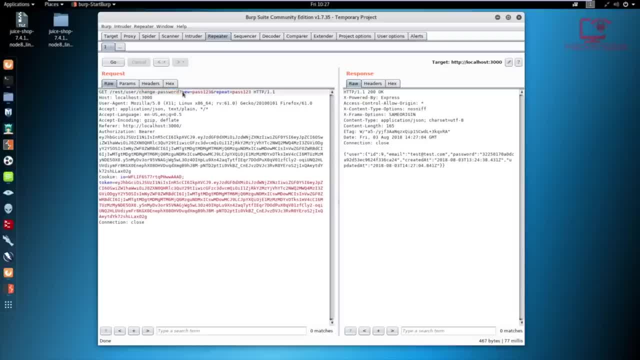 and we're only entering the fields or parameters new and repeat. what if we do that and we change them to password 123.. I mean pass 123 and pass 123.. Let me go, you can see. yes, it does work. We get the 200, the 200. 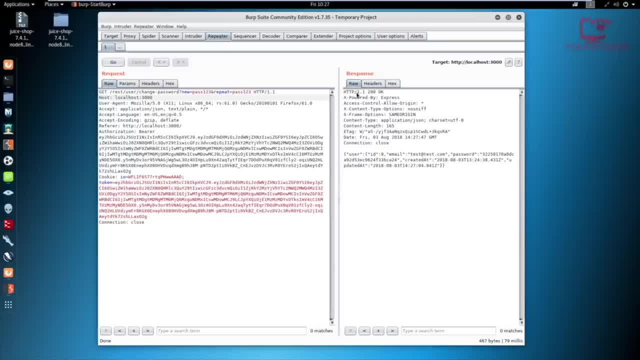 response, which means everything was processed correctly And we were able to get a password that looks to be hash, that looks to be hashed, And we got the email that we use. So, yes, we do know that it is working Alright. so we know that, we know that this worked, but we need to confirm that this 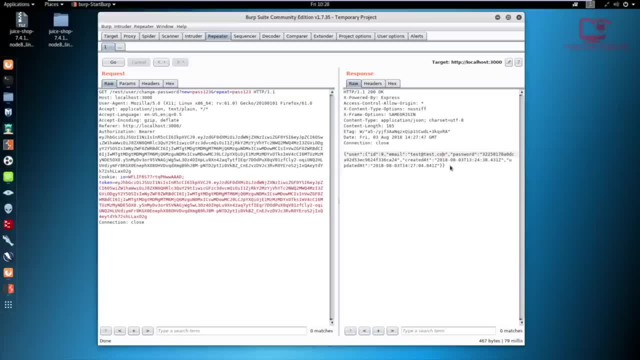 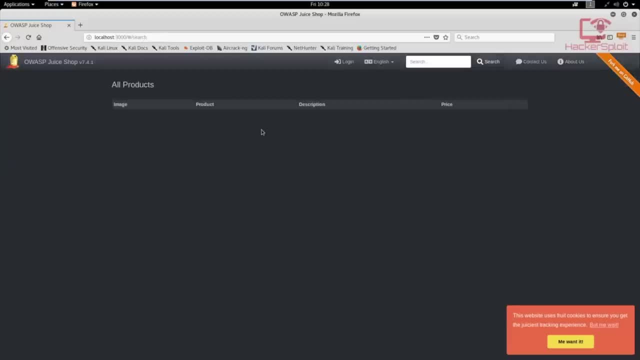 has worked. So we can do this By going back into our web application and we can log out and we can try and log in again. So log in with our new password. So we're going to say test at testcom And our new password was pass 123. 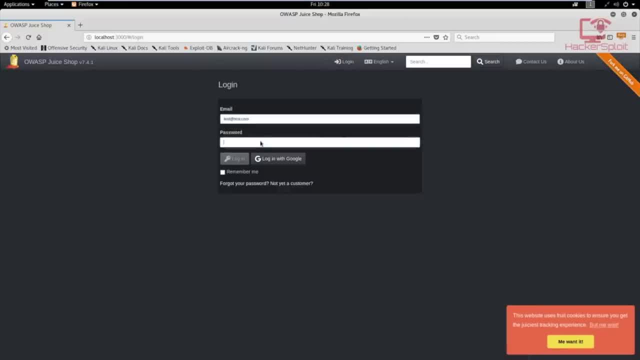 Remember we changed it earlier. But again, I was demonstrating that if we are to send this to our target, we need to specify to make sure that it will work without any pre required information like their current password. So we've manipulated the request there, So let's hit login And voila. 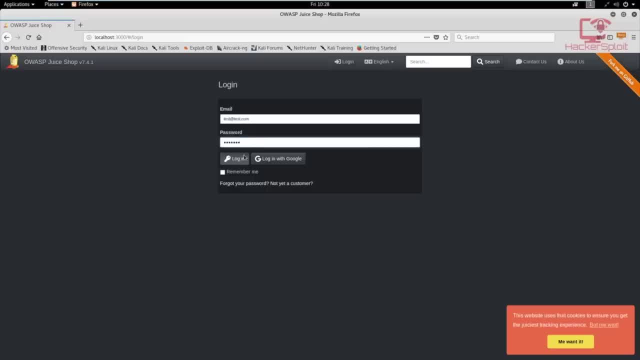 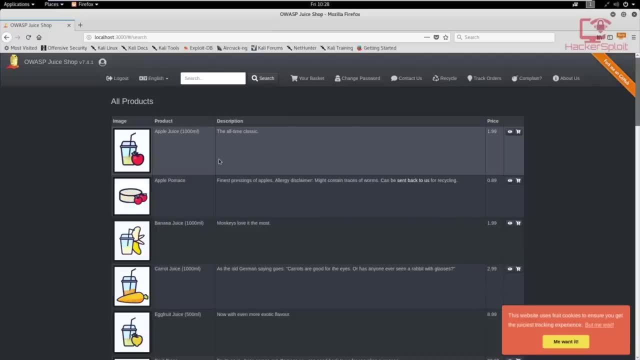 you can see it Does work. Excellent, All right. So this is a fantastic example of how CSRF can be utilized, or how it can be. X, how you can find vulnerabilities for it. Alright, so this can allow us to change, or. 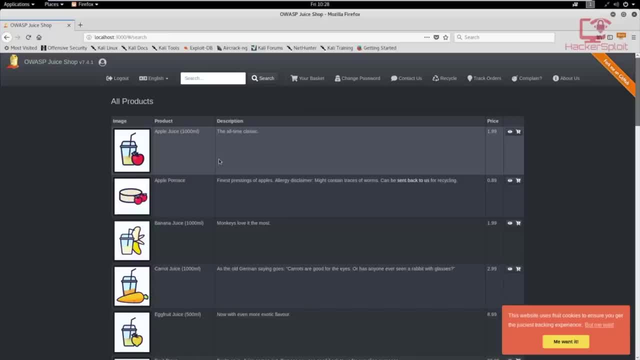 update anyone's password, anyone's accounts password that are currently logged into this web application. Alright, so now, what do we? what do we need to do? Well, we can. we can log in, As we've already seen. we can log in And once we've logged in, we can. 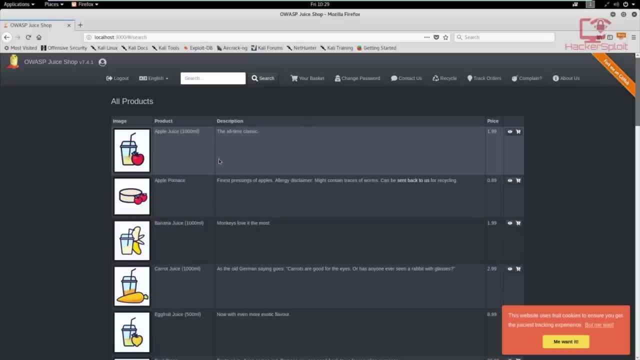 we can test to see if cross site scripting does work And then, of course, utilizing it throughout the web application is very important. So we can run a simple cross site script attack to see if it will work on the search bar right here. So I'm going to type in script and simple ones, or alert. 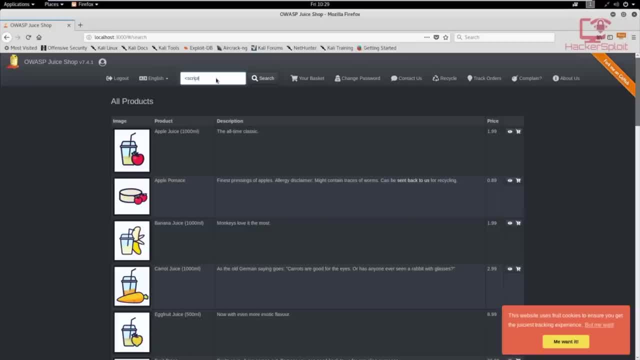 just just to test whether it works. And in the alert we can say: Hello, just something stupid, Hello world- you know that's, and I can't even type man on world- and we have typed in the alert and we can finally close the script here. Script like: 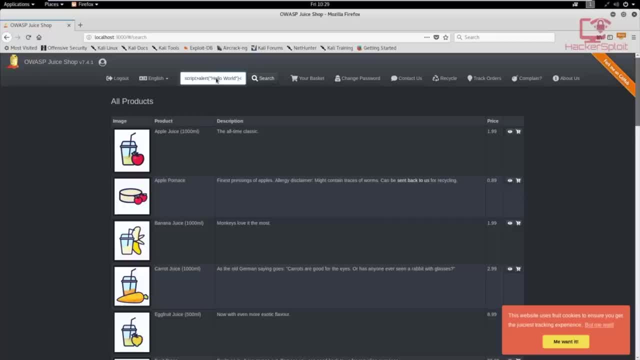 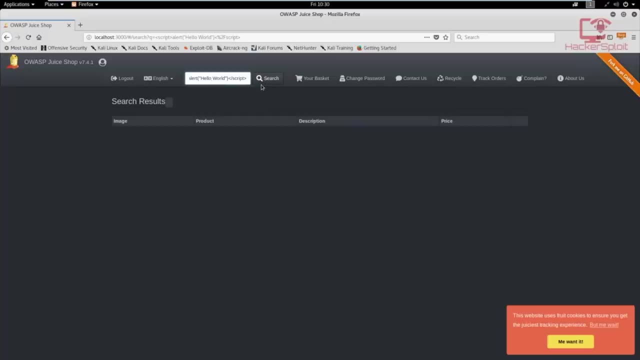 so and let's hit search And voila, we can see that indeed, cross site scripting what works, which means we can insert, we can insert our our get request inside a script and use a cross site scripting to perform the CSRF. And now you can see them conjoining together cross site scripting with 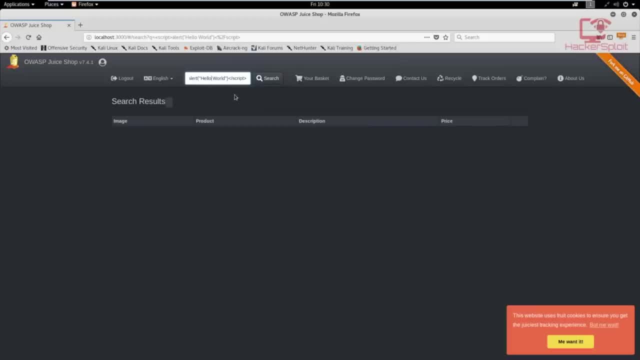 request forgery. Okay, so we now need to create our custom script that will allow us to utilize the attack, And we will be using XML and HTTP. Now, you might have seen this script right over here. let me just minimize this and open up leaf pad. you might have seen this script that I created. 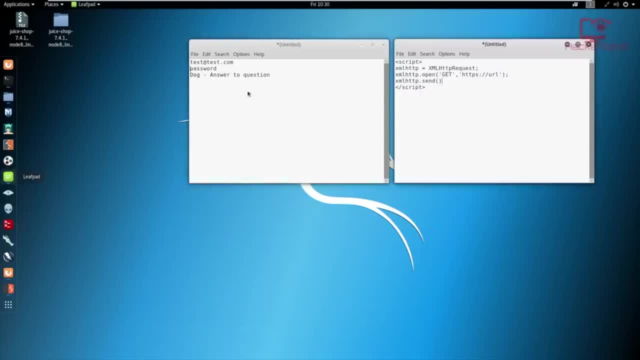 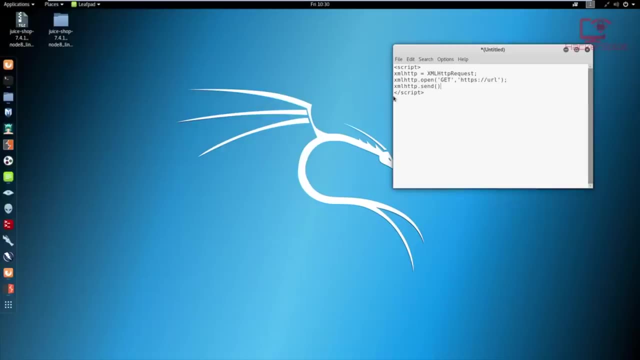 Now you can find many of these CSRF scripts online that utilize different languages. In my case, I find the one that works the best is the is the one that works with x, xml and HTTP and contains the get request, And in this case, I find the one that works the best is the is the one that works. 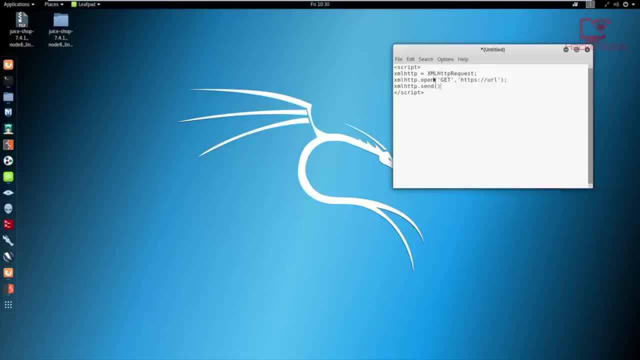 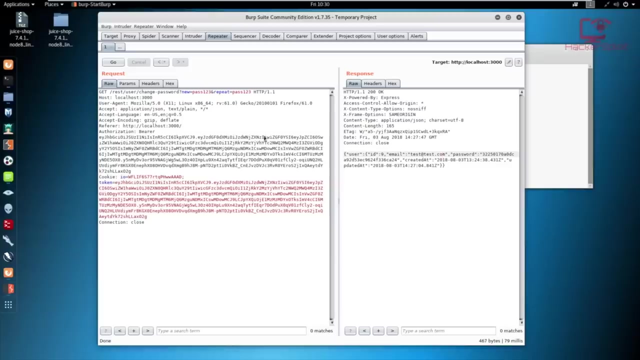 the best is the get request in here. Okay, now you can see that the get request requires the URL in which we submit the the parameters, without the current password. So we need to go back into burp And if I was to go back into proxy HTTP, sorry about that HTTP. we look to change the password. 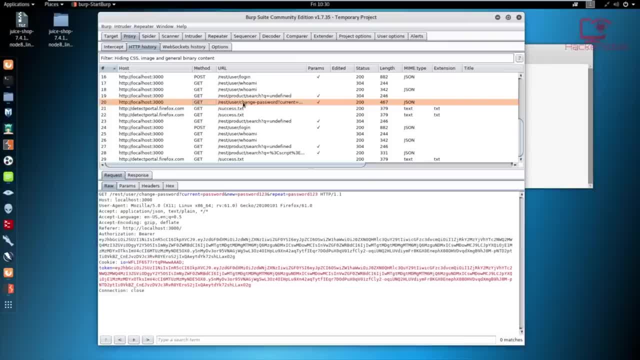 there. So if we go back into- sorry- the repeater and if we look at this now, we can see that the URL is right over here. So if we go back into the repeater and if we look at this now, we can see. 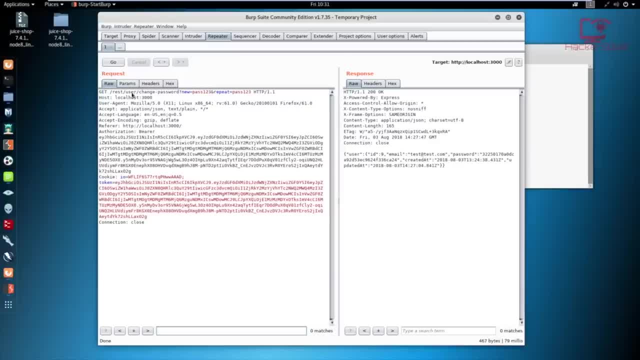 right over here. So that's the get request. So if we copy this, the localhost obviously, and we are not using any current password field. So if we can do that really, really simply, you can see how this can be utilized really, really well. So what we need to do now is understand how the URL will be. 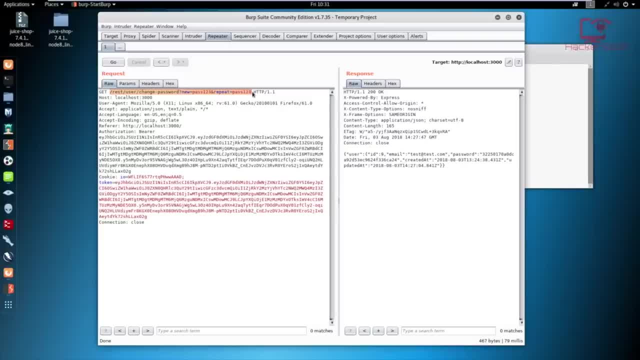 formatted And of course the web application is going to encode it and I'll get to that in a second. So we need to copy this URL right here. So I'm just going to copy the URL And we can edit our, our script So HTTPS, and we paste it in inside the URL. you can copy this script if you. 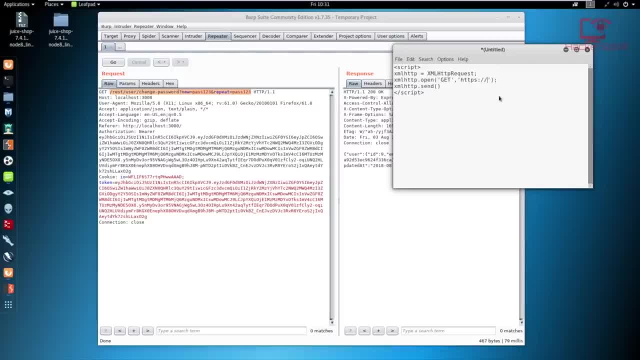 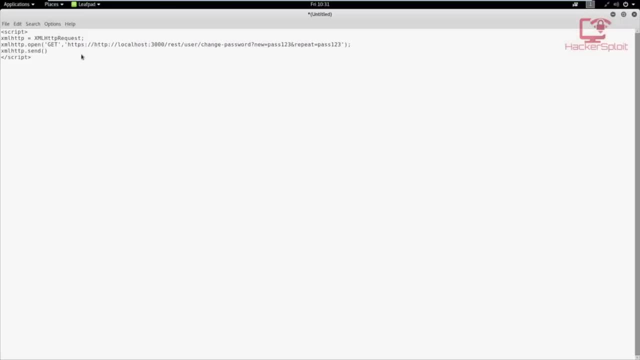 want to. Let's take a look at whether this script is formatted correctly. So get HTTP. No, that's not the way we want it. Let me get rid of the pre predetermined HTTP there, So HTTP localhost. It's hosted on my localhost with the port 3000, node, node j s standard And the. we want to change the. 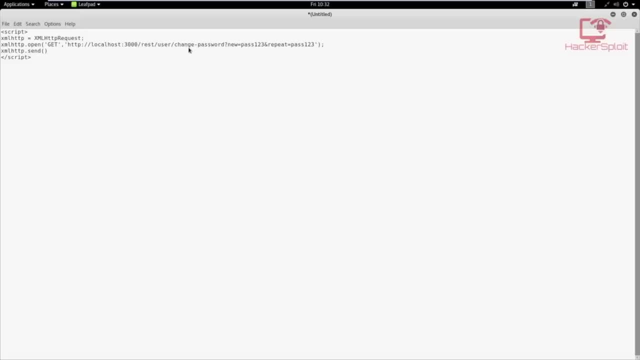 password. the new password is passed 123. And we're going to copy that And we're going to paste repeat: is passed 123.. You can change that to whatever you want. if you want to, you know, play around with a script, But in my case I don't want to do any of that. So this is the script. So 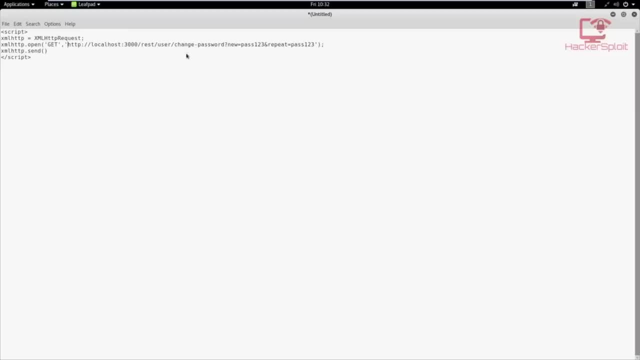 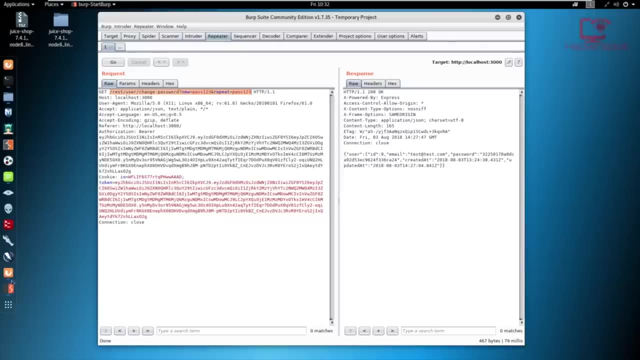 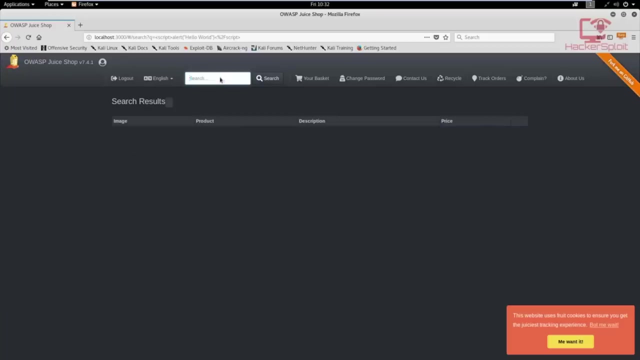 what we can do is we can copy this now And we can run this in the search bar, And that should, in theory and in practice, give us our first CSRF attack on the site. So I'm going to paste this in here And let's see whether it does this. So I'm going to hit search And you can see you. 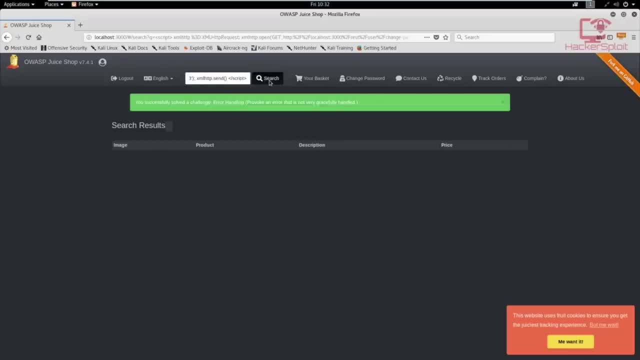 successfully solved, solved a challenge, error handling, provoking error that is not very gracefully handled. Again, this is a fantastic web application, vulnerable web application that is awesome for practicing your- your web application penetration testing skills. Now, I talked about the URL that you should send to your target, And that is the URL that will essentially make them. 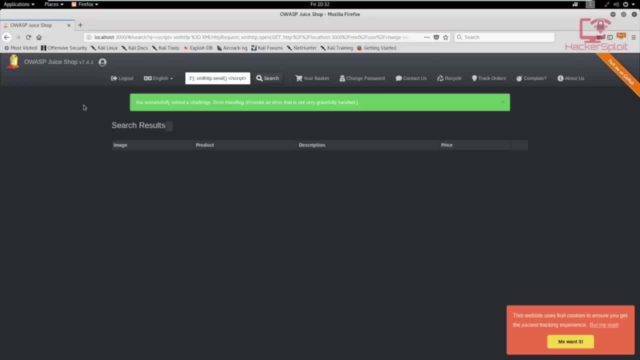 change their password without them knowing, given that they are logged in to the web application, right, they have an account. it will not work if they've not logged in, Alright. so that's very important to understand And many people, just you know- forget about this. Now, Again, if you could have, 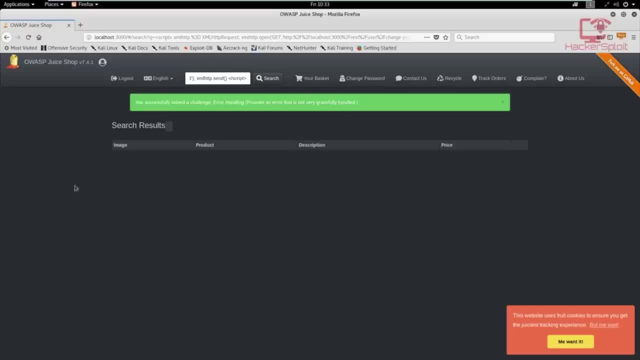 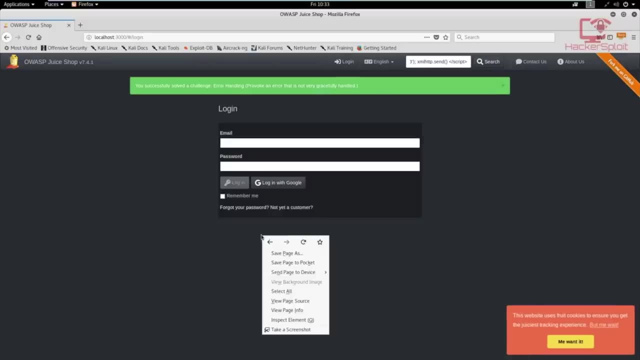 done this. you, I can log out again and I can log in. try and log in now And I can type in, for example: test. I just want to show you something very interesting here: test And I can change the password. we already changed it to password 123.. Now, before I do that, I can just 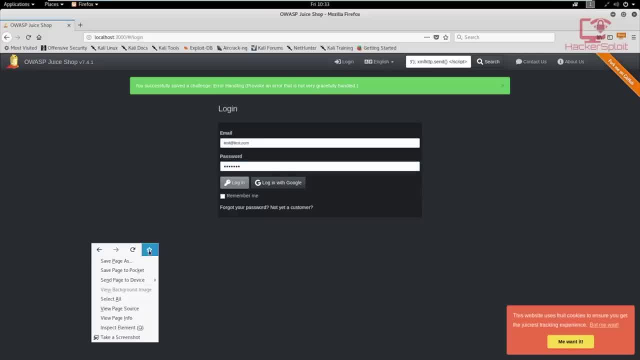 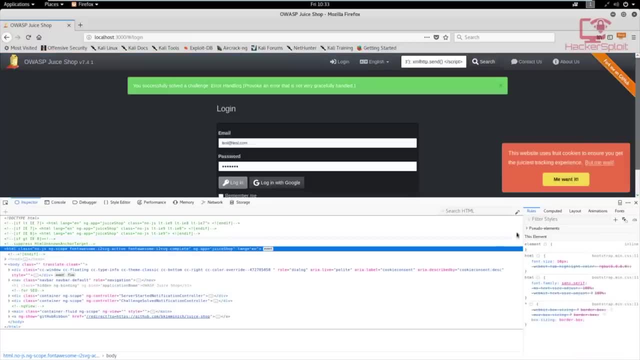 inspect the element here And I'm going to hit login And I just want you to check something out. all right, Now Let me just expand this a little bit here. If we were to look at the network, this will essentially show us all the get requests. So if I was to hit login, you can see. 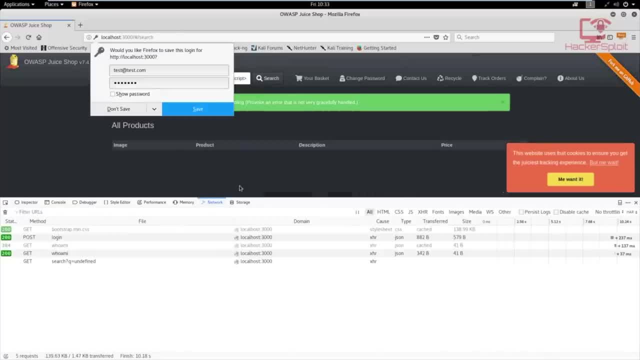 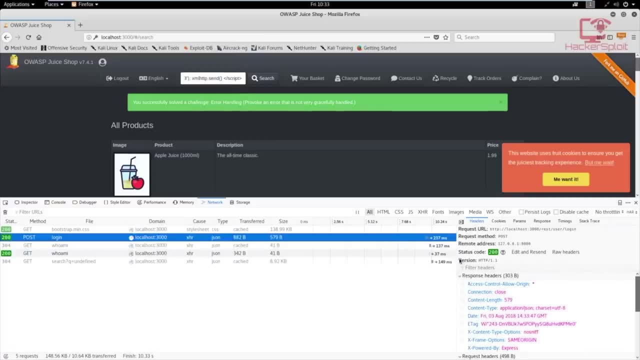 that if we are to look at the get request here, the login get request, you can go ahead and look at at the exact format in which it was sent. you can look at the cookie, the. it should give you the the authentication token, And then you can see that it's showing you the authentication token. 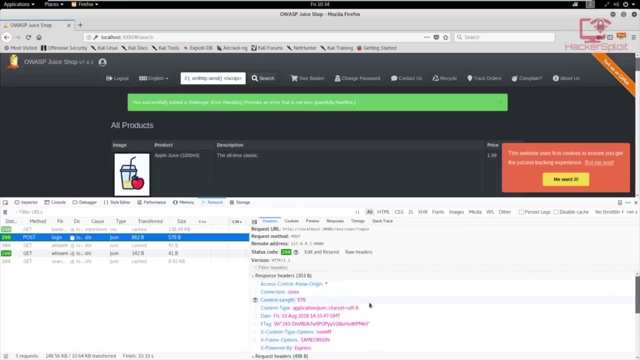 Not to show it should give you the authentic, the authentication token, But that's something for another day. I don't want to complicate you guys. you can look at the cookie if you want to, And you have all the responses right here. So there we have, there's the authentication token And you 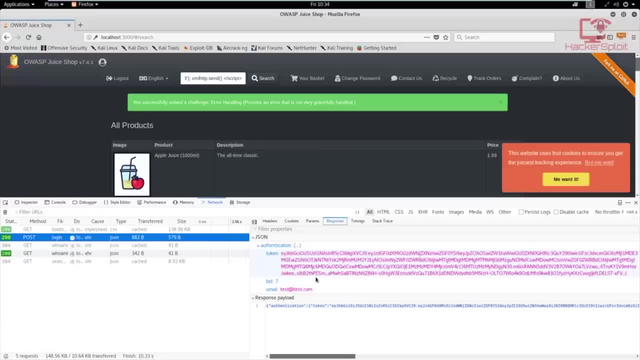 can see something very interesting in regards to the token. Alright, so let me show you this right now. Alright, so, as I was saying, you can see, all right. so, as I was saying, you can see that if we look at the parameters, the password will be displayed. 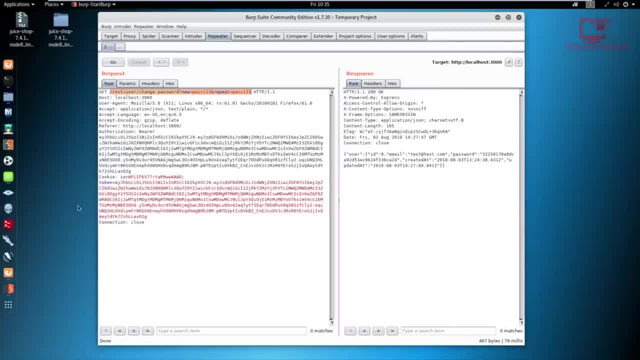 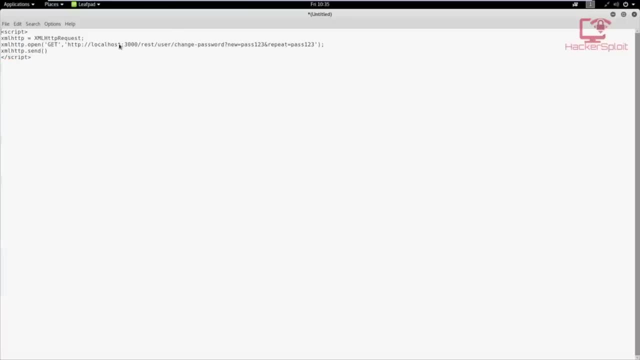 there and it will be updated to the one that we selected or specified in the script. Alright, so remember, if you want to customize the cross site scripting attack, you can do it through your script, And where is leaf pad here? So there we are. So you can change the password, the, as you. 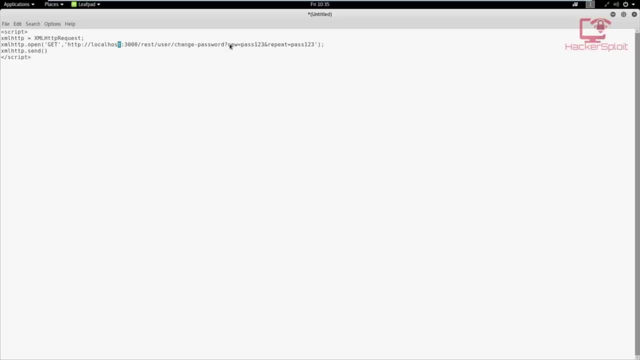 see, we just got rid of the current password parameter, which is a vulnerability on the site, but you can change the password to whatever you want. And now you might be asking, as I've mentioned, what is the password that you want to change? Well, as you can see, you can change the. 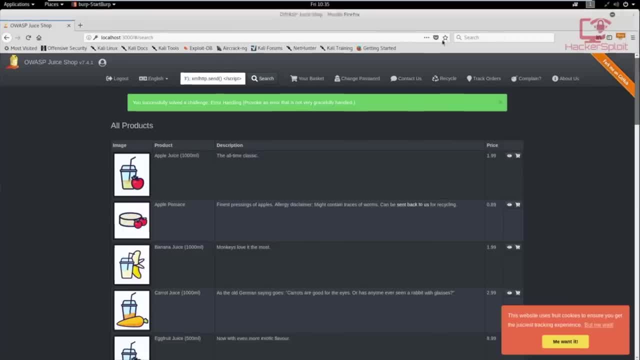 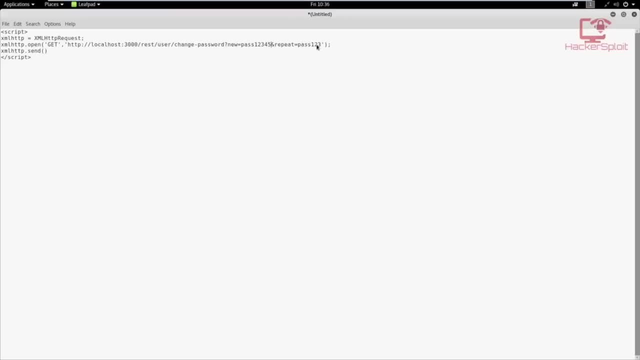 password to what link do you send to the target? And that is very, very simple. If I was to run the script again and I change the password to maybe something else like password 124, or 345.. Sorry, three, four, five, let me just add that to the password And I run the script on an authenticated 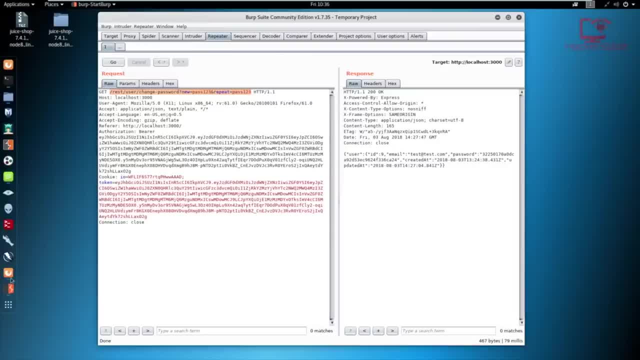 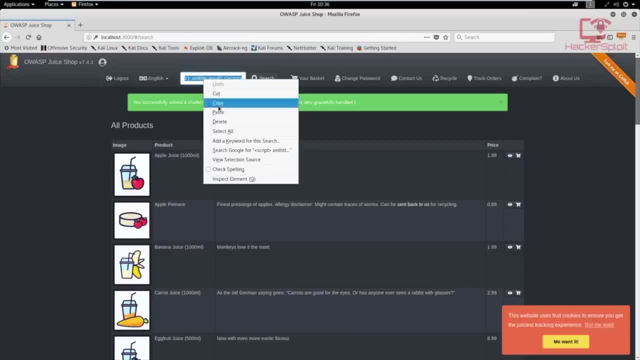 user, which is me. So let me copy that And it should change my account password And you can see, once I log out, log out and try logging in, it will have changed it successfully. So let me just run it in here. 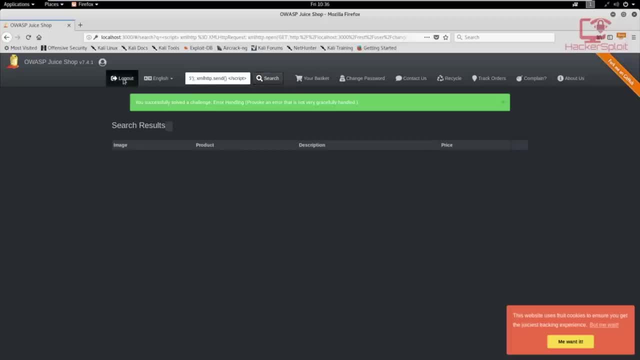 So I'm going to paste the new one in here And I'm going to search and there we are. So now it's changed my password And if I log out and I try and log in with with the old password, which is: 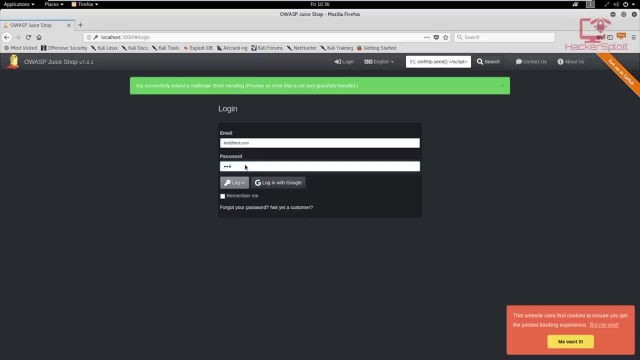 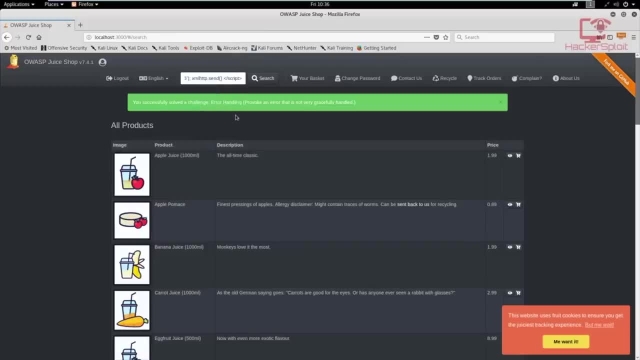 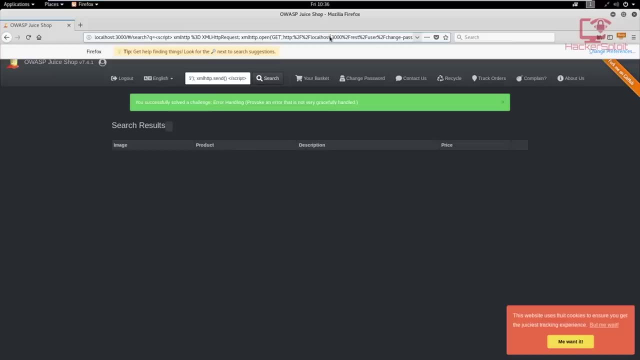 password: 123, you can see- whoops, sorry, I think I typed that in wrongly- 123. Like so fight login. there we are. you can see that we entered the new password and it did work. Fantastic. So we were successfully able to execute the script. And again, when? if I just run the script again, this: 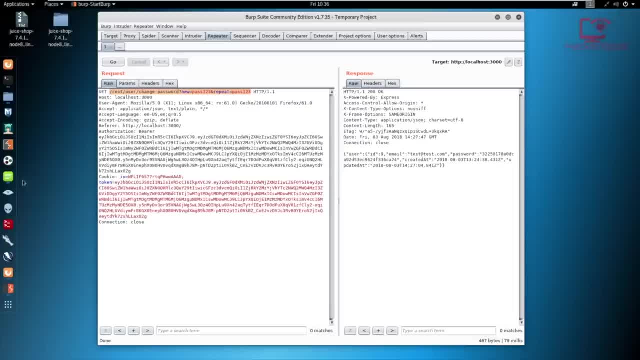 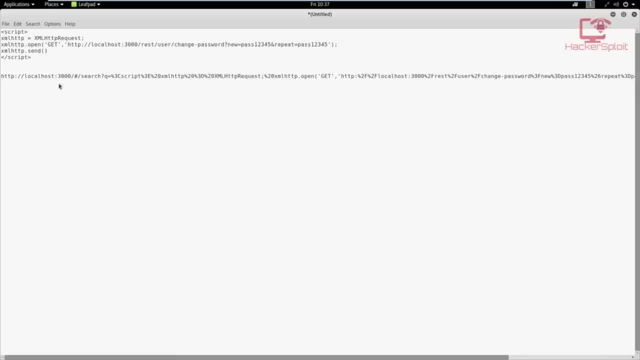 is the URL that you will send to your target. Alright, so if I just copy it and I inspect it in my leafpad here- I really love leafpad. I don't know that you guys love it too- If I just inspect. 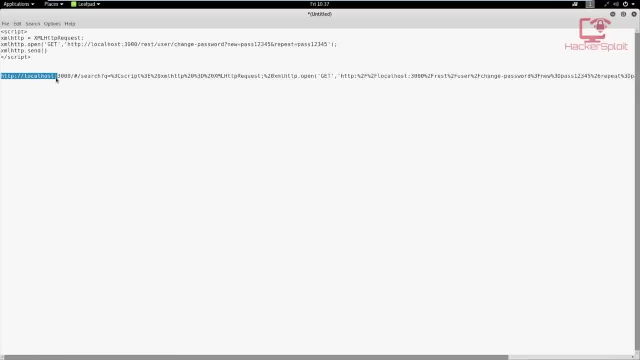 it. you can see that this indeed is a URL, And if the web application was being hosted on a server outside my local air network, it would give you the website name, the port, if it is port specific, and the URL here which, as you can see, is encoded. So what I would recommend is that you copy this: 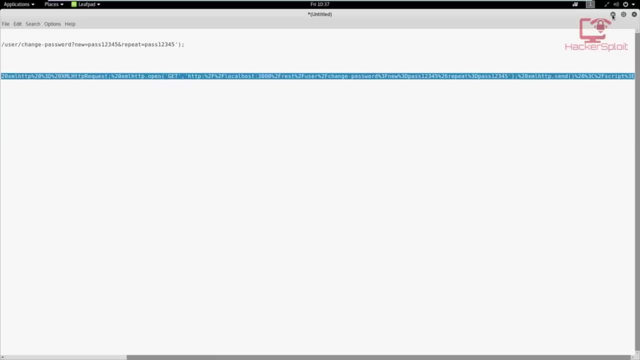 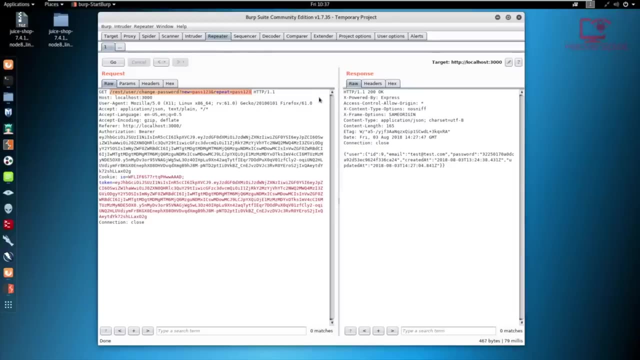 link here and you use a link share shortener like bitfly or any of the other Google shorteners and you send that to your target And once they click on the link and if they already logged in to this specific web application. 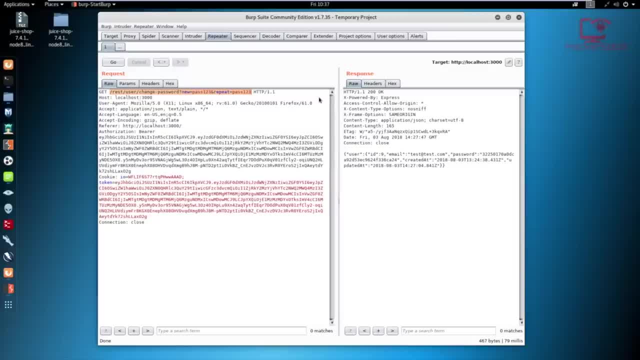 it will update their password and you can. essentially, you have their password now because you've updated it And you're. all you need is the email, which I'm pretty sure you must be knowing if you're performing this attack, or you could just be gathering passwords of users. 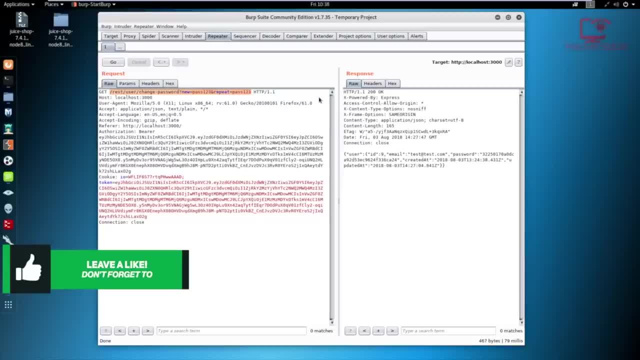 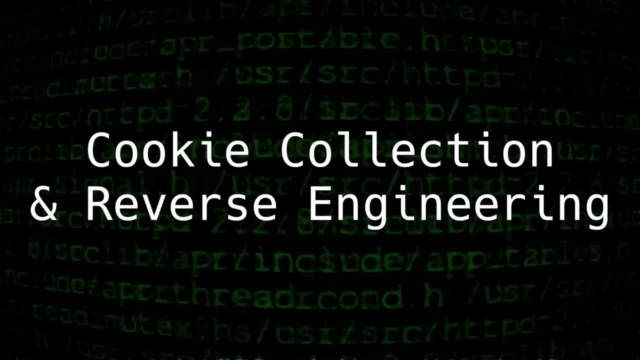 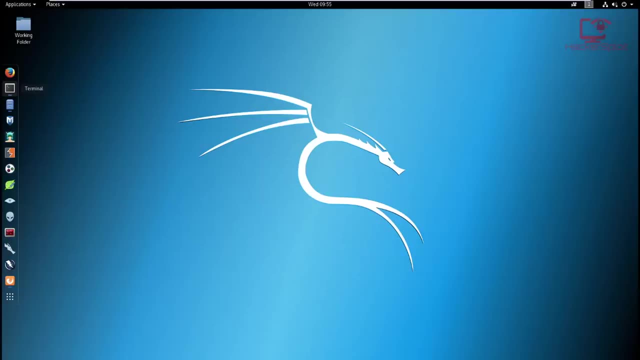 or of which you can, you can send this link to, and are authenticated with the web application. We're going to be taking a look at session management And, in this video particularly, we'll be looking at cookie collection. Alright, so, as you know, you probably would have known what a 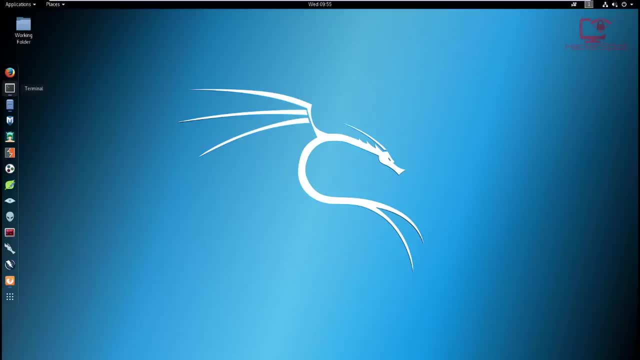 cookie is Now. there are three types of cookies that we really need to be focusing on in this section And we will be focusing on in general. The first one is the session cookies, which I'll discuss in a while. The second one is the session cookies, which I'll discuss in a while, And the 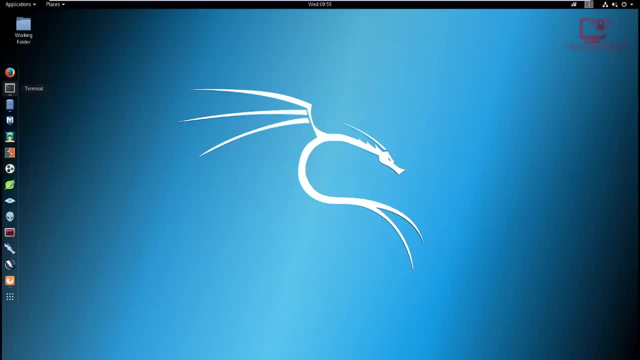 third one is the session cookies, which I'll discuss in a while, And the fourth one is the session cookies, which I'll discuss in a while. We then have the permanent cookies and the third party cookies. So third party cookies are really all to do with third party API's that may be used So for 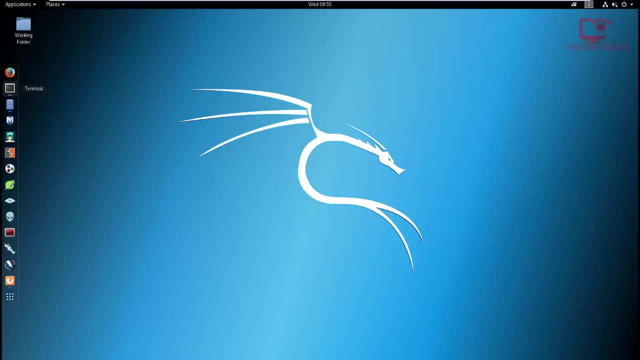 example, if you're on a website that utilizes Flash Player, you may find some cookies that that are in relate, that are related to the Flash Player. So it's very important that you understand how to collect these cookies And, as well, we'll be looking at reverse engineering them, but not 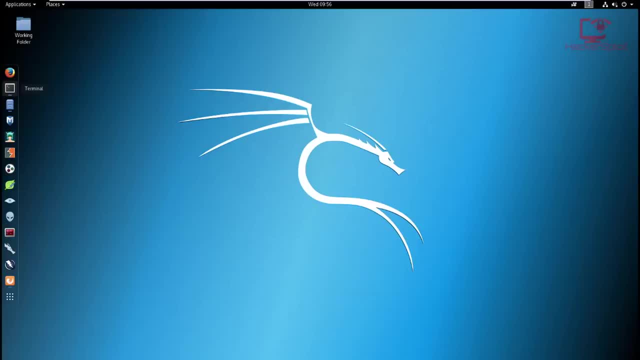 really tampering with them. So we'll be looking at reverse engineering them, but not really tampering with them, Because of I first want to explain to you guys how everything is done And then we can move on into into finally tampering with them and seeing if we can change them to give us access to 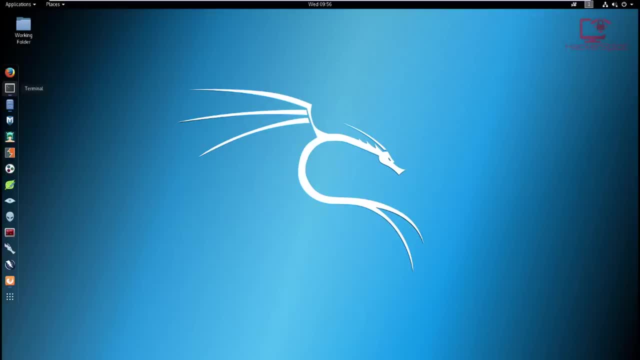 give us different type of of access And where this comes into place when you're talking about session cookies, And in the session cookies we have the, the, the authentication token, and the D and the unauthenticated token. So all to do with your access on a web application or on a website. 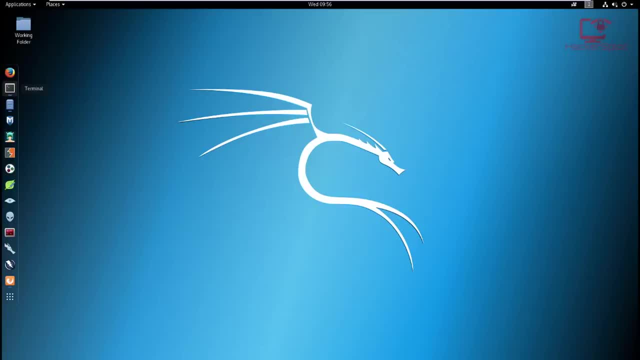 Okay, so essentially all the cookies that you can probably ever get when you visit you you get when you visit a website. they are generated when you visit the website And, furthermore, the cookies change when you authenticate with the website and you are. you log out, right. So when you log in, you get a. 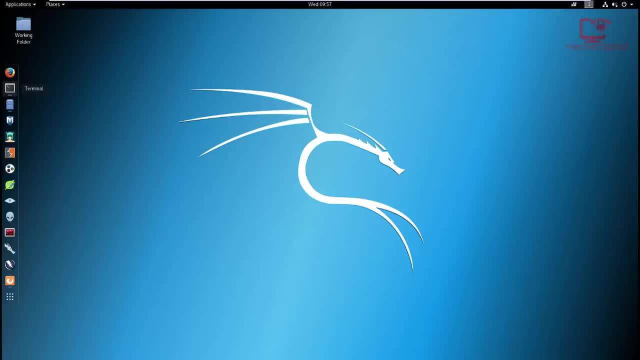 different set of cookies And when you log out you get a different set of cookies. this is where the whole idea of session management comes into play and our cookies are utilized for the system. So I'm currently running OSP juice shop, So I showed you guys how to set that up. Let me know if you. 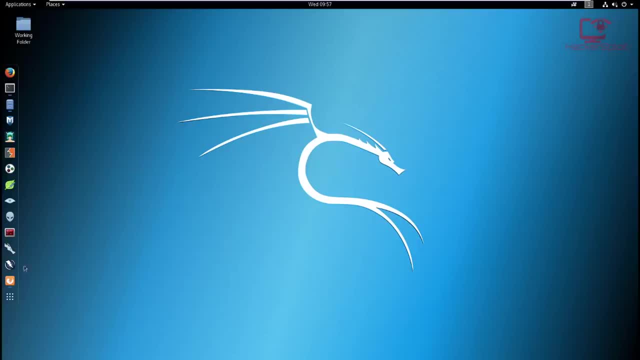 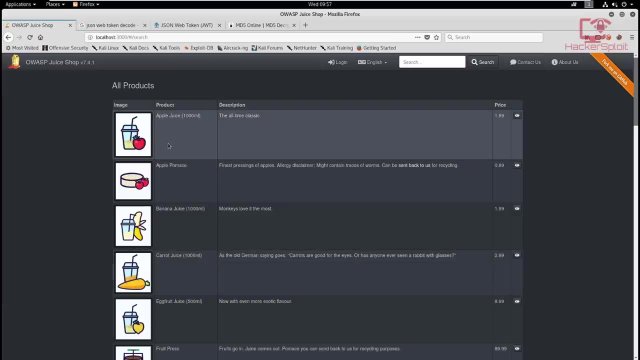 found it helpful, So I have it set it up and open. I have it open up in my browser. Now what I'm going to be covering is how to collect these cookies and understanding the difference between an unauthenticated cookie and the authenticated cookie. So usually what I have or what I use to 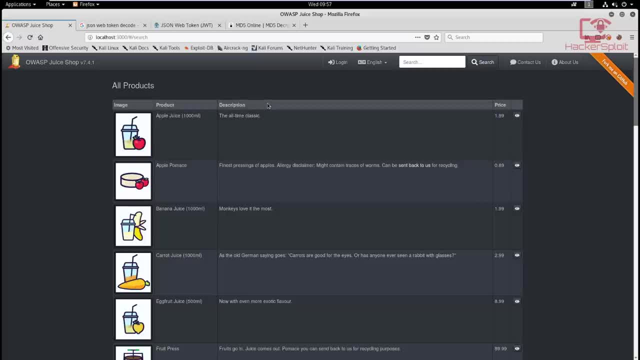 my advantage is, if you're using Google Chrome or Firefox, you you can get a cookie collection or a cookie editor add on that allows you to edit the cookies. But, as I said, we're not going to be looking at editing them right now because we don't know what to change in them. This video is going. 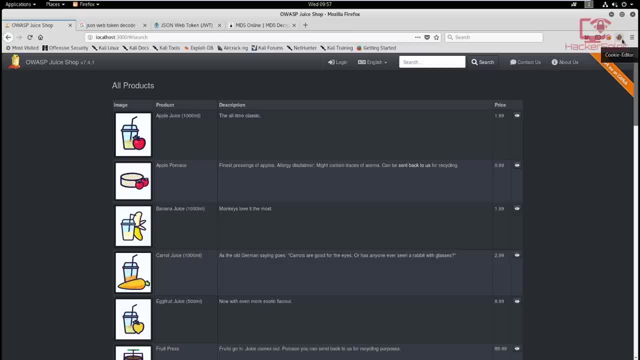 to be focused on collecting them and then analyzing them to see what information they have within them. Alright, so I've currently I reset this, the OS juice shop, and the reason I did that is just to start off fresh, And I said we're going to be using the cookie editor, So I'm going to be using 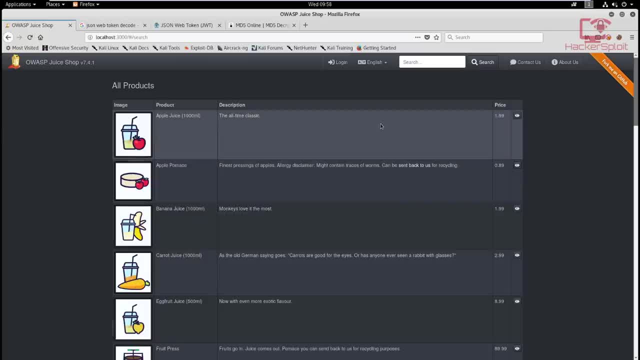 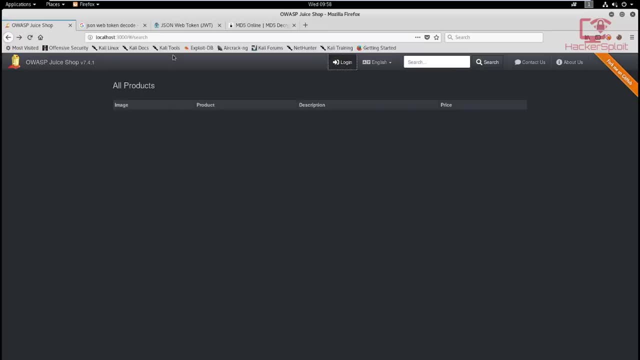 this for performing all of the examples that I'll be showing you, so that we can learn all the concepts. So I'm just gonna work before we log in. I just want to show you the first set of cookies that we'll get once we when we visited the site. Don't worry about the other links, we'll get to. 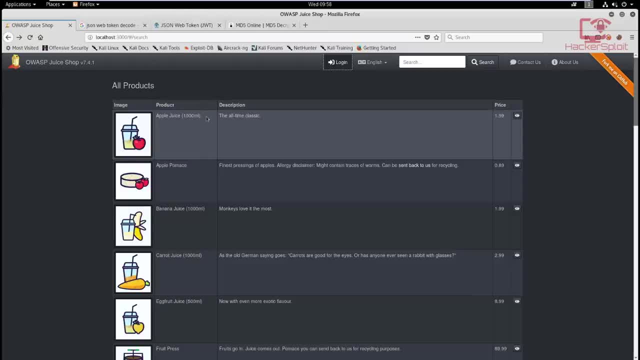 them in a second. Alright, so I'm using the cookie editor right here. you can find this same one for Firefox. that's what I'm using. There are also other ones for Google Chrome, if you want to do that. And, in addition, we're not going to be using the cookie editor right here, we're going to be 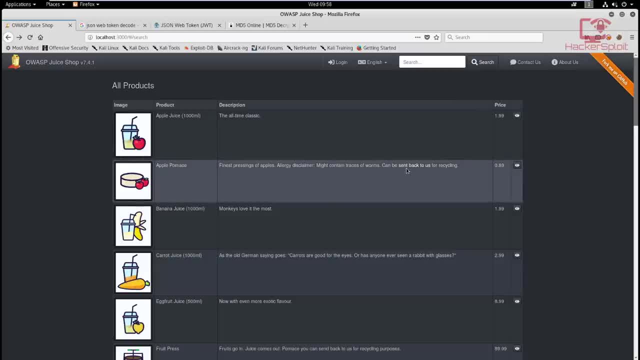 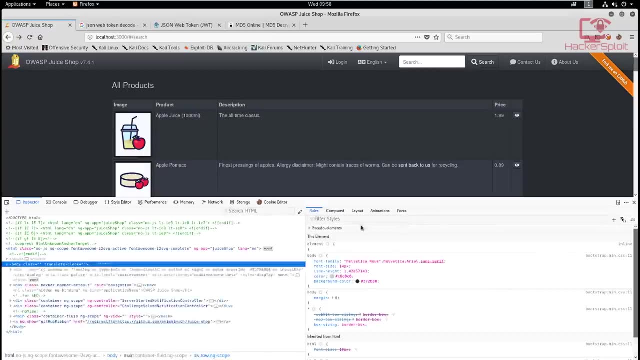 using any proxy like burp suite or the OS zap right now, because we're just focused on using the browser tools And, of course, these add ons here. So what I can do now is, if I just go right click and I hit inspect element, we have the developer tools right here, And if we are to go into once, 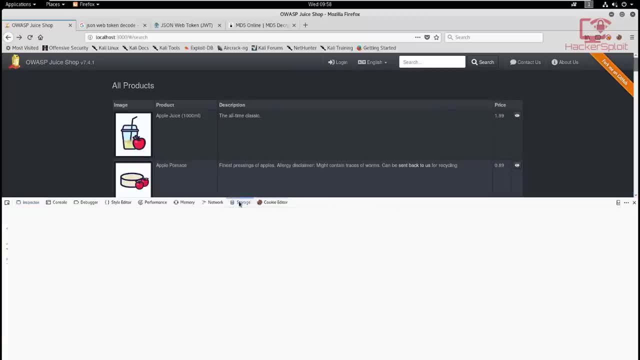 you've installed the cookie editor you can directly go into storage And in storage you'll you'll be given you'll get the cookies here and other values right here. But if you look at the library editor, if you watch what happened, sometimes it doesn't look that you're saying. 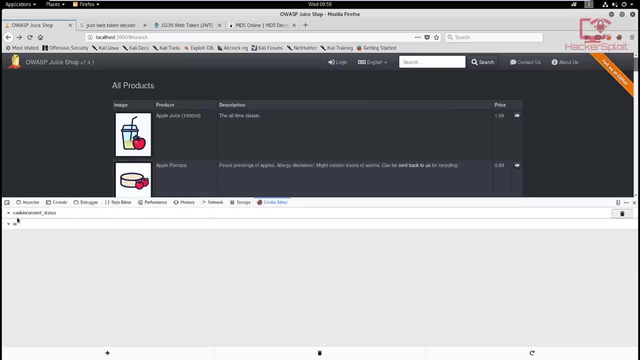 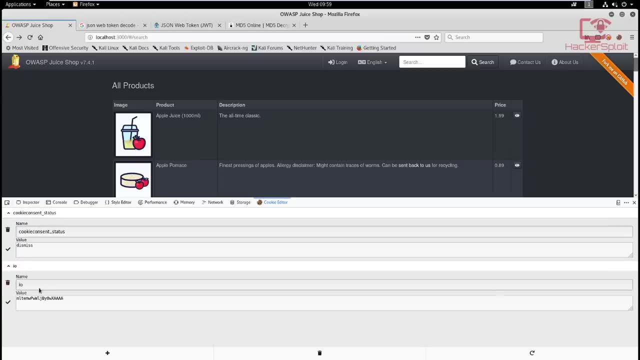 this. it appears down here. if you do clickRealize In order to take away a copy of that, look at theограф employee here and it shows the see: ¿What do you have? Here's two of your cookies. this one is currently available for both iOS and Android, So that means in MacBook. 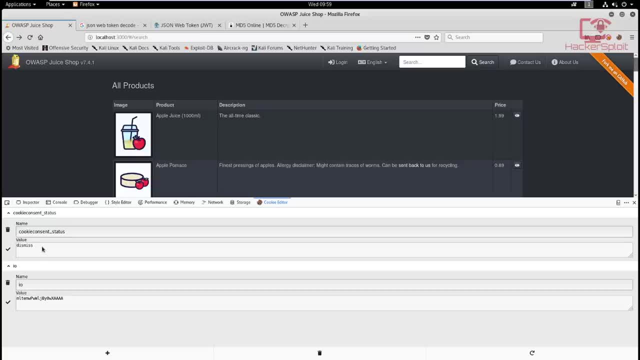 you can also download it here in this folder. so it doesn't say: to open this folder. you see the desktop. it doesn't say what he does. And then we just have a group of cookies here. And this is really all about weaving. when I open a. 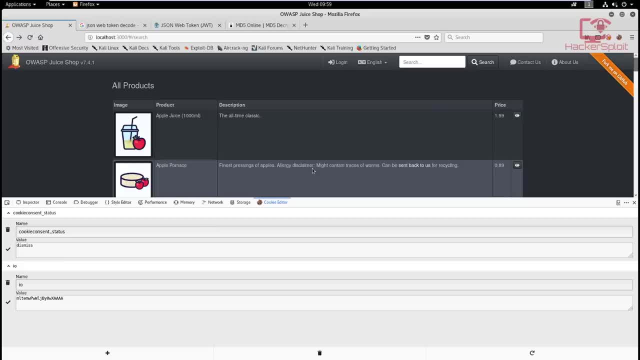 console. I'll just do this. I'm probablyЯ based on a question here, So let's open Jen. then, when I open up, it gives me a prompt asking me like all websites will ask you in 2018 to do is to accept their privacy policy. 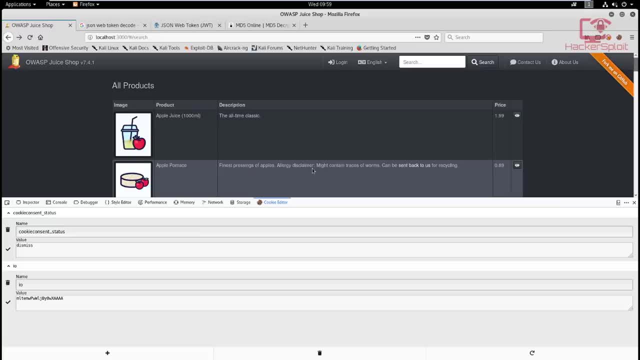 in their privacy policies in regards to their use of personal data and cookies, And the reason is is because cookies can can log or have a lot of information about you. They contain a lot of information about what you're, what you've been doing, So this is why I've created this right now. 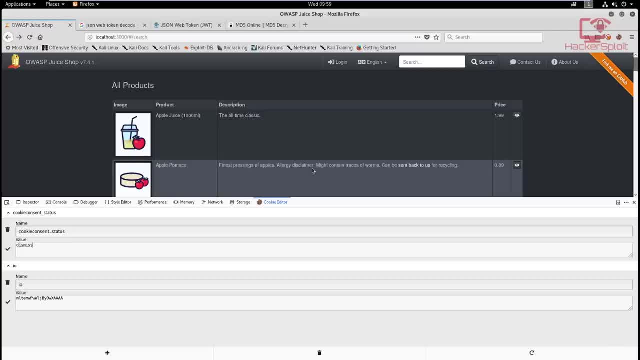 before we move along, it's very important to understand their role in session management. Okay, so we need to look at the authentic, the authentication tokens, because that's where most of the magic happens, as you would expect. So let me just close this up And let me just log in. So 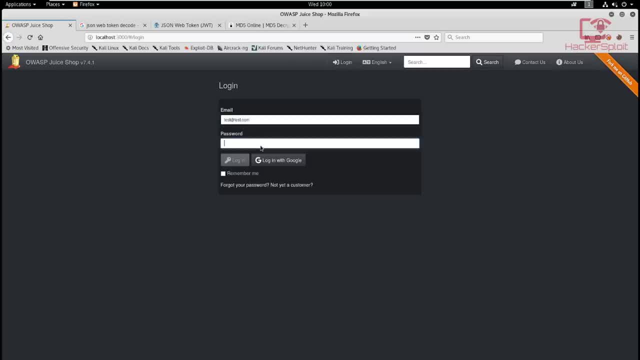 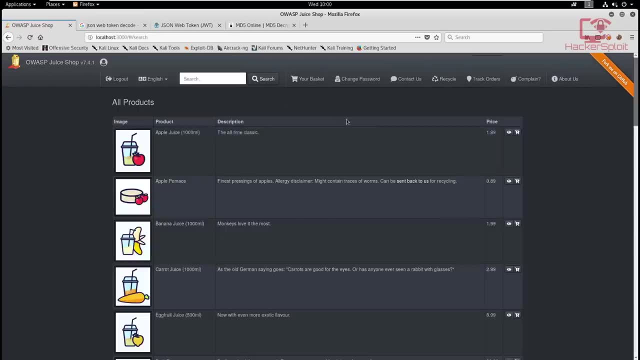 let me just use the password there, the email that I used and the password, like so, And let me just log in. I don't want to save the password, So I've logged in now And if I inspect the element, 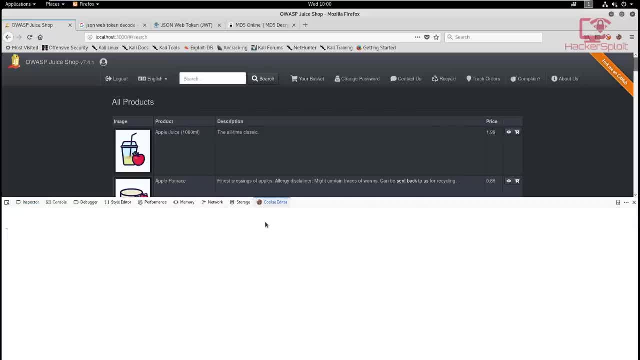 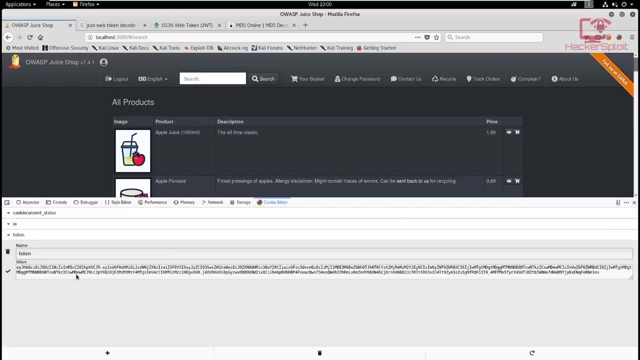 again. you can see in the cookie editor: let that load. it usually takes a while to load. there we have the token, now the token. this token is an authentication token. Alright, so when it comes down, when it comes down to reverse engineering a token, for example, let's use this as our example. 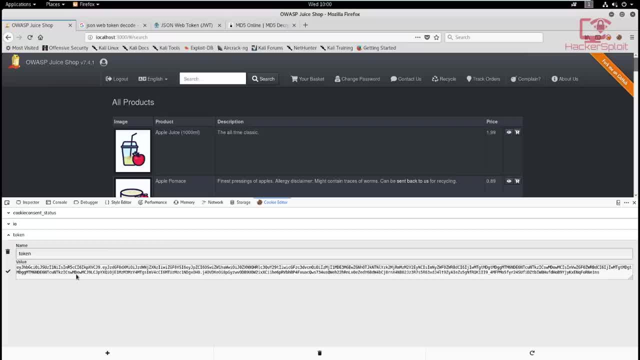 we essentially testing it for vulnerability, similar to a penetration test. Now you might be a little bit confused. you might be asking: well, what, what? what do you mean by this? How can we perform a penetration test on this token? Well, this token is encoded, alright, so this is. 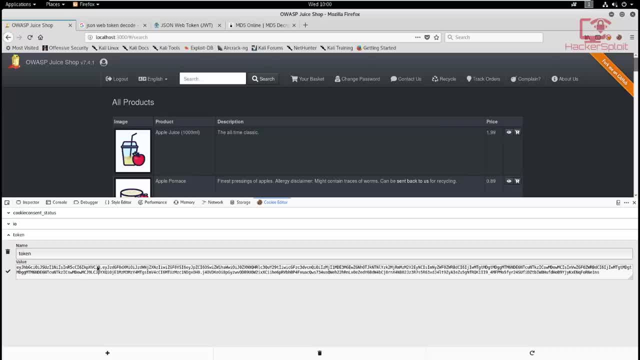 if we just copy this. I don't know whether you know about this, but this is a JSON web token. Alright, so it is. it is a JSON web token And you can use the JSON web token decoder. I'll be posting this link in the 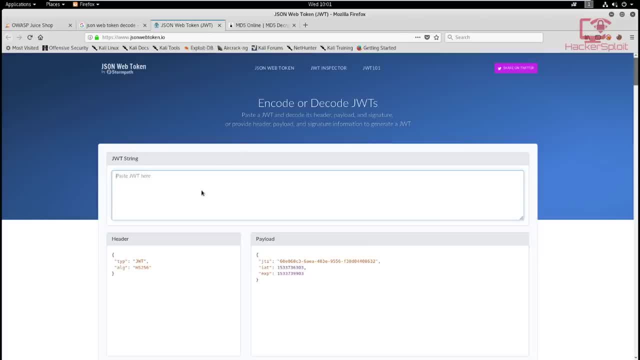 description. This is the one that I prefer to use If I am to paste this in here and you can see. but once I've pasted it in here, it's going to give me all information And I'm going to help. 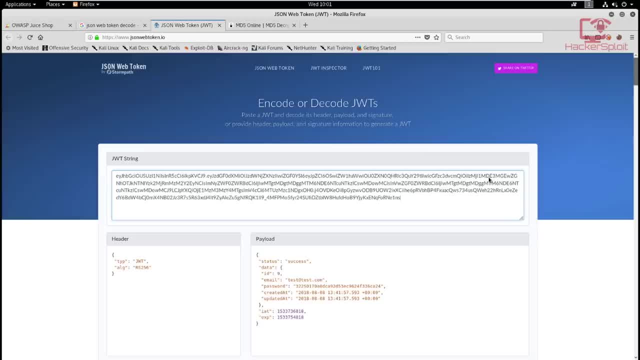 you understand what we've just done. So, essentially, what we have done is we have reverse engineered what this web token is all about. So now we need to look at this, So we're going to look at this. So look at what, what it contains and what type of authorities or privileges is giving to us, because 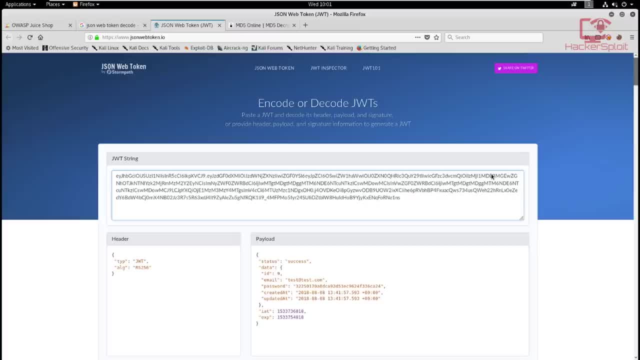 remember, this is an authentication token And it is unique to us because this will this will determine whether or not we are logged into a site or we're logged out, and what access we have on the website. I'm pretty sure you already know that. Alright, so when it comes to the header. now. 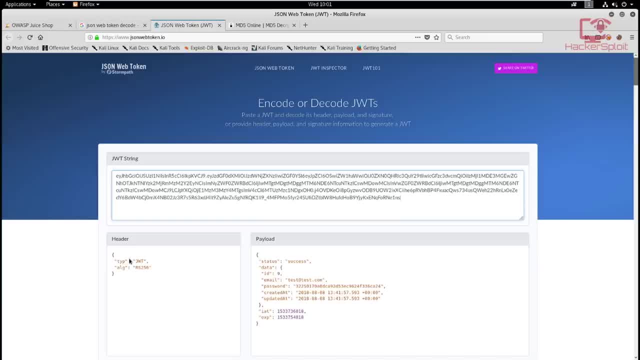 this is very important. I've seen many web people claiming to be bug bounty hunters and they don't understand how the the web token is even structured. What is the header? the header is separated from the payload. this is the header right here, up until the first full stop that. 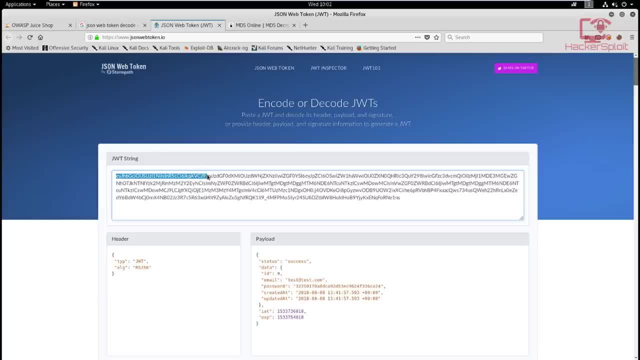 is the header. it's very important to understand that, because they are separated from each other. In fact, the JSON web token is sorted into three parts. right here. you have the, you have the header, you then have the payload- until here, And then, finally, you have the signature, which is right. 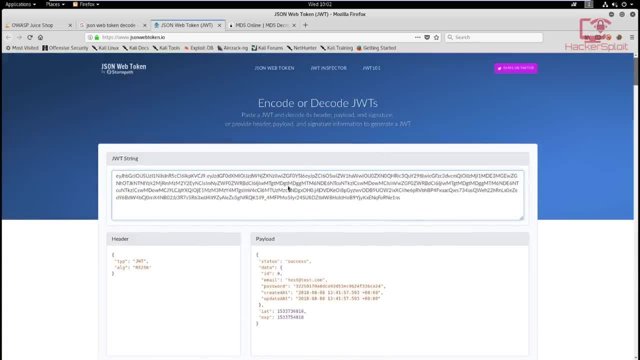 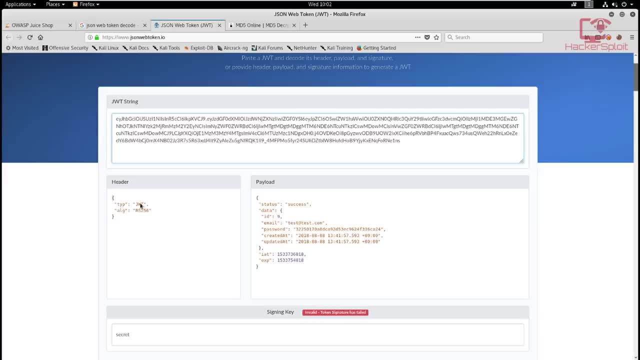 right at the bottom here, which is also separated from the rest. Okay, so when it comes down to the header, alright, the header is going to give you the type of the of the token, And in this case, we know it's a JSON Web token. we then have the algorithm, which is: 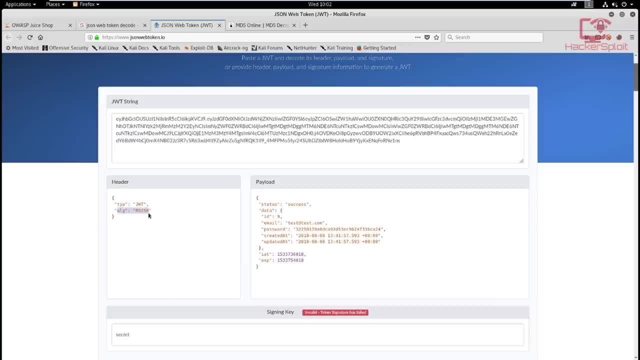 the hashing algorithm used, which is the Rs 256.. And then the payload. now, in the payload, This is where things get really interesting. as you would have expected, you have the status, the status code here, the data, if any data was passed. the Id- we can always use. the ID Two- we can always. 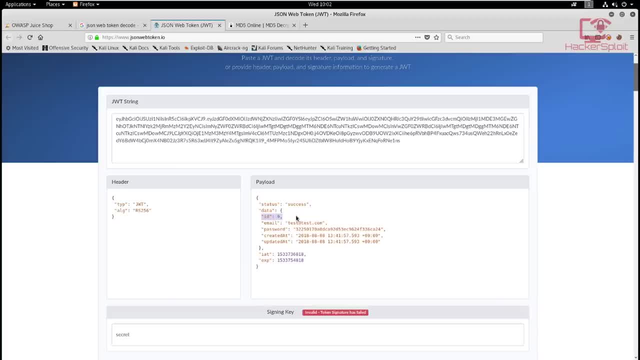 Say, always edit the ID to see what else it can give us in terms of authentication, because different types of identifications or identification tokens give us different types of access. So, as essentially this is what I was talking about, this is where you will scrutinize the, the, the. 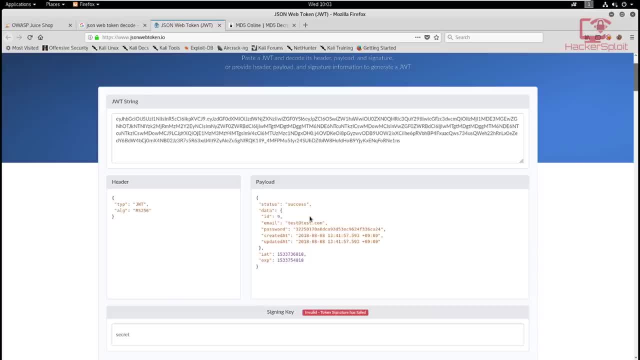 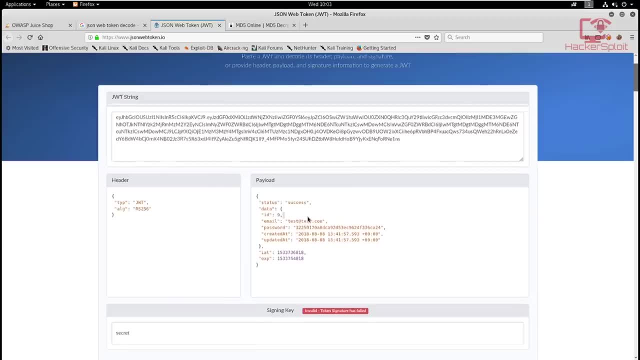 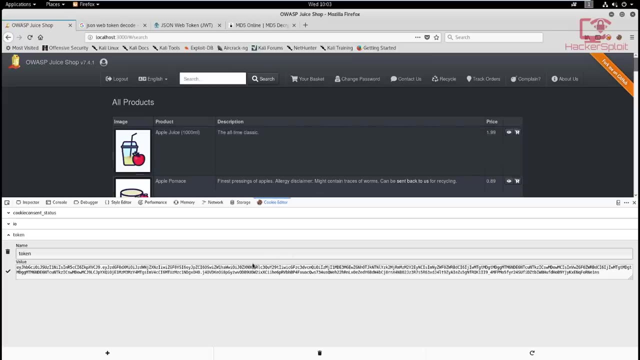 authentication token and try and tamper with it to see what different results you can, you can get. So remember we can edit this token, alright, and we can edit anything about it, And then we can finally copy it And we can use that in the OSB shop and paste it right here and re authenticate. 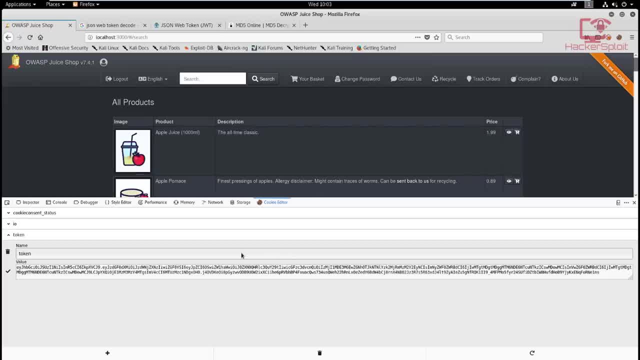 with that new token and see what results we can get. Now, of course, we're not going to do that right now, because I wanted to introduce you as to what information you're going to find and what exactly is going on here. Okay, so one step at a time, So you can see that something. 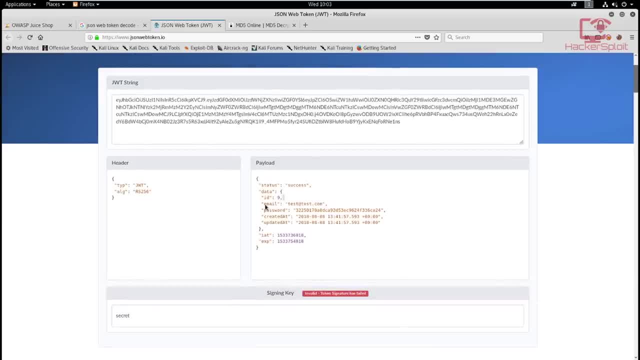 interesting props up here, something extremely interesting. We have the email which, for some reason, in this token, we can see that it's not very well designed because the email is in plain text. which means, which means if, in any case or in any scenario, someone is able to get this token in which I 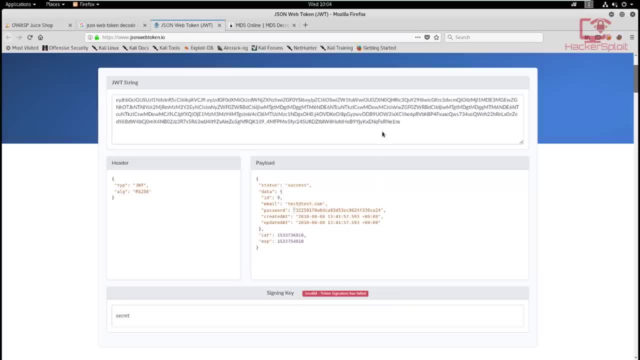 authenticated within a site, they will have access to my email and my password. But you must be saying: Well, I didn't see you type out all of these random passwords here. Well, I can easily guess that this is an MD five hashed password, which means I can, depending on what you're. 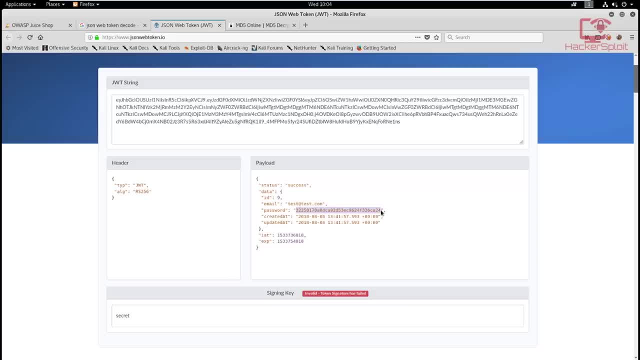 signing on the on the strength of the password I can decrypt online in a second using any of the decryption tools. So if I was to just copy this right now and I wanted to know the password, let's say this wasn't even mine. this authentication token wasn't even mine. 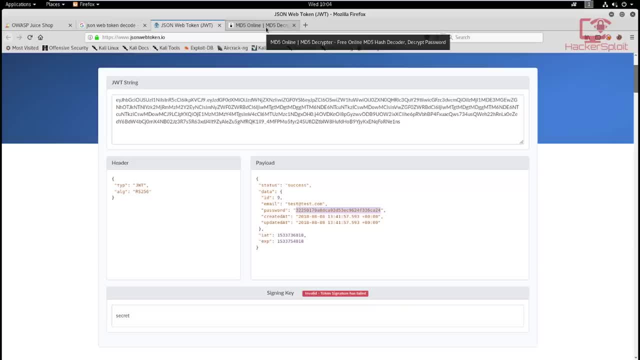 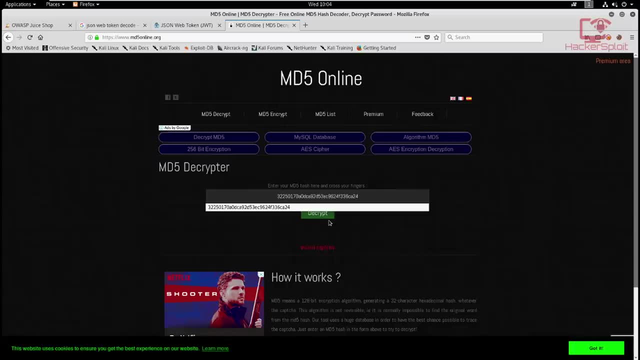 and I found the, the email and password. all I needed to do was unhash the password. I can go to MD five onlineorg, which is what I use a lot, And I paste that hash right in here and I hit decrypt And you can see well, first of all is going to prompt me to enter: capture your 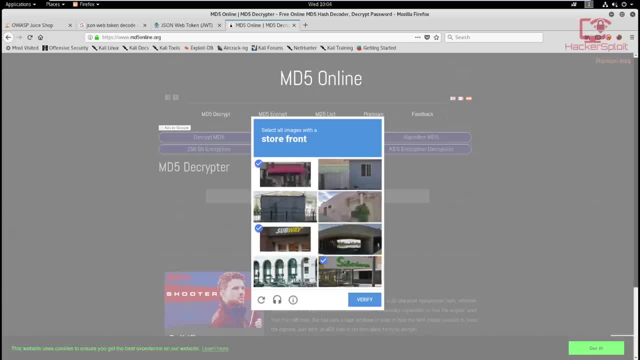 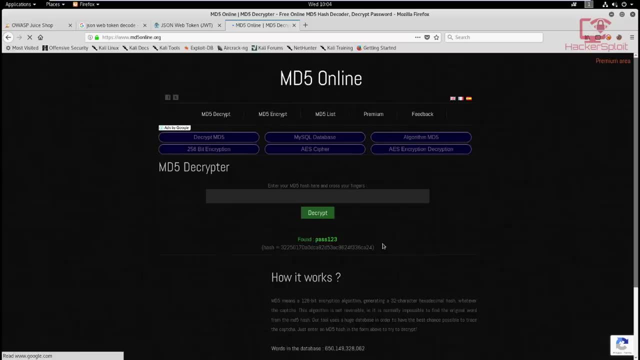 storefront. This is getting really annoying now. For some reason, it always does that. as you can see, it's going to. it's going to find the action. of course this is. this is dependent on the difficulty of the hash and whether or not it can find it online. Okay, so you can see that. 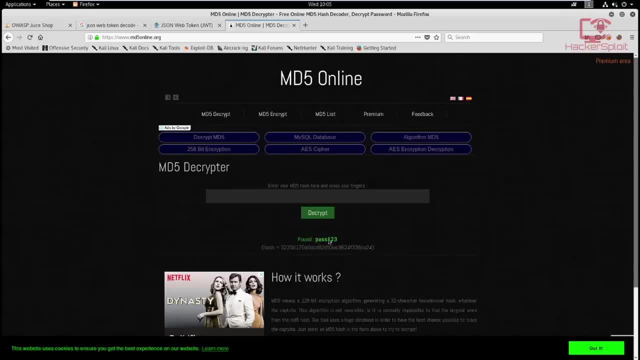 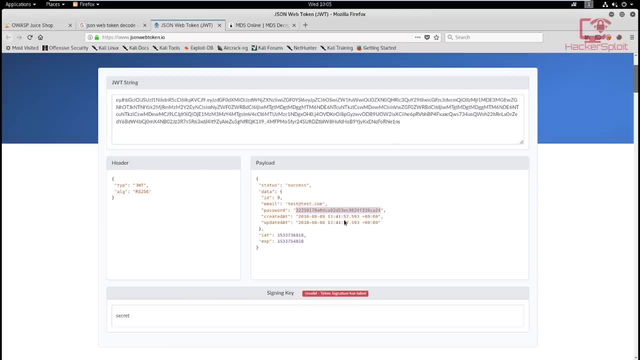 the display, the hash and the password in plain text, which in this case was pass 123.. Now, of course, you can experiment with this, And you can also also experiment if, for example, the authentication token that you found was using a different encryption. 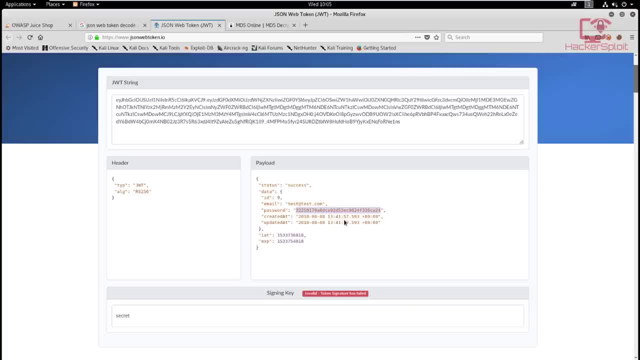 or a hashing algorithm for the password. the first thing you need to do is identify what it's using and then you go about decrypting it. Now, I'm not going to be talking about the other parts here, because that's a bit. that's a bit advanced And, as you can see, by default 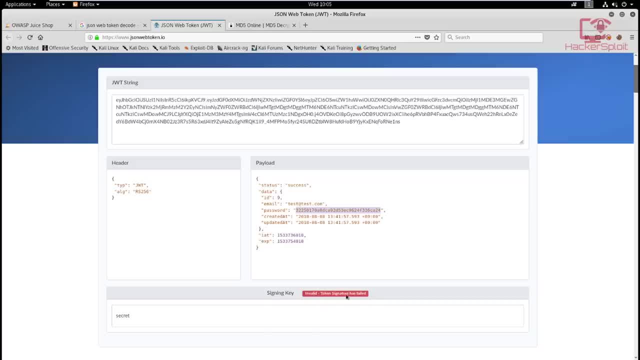 the signature. the token signature failed, which means we can tamper with this token and we can make changes to it And we can authenticate with it Because, as I said, the OS view shop is is designed to be vulnerable And this is where you perform all of these tests. 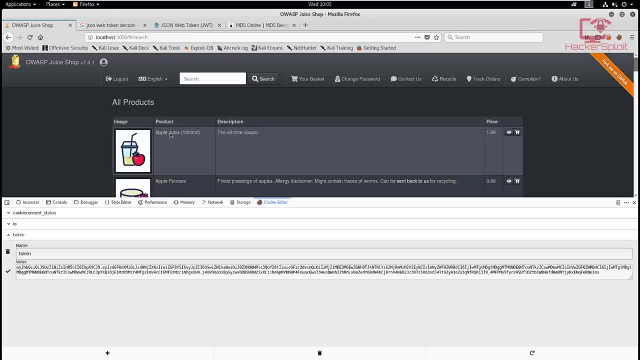 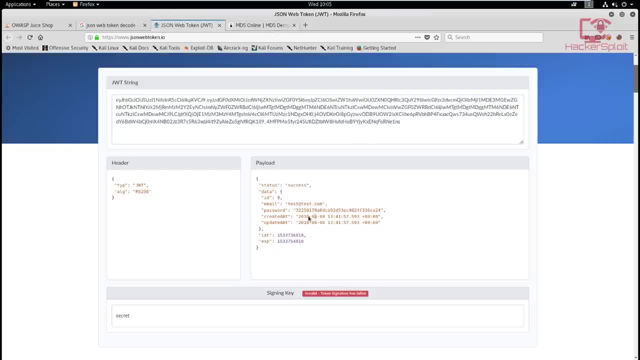 Okay. so when it comes down to the payload, the most important things are to look for the status, the ID And, obviously, if you can get any other information in the data section or in terms of the email and the password, that's also very important. Now, of course, it's not very easy. 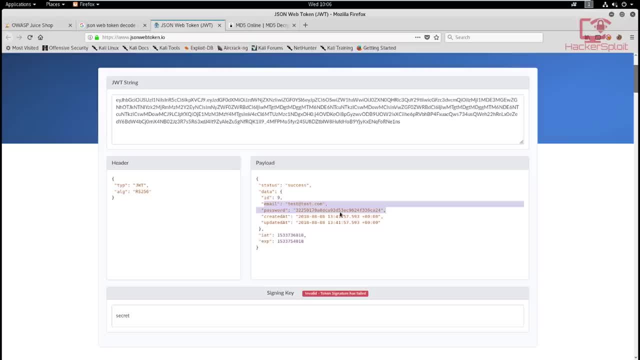 to get a hold of someone's, of someone's token. but you can do it. But and then you are performing the penetration test on the token. Because if someone wants to write in the comment section of this video, what if I was to grab the, the authentication token? 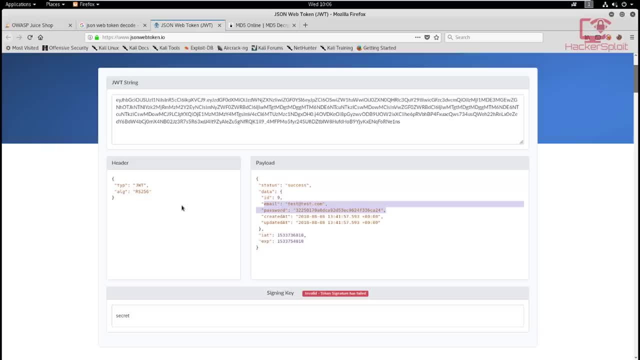 that belongs to Facebook, let's say, had access to someone's computer for a few seconds and I was to get the authentication token. what would I be able to do? Well, first of all, you have to test the security of that token, And I can guarantee you that their tokens are. 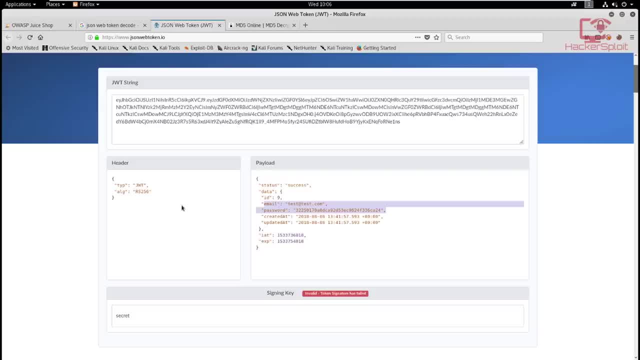 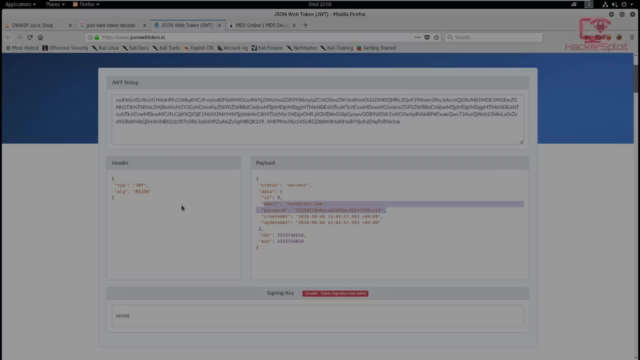 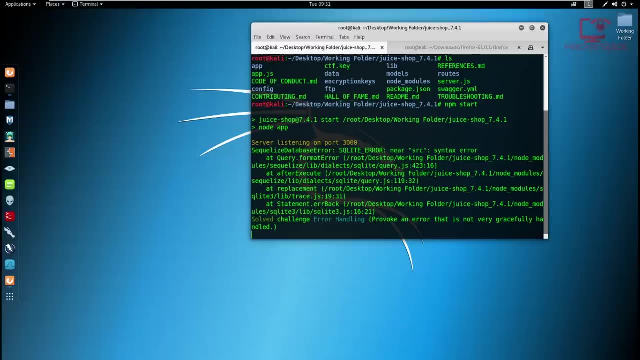 going to be very well secured and performing the penetration- the penetration test- on them will be a different ballgame, So we'll be looking at changing them or or tampering them to give us different types of access. We're going to be talking about HTTP attribute attributes and cookie security. I am currently running OSBJU shop. 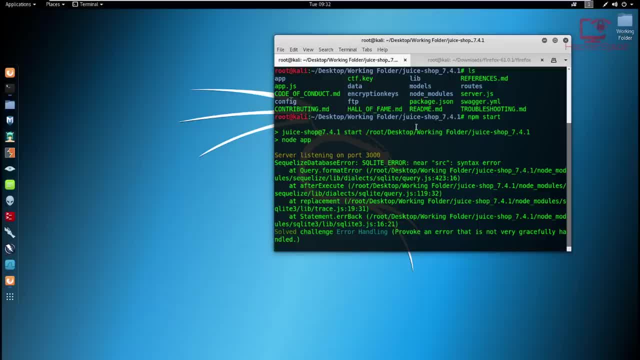 And what I did is I started a fresh, new instance, So I unzipped a new OSBJU shop. That's because I wanted to start a fresh and, of course, in the previous video we looked at cookie analysis and tokens, But now we're going to look at how, at the security aspect of how these cookies are secured. 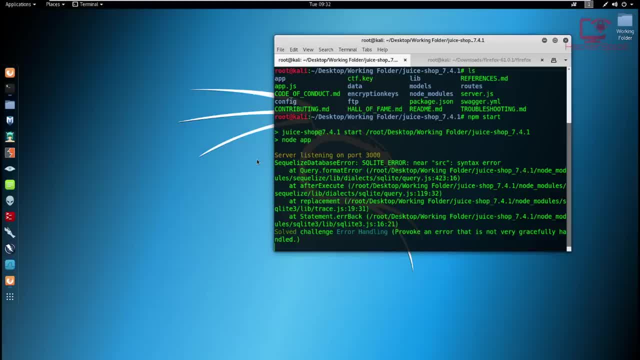 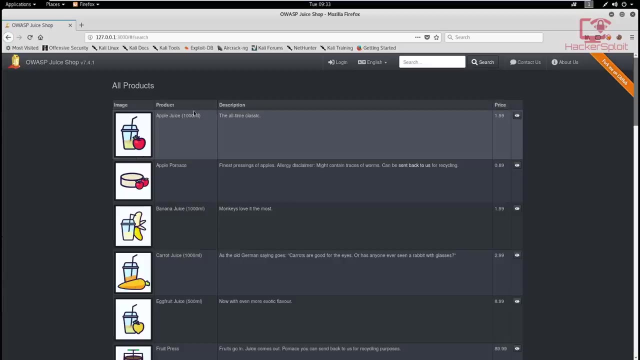 and how you know how cookies are stolen and how these can be exploited with, with with other exploits or functionality like cross site scripting. Now you'll get to what I'm saying in a few seconds. So I have OSBJU shop running And I've created the same user and password as 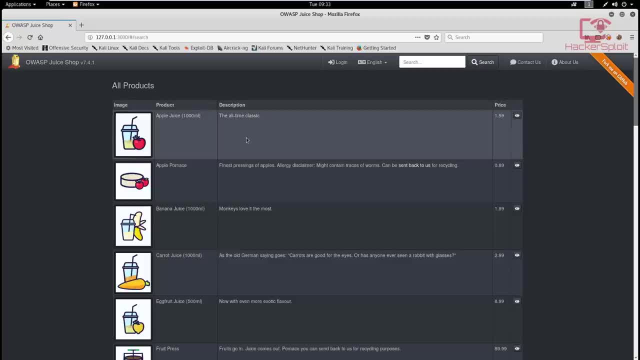 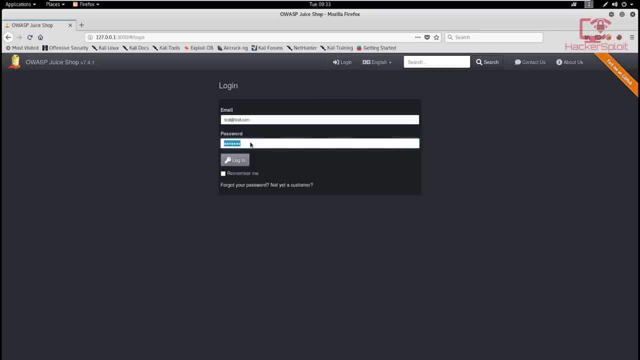 I did last time, So it's a test at testcom, That being the email, and the password is password 123.. Just so you know, and I'll do that right now I'm just going to log in, as you can see. test. 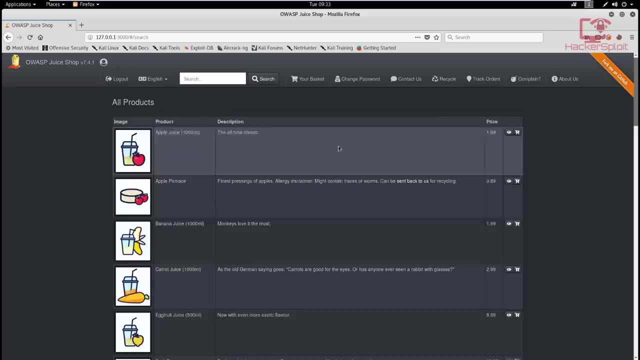 at testcom And the password is password 123.. So let me just log in. And there you are. So I've logged in and haven't solved any challenges. So when we talk about cookie security, what do I mean? Well, this can be done or can be inspected really easily. Now, of course, for this you're not going. 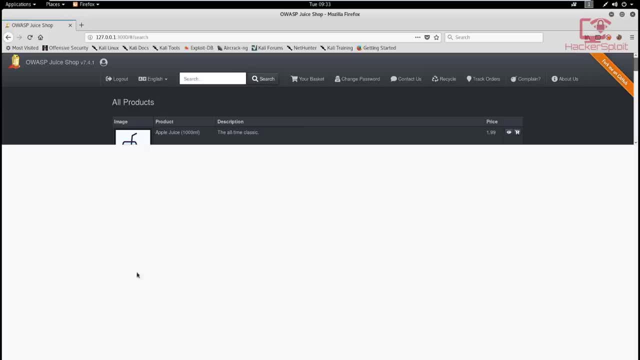 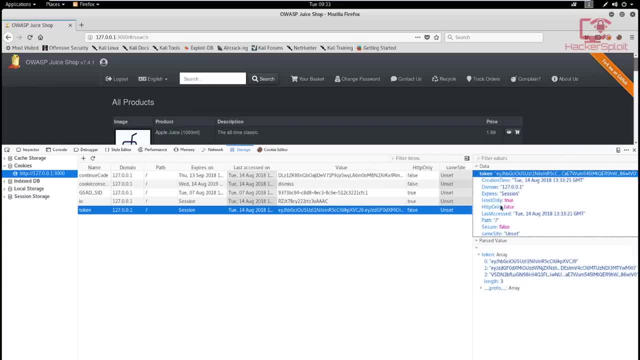 just look at the data. you know that we can see within the token. If we go to the HTTP only section here, you can see that that is set to false. Now what does that mean? Well, that means that we can potentially exploit this cookie and its storage location in the sense that it is. it is 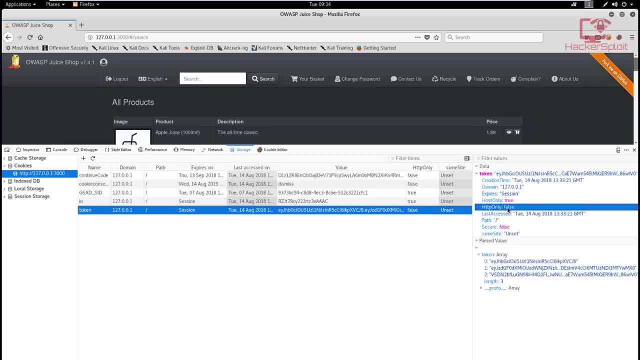 it is not secured. Now I'll get to why and how this is happening in the in a few seconds. Alright, so if the value is set to false, it means that the value is set to false. So if the value is set to, 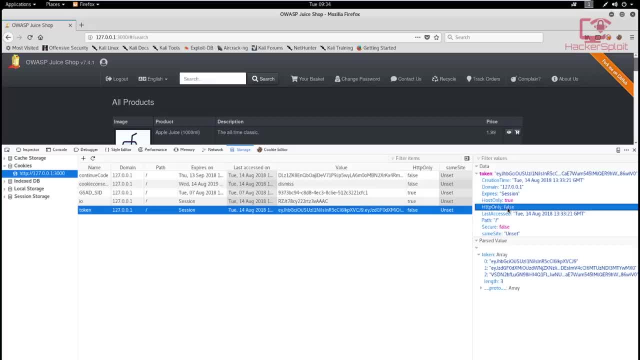 false, it means that the cookie can be accessed and written to. now how can one use this, you know, for potential attacks or cookie cookie stealing as we know it now? if you are an advanced web application penetration test and you know about cross site scripting, you know that usually. 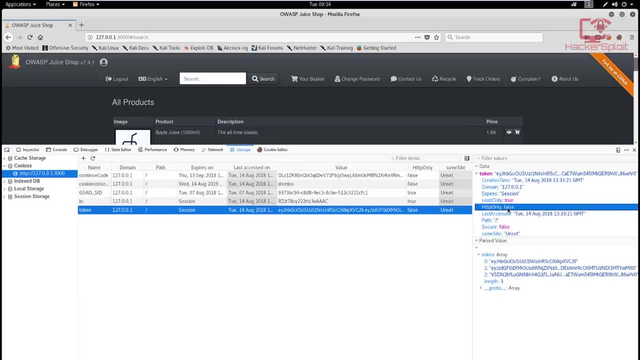 attackers will use cross site scripting to steal cookies by sending you links that then you know, by sending you links to pages on the site that you're already authenticated to that have the, the malicious JavaScript code that will then send your cookie, your authentication cookie, with your. 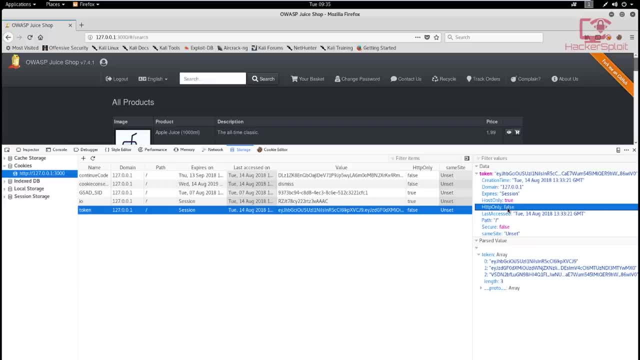 token, etc, etc. to their attack server And from that they can then use that to authenticate into your account. It's not common because mostly the the cookies are usually secured. Now you will run into sites that have this and this is a very, very big vulnerability in terms of severity. So if you 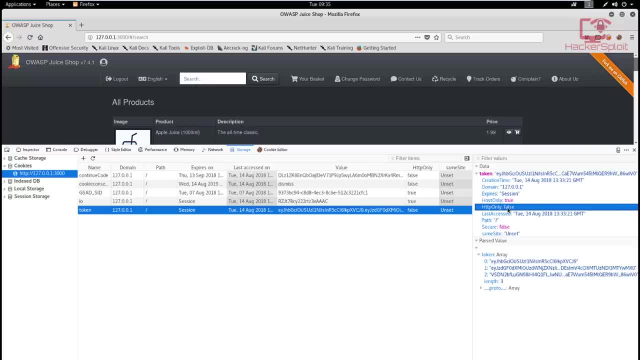 are a bug bounty hunter. this is in the medium to low category, So not really a big exploit, But still a very, very big problem that many, many, you know- usually, I would like to say, rookie developers miss, especially when dealing with huge frameworks like node, etc. I'm not going to get too deep into 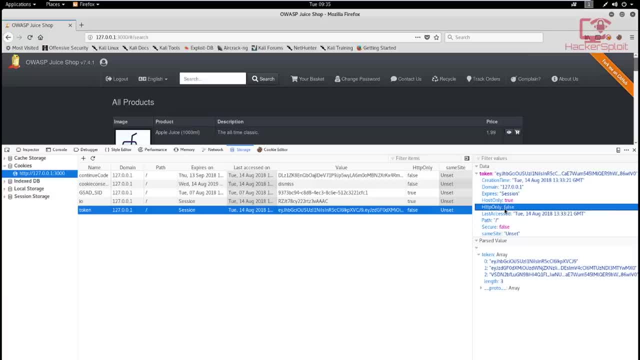 that, So you can see that the HTTP only is set to false. Now, what does this mean? This means that we can use, utilize a lot of functionality to exploit or to display the token, or, even more, to send this the my cookie or you know my token, whatever you want to call it, to a server, or to say: 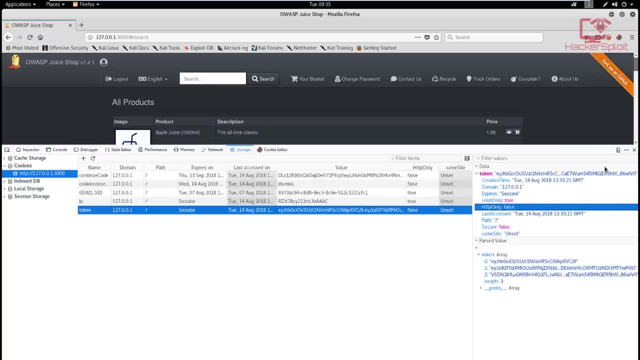 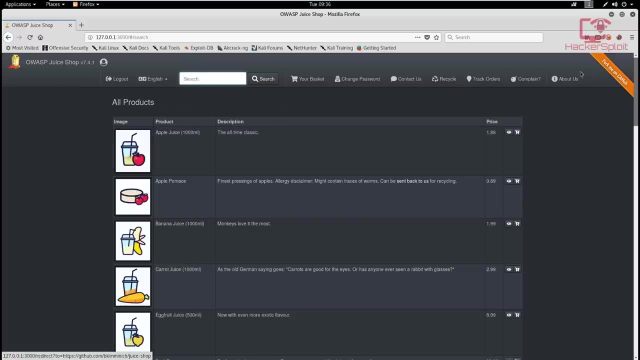 it all right to grab it, to steal it, you know, simply put. So how can we exploit this? Well, we can use cross site scripting, And this is probably the most used method for this. And to do this we can, simply, we can- use any of the, we can use the search or we can use the contact, But I like using 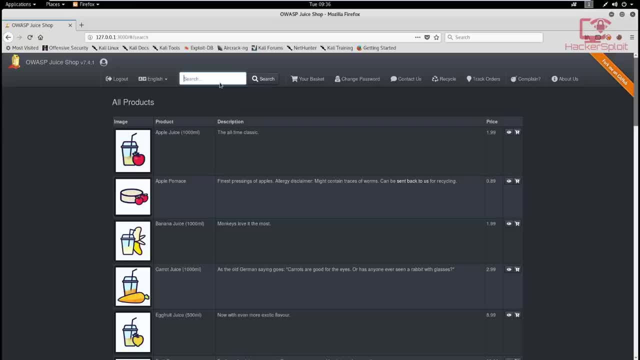 search because usually it is unfiltered. Now, when I say this, I'm you know, many of you will say: well, most of the big sites. well, I'm not talking about the big sites, the big sites. obviously I have to take this into consideration. I'm talking about sites that are developed by small. 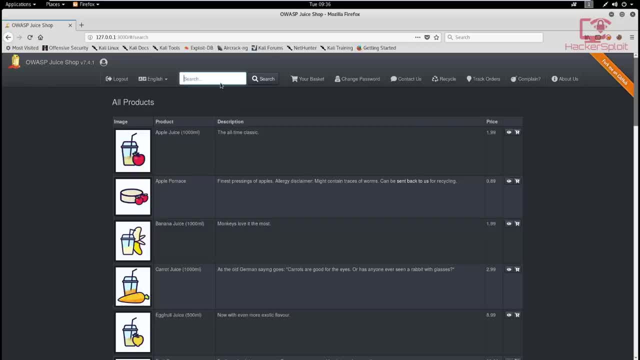 teams. they usually don't take this into consideration. So if I was to just type in a simple cross site scripting script, that will essentially display my cookie right now, as I'm authenticated. So to do that I'll just type in script, And for this we're using an alert here. 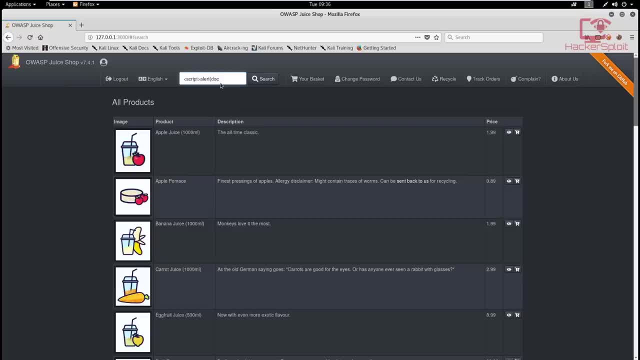 to display to us So alert, and we're going to say document, whoops, stop, sorry, document dot cookie, And then we're going to just close the script, like so. So this will display our cookie to us. not really helpful, But you can imagine if we were to have this permanently posted. 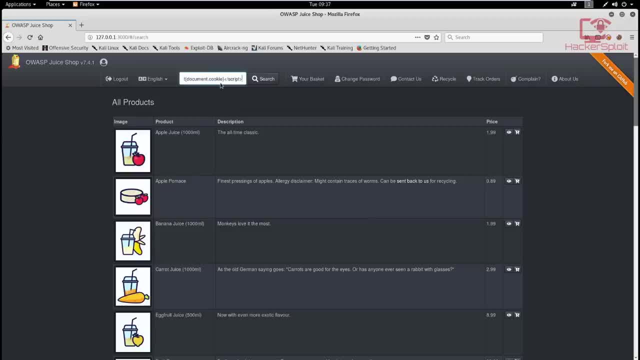 for example, as a post here, And then whenever we send that link to someone and they click on it, we can customize this JavaScript code to send their cookie to our web server And once we get the cookie, you basically know what's going to happen there. So if I hit enter to search, 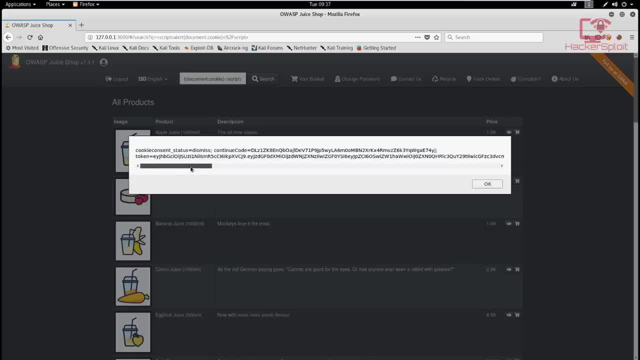 you can see that it's going to display our cookie and our token, And this is extremely dangerous. You might not get the context, but I'll explain it in a second. So essentially, this information can be passed and sent anywhere across the world, provided that the that your 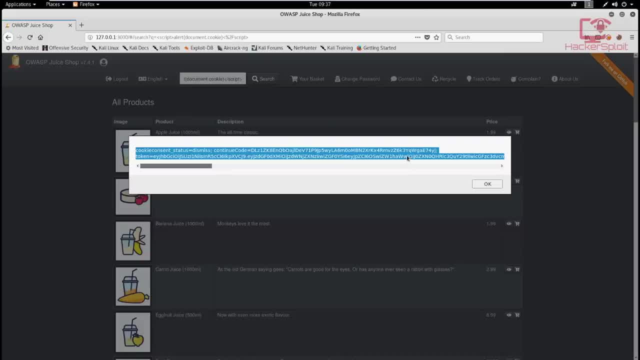 target clicks clicks on a link in which this, this script, is executed. Now the question that you might be asking yourself was: well, where else can we post this in sort of a malicious way? and I know that I sound malicious right now, But I'll also get into how to mitigate this, And again, 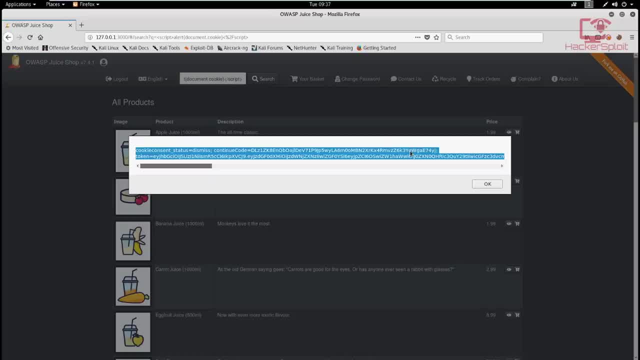 mitigating. it is really simple. Just set your HTTP status or your HTTP attribute to true or set it to on essentially securing your cookie. Now you can see that, once we have this, you saw in the previous video what we could do with such information and what info it contains in regards to the user, And now we can. 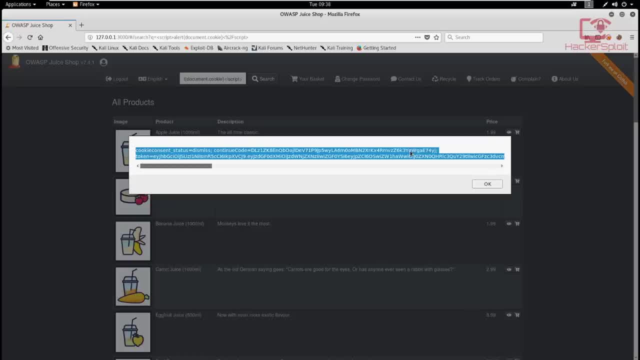 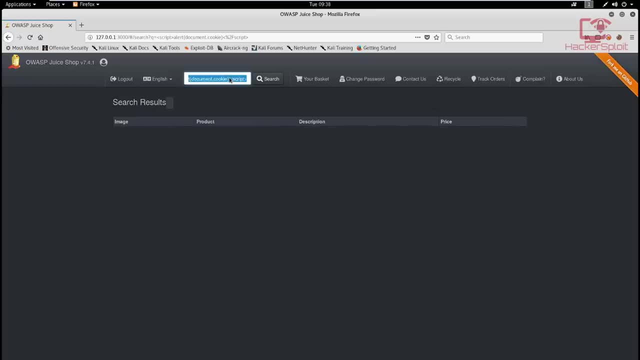 we can, you know, crack the password, But for now let's focus on how this can be utilized to steal the cookie or how attackers do it. So you can also get insight. if you're a white, so usually I can post this in here, I can put you know, I can type the script in here, But this: 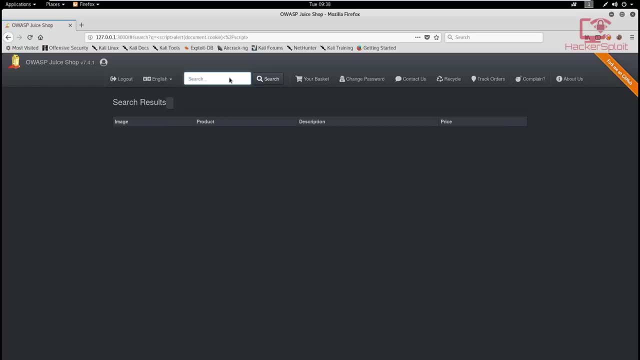 is not. it's probably not the best way of doing it, because you essentially have to convince the user to go into the search bar and type this in- not really the best of ways about going, you know, about going about this. So usually we look for a page that allows us to, you know. 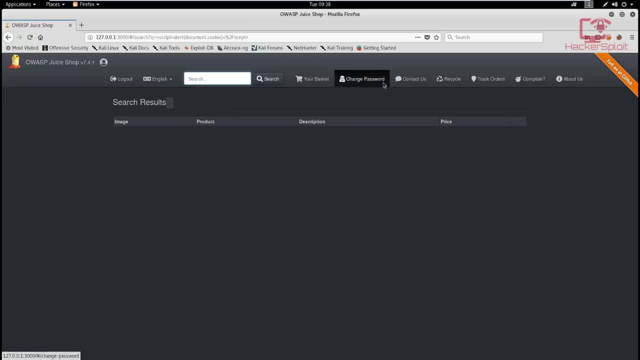 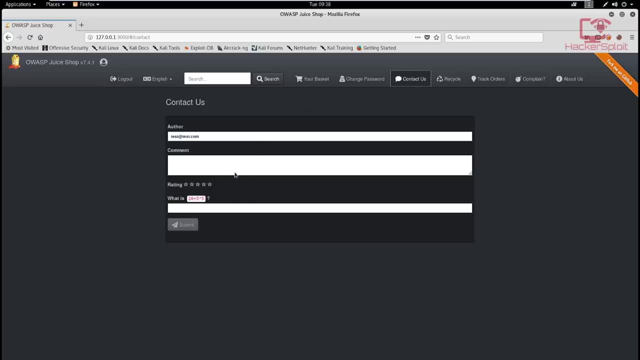 to post our own stuff or to save this to a database or to save it to the website itself. So let's try. contact us. Alright, so contact us. Yeah, that looks like a good place to start. So in the comment it's already added our author for us. So in the comment we can enter, we can enter our. 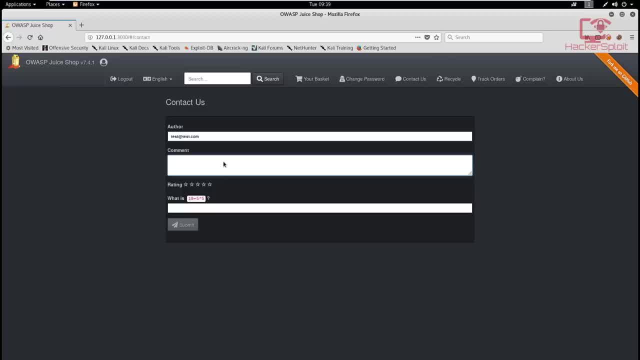 script in here And this will probably probably be saved, But we have to test it Now. of course, the cookie stealing JavaScript code is not something that I'm going to be telling you how to do. you can probably perform a lot of Google searches. It's part of the terms that I have to 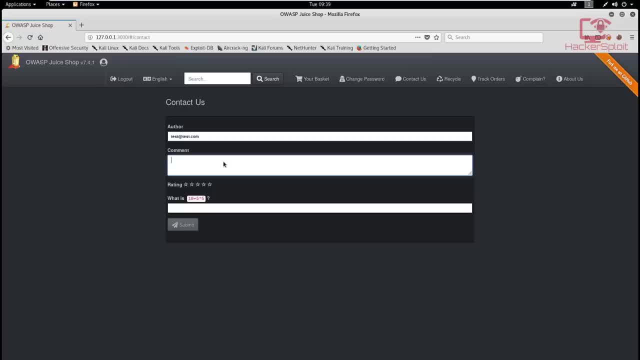 follow in regards to YouTube's, YouTube's policies about malicious content and when whatnot. so I'm not going to show you the exact code, but I'll probably have it on my website if you want to take a look at it and experiment as to how to send cookies to another server- a server that belongs to you, for example. 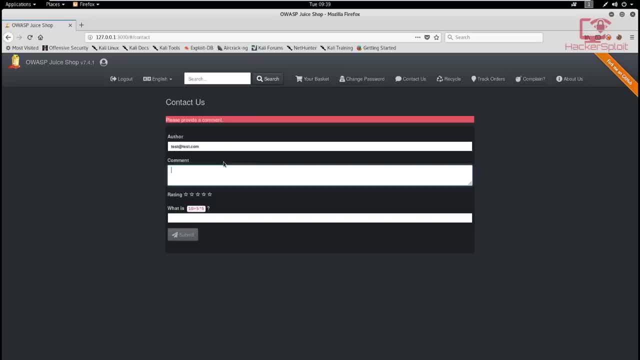 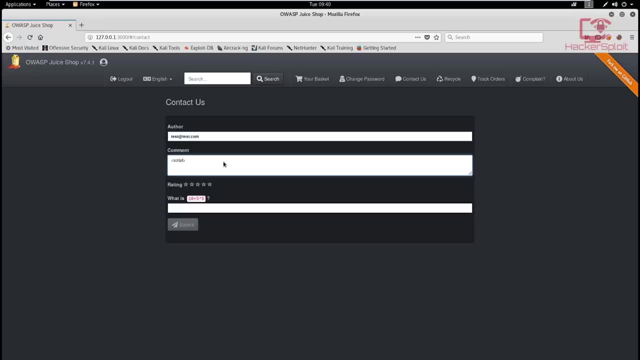 So to do this. so now, essentially, what I want to do is I want to save this script into the contact section, because I believe this is saved. If I looked, I looked at the structure And indeed it is saved. So the script is quite simple, So we can say we can give it a title, because I know 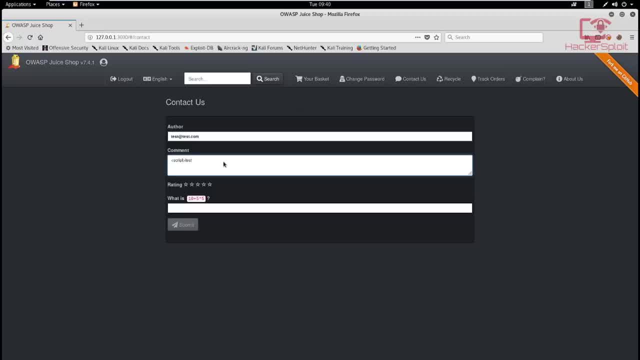 the feedback is left like that. So we can say: script test and we can close the script here, So script. but then we have to include the, the actual JavaScript code. So yeah, so let's include this script within the main one, So script. and then, once we close this one, we can then use the other. 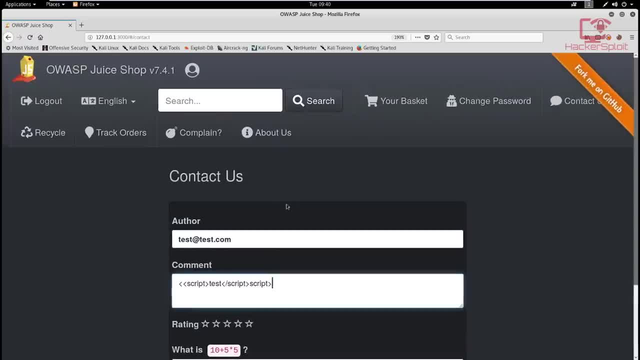 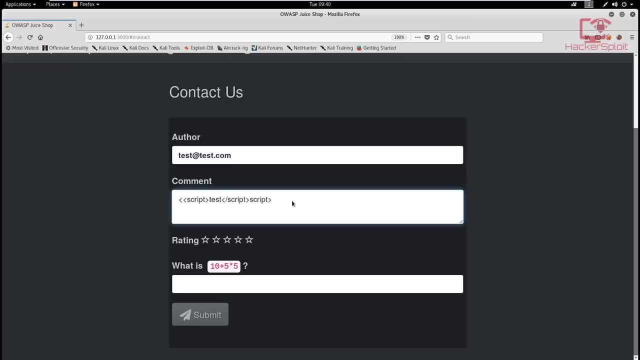 script. So yeah, script, oops in. you can copy this code if you want. by the way, let me just zoom in, because a lot of you had actually talked to me about that, that you couldn't actually see the code. So script and. 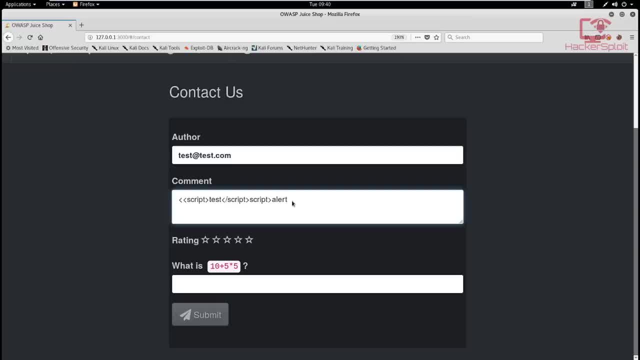 now we want to bring up the alert Now, of course, as I said, this is not really useful because all you're doing is displaying the cookie to the user themselves once they visit this page. So, you, you, you probably get the idea. So, script alert and we are just simply just going to write the. 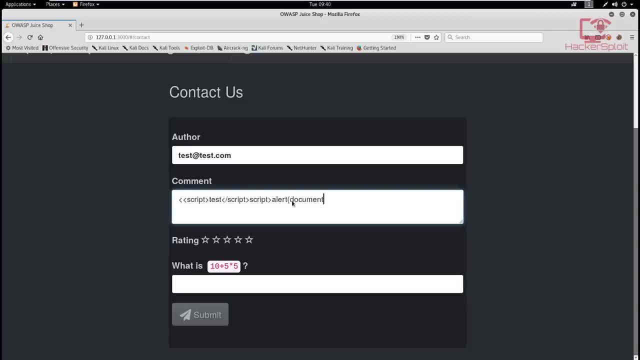 document, Of course, if I'll say sending it to a malicious server. what I would have done is I would have used the document dot cookie and I would have appended it to be sent in in the form of, probably, a PHP file or a PHP get. 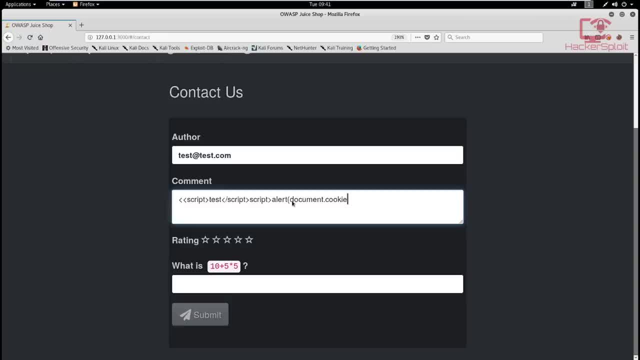 request to my server, and then my server would log all of the information being sent back. So that's the concept there behind. So we can then close the script here. And sorry, we have to actually close the script. Oops, sorry, my bad. And then we close the script. And then we close the script, And then 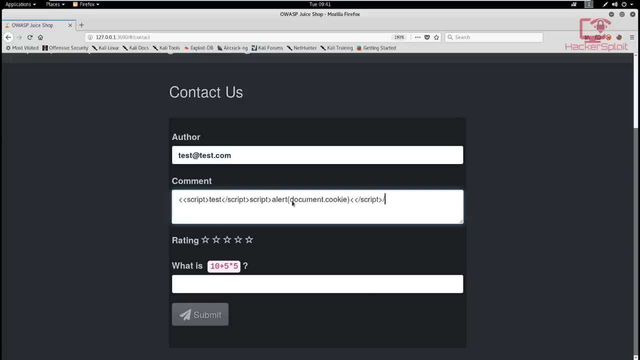 we close the script there And finally we can close the final script ending here. So script and there we are, And we can leave a rating if we want to, And there is a capture here, or authentication: 10 plus five, you you basically have. this is also an exploit here that you can. 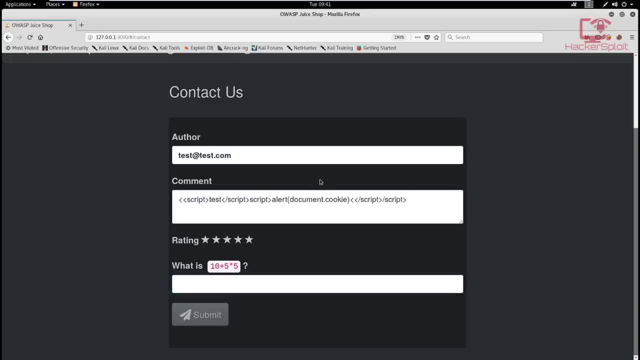 enter. Because if you look at this very, very, very basically, from a simple perspective, the capture here is again is another false positive, And again, I know I'm dragging this, I'm dragging it a lot, But. But what I'm trying to explain here is: if you are going to, you are. 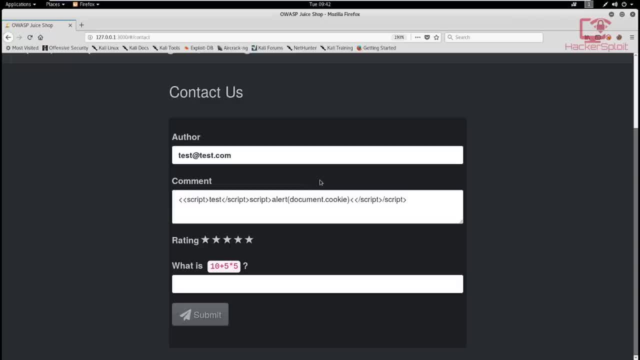 going to be performing a penetration test on a website. you need to understand that, from the perspective of false positives, you should not go after the big exploitations or the big exploits first. Alright, so if I submit this, as I know the structure of the OS view shop, this will be: 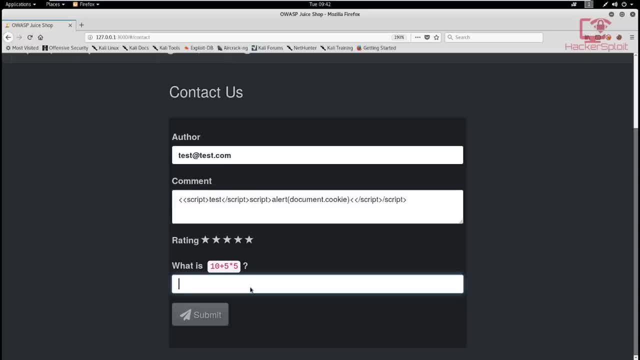 submitted to one of the pages in which, after I click or any other user who is authenticated clicks, will will run that script or this script and will the cookie will be displayed on their screen And, if you want to manipulate or use your own script, to send their cookie to your server. 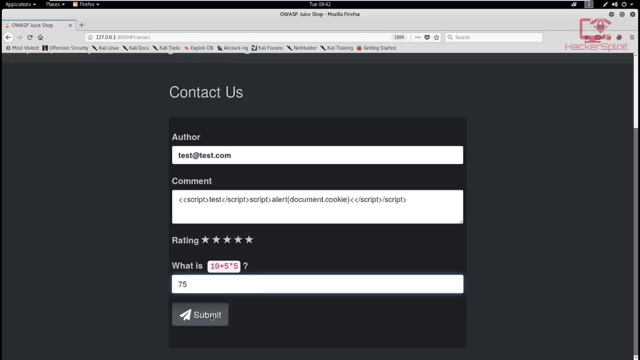 by all means go and do that. I'm not condoning it. So that is 75. And I hit submit. And what? that's wrong capture 10 plus five, actually 25.. Yes, brackets, of division, multiplication, addition- you guys must be thinking I suck at maths. So that is 25.. 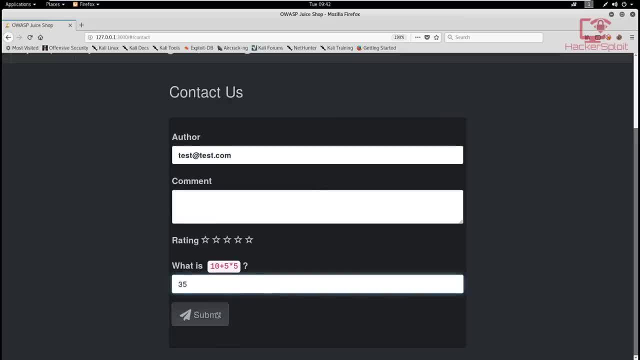 Plus five plus 10.. Sorry, that's 3535.. And I submit that. oops, we have to actually type our code back in. Sorry about that, guys. So we can just type in script and we're simply testing. 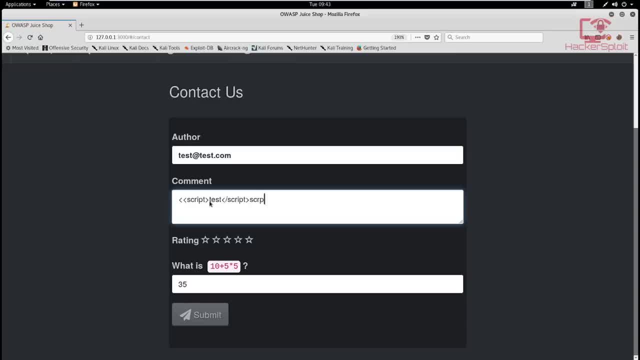 test And then, after this, we can close the first one and script here- Oops, sorry about that, My keyboard is quite a distance from me. I let- and my spelling mistakes are really annoying- Script and finally we can use the document. My God man, my typing document, dot alert, dot. cookie. 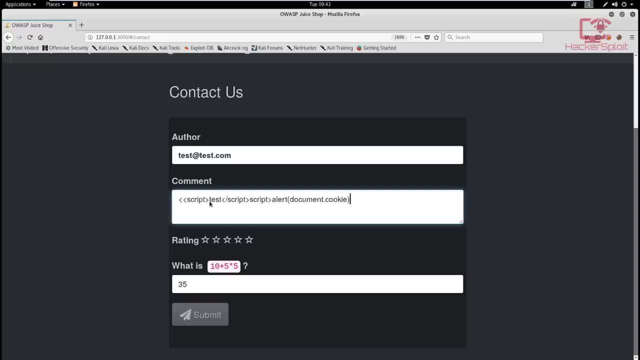 sorry, we have already sent the alert. we would use the document dot alert would essentially display the entire web page document dot cookie. And in here we close the first script And, sorry, the initial script And then we close the last one here, So script And we close that right there. 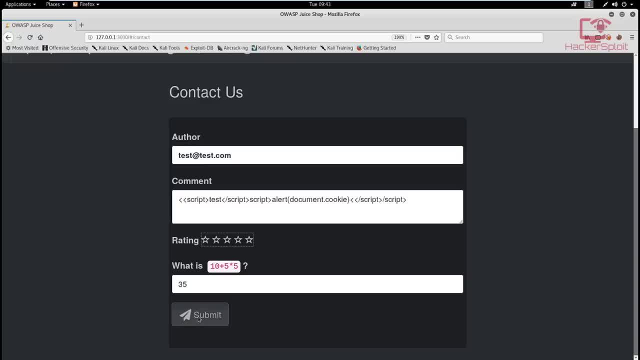 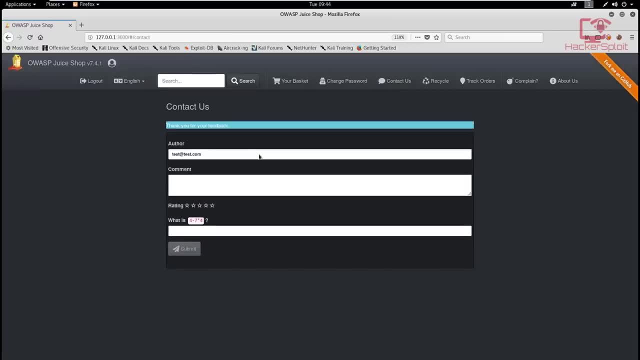 And finally, we can give this a rating and we submit, and that should submit it. I don't know what the issue is. here And there we are was for some Alright, so there we are. Thank you for your feedback. So he did submit it there. Let me zoom back out Now. you can see that. where would you? 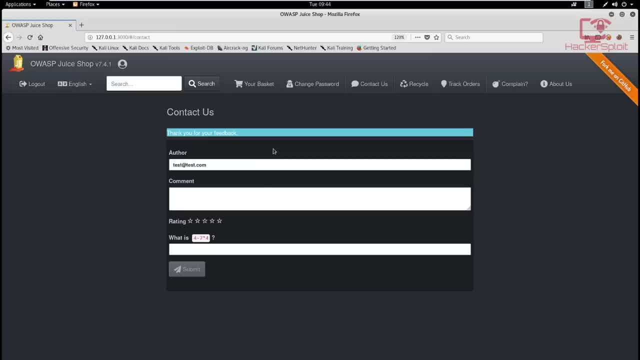 go to launch this script. That's that. that will be the question that you might be asking. So, on this, in this structure you can pretty much experiment with all the other pages And again, I do recommend that you use, you know, direct. 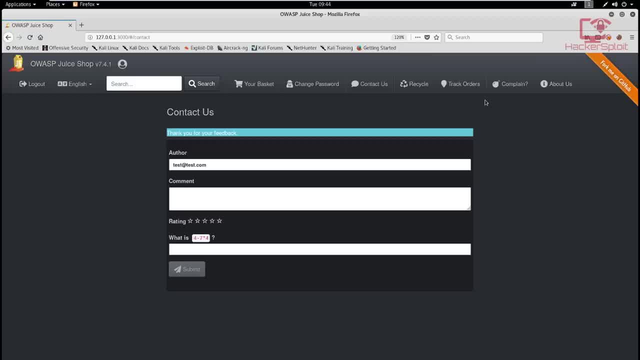 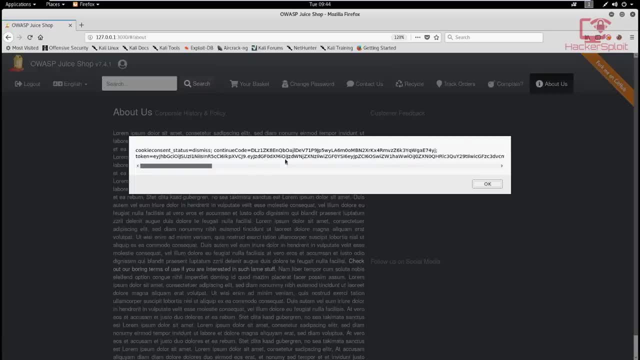 tree discovery tools like the Buster or go Buster, whatever is comfortable for you. So, with this in mind, if first we just click on about us, you can see that that is where the, the feedback in regards to contact is stored. So there you are, there's the cookie. And if I was to, if I was to 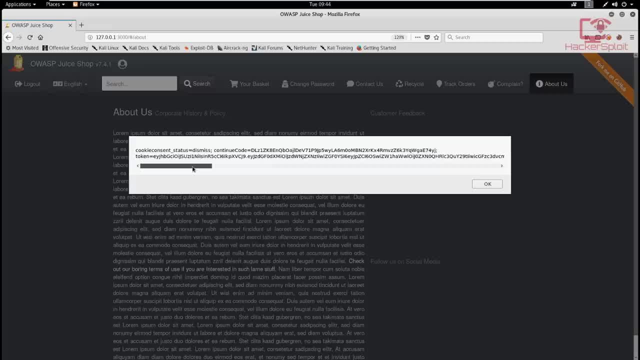 have implemented a script that would send the cookie to my server once I access to this page as an authenticated user. it would send my, my session ID, all of that good stuff- to my web server and I'll be able to crack the password and. 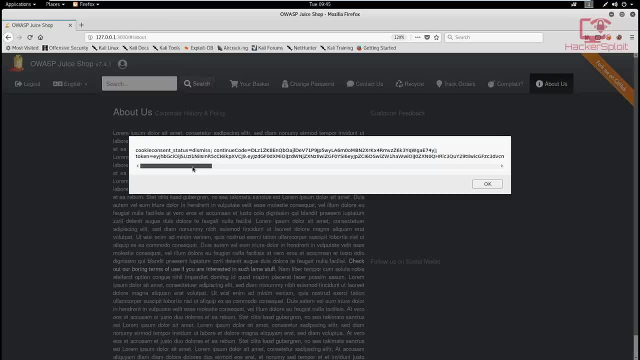 authenticate with your account. as simple as that, without ever knowing your password, without ever trying to have guessed it, without, without ever trying to have exploited your system, I exploited the web application And, because of the- the inability of the developer of the web application to secure the cookies, I was able to get into your account, and God knows what else you can do in that. 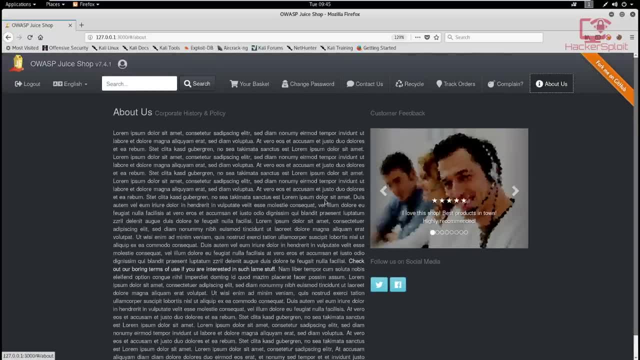 person's account This is. you know, this is tribute to my all my Facebook hacker friends out there who think hacking Facebook is is about cracking and brute force. There you go. you know, applications can can be cracked in or can be exploited in different ways. Now, of course, 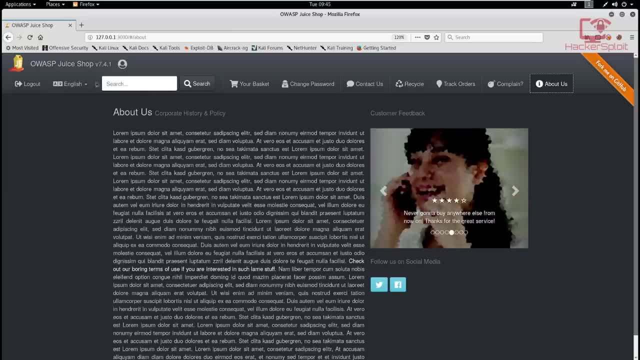 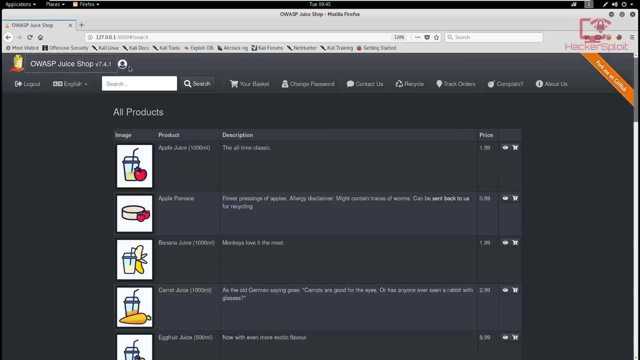 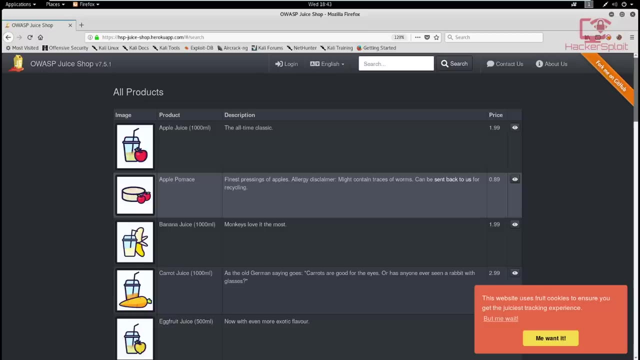 I said, it's going to get really exciting as we move along with do shop And that's the reason I'm using it, because it explains how this can be done on a real website. And yeah, we're going to be looking at OS juice shop And it seems to replicate what a real web application. 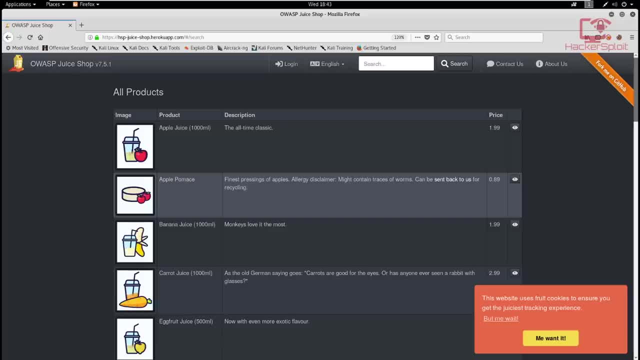 would be a fairly poorly designed one, But the thing I like about it is it has varying live levels of difficulty, And that's really, really awesome. I have it set up on Heroku, as you can probably see right over here, And that works perfectly fine for me because I, you know, I wanted to set it up. 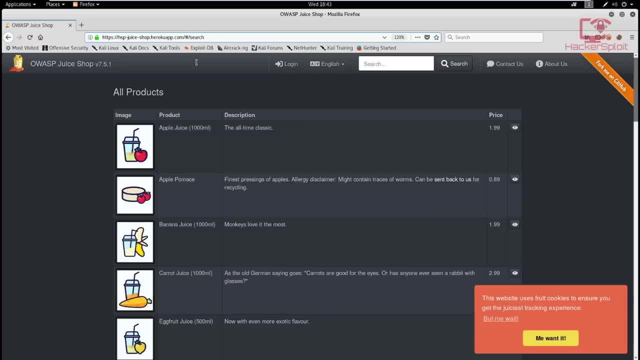 really quickly. I don't want to run it on my local server, you know, using node or Docker That's. I really didn't have the time to do that. But if you want to, you can. you can use Heroku and it. 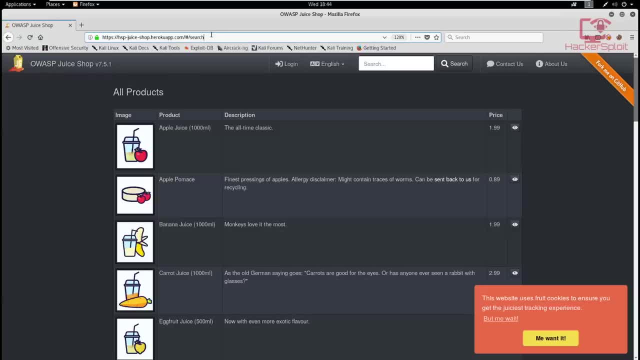 should be free for you. So, yeah, definitely go ahead and give it a try, And you should have an instance set up for yourself So you can go ahead and do it. And it's giving us a prompt here telling us that this website uses fruit cookies to ensure you get the juiciest tracking experience Now from 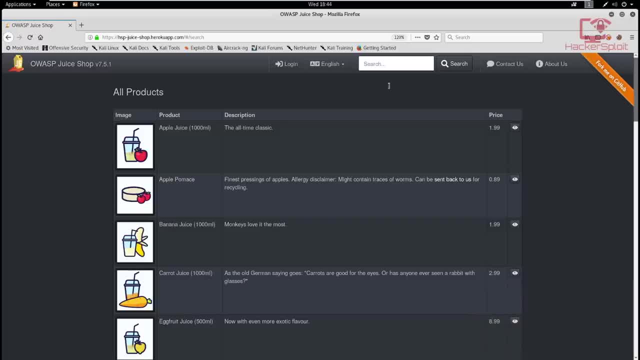 my experience, I would hit accept the cookies because essentially that's what keeps track of your progress And yeah, that's pretty. that should be quite good. Now, as for my browser, I'm using the latest version of Firefox And I have you know plugins or add ons like cookie editor, And that's pretty. 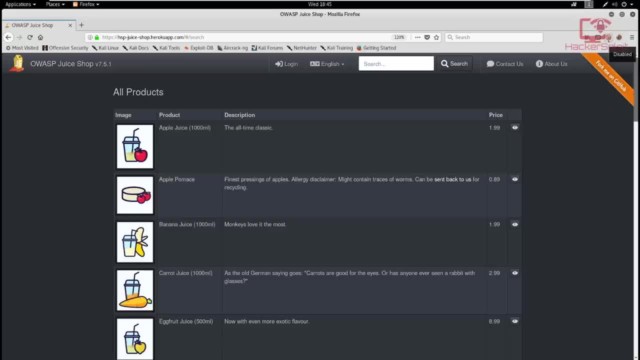 much what we'll be needing in this video, I hope. And we don't have the, the proxies here, like sorry, foxy proxy- to allow us to use things like burp, suite or zap, whatever you want to use. Okay, so let's get started Now. the first challenge, as I believe, is to get the, the. 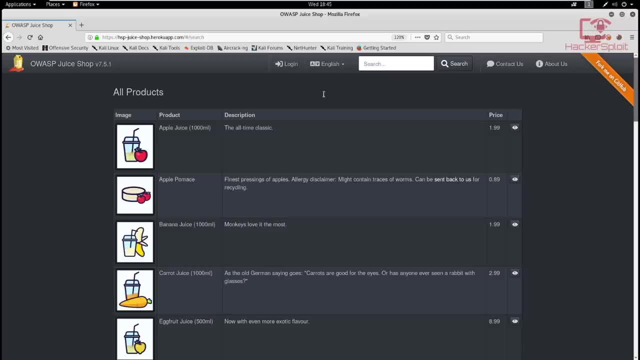 scoreboard And we should start from there And to do this. I think I have done this already. That's really very simple. All we need to do is well, first of all, before we actually do that, the interface is quite simple. It is a juice shop, as you probably can see and could have understood. 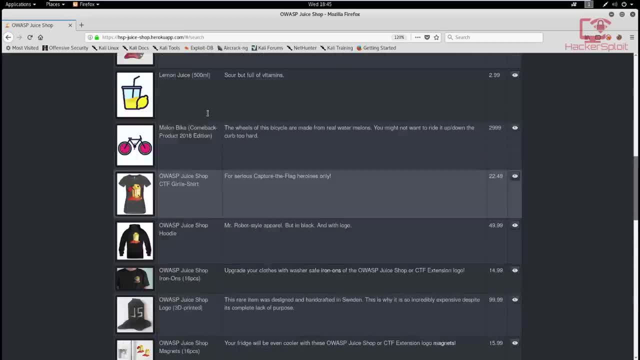 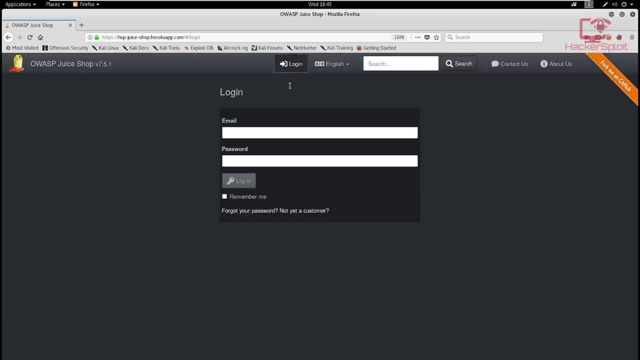 And they sell juice. Now, the great thing that I like about OS view shop is that this replicates a real life web application with, you know, security, misconfigurations, etc, etc. So if I log in, you have your login page right here And then you can see that the interface is quite simple, So you can. 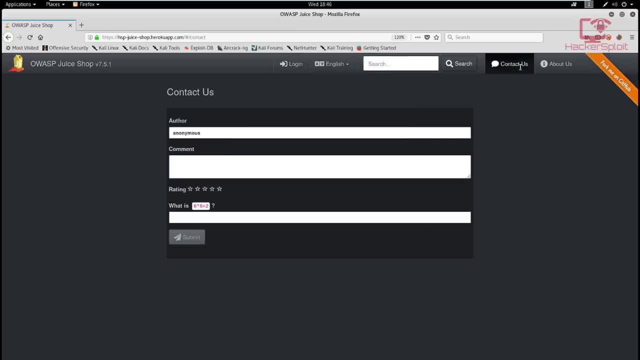 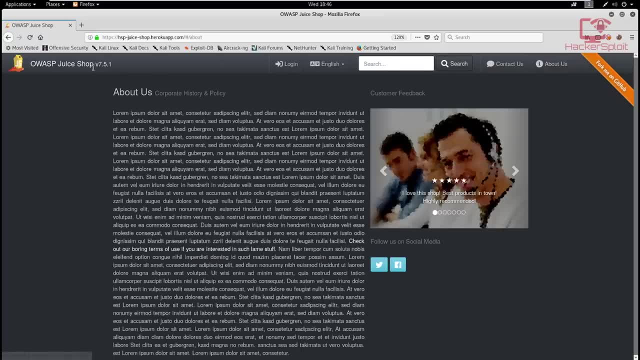 right over there and you can create a new account if you want to. you can search with a contact us page that allows us to you know, essentially contact whoever is behind the site, and we have an about us page, And the thing I like about this is, as I said, it replicates what I 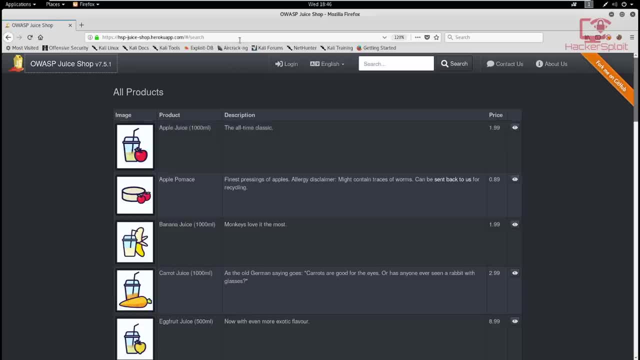 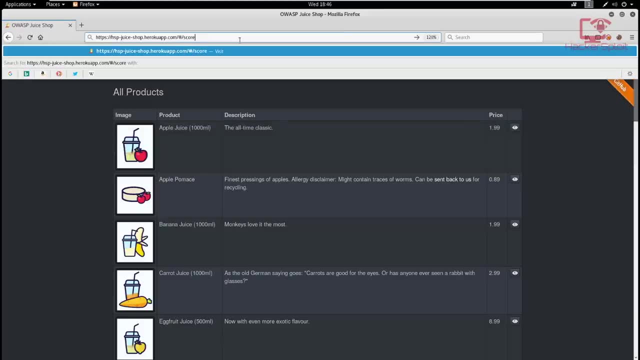 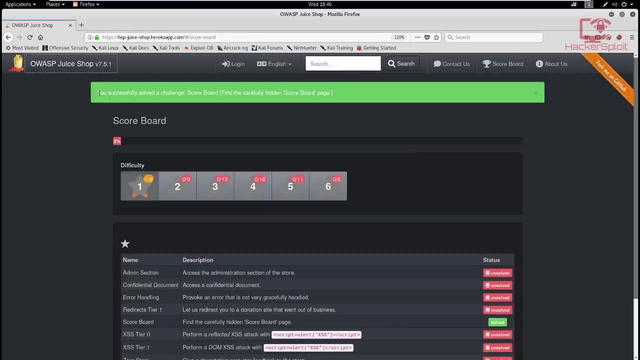 would call a real web application. Now, when we talk about about the scoreboard, I think that can be accessed really, really quickly by going into scoreboard, like so. So you know we can just hit scoreboard And if I'd enter, that should give us the scoreboard. Alright, so it gives us the notification Once you've completed. 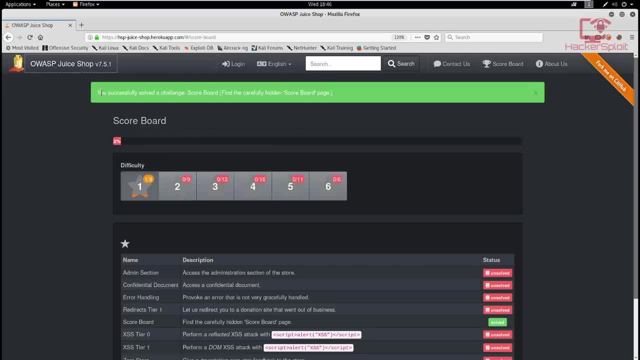 a challenge, and the reason it does this is to notify you of your progress. Remember, this can be considered a capture the flag type of challenge, but I wouldn't call it this. I think this is fantastic for essentially explaining the concepts here. Alright, so let me explain how the scoreboard 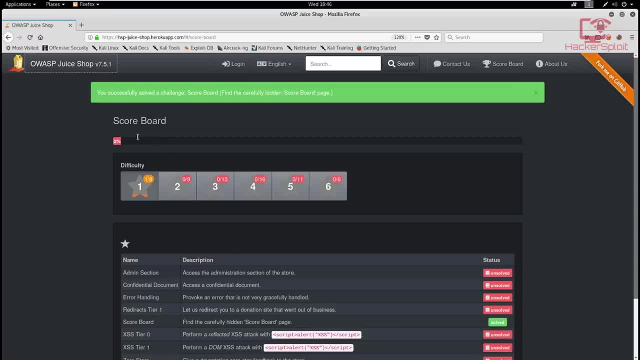 is essentially works Alright. so your scoreboard is as follows. Sorry about that, if you had my phone, it always seems to do that. So we have. we have the challenges sorted in terms of difficulty. so we have a one star, two star, three star, four star, five star and six star, And they all have. 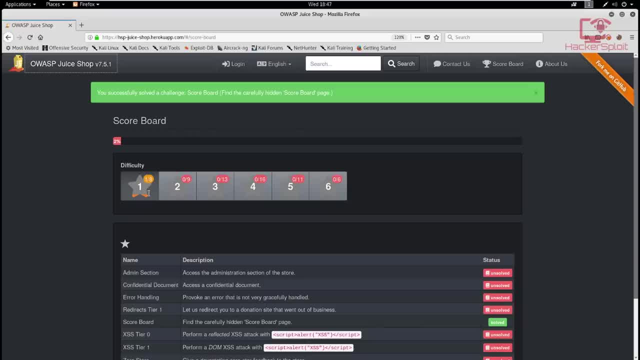 various challenges within them. So, for example, the the difficulty sorted in terms of stars. so you get the idea. one star is quite easy. two stars, you know, not so easy. we have three stars. things are getting a bit sweaty here. four stars- now we're talking five stars. I'm banging my head. 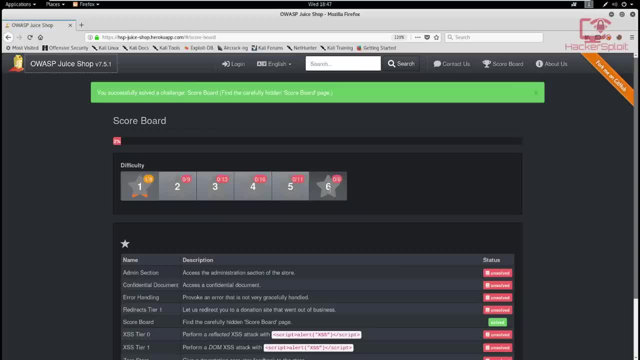 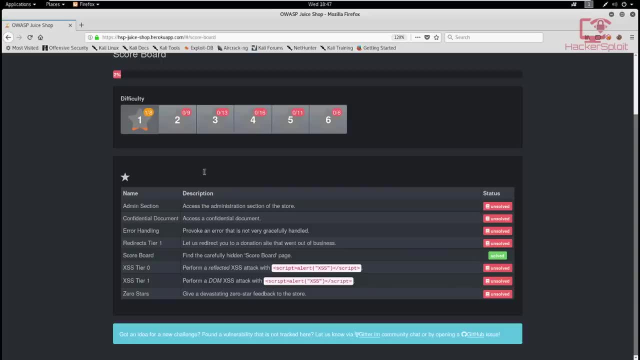 on the wall and six stars. that's going to take you probably a few, a few days or, you know, hours, depending on your detail elimination. Alright, so you can see it also gives you the. gives you the challenge names here. 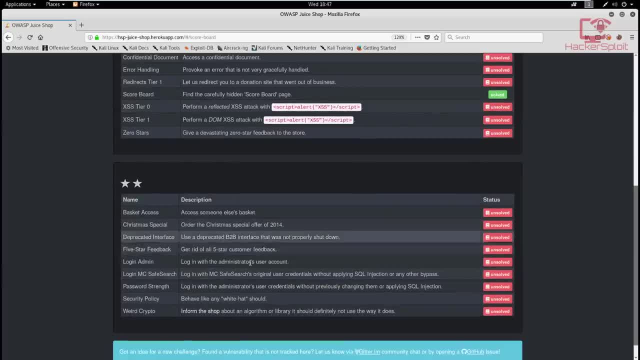 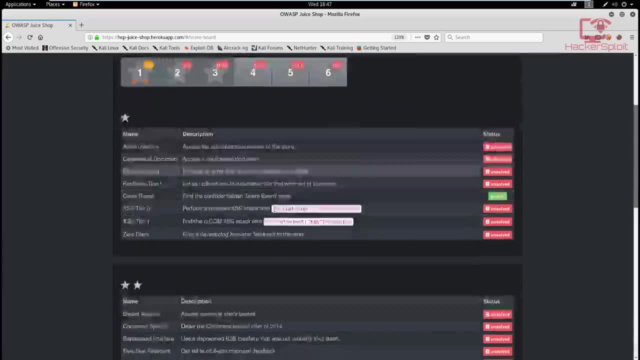 So if I click on the two star challenges, you can go ahead and look at the challenges there. And we- I think in the previous videos we- covered a lot of the two star and three, some of the four star challenges. That's what I wanted to go through. So the three star challenges are where. 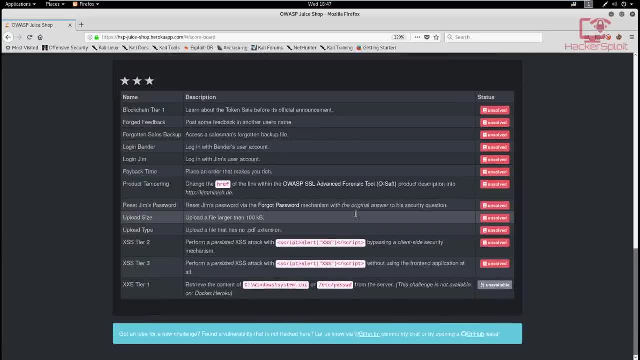 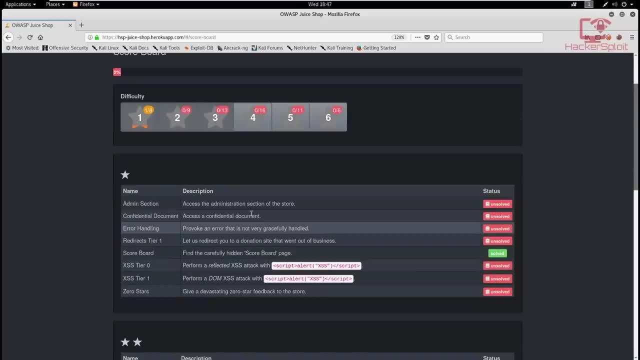 things get really awesome because it tells you start logging in with other users And there's a bit of cross head scripting. I'm not going to go through all of that. Let's start off with what we can do. Alright, so the first challenge in the first is access the administration section of the store. 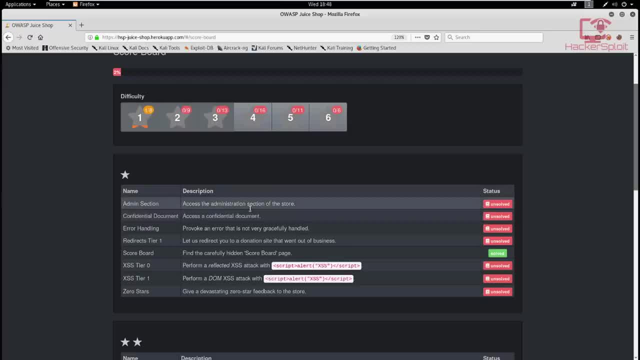 Alright, so I'm guessing we have to try and log in. I think I've done this. this is the first challenge. we have to access a confidential document, provoke an error that is not gracefully, very gracefully, handled. Not to show that is. let us redirect you. I'll try and cover as many as I. 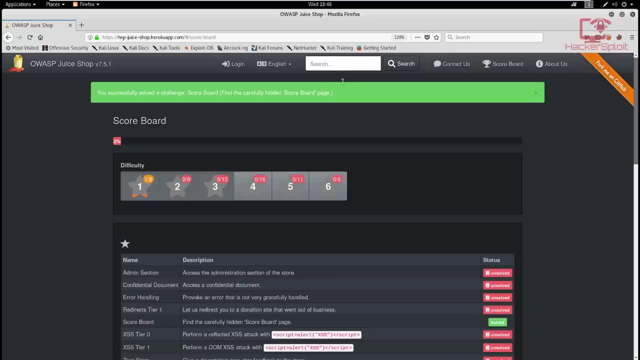 can. In one video we have a cross head scripting, Cross head scripting attack. This was simple. I think we covered this. So, yeah, we can pretty much run that in one of these right over here. So script and alert, as it already gives you hints. 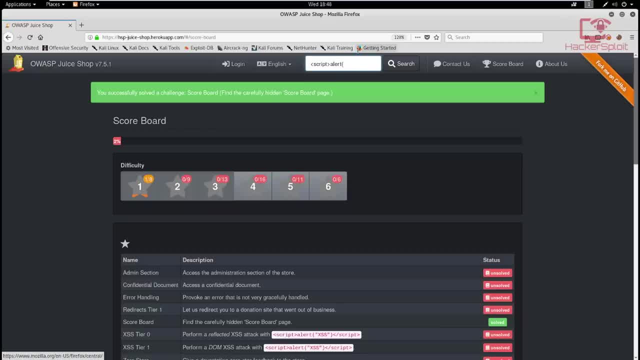 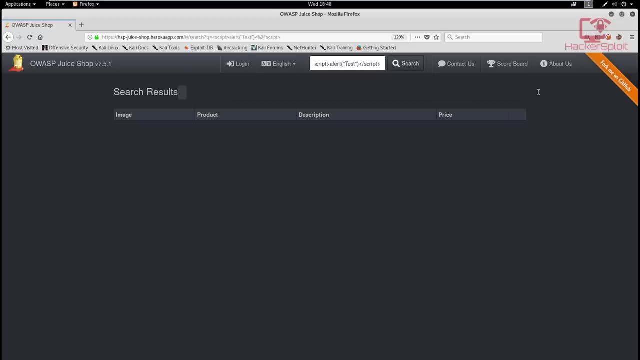 these are very, very easy. So you can just say: test, Have I given the oops? sorry my bad. So yeah, there we are, test And we close that up. And we also close the script right over here And we hit enter And there we are. So that is one of the challenges solved. Hopefully did pop up. 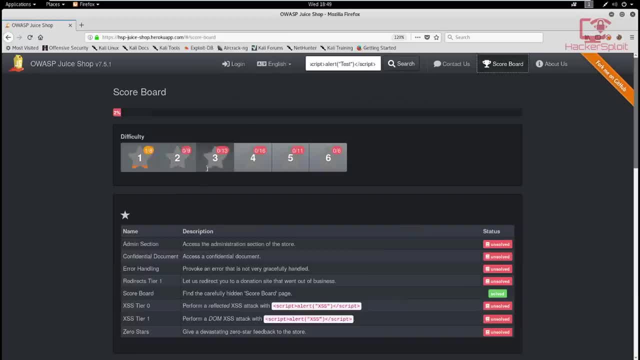 There. So if we go back to the scoreboard, it still tells us: well, for some reason the web application is too low. It's not told us that we have performed a reflected cross head scripting. All those are done, Alright, so reflected. Anyway, we'll get to that when we get to it. So if we 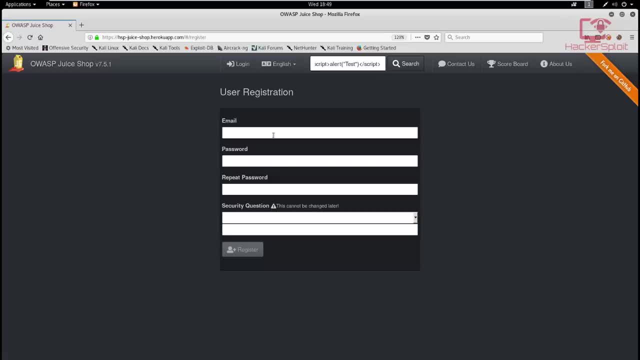 inspect the login page. what we can do is we can create a user. So I'm going to create a user here And I'll just use a simple user here called test at testcom, And the password: I'll call that password And I'm going to repeat the password here. 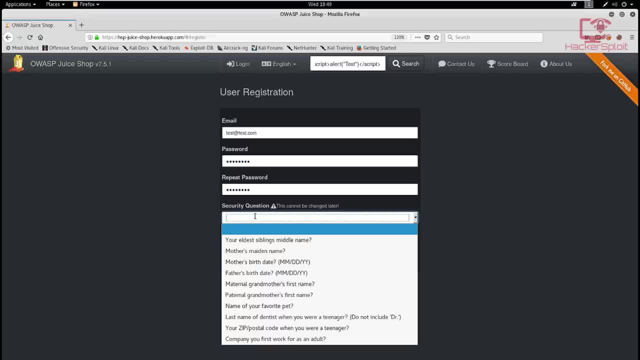 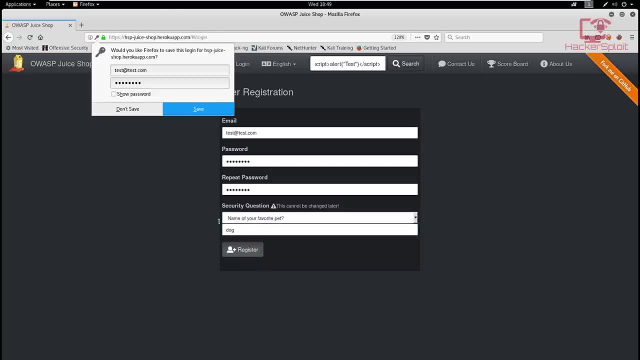 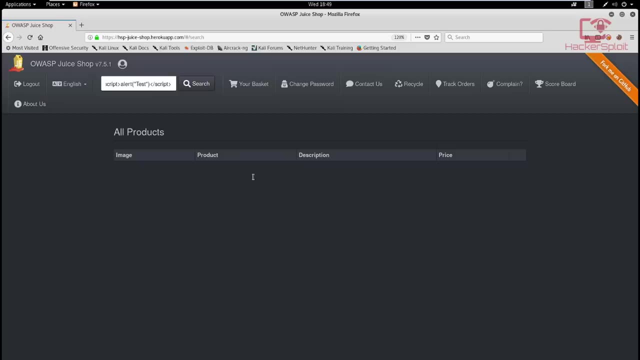 And I'll just call the password password And I'm just going to use name of your favorite pet And I'm just going to say dog, right over here, I'm going to register And we're just going to save that. Alright, so I can log in now. Did I log in with the correct? 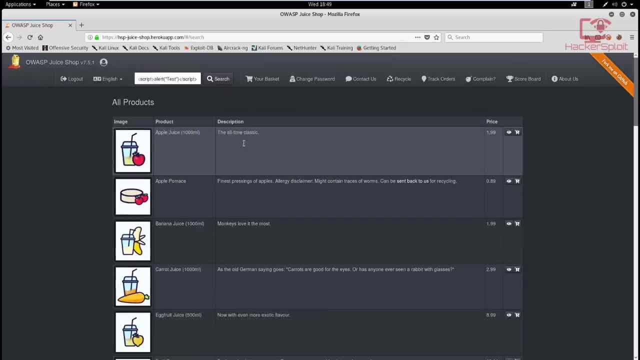 test. Yeah, there we are. And when I log in and we are logged in, Alright, so let me just zoom out So the interface does not really crash on us. Let me just get rid of that, Alright. so it's sorted out really well. we have the language selector here, your basket, which essentially 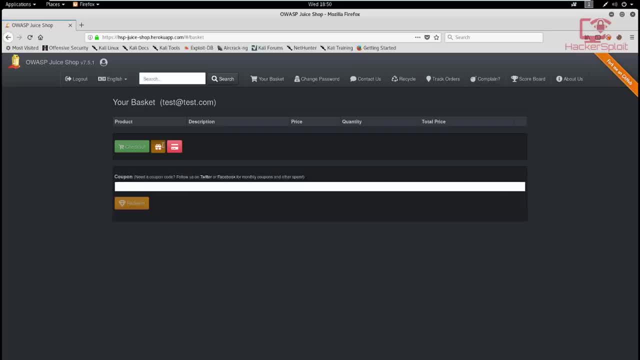 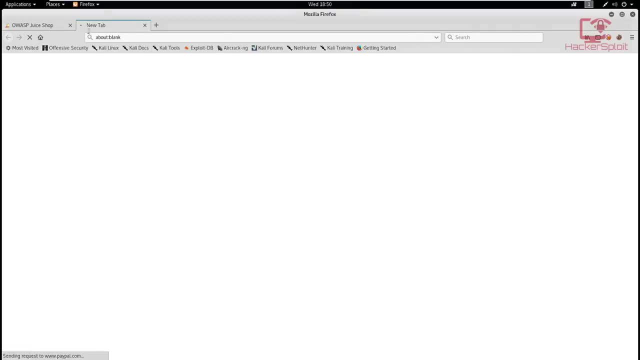 allows you to select your, to view the items in your basket. you then have your coupon if you want, if you want to use a coupon- and you have your checkout, which essentially, I believe, takes you to the the OS do shop donate page, if I'm not wrong. Let's just see if that is correct. 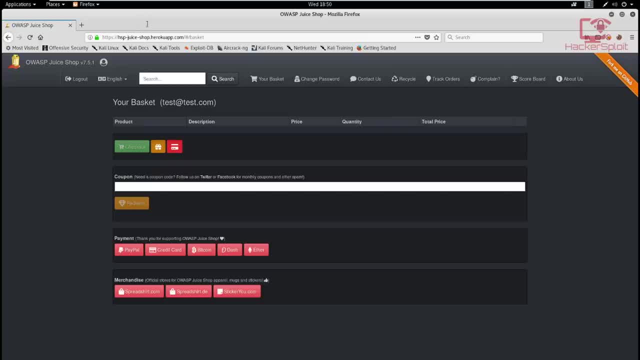 Yeah you. so if you want to support the project, I would recommend you know you can donate to them. it's it's a really great project. So if you want to support the project, I would recommend you know you can donate to them. it's a really great project. 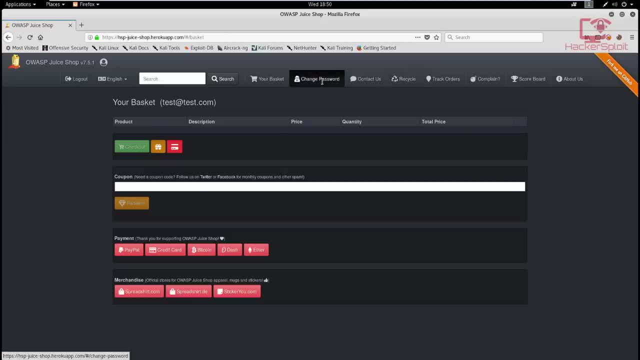 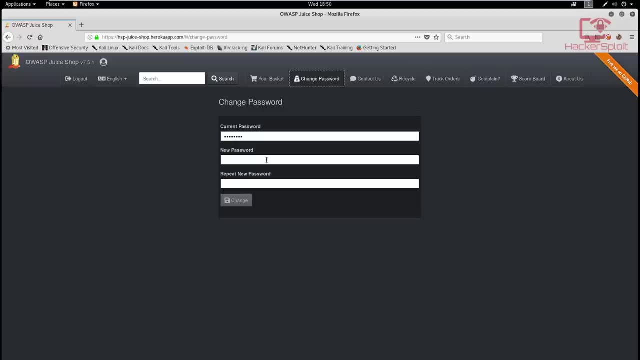 I really do recommend that. if you can, you do so So you can change your password, which is awesome. I think we also took a look at this- and how to change it using using the get requests, Contact us, where you can essentially write in. you can contact the, the person behind the site. 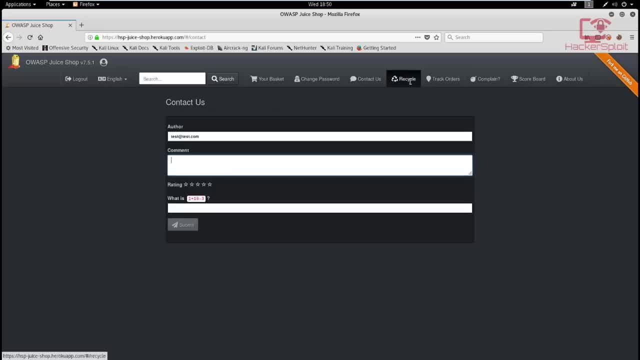 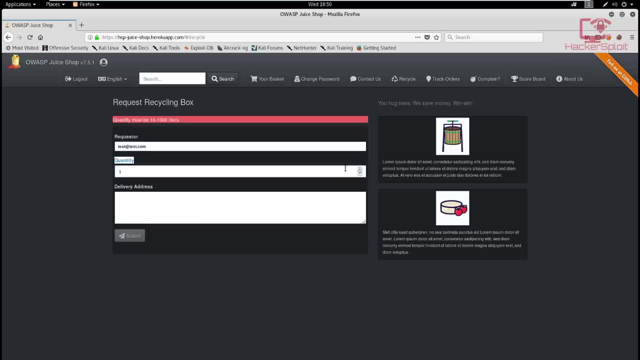 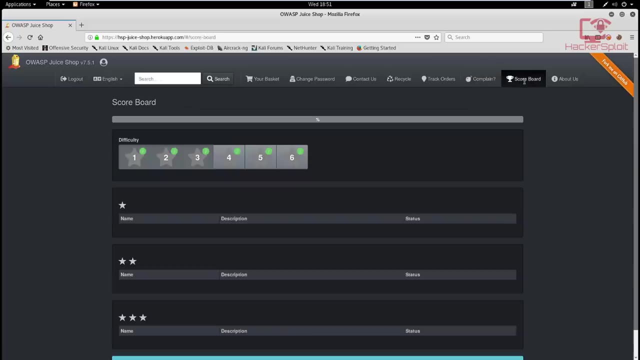 or the administrator, as I would believe You can comment: recycle, recycle. what's this request? a recycling box So you can type in liters here? that has a selector? All right, Okay, that's not too bad. We have a complaints board and the scoreboard itself here, which for some reason keeps, doesn't. 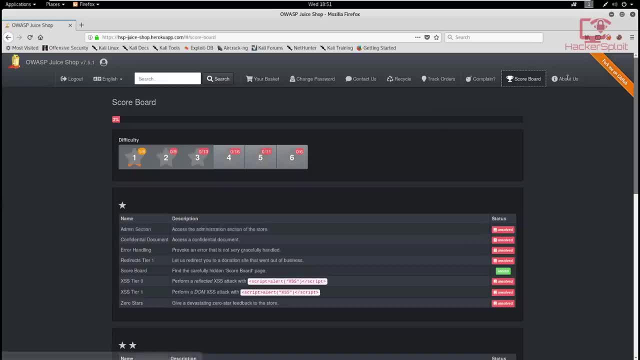 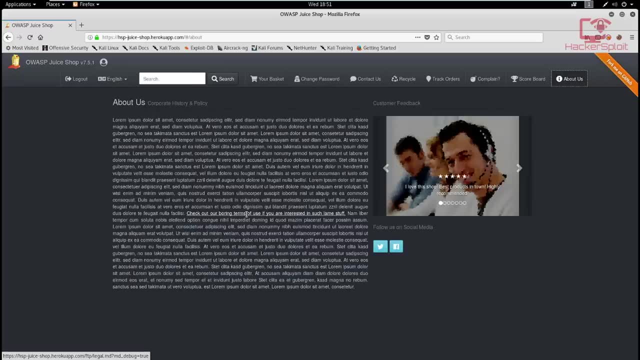 really load. So let's try and work on the first section. As I mentioned, I'll try and cover as much as I can here And you have the about us here that has some sort of a- let's see, some sort of checkout or boring terms of views. 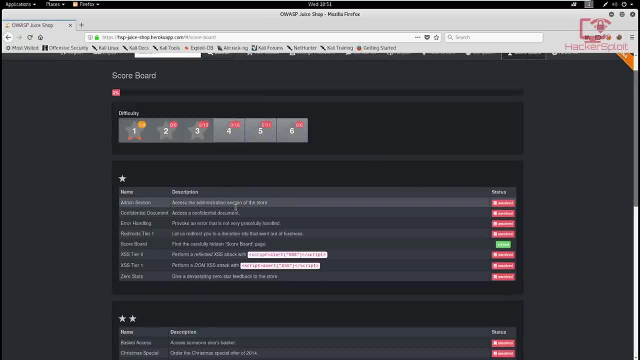 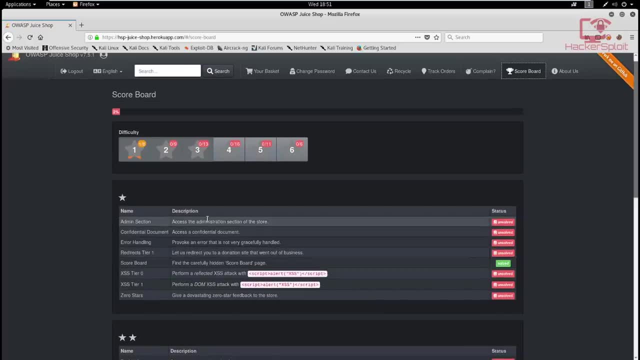 Let me just check the scoreboard. What exactly are we supposed to do? because access the administration section. What's in the two star here? login with the administrator, All right. so we're trying to access the administration section, So let's try and access that right. 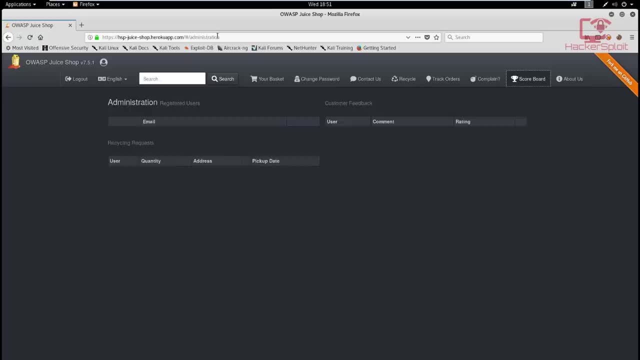 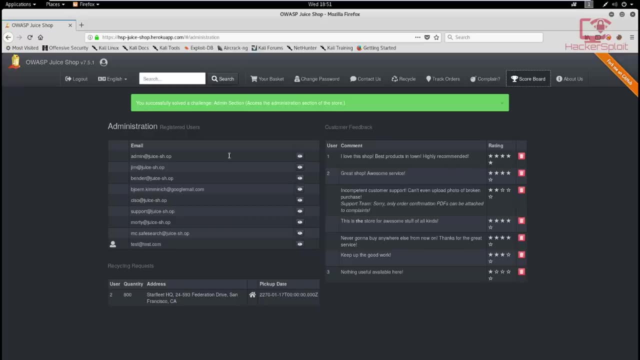 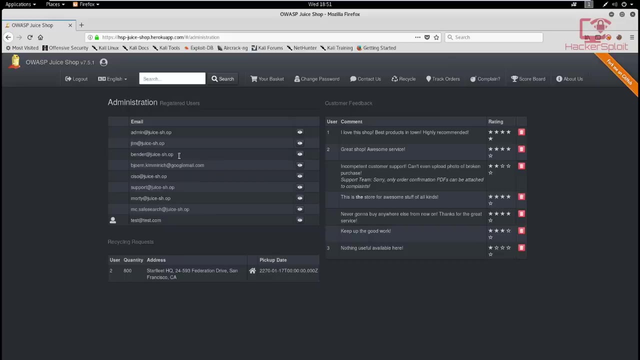 over here. So I'm just going to type in administration, like: so I'm going to enter and yeah, that was pretty easy And we get the email right over here: admin and do shop. That's the main email and we have all the emails right over here. So we have Jim and juice, do shop, bender and 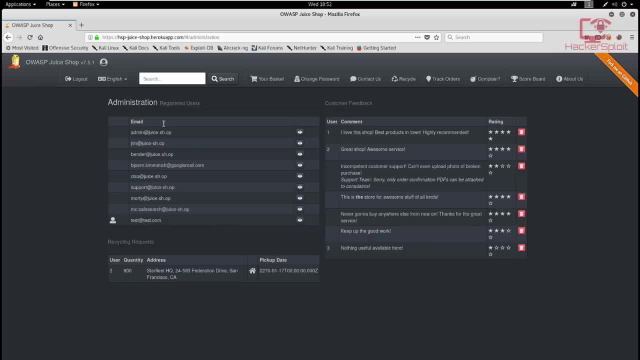 some other users and we have our. so yeah, alright, so we got the registered users, customer feedback and the recycling requests that have been posted so far, which means we're starting from the basic. so I think we can try and log in with admin, but we don't know the password, So yeah, so I'm just 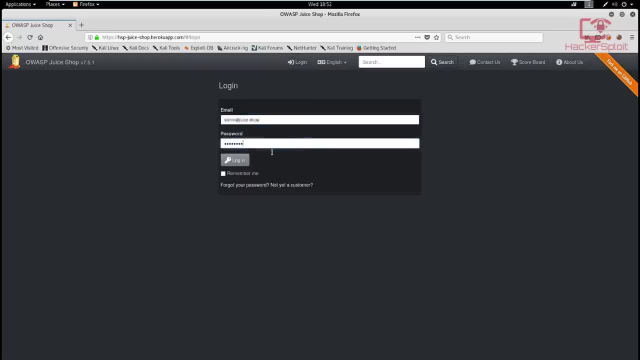 going to log out And let's see if we can log in with the password here, admin, I do shop and I probably- I'm probably- guessing- we have to use SQL injection And in this case I think I know what to do because I have done this before, But it has been changed quite a bit since the last. 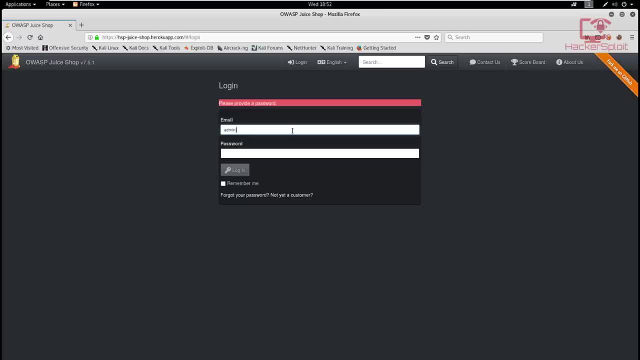 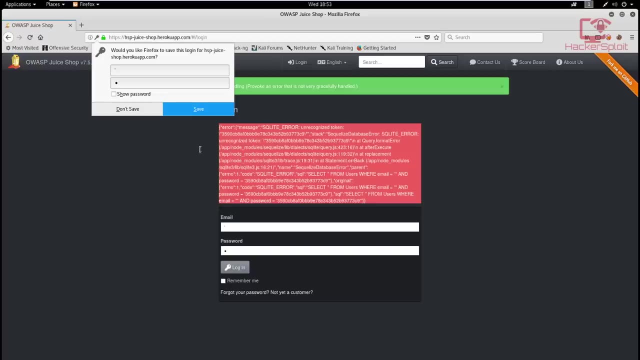 time, because I think in the previous versions it was with admin only there was no domain, or was there username? I'm not too sure. Anyway, let's try and see if we can throw some errors here. I log in, alright, so that means you have to provide a password, So let me just try and use. 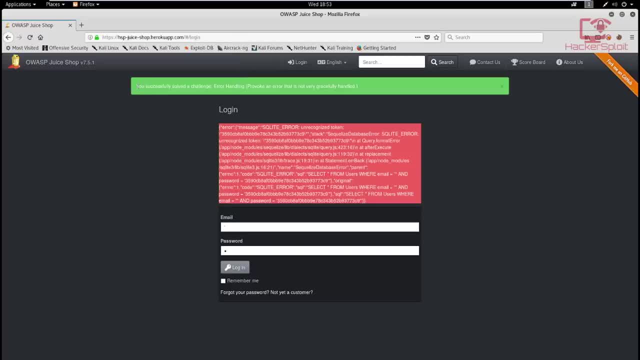 the single quotation And let's see if that, Yeah, it does throw an error. And, yeah, we completed the other challenge which you successfully solve, the challenge error handling provoke an error. So, yeah, so essentially performing error enumeration, if that's something you've never heard of. 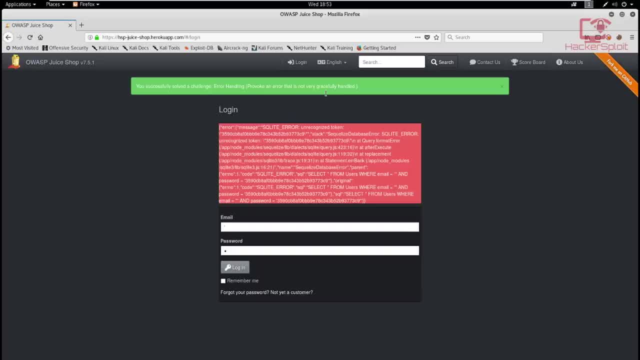 it's essentially where you just try and see how the CEO is fuzzing, really just throwing you know information at a system, seeing how it responds, And we get here the query. So we are performing SQL injection because, as you can see, tells us, here we have the the query, right over here. 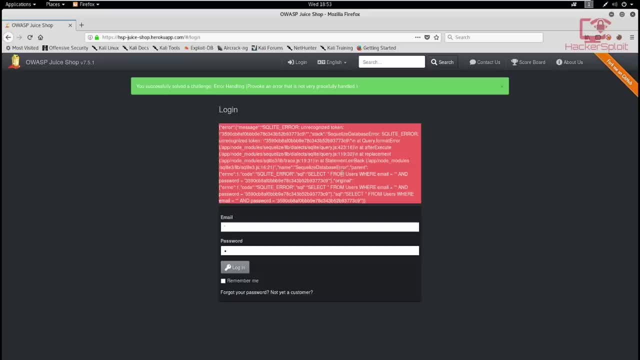 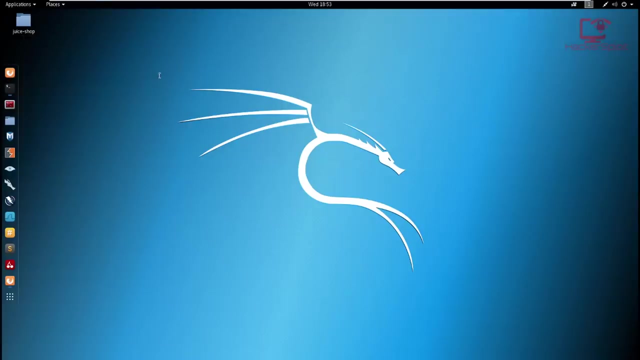 which is telling us select, And what this is saying is select all entries from the user table where emails are equal to and we specify the single quotation And the password is. what is this? this looks like a hash. What hash is this? Let me just check. I'm think it might be MD five, I'm not too sure. Let 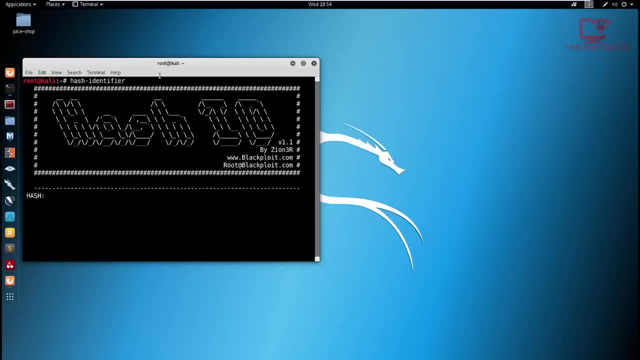 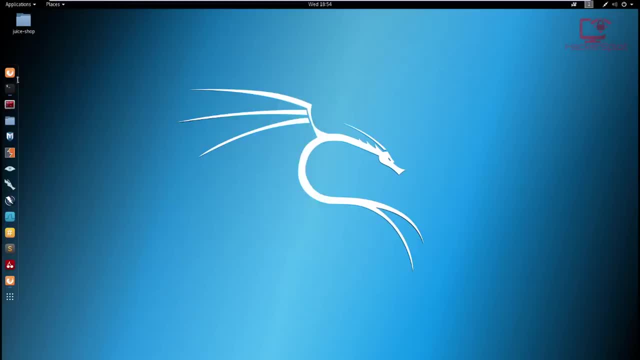 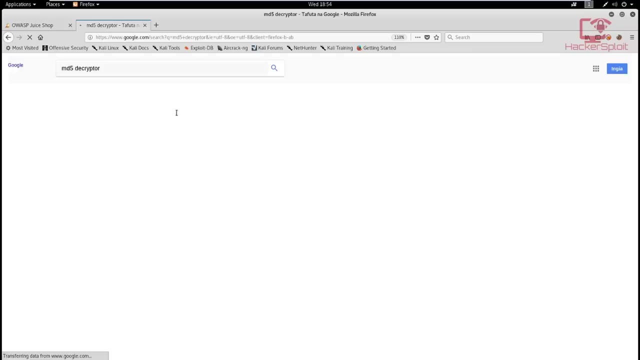 me just check this hash identifier And we just paste that in there. Sorry about that, Let me just paste that in there. Yeah, this is MD five hash, So that probably. let's just see if we can decrypt that or decode that. So I'm just gonna say MD five decryptor or something like that. Let's just see. 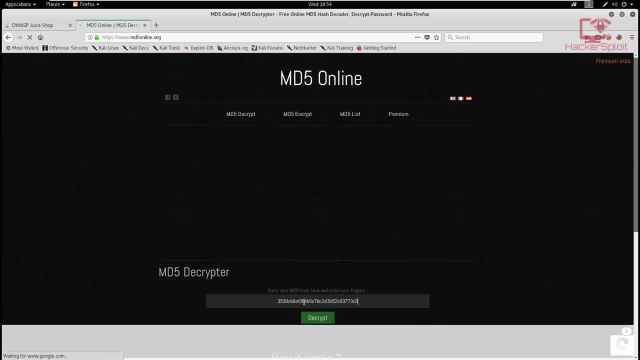 if we can do this online Really, really quickly. Come on, come on. I want to see what error, because that's telling us that's a password. Let's decrypt that. And well, for some reason, it's taking too much time here, So yeah, 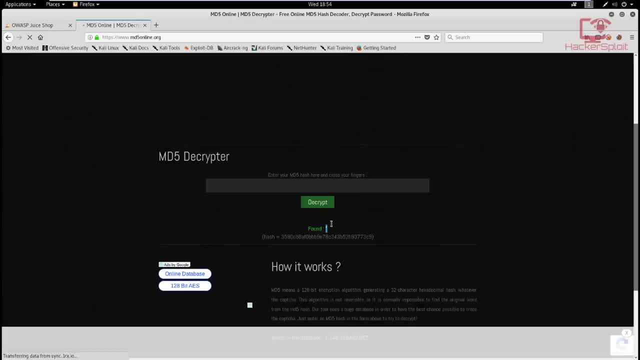 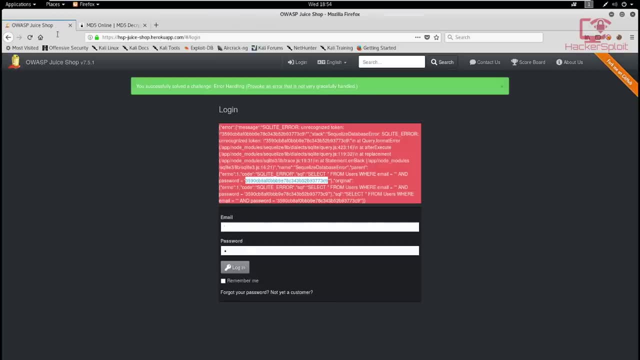 yeah, it's essentially hashing the password. Alright, interesting stuff there. We actually now know that the password is being hashed, Obviously, you know, with the MD five hashing algorithm or protocol, whatever you know, call it so original. And yeah, that is the. 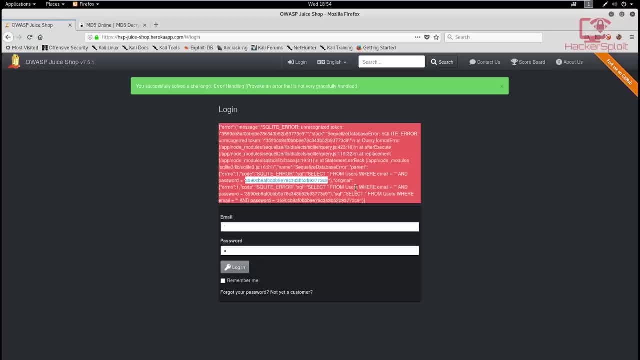 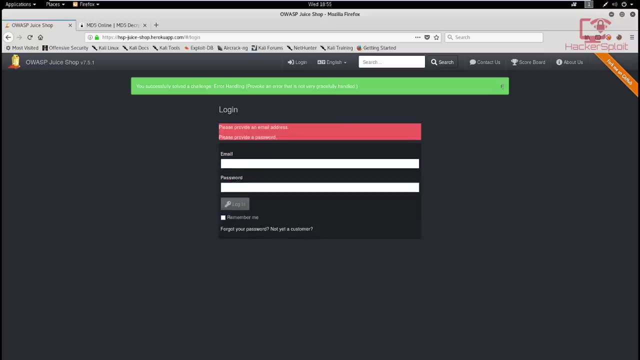 query statement there, So we can try some basic SQL injection And some of the basic ones to log into admin or to essentially log into the administration. The admin panel is now. the thing that's weird is: are we going to use the password? here we're trying to get authentication. 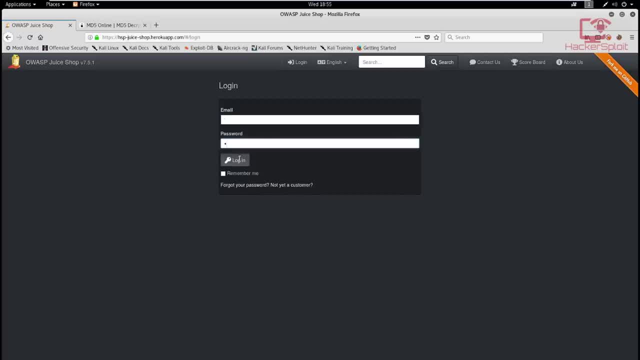 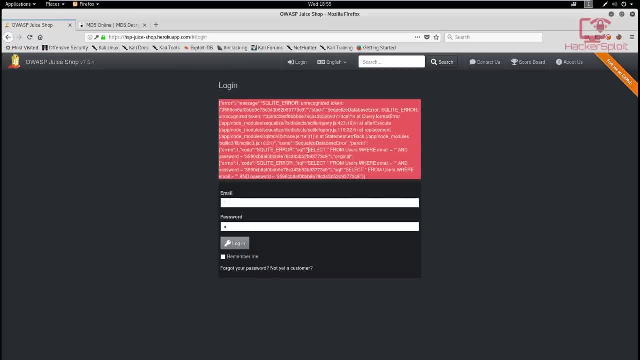 So that means- let me just close that That means if we just throw the error one more time or get the when you're able to get the query here. So we're saying select actually starts from there, Select from users. So select all queries or all. 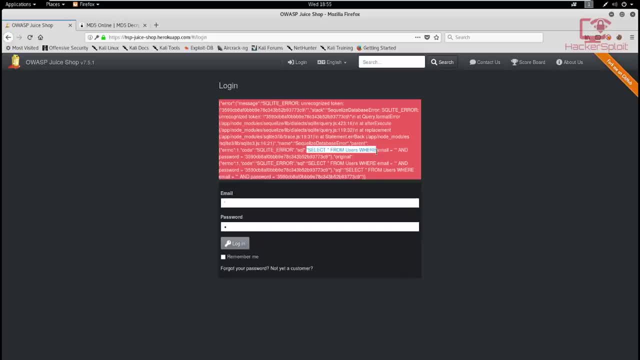 entries from the user table. from where email, user table. So there's users. Alright, so the user, the user table as email and password. okay, I follow now. So that means we can try, we can try, we can try and use the or statement here And probably we can use the. 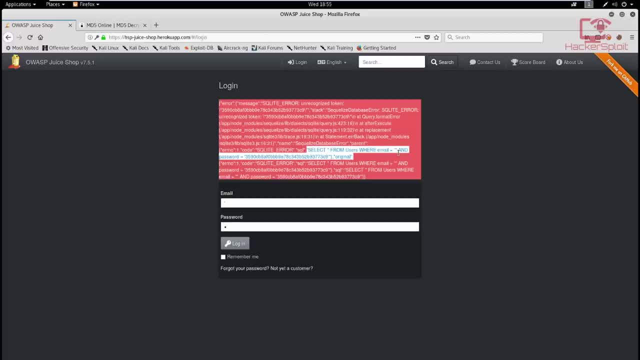 not statement. if we are going to, Yeah, that will make a lot of sense, But we only using email, So we'll keep the single quotation. So what that means is is, if you know about SQL injection- hopefully I can explain what's going on here- So we know that the password is being hashed, So we're 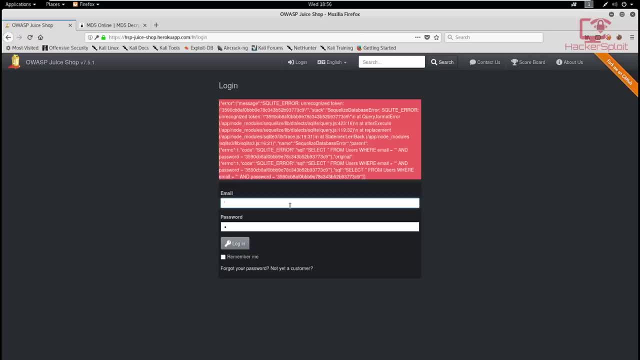 saying select from the table where email and password- So that's the statement. So select from the table for so sort of select from the users table where the email and password is going to be equal to, is going to be equal to what we have entered. But remember the the 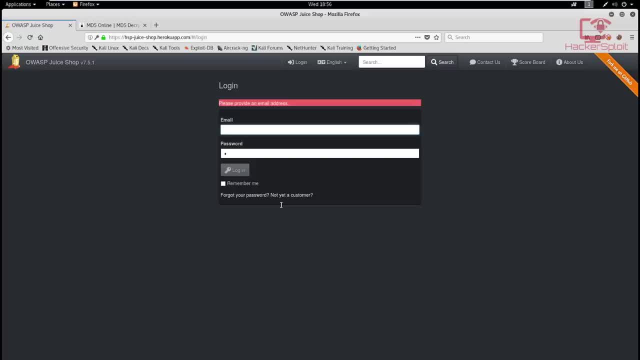 password has to be, has to stay as the single quotation. So that means, yeah, we are going to be using the or. So this is basic use. you guys should be knowing this. But if you want me to cover it, let me know. So or equals, or one equals one, and the other ways of doing this. I think I'll 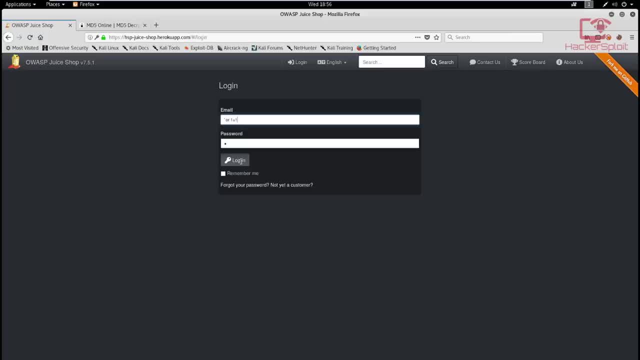 post a cheat sheet in the description section And check it out for yourself, just to get up to scratch with what's happening here. So what we're saying is we're using the or the or. the syntax of or is very simple. It's where we have the what's. 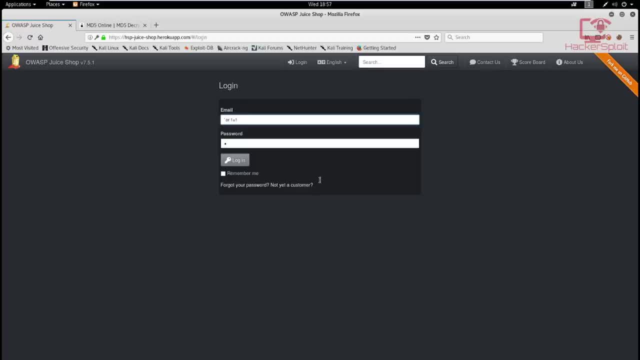 happening here is we're saying we're saying okay, so you've. if you know, the syntax for how a query is made in SQL is really very simple. So we're saying select from from the table. Remember, this is specifically a table, not a column. So it says select from the users table. 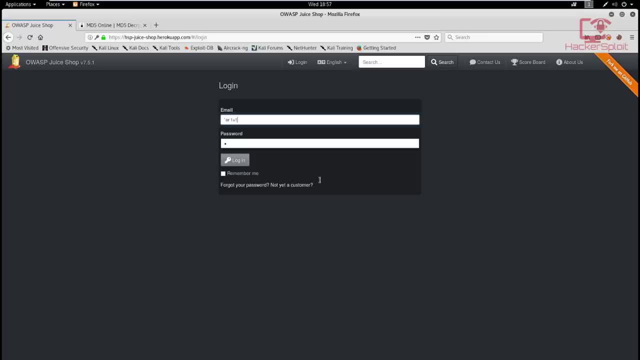 from select from the users table email password, So comparing, and then we say all and then we specify the condition where the value we can enter are in two fields. So we can say: the value of the email can always be changed And we obviously know that that is the first account that was created. 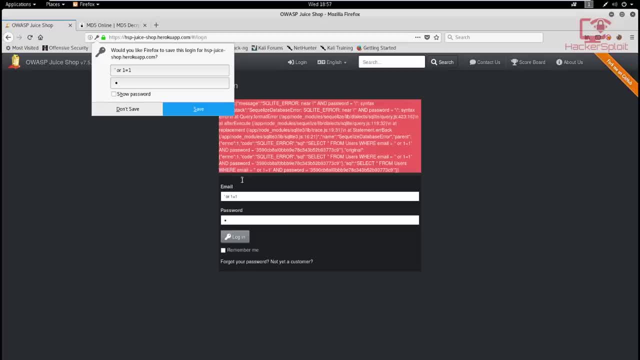 And the password is going to remain the same. So we hit login And, yeah, we get. still keep on getting an error here. Now that is weird. No, because if I specify, there is no comment here, Or one equals one. Yeah, so it is working. So you? 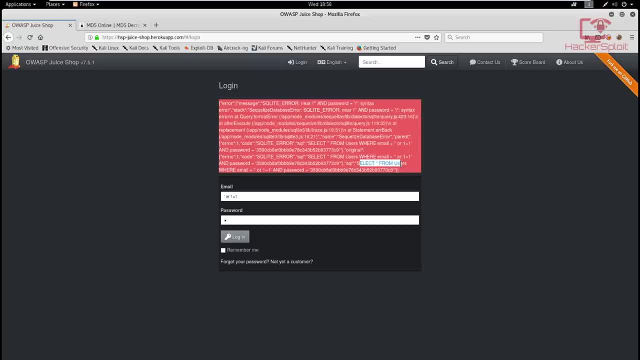 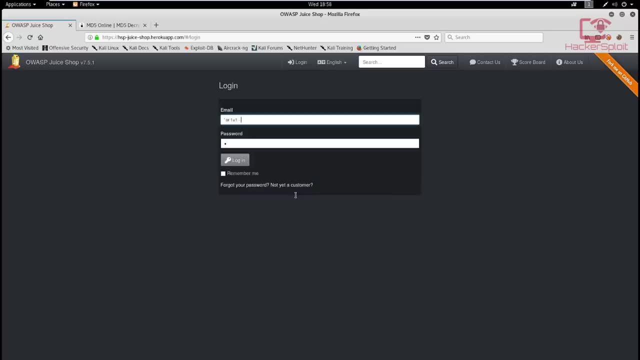 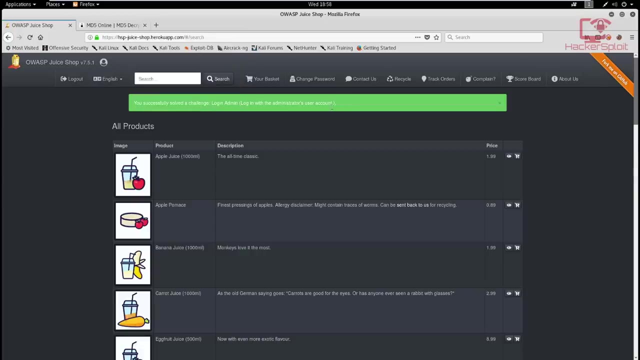 can see. so select from users where one equals one and password. Yeah, so we want to nullify and password we don't want and there, so for that we use the user comment here And there we are excellent, So we're able to log in to the administrators user account. Alright, so let. 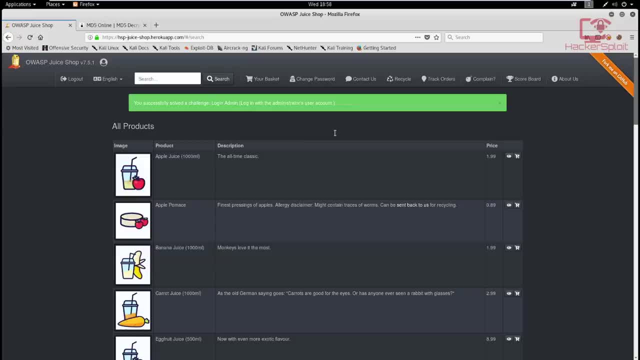 me explain what happened there. So, as I said, the, the syntax or the query was as follows: So we're selecting from the users table, we're selecting the email and password and comparing them to each other So they have to match. So we're performing a query, a simple query, And what we said is, or that's a conditional. 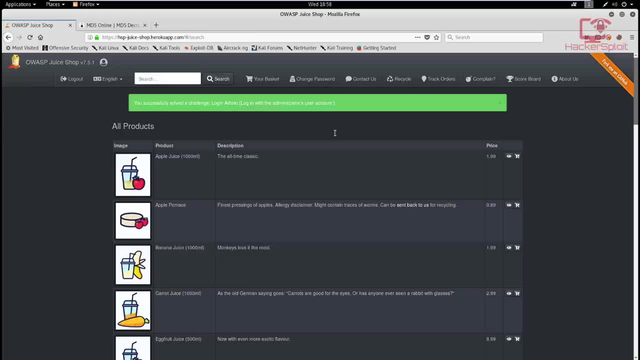 statement. So we're saying, or that we specify the condition where the first value is going to be equal to the, the first one is going to be equal to one, And we nullify the, the password, where the password was essentially removing authentication. And we are what? because we're including the 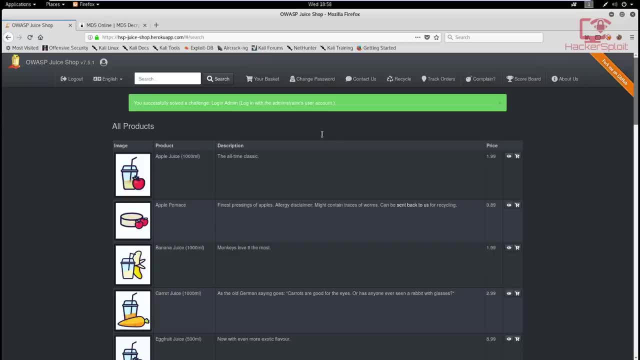 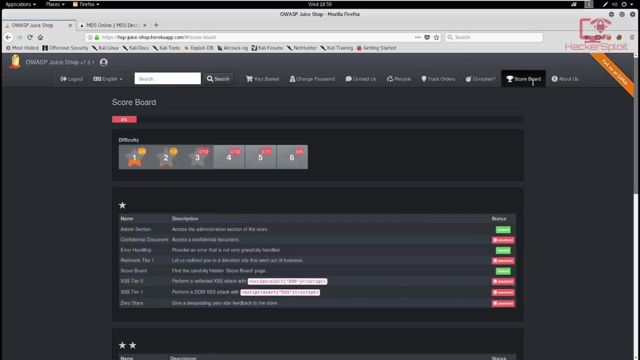 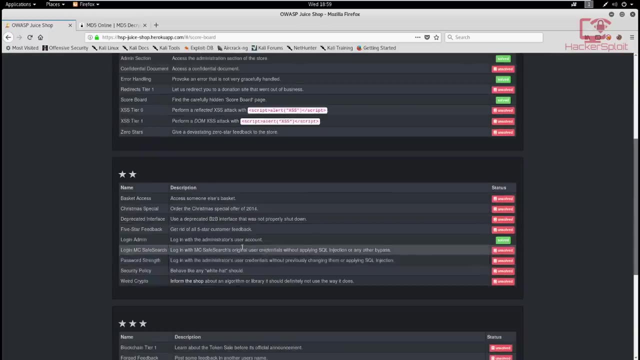 comment: syntax for SQL. Alright, so that was pretty simple. But now the thing that's bothering me is we don't have the password. So let me just check the scoreboard And let's see what progress we've made so far. So we've accessed the administration section, that's. 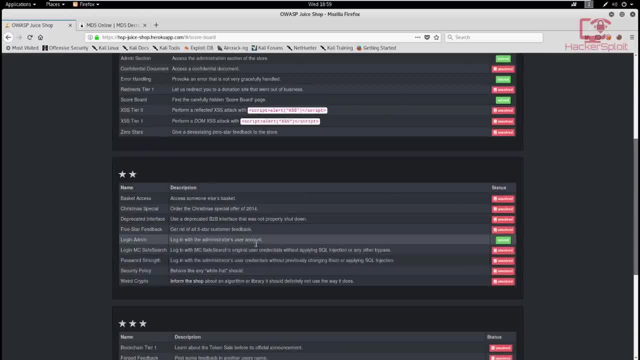 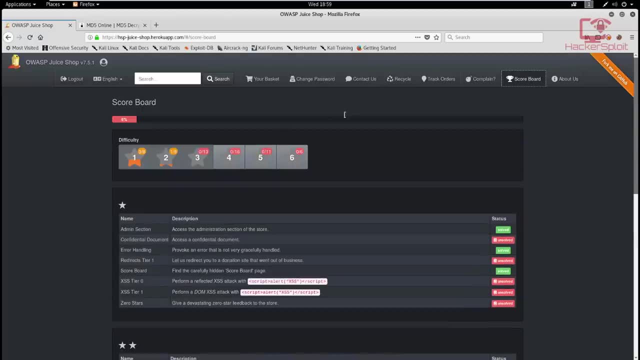 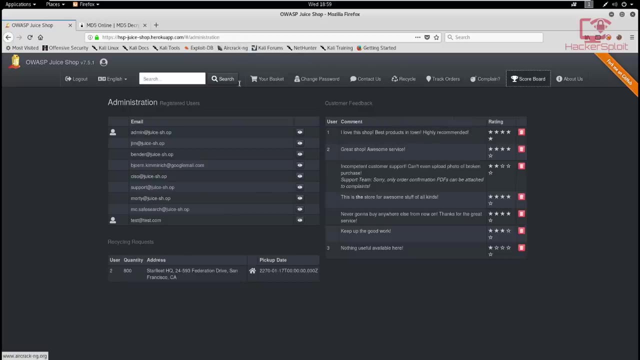 not in here. that is in here. So log in with the administrators user account, But I don't know the password. So I think that's how we're going to be logging in. We know the email, because if I just go back into administration here- administration- I hope the video is not getting. 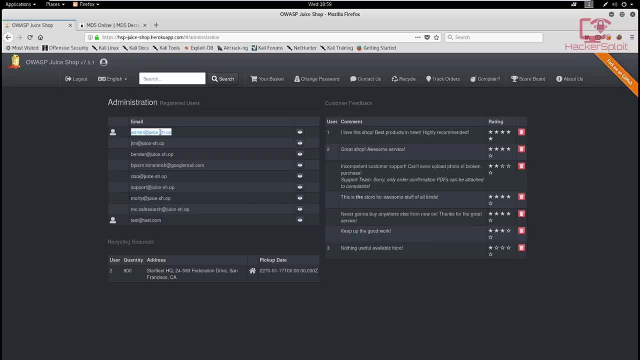 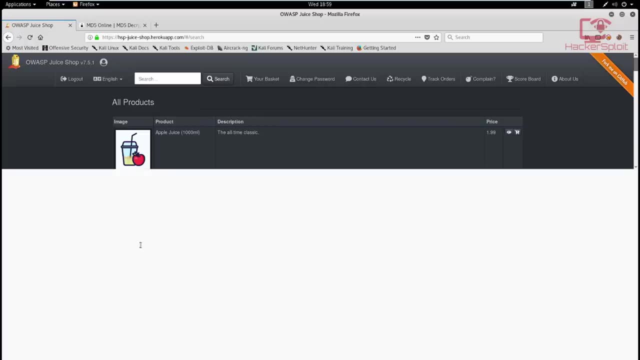 too long. So we have the admin, We have the admin email here. Oh, yes, yes, yes, yes, we have the token. So if we inspect the element and we go into the cookie editor, for example, we can use that. 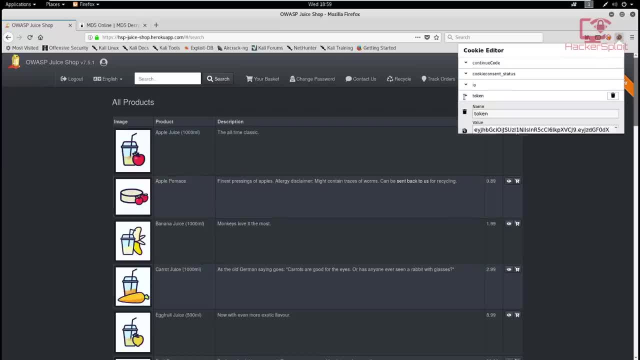 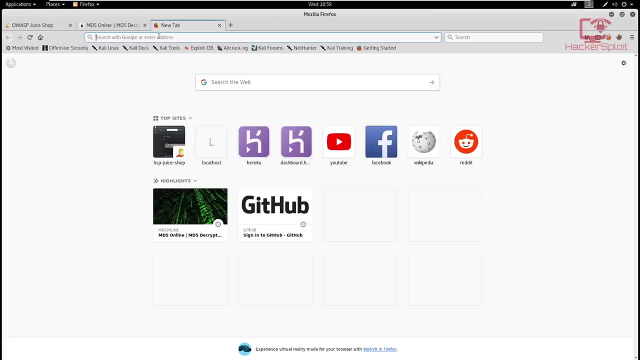 Or you can just use storage. Well, I should have done it, you know, from the cookie editor from the beginning. So we have the the token here, And I talked about this in my other video, actually went through this with the token, So. So we're going to say token. I think the site was. 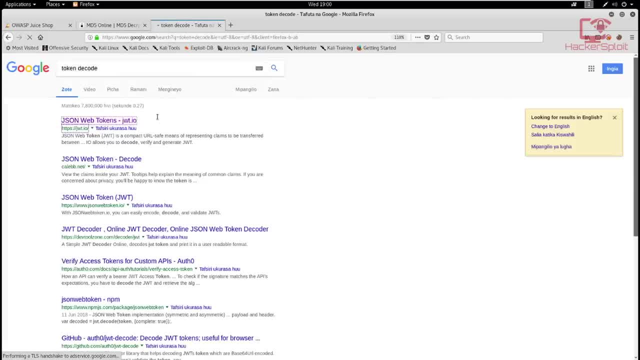 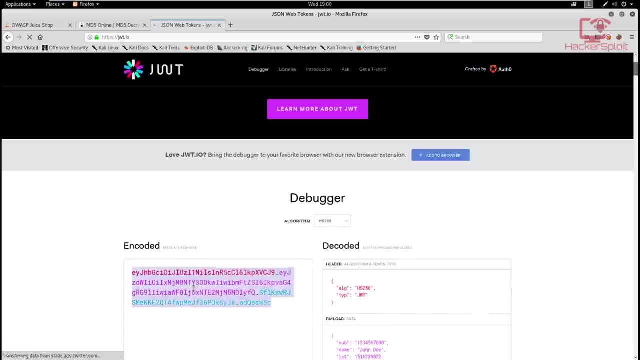 it's a JSON tokens, a token decode, And should be the first site here- their JSON web tokens. So JWT dot IO. that's an excellent site And we talked about this, So if you want to watch that video, I'll post it in the description. 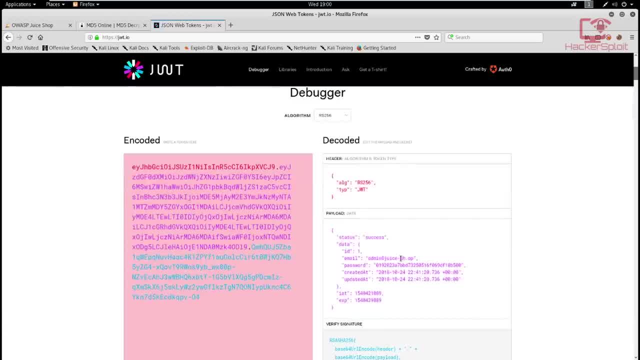 So you can check it out. And the email is admin, So that's the authentication token And that gives us all the information we need. Alright, so we have the password here. But again, what is this hashed into? That looks like md five again, but let me just confirm. 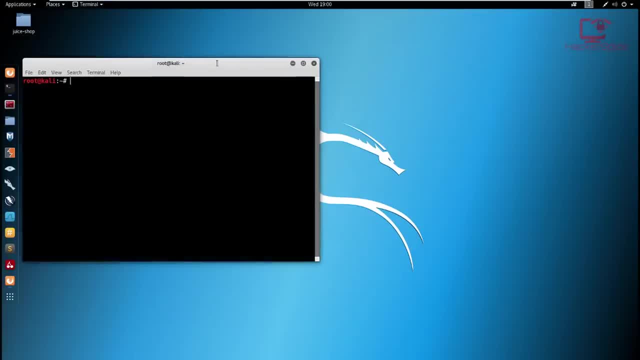 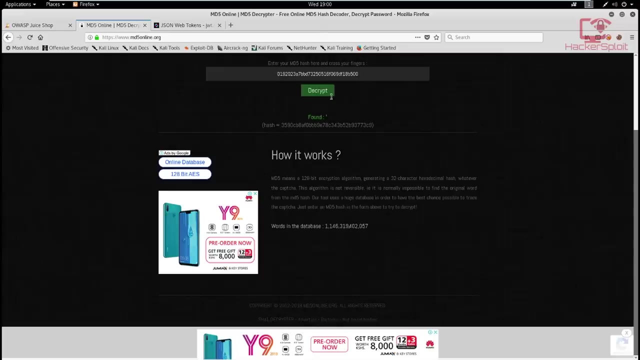 and let's see what that gives us. So the password is hashed, as we know, with MD five. So let's just confirm hash identifier. because there we are. yeah, it is MD five, So let's just decrypt that one more time. So I'm just gonna paste in that hash there, I'm just going to decrypt. 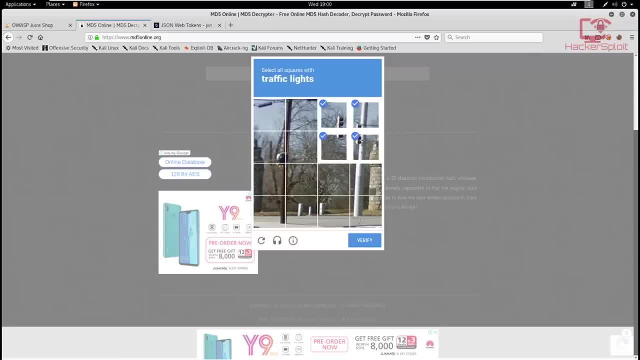 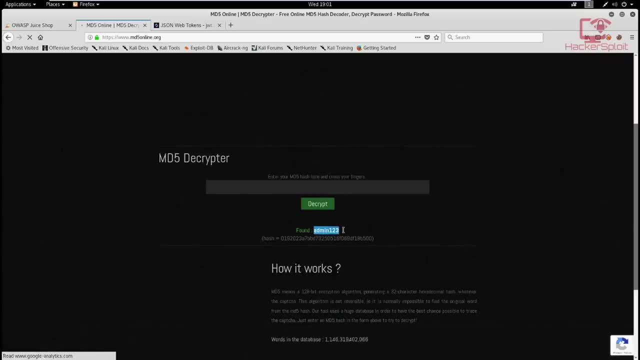 Let's give that a few seconds. Oh my god, man, all the traffic lights And let's hit verify. And yeah, there we have. the password is admin 123.. Yeah, that's, that's pretty basic, But again. 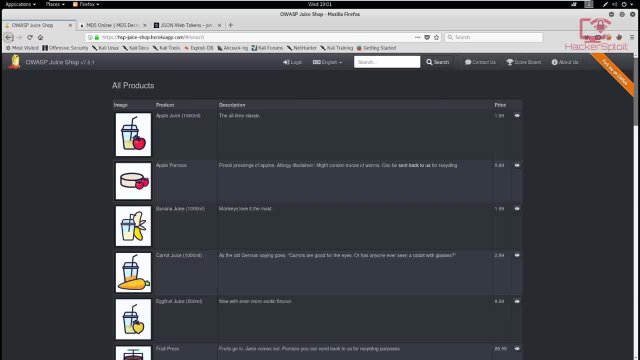 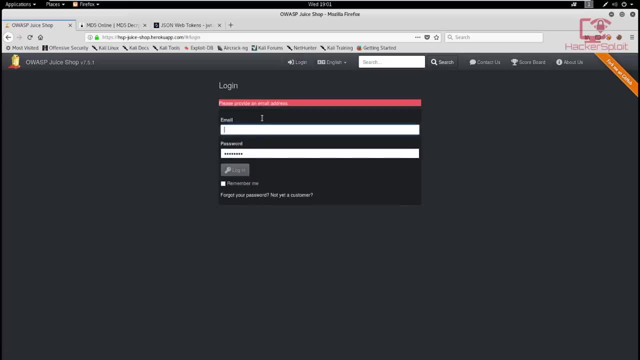 replicating common practice that you would find. So what was the email? Oh boy, what was the email. Let me just log back out, Crack Alright. so let me just use the statement: So yeah, we're logging in, So all one equals one, because we're. what is the? I think we can access the, the email from the. 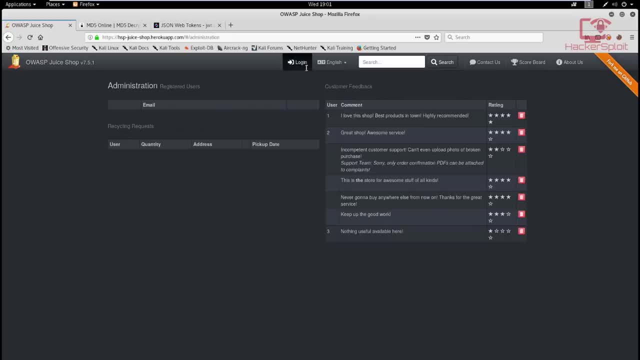 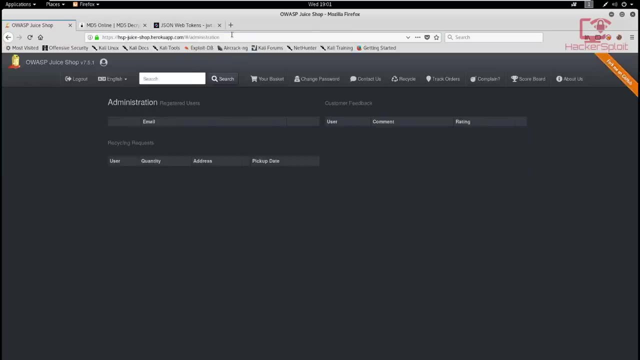 administration. Sorry about that, guys, I know I'm getting really mixed up. Well, we're not logged in yet, So anyway, let me just log in And we can do the administration here. station and the admin address: Shop at juice shop: a juice dot op. Yeah, that's there to confuse people, So you can guess it. 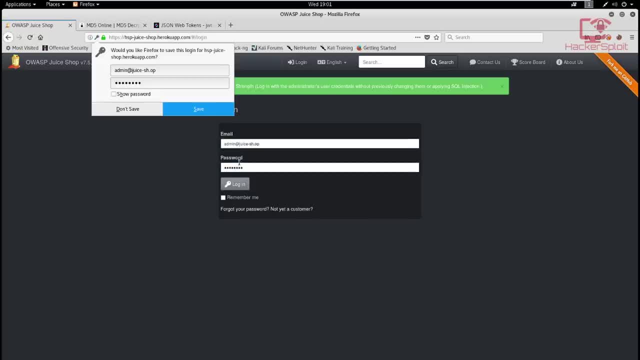 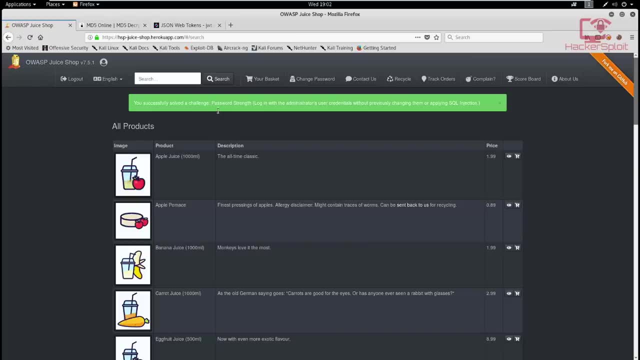 And we're logging in with that And the password is admin 123.. I'm going to log in And, yeah, fantastic, So you solved a challenge: password strength. So that was the problem there, that that's the vulnerability that they're trying to say exists. So you know again: password strength. 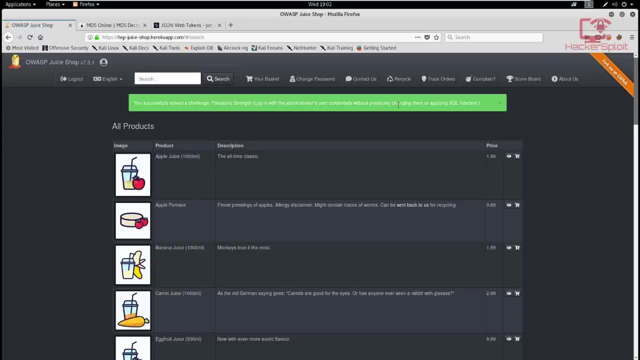 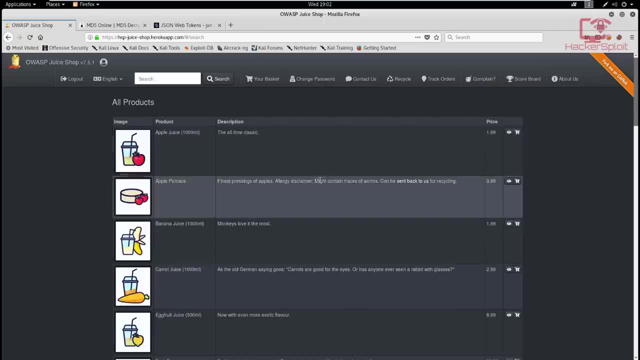 is something that people don't take into account. login within message, you user could credentials without previously changing them or applying as cute. Could you have done this with SQL injection? Probably I'll have to cover SQL injection because you know SQL injection is one. 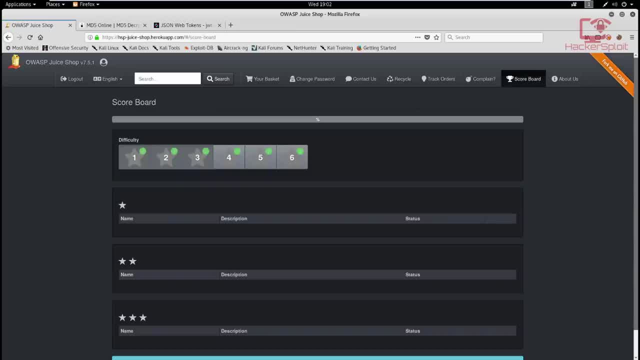 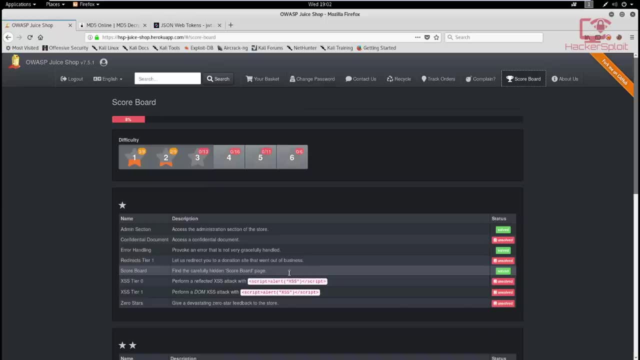 of those things. that's really dependent on the query. So let me just go back to the scoreboard here. I don't understand what else is left. There's still a lot of stuff that I have to cover. I talked about cross site scripting, but I think I'll cover that in the next video. I'll explain it. 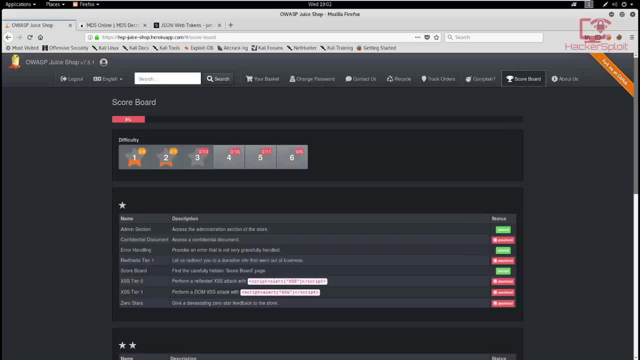 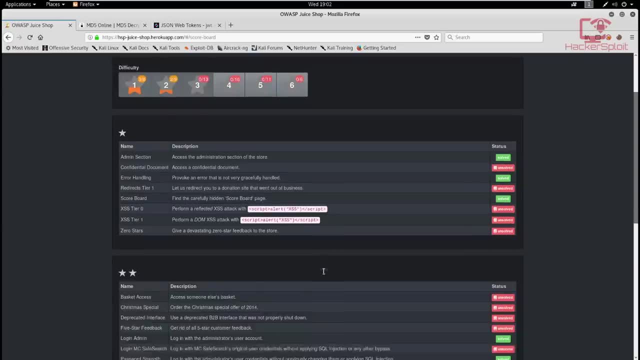 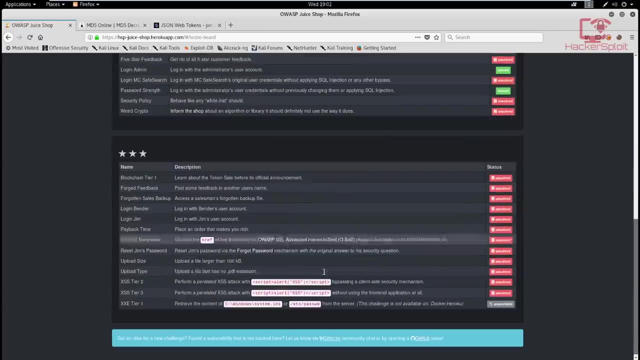 again, What is the? what is the? the confidential document, error handling or we don't have anything much there. access someone else's basket. I did that. What else should I want to cover here? Let's look at these ones right over here. So yeah, so the authentication area here is where I want to look at. I think that's what I'm. 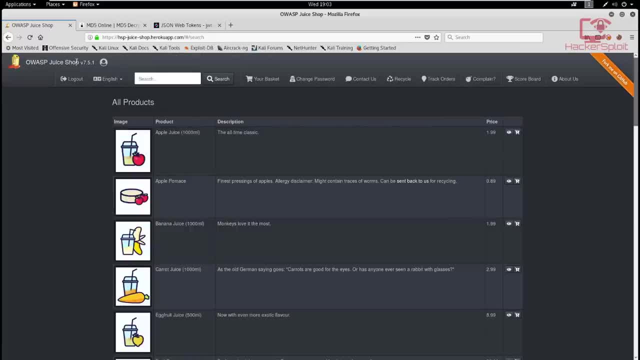 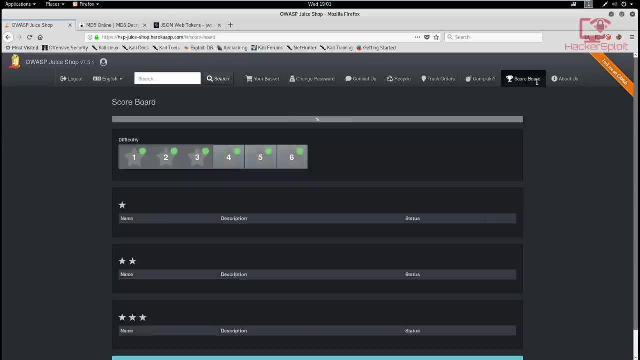 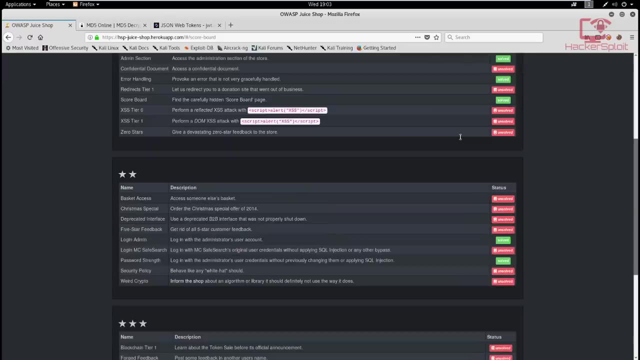 going to end this video. I know I haven't covered any advanced stuff, But hopefully that's like an introduction. So we, where we have been able to log into the administration's in the administrators account, we're able to get the scoreboard, the administration panel, what else we're able to do, we were able to. 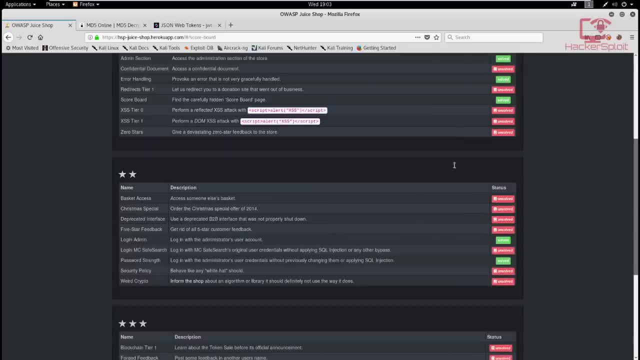 provoke an error not signing on. nothing really complex there And we were able to log in with the administrative at the administrators cred user credentials. We looks like we can actually get access to MAC safe search original user credentials. So again, another user that we 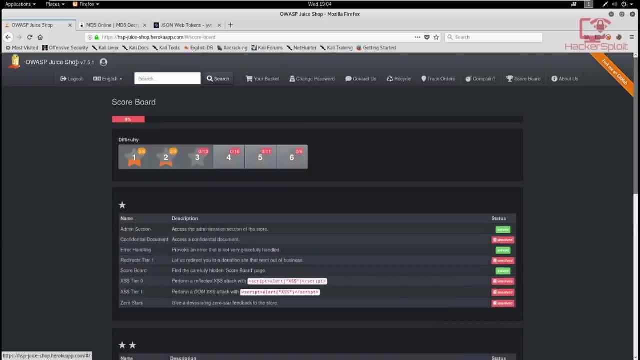 can try and get access into. Yeah, that's going to be it for this video, guys. If you found value in this video, please leave a like down below. If you have any questions or suggestions, let me know in the comment section, on my social networks or on my website and I'll be sure to leave your reply. and I'll be seeing you in the next video. Peace, guys.